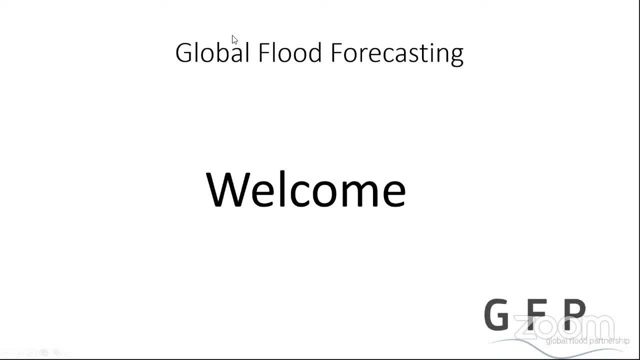 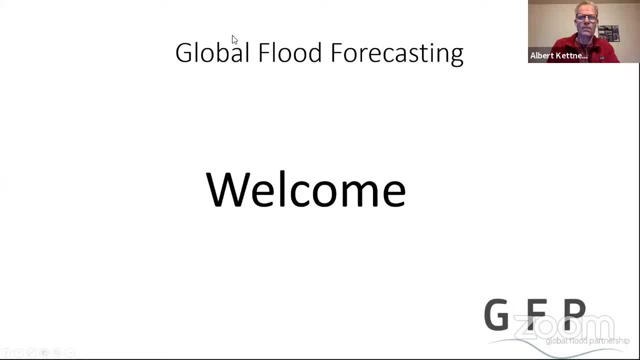 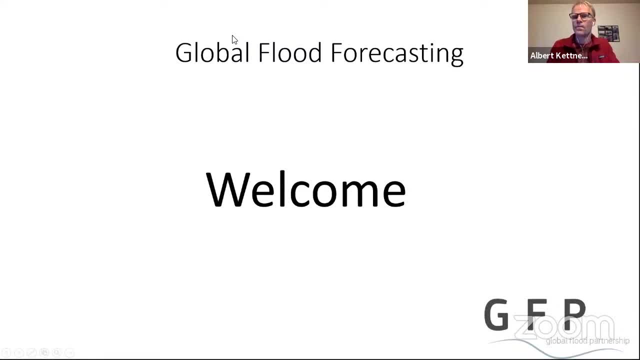 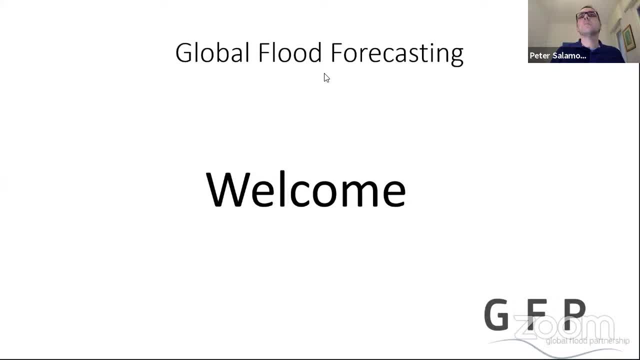 Thank you. Okay, I would say we start now. So good morning, Good afternoon, Good afternoon or good evening, depending on where you are, to everyone. My name is Peter Salamon from the Joint Research Center of the European Commission. 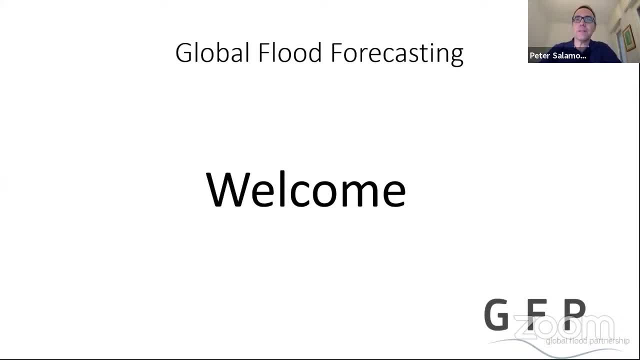 I'm chairing today's second Global Flood Partnership virtual session on global flood forecasting, together with Roberto Rudari from the Chima Foundation, and also with the help of Albert Gettner from the University of Colorado, So it's really a pleasure to see again so many of you here today, and let me see if I 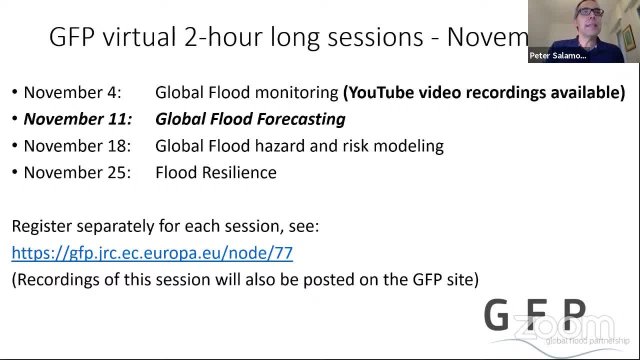 can change the slide. So today, as I said, is the second session of the series of Global Flood Partnership virtual assessments that we are having. The last one last week and the first one that we actually ever made was really successful And I hope many of you have seen it. 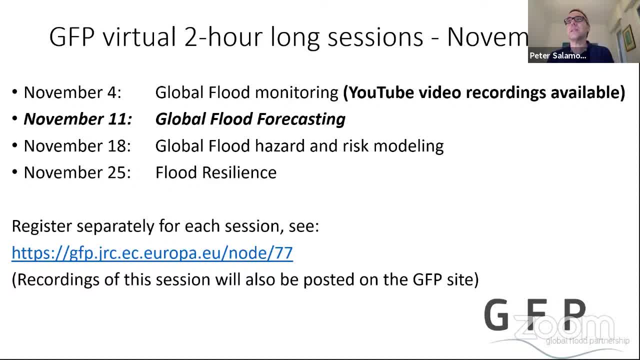 For those that haven't, there is now the YouTube video recordings. The links are now available on the GFB webpage in the section where the virtual sessions are described. So, but let's move on now with today's session, which is on global flood forecasting. 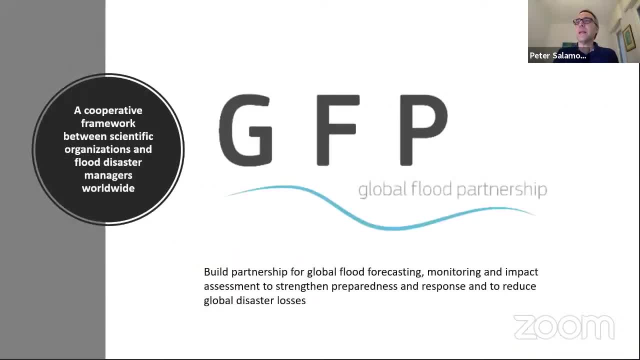 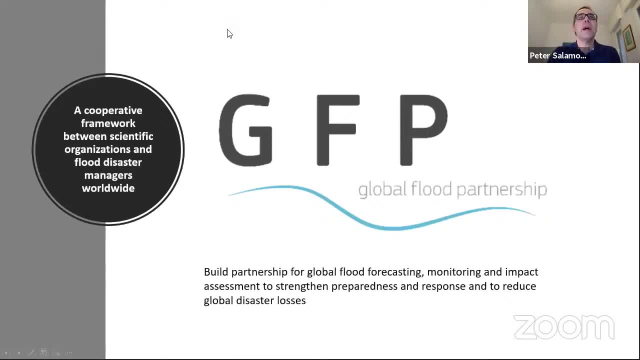 Because I mean, many of you that are here today have either heard this already last week or know, have been to the Global Flood Partnership meetings before, or know a little bit about it, But I'm sure there's also some newcomers. So just a quick reminder. 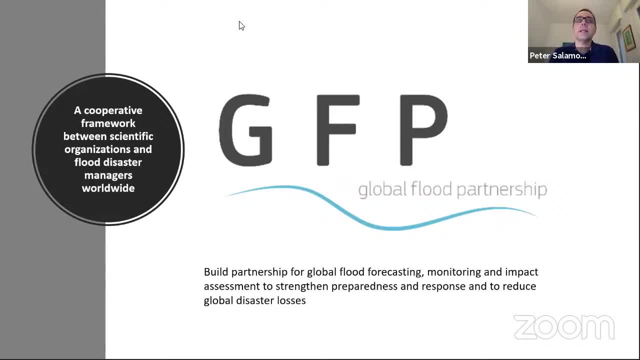 The Global Flood Partnership is really about building a framework, a cooperative framework between the global flood partnership and the global flood partnership, And so I'm going to start with you. So, first of all, I would like to start with you, So I'm going to start with you. 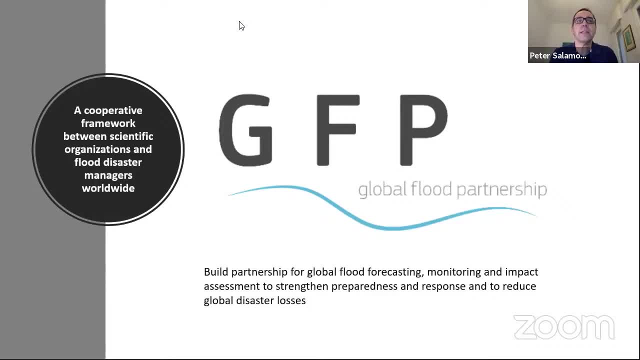 So I'm going to start with you, between scientific organizations and flood disaster management managers worldwide, to really build a partnership between those groups and look at how we can commonly bring forward all the global tools that we are working on in relation to flood risk management. 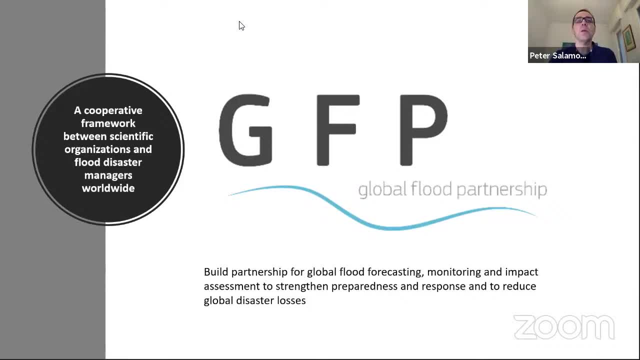 So global flood forecasting, global flood monitoring or global flood impact assessments, And really make use of those tools in order to reduce the impacts of floods worldwide, which is really the main aim of, probably, or hopefully, of all of us. So, really, this bridging the gap between science and users. 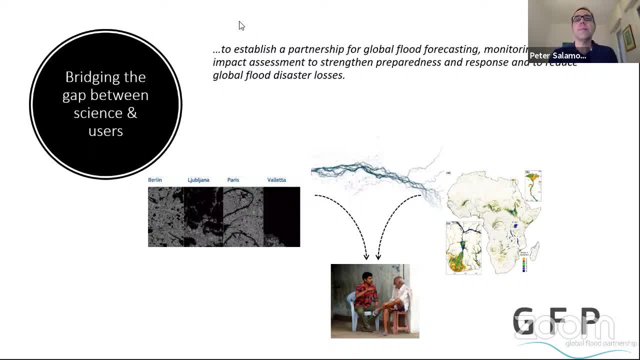 is really at the heart of the Global Flood Partnership And, as you can imagine, this is even more so important when we are trying to use global tools that we are developing and trying to apply them for local problems in flood risk management. So this is really a big challenge. 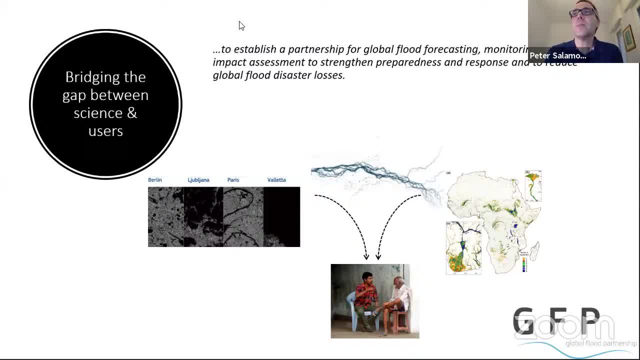 And here we try to really establish a dialogue between the end users, or possible end users, and the scientists and the developers of those global tools, to make sure that we can really make a change and an impact in improving flood risk management. There's a number of ways how we do it. 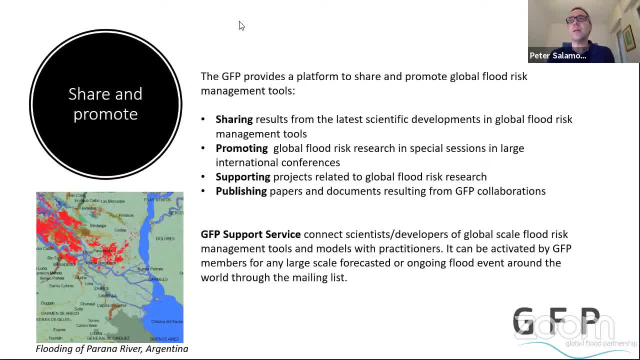 There's a number of ways how we do it. There's a number of ways how we do this, how we try to build this framework and bridge the gap between science and users. We try to share the latest scientific results or promote global flood risk research. 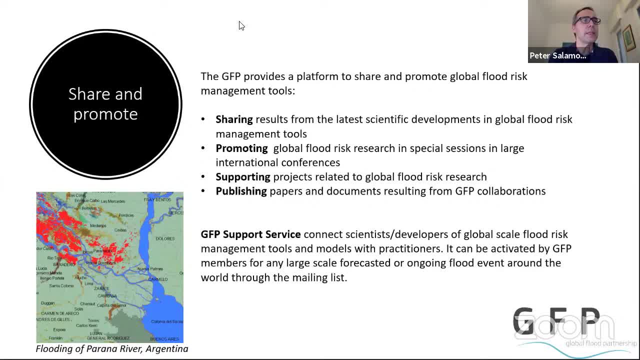 We also try and support projects. One of the key elements that we have in the Global Flood Partnership is the support service that really enables, through a simple mailing list, access to the information that is available to the public, So for in the case of a flood happening somewhere in the world. 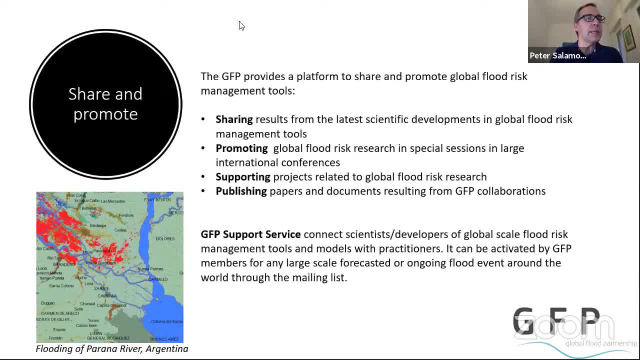 to be able to ask if somebody in the Global Flood Partnership may have some information- be it a forecast or be it a monitoring map or some other information about exposure or vulnerability that he can share in for this specific emergency or event situation. Just the last word. 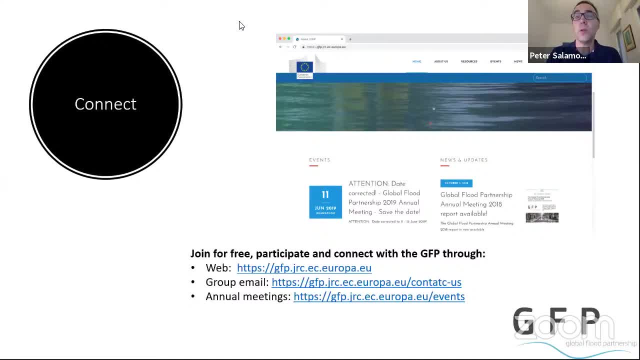 So if you want to find out more about the GFP, have a look at our webpage, or if you really want to be fully involved and then subscribe to our Google email group. you'll find how to do that on the GFP webpage. Usually we have annual meetings, but physically. 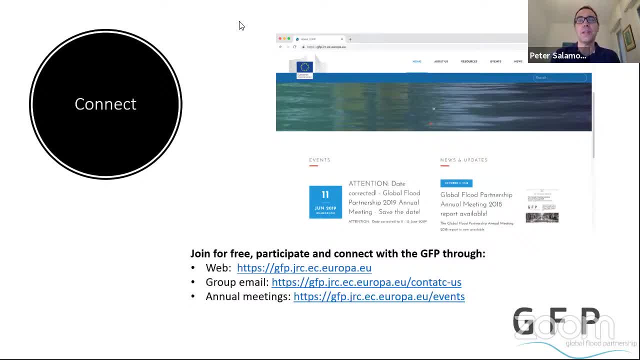 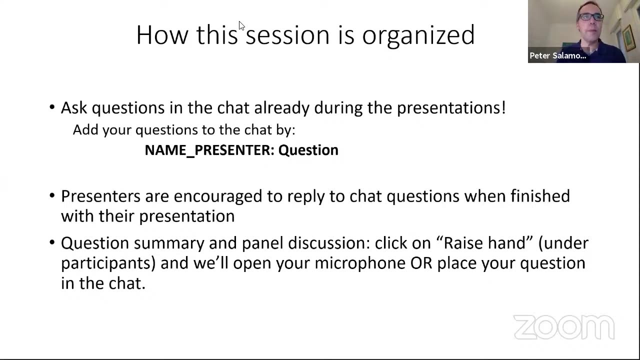 as you know, this is, due to the COVID situation, unfortunately not possible. So I hope you will enjoy now these series of virtual sessions And, having said that, a few administrative comments. So you are encouraged to ask questions already in the chat during the presentations. 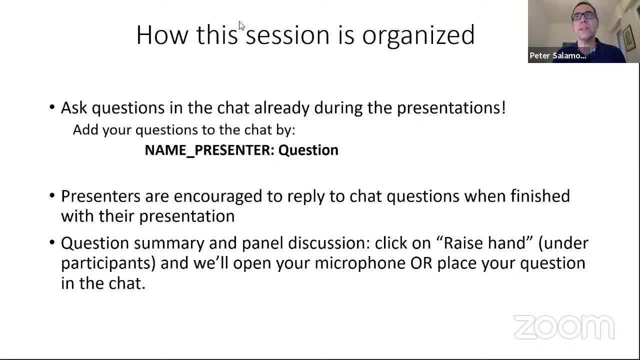 we will not have questions directly after the presentations, but we'll be able to summarize a few key questions at the very end after all all of the presentations and then have a discussion and the presenters will all will already reply to your questions in the chat. 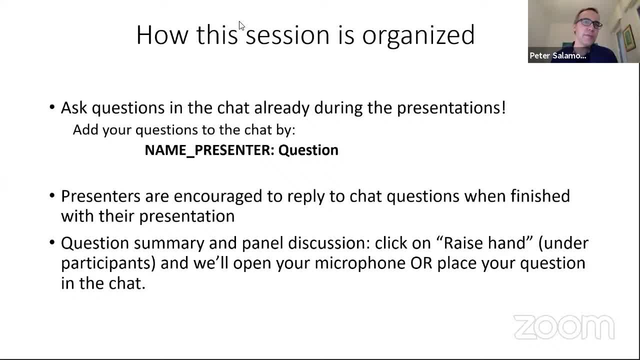 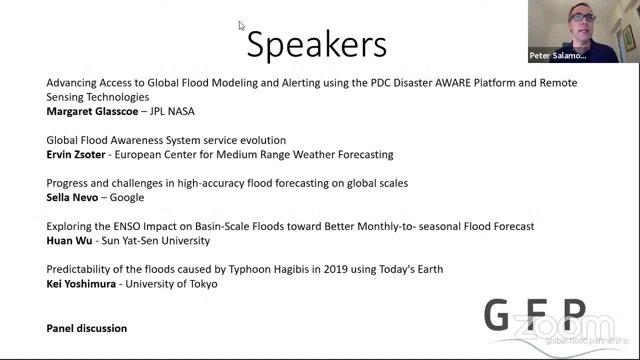 once they have finished their presentation And once if you want to then still have a question, or you have to raise your hand and we'll open up your microphone then at the very end, when we have still time for the discussion session Now today. I'm really glad to have those five speakers. 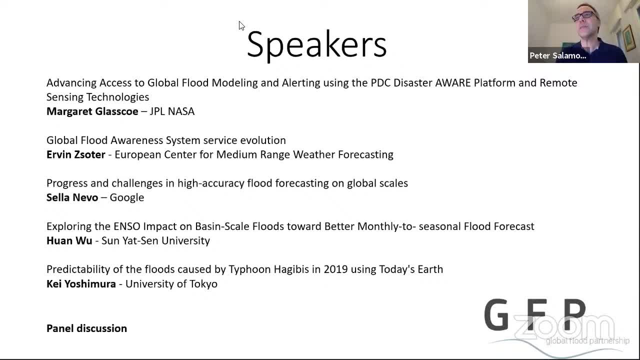 presenting really the latest state-of-the-art developments on global flood forecasting tools. So we'll start off right away with the first one, a presentation from Maggie Glasgow from the JPL, NASA, Advancing Access to Global Flood Modeling and Alerting Using the PDC Disaster Aware Platform. 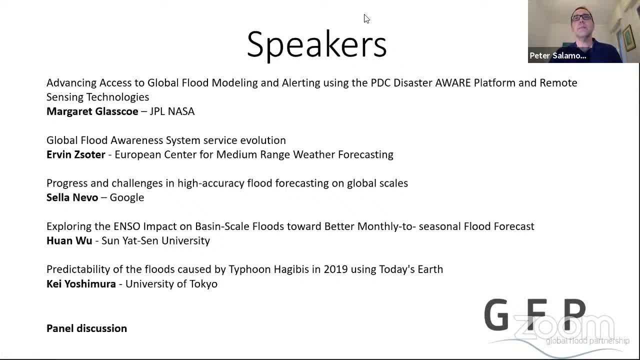 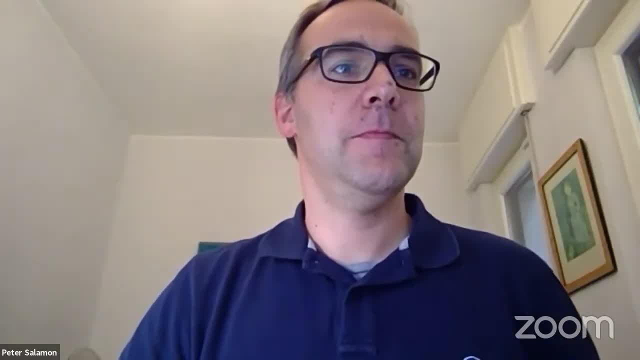 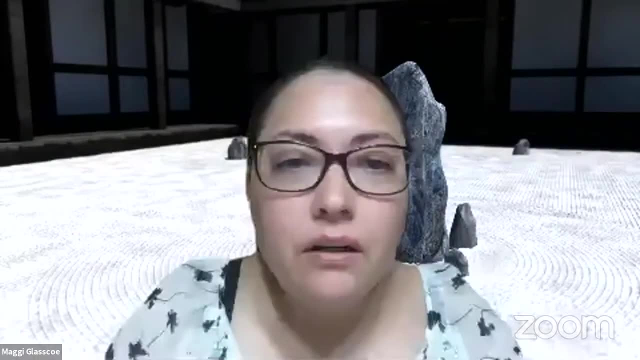 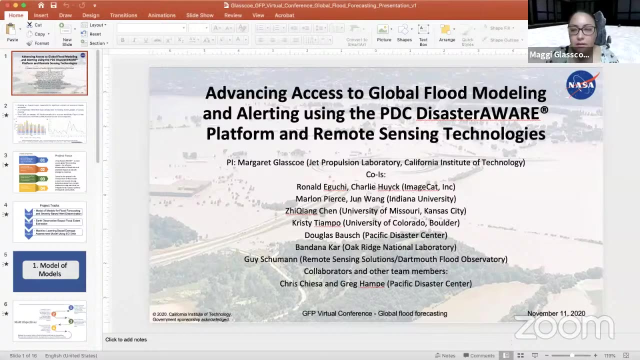 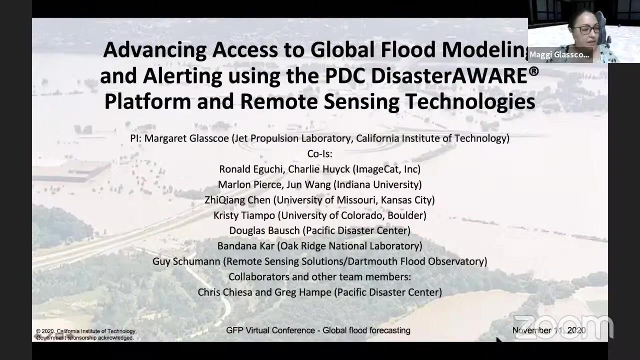 and Remote Sensing Technologies. So I stop sharing, Maggie, the floor is yours. Great, thank you so much. Let me start sharing my screen. And can everybody see my screen? Yes, Okay, great, wonderful. Thank you so much for the opportunity to speak today. 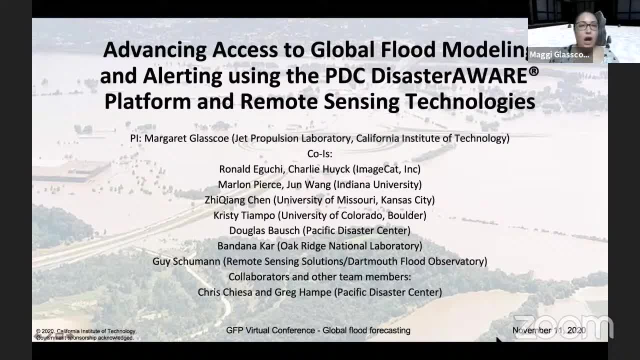 and good day to everybody. Thank you, Thank you, Thanks guys, Great, thank you. Thank you. Thank you, Maggie, for this presentation And, as Peter said, my presentation today is about Advancing Access to Global Flood Modeling and Alerting. 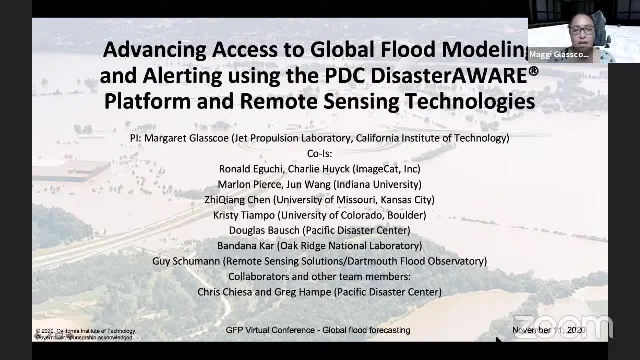 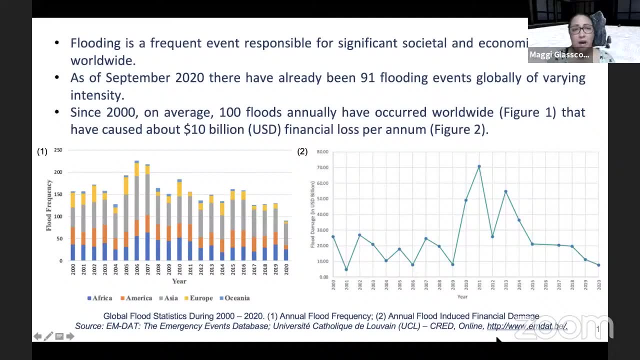 And this project is a large project with a number of co-I's, as are listed here on the title screen, And I'll jump right into it. As you know probably, flooding is a frequent event responsible for significant impact worldwide. worldwide, As of September 2020, there have already been 91 flooding events globally. 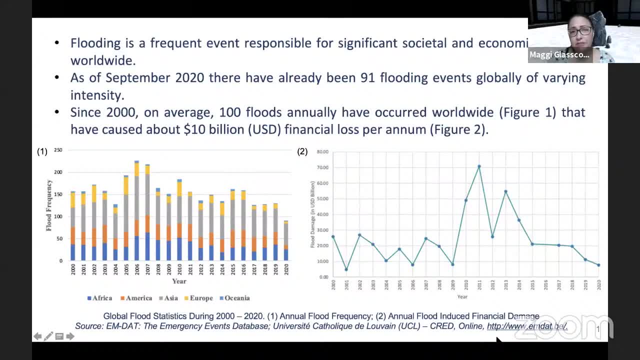 And since 2000,. on average, there have been 100 floods annually occurring worldwide that have caused about $10 billion US dollars financial loss per annum, And this slide shows the flooding frequency per year across the continents and the flood damage in US billion dollars per year. 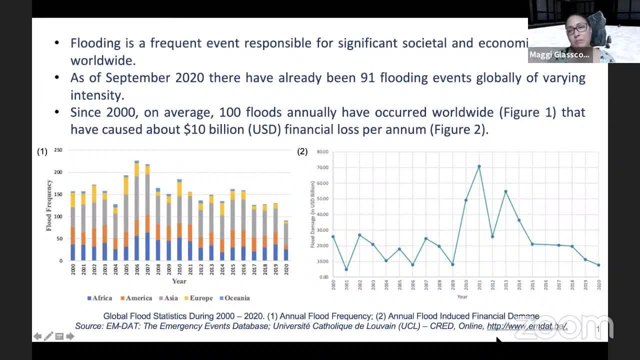 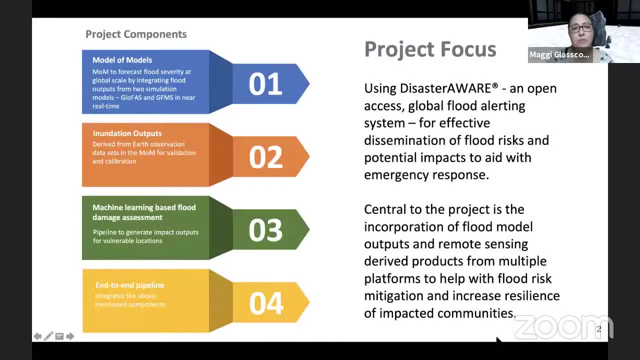 And, as you can see, this is a great global impact across the world. So the focus of our project includes four major components. It uses Disaster Aware, which is the PDC's open access cloud. It's a global flooding alerting system for effective dissemination of flood risks and potential impacts to aid with emergency response. 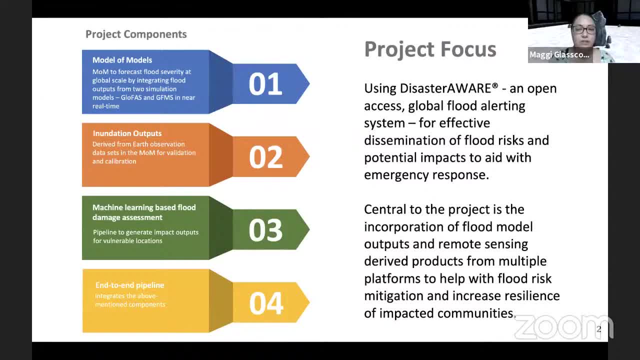 And central to the project is incorporation of flood model outputs and remote sensing derived products from multiple platforms to help with the mitigation of flood risk and increased resilience of impacted communities. The four main components are: a model of models approach to help forecast severity at a global scale by integrating flood outputs from two simulation. 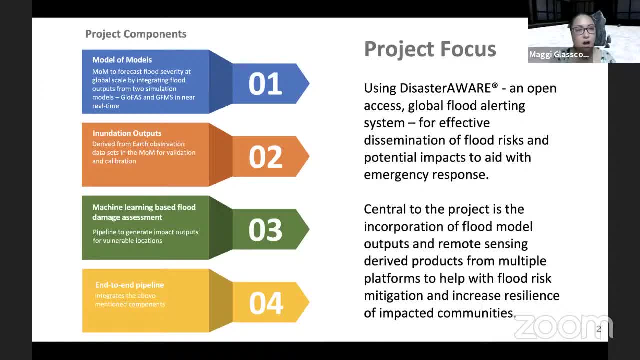 models And I'll go into that specifically in this talk. But there are other three components to the project, which include inundation outputs from Earth observations that will validate the model of models, a machine learning based flood damage assessment that will generate impact outputs for vulnerable locations and an end-to-end pipeline. 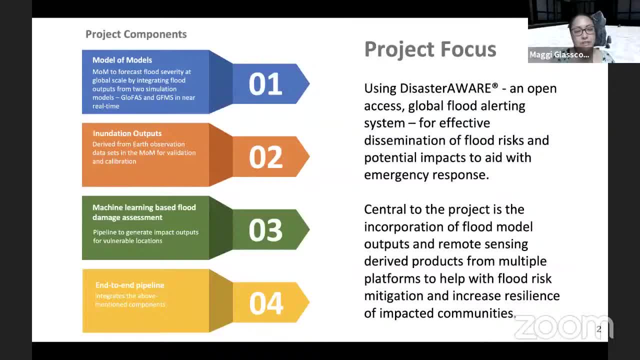 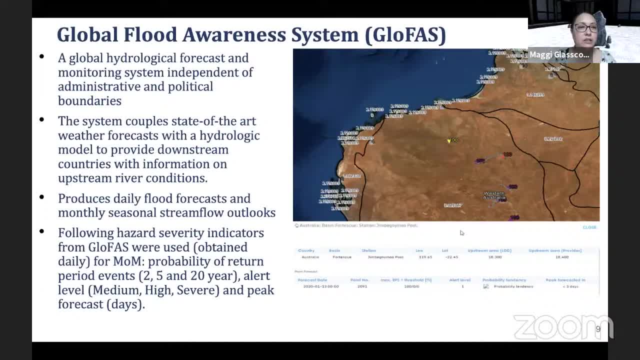 hydrologic forecasting and monitoring system, independent of administrative and political boundaries. It couples state-of-the-art weather forecasts with the hydrologic model to provide downstream countries with information on upstream river conditions, produces daily flood forecasts and monthly seasonal extreme flow outlooks and severity. 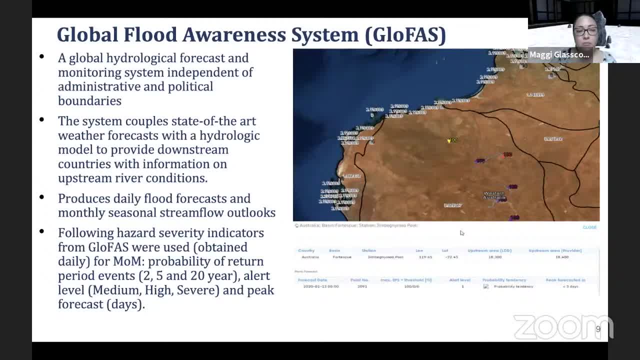 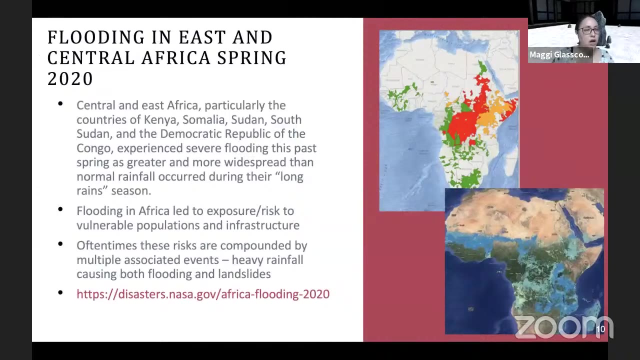 indicators are used daily for the model of models: probability of return period 2,, 5, and 20 years, alert, peak level and peak forecast in days. So how is this used in our system? So we had a case study in spring of this year for the flooding. 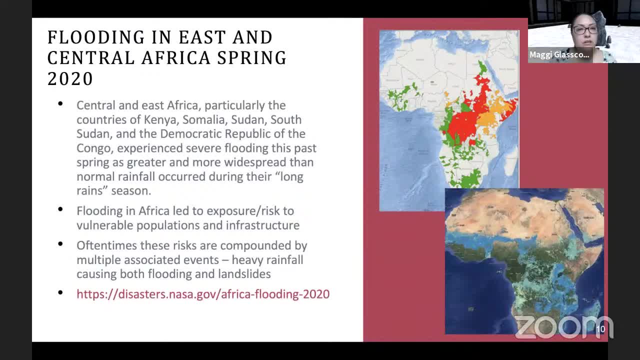 in Central and East Africa. The countries, particularly Kenya, Somalia, Sudan, South Sudan and the Democratic Republic of Congo, experienced severe flooding this past spring, as they had greater than normal rainfall occurring in their long rain season. So flooding in Africa led to. 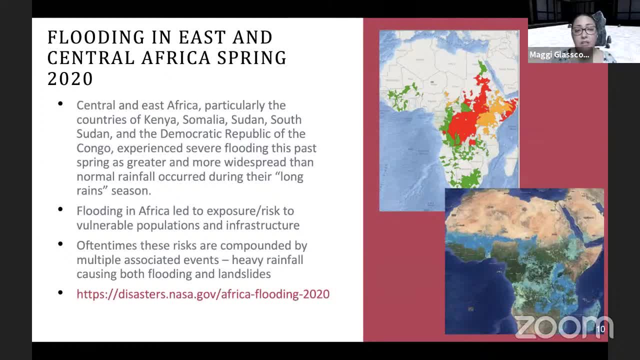 exposure and risk to vulnerable populations and infrastructure, and oftentimes these risks are compounded by multiple associated events: Heavy rainfall, causing both flooding and landslides. The disasters program at NASA in fact activated for research purposes for this event, and you can see what we did for this particular 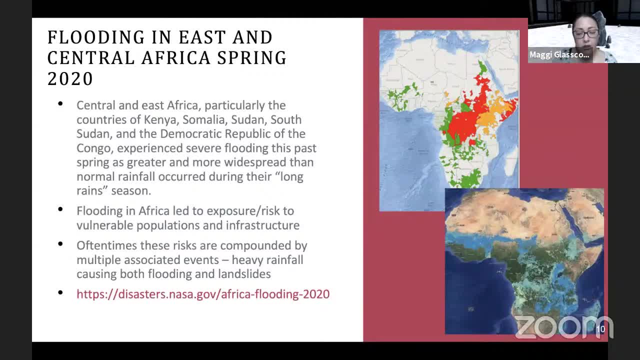 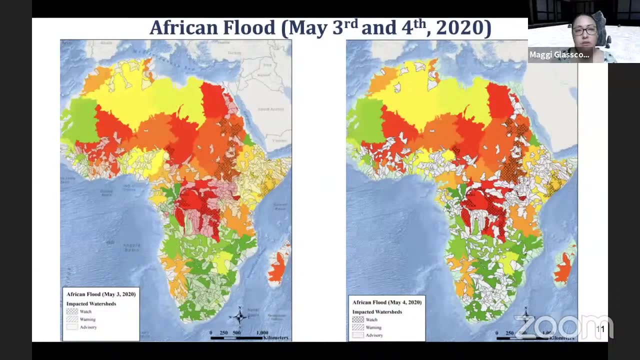 event at the following URL. Now, what we did for the riverine basins was to capture the watershed risk in terms of of watches, warnings and advisories. Now, the riverine basins that have no hatches or dots are not affected at all, but as you can see- you can see in some basins- 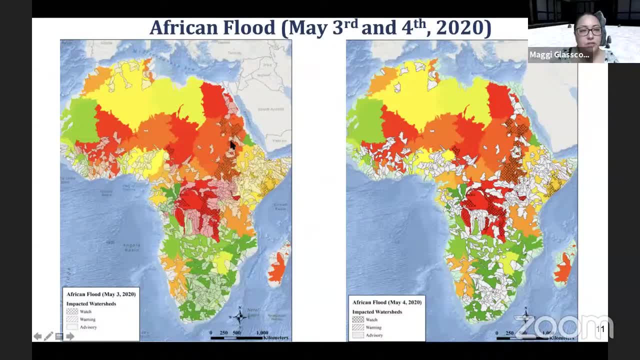 you have hatches, which are watches, dots, which are advisories, and slants, which are warnings. Now, the most severe of these are the watches and the least of these are advisories. Now we have a comparison here of the model, of models output and the 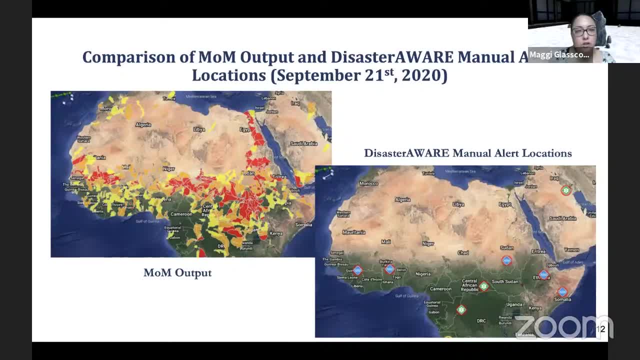 disaster. where manual alerts for September 21st 2020.. As you can see, we have a number of alerts here that were indicated by the model of models outputs compared to disaster aware alerts, and we have a fairly good alerting in comparison. but you'll see. 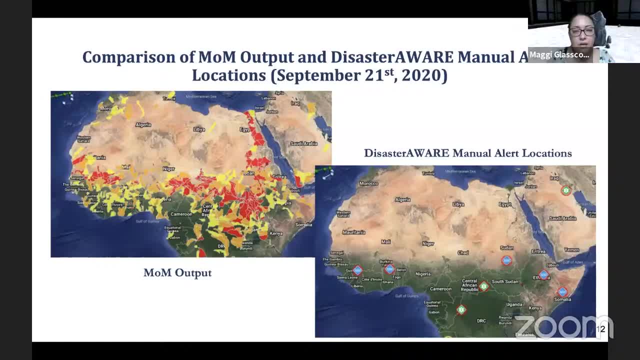 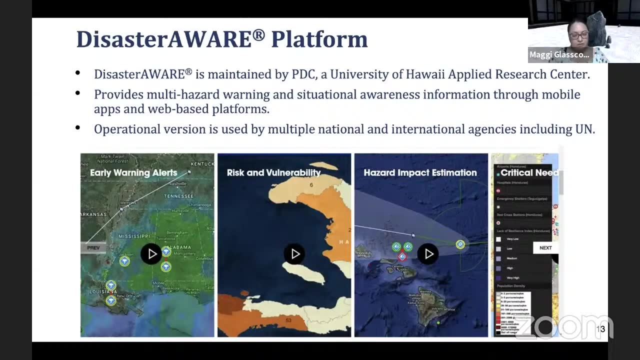 that in some cases there we have a better alerting than disaster aware. Just a little note on disaster aware, On the disaster aware platform. disaster aware is maintained by the PDC, which is a University of Hawaii applied research center. It provides multi-hazard warning and situational awareness. 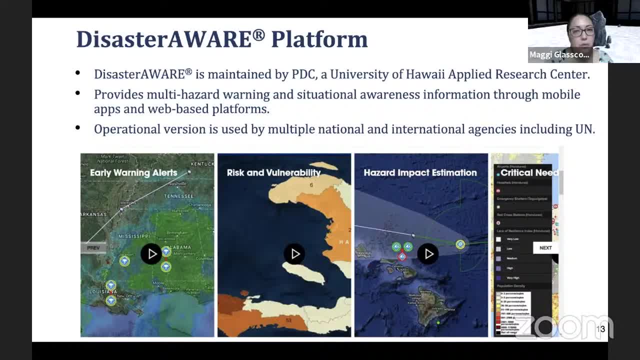 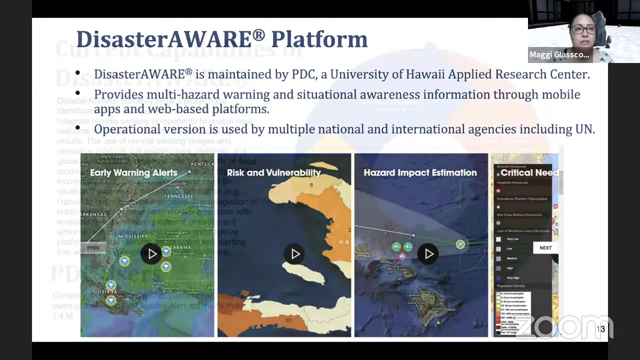 information through mobile apps and web-based platforms, and the operational version is used by multiple national and international agencies, including the UN. It provides early warning, alerts, risk and vulnerability, hazard impact estimation and lists the critical needs. Now, the current capabilities of disaster aware lacks a global flood identification and. 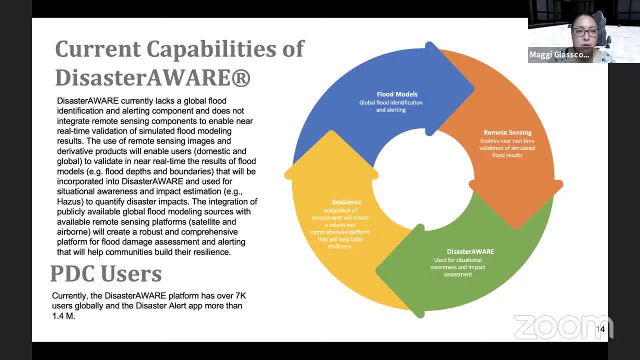 alerting component and doesn't integrate remote sensing components to enable near real-time validation of simulated flood modeling results. This is the reason why the PDC approached us to work with the US Department of Health and Human Services and the US Department of Health and 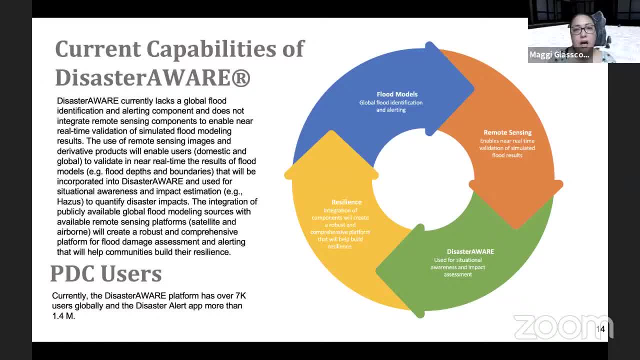 Im dotted уб der, the library, to help us with this and collaborate with them on this particular project. They've used remote sensing imagery on this particular project. The use of remote sensing imagery to validate the near time results of flood models incorporated into disasterware will help them with situational awareness and impact estimation to quantify their disaster impacts and the integration of these publicly available global flood modeling's salary is and remote sensing platforms will enableael wydaje mode line up to the flood. finally, images, which will help them with situational awareness and impact estimation to quantify their disaster impacts and integration of these publicly available global flood modeling's salary, isar s sources and remote sensing platforms will enable them to process and região what's appropriate connais, cold raintag impacts and expert data. 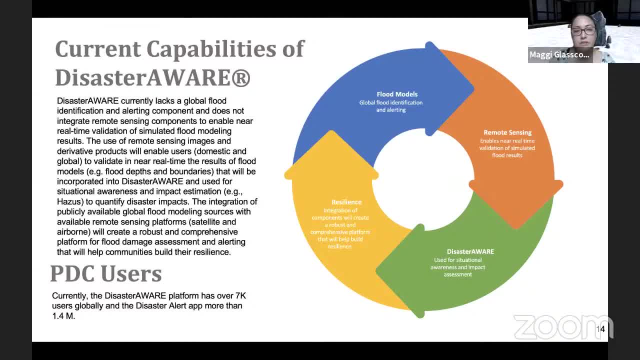 will help them to create a robust and comprehensive platform for flood damage assessment alerting that will help them with community resilience. So we see here that we have this sort of feedback loop here where we have the flood models to help with global flood identification and alerting. remote sensing that enables the near real-time validation. 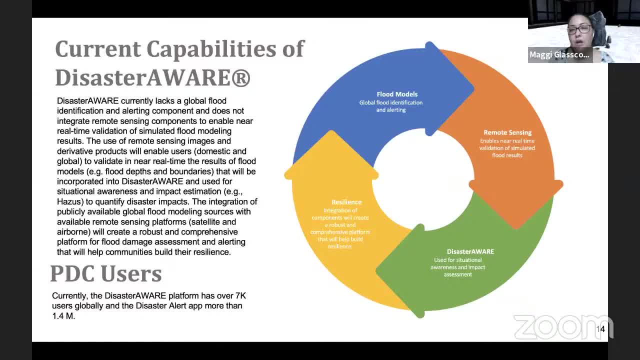 of simulated flood results. which feeds into disaster aware. which is used for situational awareness and impact assessment. which leads to greater resilience. which includes integration of these components which will create the robust and comprehensive platform which will help with resilience. Right now, PDC has a platform for disaster aware that 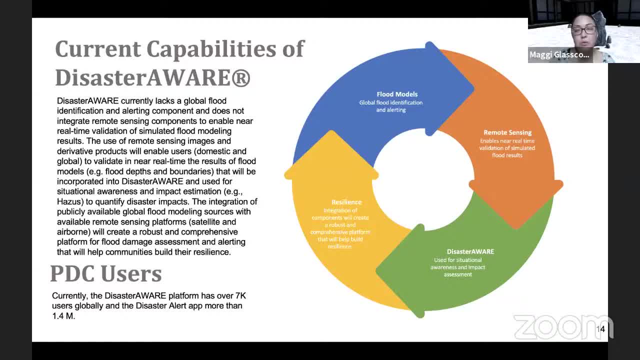 allows them to do a lot of work on disaster awareness. So we see here that we have this platform that includes 7,000 users globally, and they're free to use disaster alert app that has over 1.4 million users globally. And with that, I think that is the end of my presentation. So I 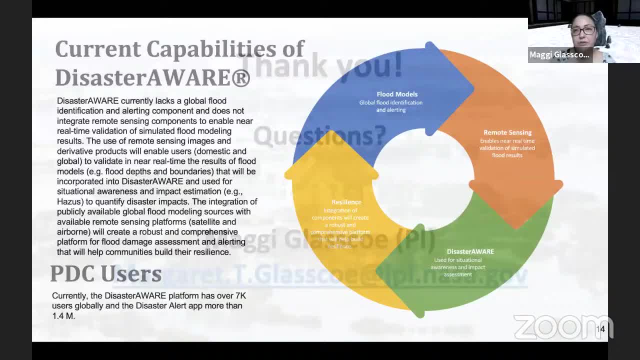 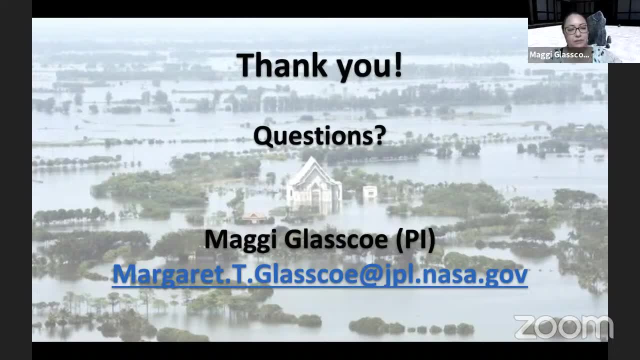 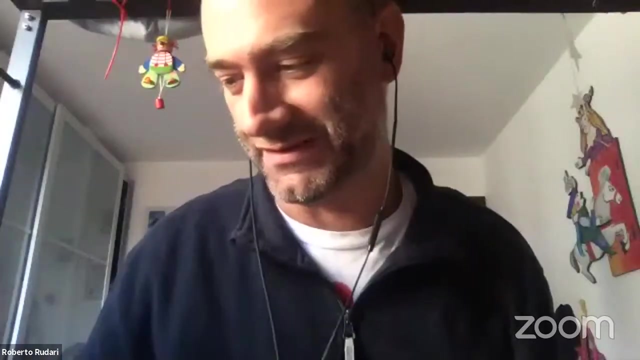 can take questions in the chat and we'll be happy to participate in the discussion at the end of the rest of the discussion. So thank you very much. Thank you, Margaret. Thank you for the presentation. Thank you a lot for keeping the time almost. 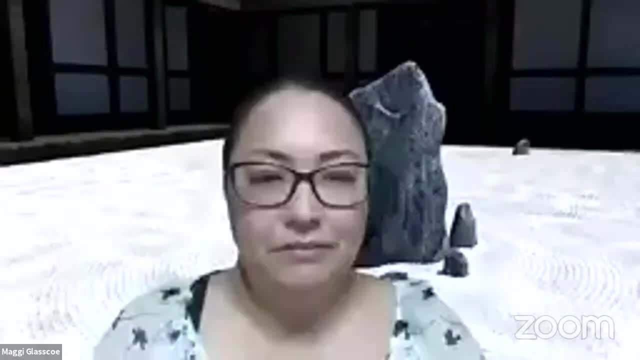 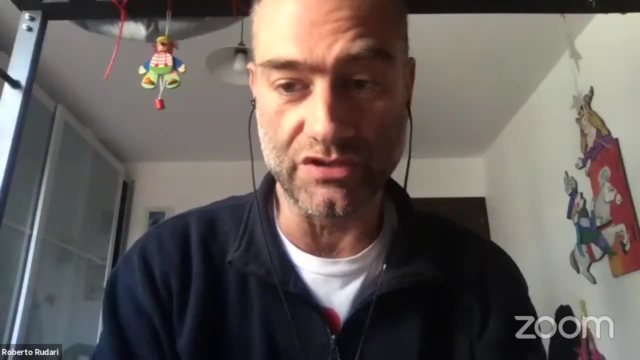 perfectly. Thanks a lot for that, Very much appreciated. I knew I mean let's say the invitation, I mean to all the to the audience, basically to pose questions already in the chat so that Margaret can already like repair and read the questions. So thank you very much. 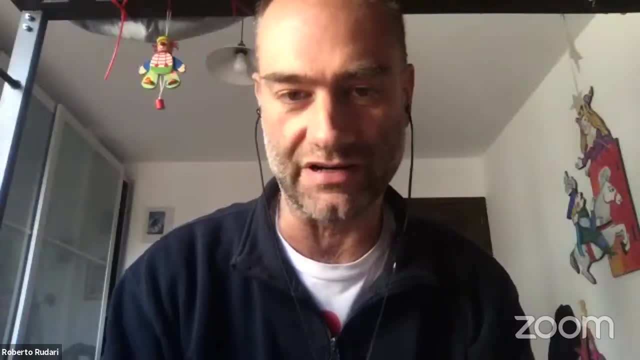 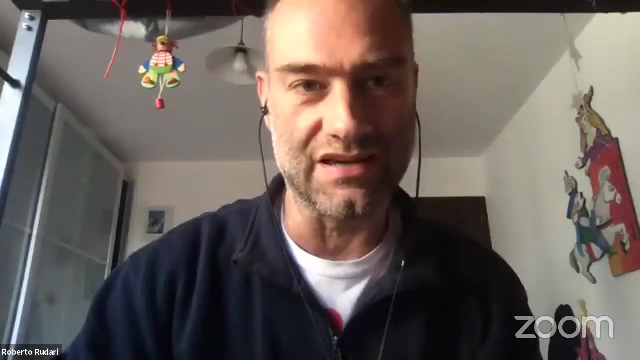 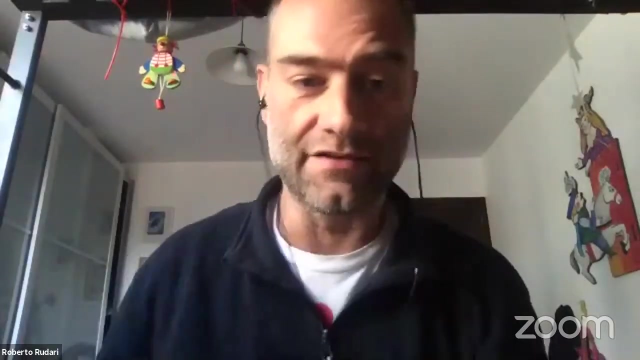 May be, I mean responded into some of them, I mean directly into the chat, but we will certainly have, I mean time for discussion later on. I would like now I mean to introduce the second speaker of today, That is, Erwin Sauter from the ECMWF. that's will actually go on and explain them and what are 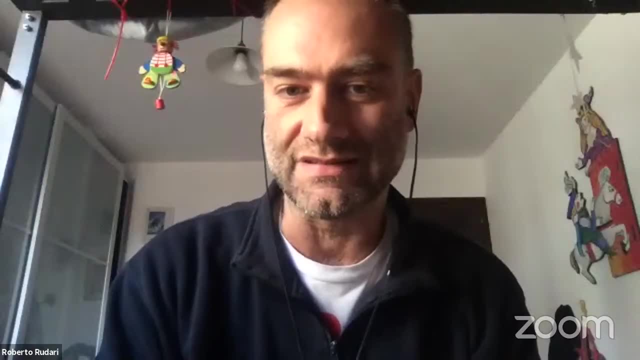 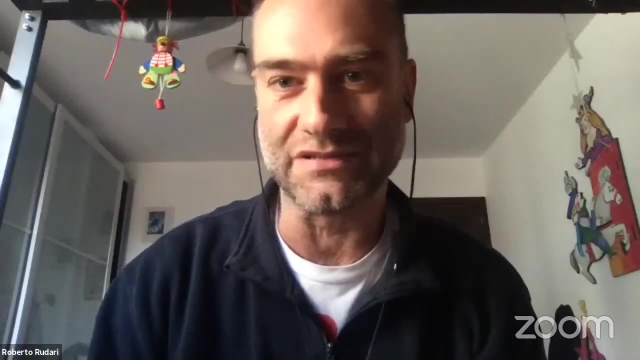 you know, the new development of the globalεν, the GlobalShadowAwarenessSystem. the Global, located in Data Science and Energy, is one of the the components of the model model that we just and then seen in margaret's presentation. so, irvin, please, the floor is yours, and then try to share your screen a minute. 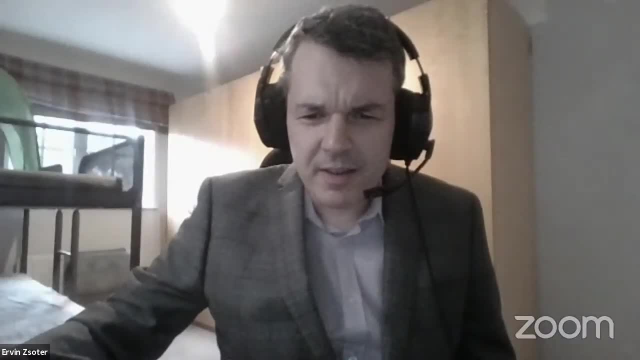 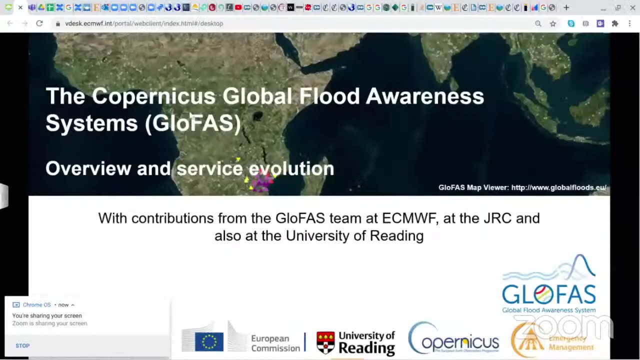 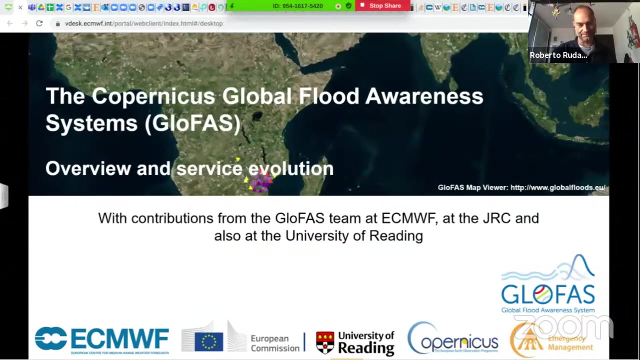 jackie, if that works, thank you, thank you, uh, and hello everybody. i'm sharing now my screen. i hope will work, so let me know if it's on the screen, is it? yeah, perfect, thank you. thank you so much for the opportunity. i'm very happy to talk about the global federal awareness system. alas, glowfast. 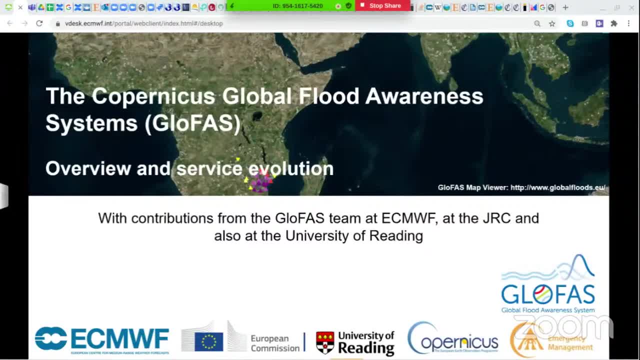 as we call it in this talk. in particular, i will focus on the service part, the service evolution of the system, basically in the last few years, as it has been developed. glowfast is, uh, oh yeah, how to move the slides forward. okay, so this is a ah. 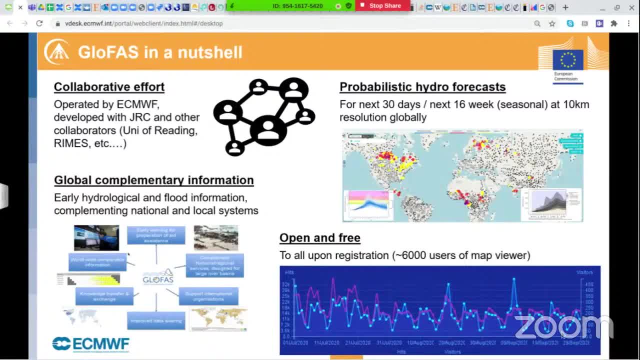 worked so glowfast is a collaborative effort. uh, collaboration at its best, i would i would say ecmwf. we operate the system together with the joint research center of the european commission, jrc. we developed the system, but there are also other institutions, collaborators like the university of frederick rhymes and others. 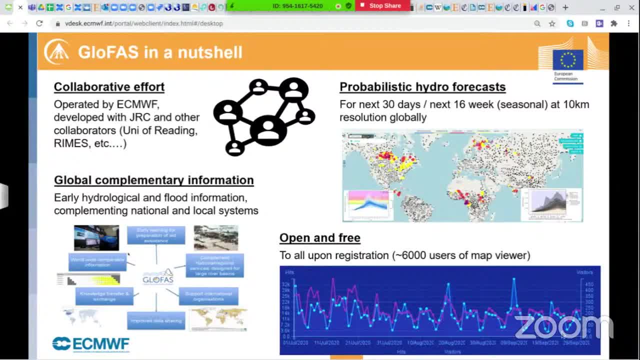 who actually help mainly in the evaluation and the analysis of the data. glowfast tries to be a global complementary information, so we we are there, if basically on top, either on top of the local, national, regional hydrological prediction systems or basically as an only available uh system in in some areas, and this is especially useful if disasters strike in in areas. 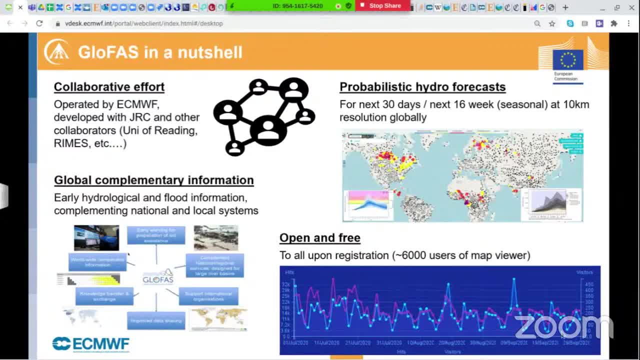 and unfortunately they don't really uh, look out for areas where where all the capabilities are there and humanitarian agencies, red cross and others are then going to be able to use our predictions and especially use it in in kind of like medium range mode, when when early warnings kind of will be there. 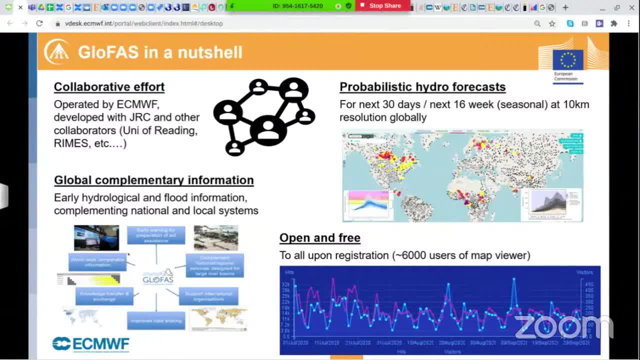 to use. it's a probabilistic system providing a hydrological forecast- as maggie nicely introduced it before me- for the next 30 days and also, in the seasonal component, for the next four months or 16 weeks. at the moment. it's run at the moment on 10 kilometer resolution globally. 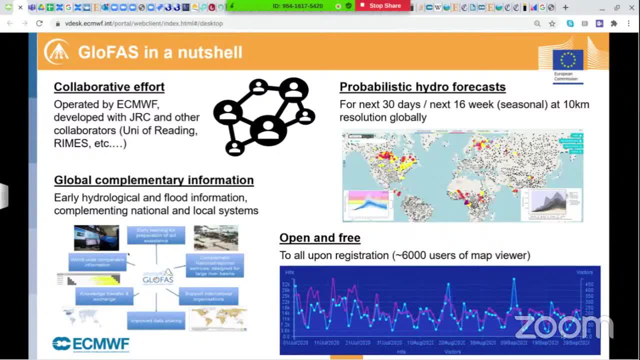 Glowfast has this wonderful advantage of being part of the Copernicus infrastructure, so we are part of the Copernicus emergency management service. all our data is open and free for actually any user it is. it's really encouraged that users actually take this up and use it. so 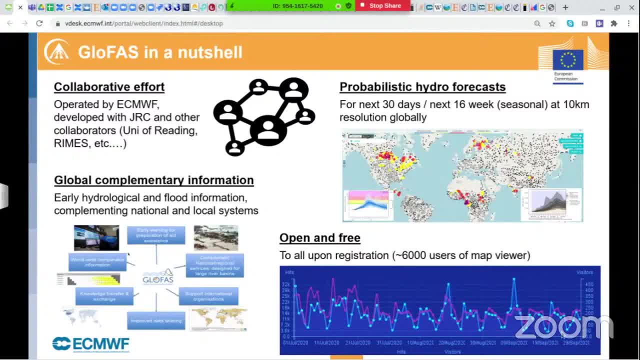 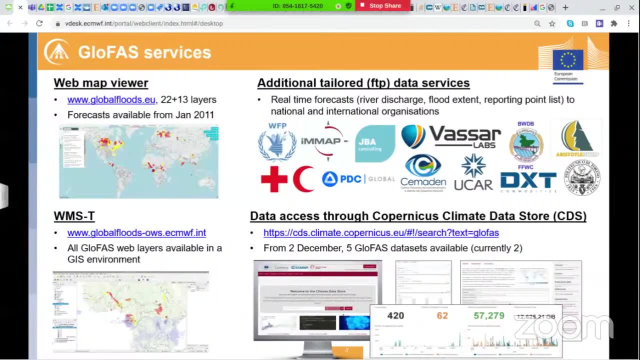 we are around 6 000 with registered users. data, web data, kind of products are available after registration. several hundred people seem to be using it daily, so hopefully it's kind of like acknowledged as well. how can the users access our kind of products through which services? 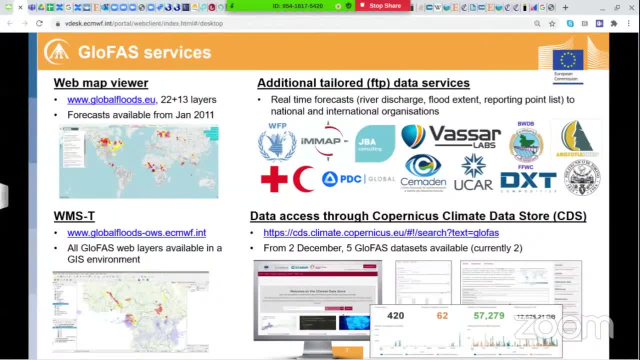 first of all, there is the web, as I mentioned. so the web map user viewer: currently 22, but from December, when we have the new model version implemented, there will be 35 layers in total. available forecasts are available. users can go back out to 2011. so basically all the real-time forecast. 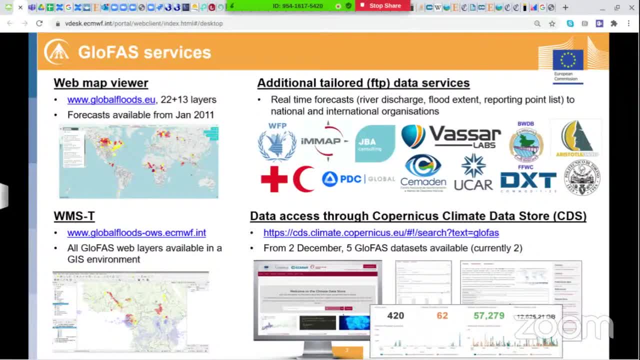 whichever number of layers back then were available. so it's a good way to actually see also the evolution related to this. the web map service is there to basically service all these web charts and the users can ingest it in any kind of GIS applications also. we run an additional, have been running an additional. 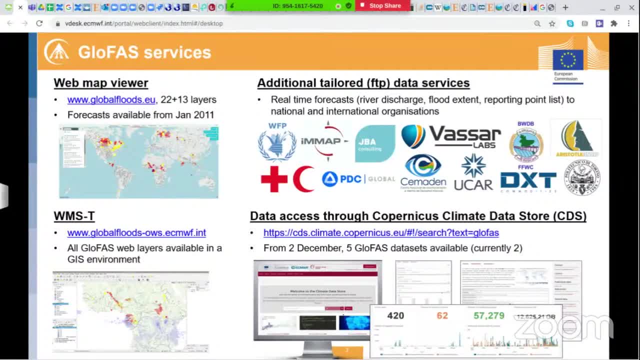 tailored data services through a dedicated ftp stream. so there are quite a few participating and collaborating institutions: national, international organizations- I just heard that- the PDC itself, or the workflow program, as it was mentioned last week, or the red cross in many locations around the world, in the, especially in the 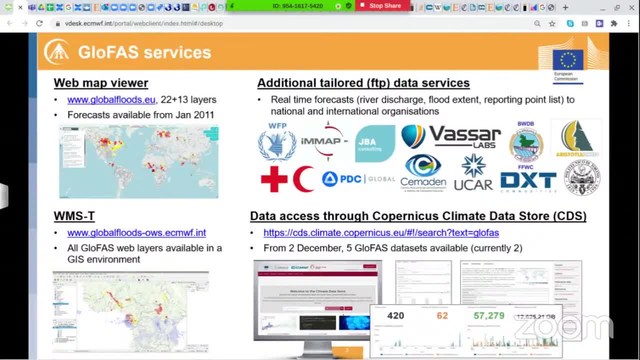 United States, and the United States and Europe has been working on it, so I think it's in the top three there in the top three. so it's a good opportunity for us to go back and see the global data on the ground as well, but it's also an opportunity for us to have a little bit of a 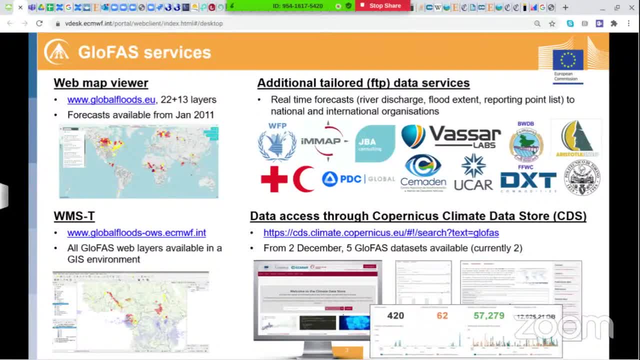 bit of an overview of the data and also the, the, the focus based financing projects. they are using heavily glowfast and the most recent area where we can actually provide the data is through the them. now GlowFast is also available together with EFAS, which is the European part of this. 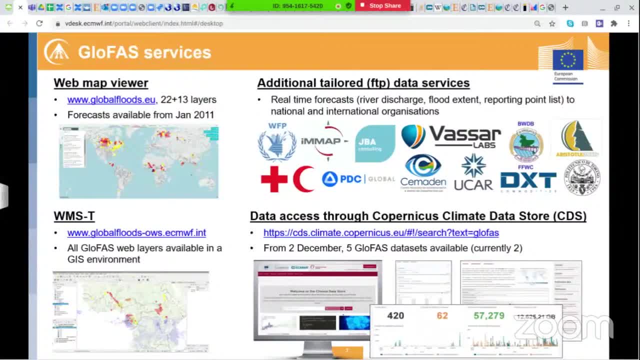 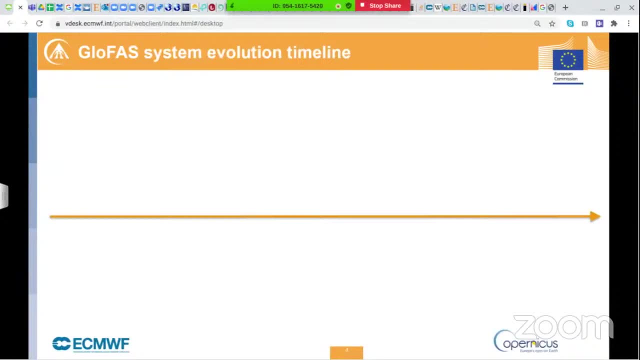 CHEMS flood project and from December 5 data sets will be available, accessible- downloadable again- only after registering. a little bit on the on the evolution. so basically, what was the timeline? so how did we end up having this global flood awareness system? it started out at least 10 years. 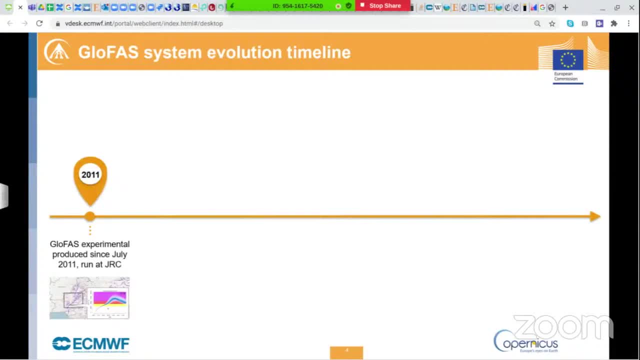 ago, 2011 was when, still running, the system was running at the JRC kind of like in an experimental fashion, but every day forecasts were produced, a data set- sorry- a website was designed, and ever since the data and the web products have been available. and then in 2015, when ESMWF was already. 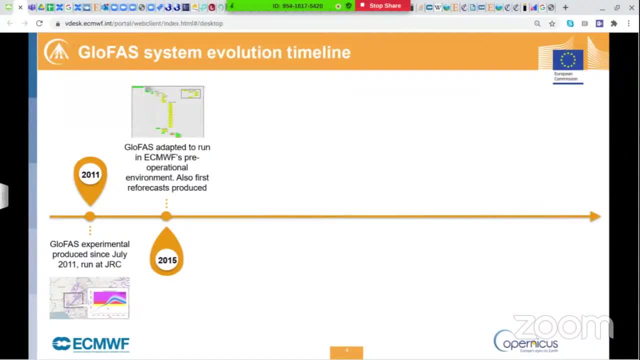 the computational center for EFAS system was ported onto ESMWF platforms and since then it has been basically running there at ESMWF, back then still not operationally supported. another big step forward in November 2017, when we introduced the seasonal component, the first of its kind providing global hydrological 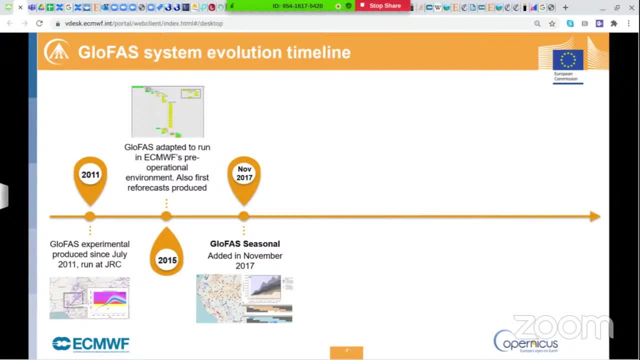 information out the four months lead time for high flow- low flow probabilities using some kind of like ways of portraying the data. the big kind of change happened in April 2018, when Glowfast was finally was implemented operationally. before this time, officially no money was spent on the system or the development, so since then it's fully supported. 24: 7 supported. 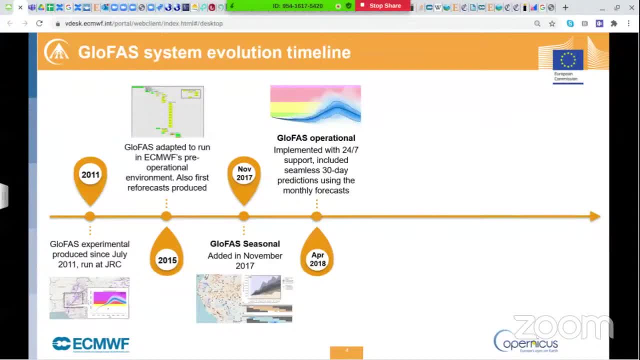 and as part of this upgrade, we also introduced the seamless forcing system relying, after the first 15 days, on ESMWF extended range forecast which ever since basically has been in the system. a modeling upgrade- mainly a modeling upgrade- happened in November 2018, since when we actually number the system to have the users obviously refer to the actual 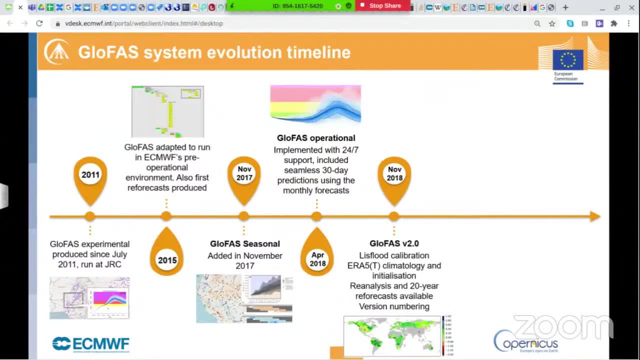 forecast version they are using or referring to. this was version 2.0. the routing component- component which is done with the list flood hydrological model was calibrated at over 1000 stations. the discharge time series On top of it, ERA5 and ERA5T, which is the 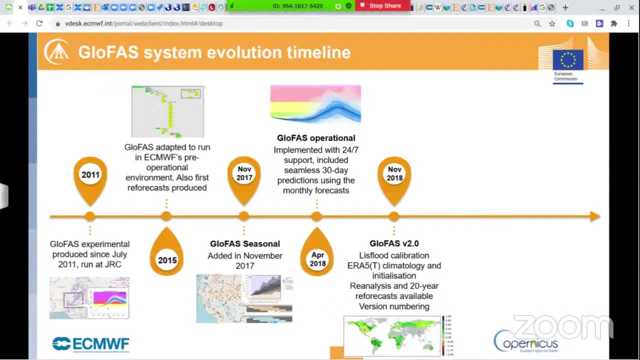 timely, almost real time, very near real time. available part was introduced into climatology and also in initialization. We also introduced the refocus, the concept of the 20 year refocus, and I will talk about that some more a little later. The last before now upgrade happened. 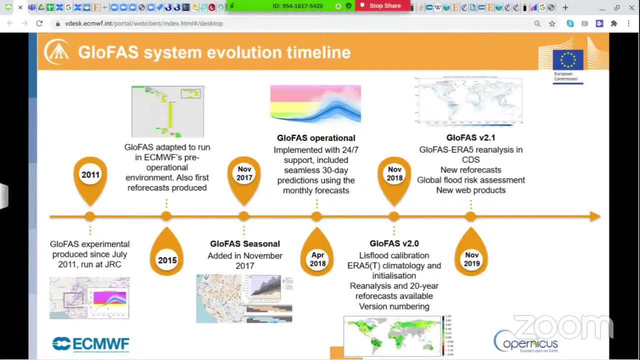 November last year, 2019, version 2.1. When the reanalysis was the first dataset we actually entered into the CDS. So since then it's over a year now. the dataset has been available. obviously, many times it has been downloaded, lots of data volume, etc. With each model. 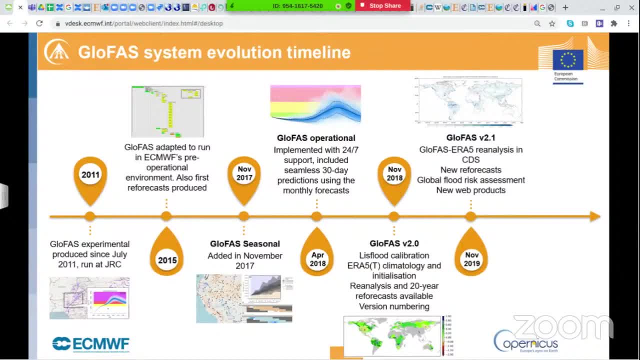 upgrade which actually impacts river discharge. we recompute all our products: the reanalysis, the refocus, the seasonal datasets, everything. So from this upgrade, basically this protocol has been introduced. On top of it, we have also added few products. one of them is the global. 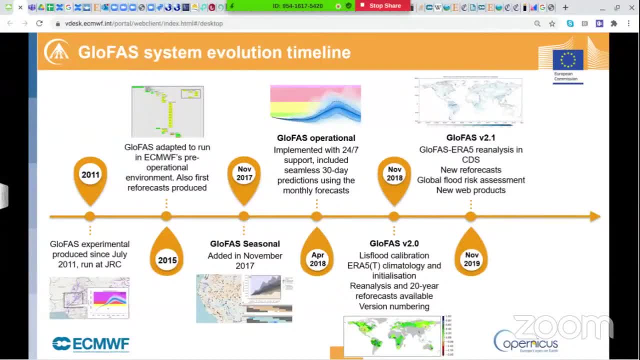 flood risk assessment again will be introduced a little further and several new products. The next upgrade is happening very soon, so almost imminent beginning of december. it's planned for the 2nd of december, so please look out. there will be kind of many, uh, new additions which you, you will. 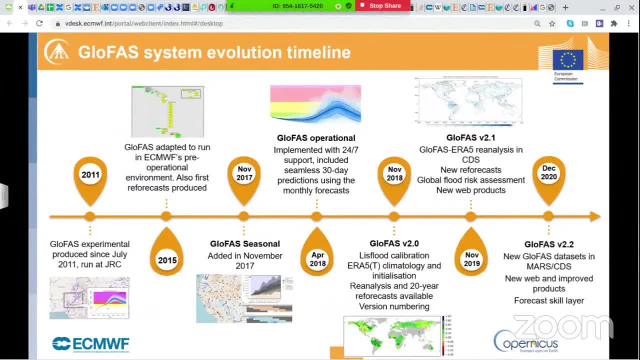 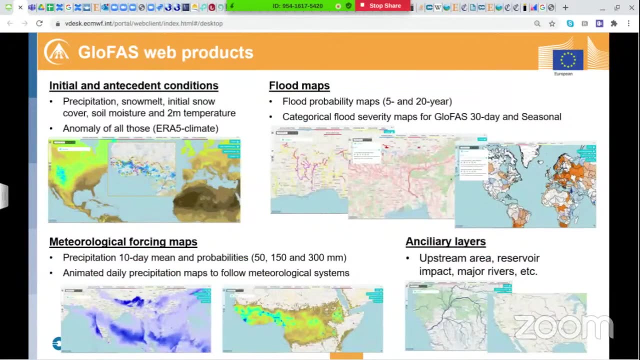 be hopefully be happy to use on the web. it will call, obviously called version 2.2, further data sets in cds and, as i said, different products, forecast, skill layer and so on. just a little summary on kind of like a flavor on what products we actually offer at the moment to the users. 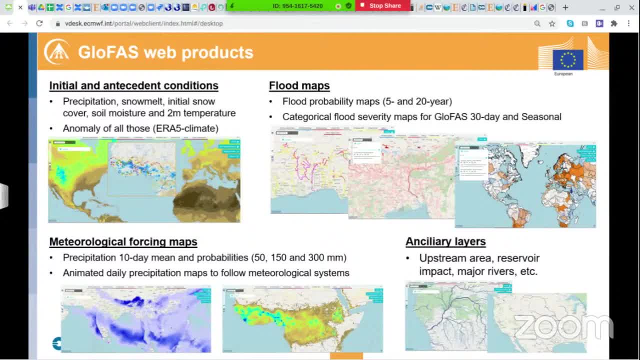 on the web. a new group is the initial and decedent conditions, which will be added in december. it relates to how we start basically the forecast, how the users basically interpret what is this kind of like starting initial situation, precipitation, storm, world, other variables and also anomalies of these using the other five, which is also 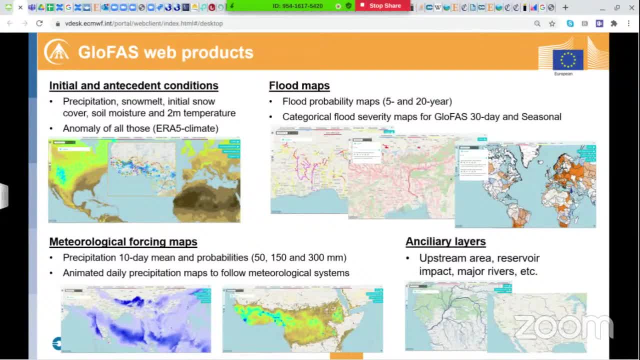 so part of our uh forcing, the reanalysis and and the initialization, to provide anomalies from the methodical forcing. currently we provide precipitation. so for forecast maps for the next 10 days, the mean probabilities for over a few thresholds and there's a new edition from december. 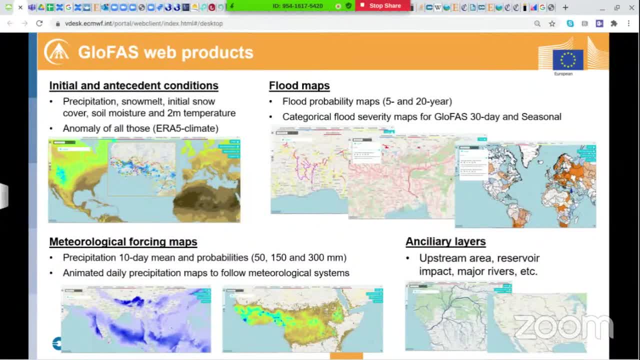 the daily animated precipitation will also be available. this, hopefully, will have the users basically kind of like track weather systems and and give a better idea on how that actually evolves. we have a similar data layers river network with upstream area location of kind of like implemented reservoirs, lakes, all sorts of other information. 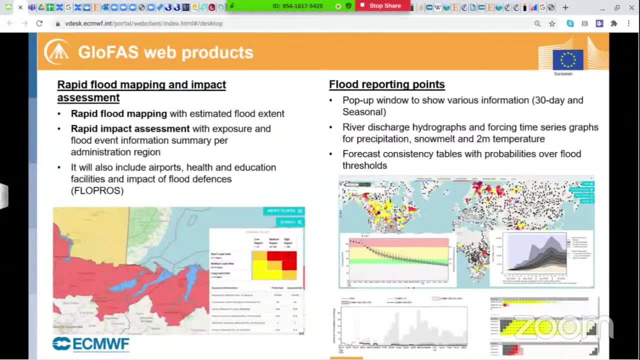 as well the flood risk uh product, which is our first step, hopefully of many, to basically going towards the impact based forecasting, which is which is kind of like the longer term target. so in this product we use the discharge information as much like the highest discharge in the 30-day. 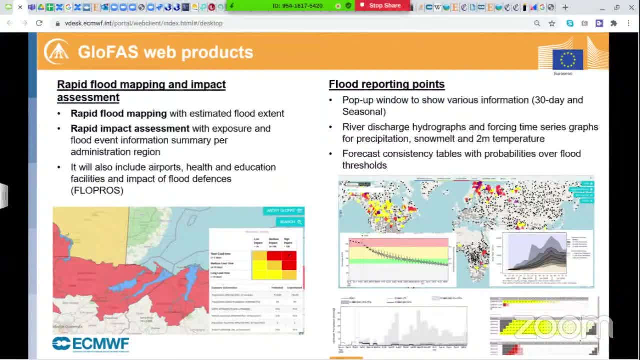 forecast horizon and, based on the catalog of flood inundation maps, produce kind of like an estimate on where flood inundation is expected. and then it's kind of like cross related with vulnerability and exposure data sets, and then it's kind of like a pop-up window with a matrix, as you can see in this example, with all. 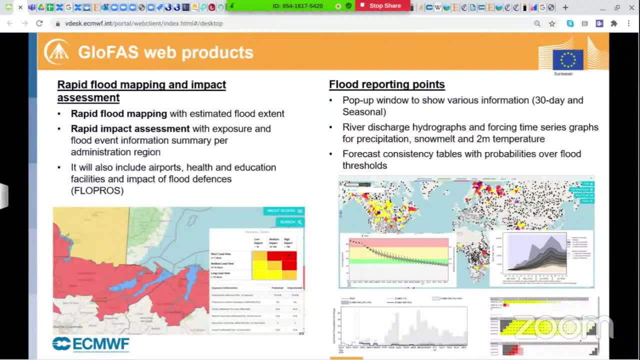 sorts of qualitative information on kind of like the estimate on the impacted number of people, infrastructure and also, from december, this will be extended by the airports, health and education facilities and also including information on the flood defenses from flow pros. therefore, if the defense is there, then maybe you won't see the colored area. 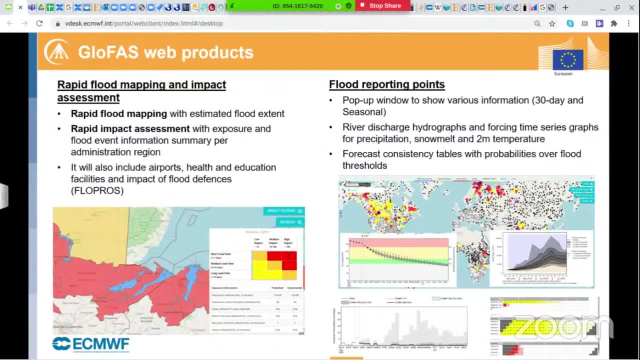 and so we also have a quite detailed map and a beginning map, and it's very simple and, uh, that's what we do and that's how you can come to the background of the기도 and the data. so i'm going to do an introduction and then i'm going to hand it over to you one more time. 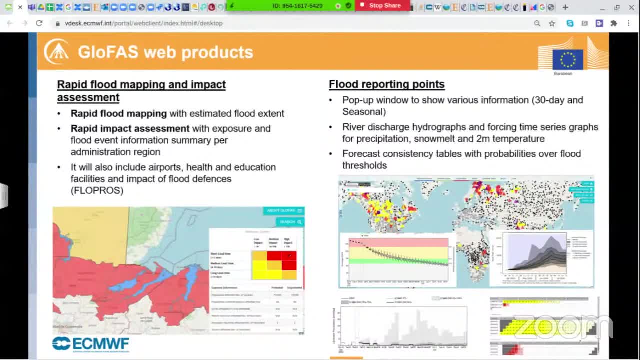 but i'm going to do an introduction and then i'm going to explain how i got started. so, basically, here are some links that you can find in the video. so the first- we have some of those- is the general map and the second is the map that the people drink. 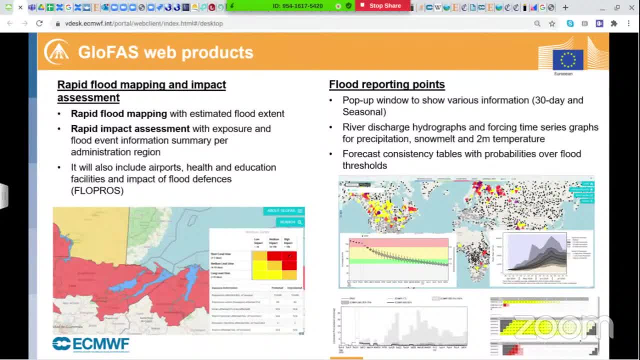 their morning breaks down. and then the third one from this is the map, which is the industrial precipitation. snowmelt and temperature will be included, And on top of it evolution of the forecast probability. the exceedance probabilities are also there in tables. 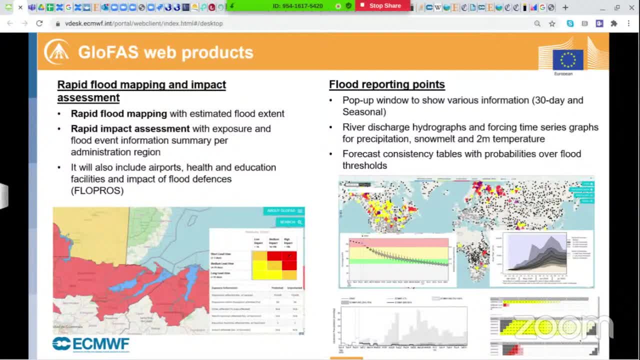 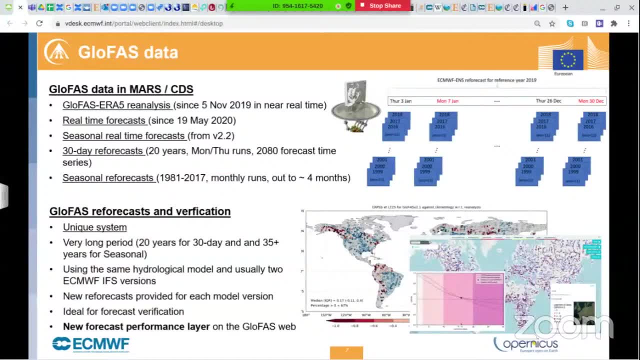 So, basically, more and more information is available. How about this data sets? I mean this we really believe is a very strong point of ChlorFast as a unique system. All our data that we produce is going to be available in Mars, which is the methodological archival retrieval. 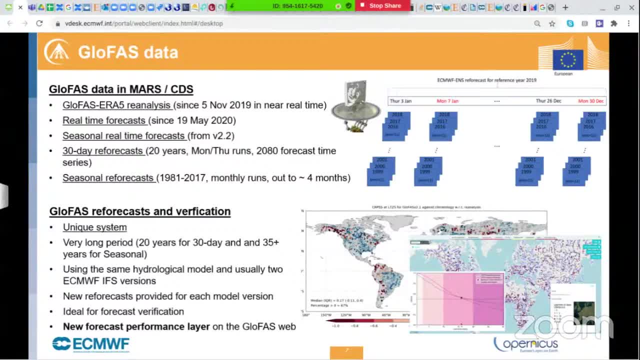 system of ECMWF. It's a data archive, basically. that is behind the CDS climate data store. It has hundreds of petabytes of data, which now also includes hydrological data, which we are very proud of. The reanalysis was the first, a year ago, entering the system. 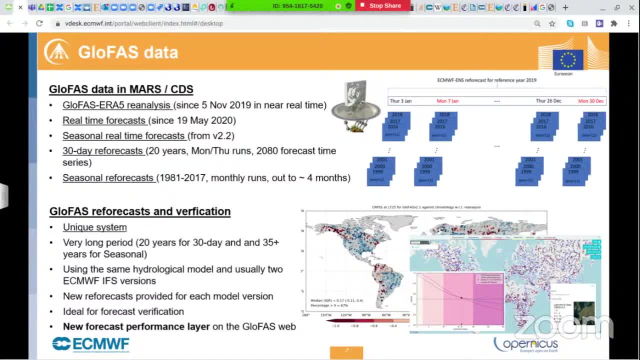 Then this year in May we added the real time, ChlorFast forecast, the 30 day forecast And in December the remaining three. so the seasonal real time forecast, the 30 day refocus and the seasonal refocus will be added. 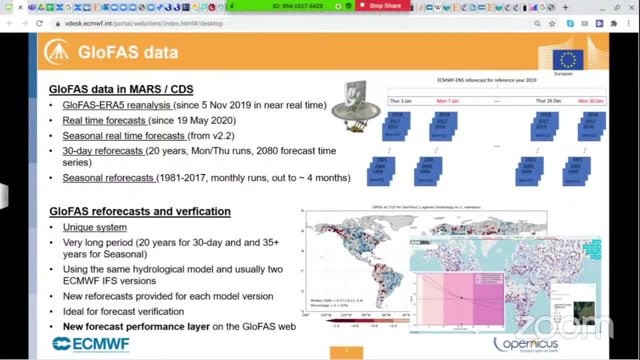 This is kind of a large data set if you look at it this way, especially the refocus, the seasonal refocus, start in 1981.. Every month, basically, we have a forecast, So it's a long stretch of forecast kind of like similarly produced. 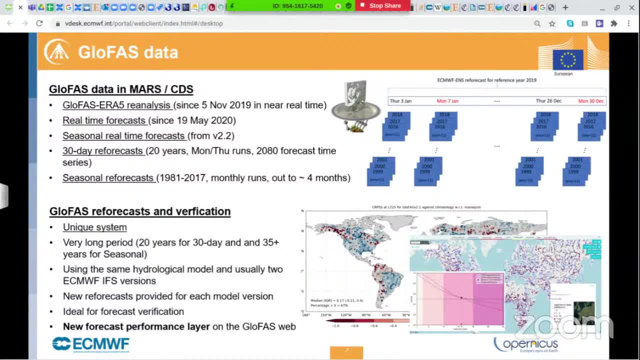 For the medium range, or the 30 day as we call it version. we rely upon ECMWF's third 20 year refocus, as we call it, which basically is a system in real time. They produce forecast for the past 20 years. 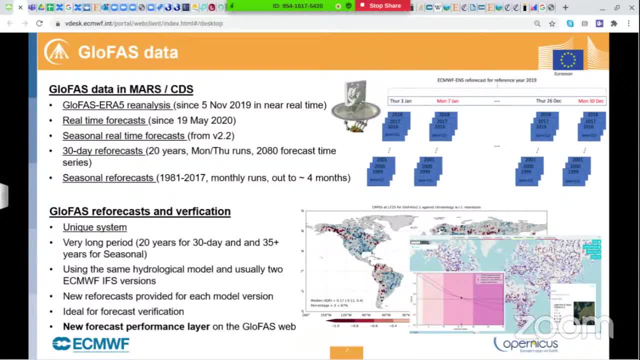 always for Mondays and Thursdays, with a limited number of ensemble members. for computational reasons It's not possible to produce with the full 51 ensemble members, as it is in real time, Over 2000 forecasts in the system over 20 year period. 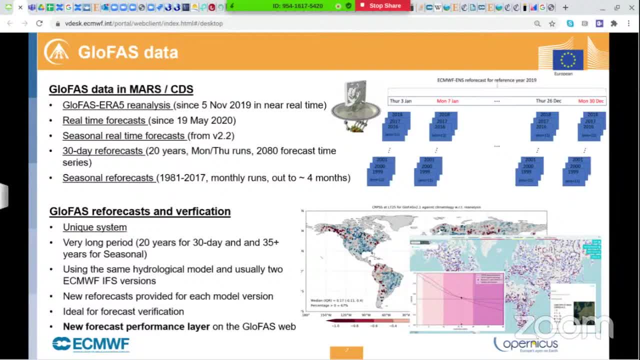 So it's a long period, many forecasts. It's an excellent way of kind of like evaluating the forecast or the focus performance of the system, kind of like working out post-processing our algorithms and the like As a first application in the verification arena. 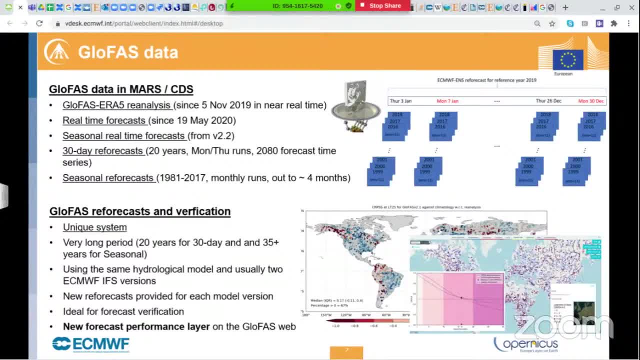 in December we're introducing a new layer, which is a focus performance layer, And that is where we'll utilize this 20 year reforcast and produce kind of like show: the lead time when the CRPS scale score drops below 0.5,. 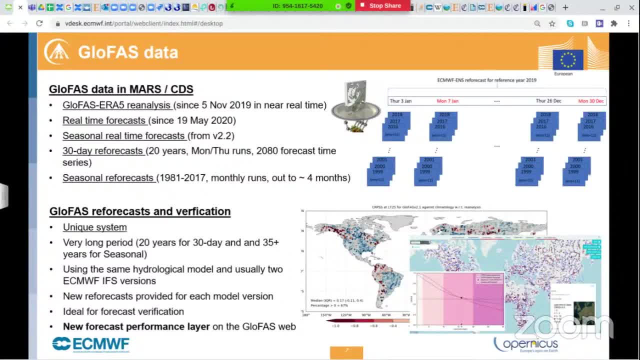 kind of like seeing against two benchmarks, the persistence and the climatology. So in this work and this product everything is verified with or against the reanalysis. So so far no observations are used. That will be further developed in the future. 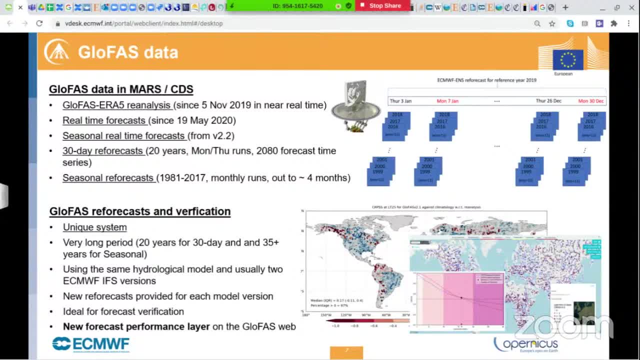 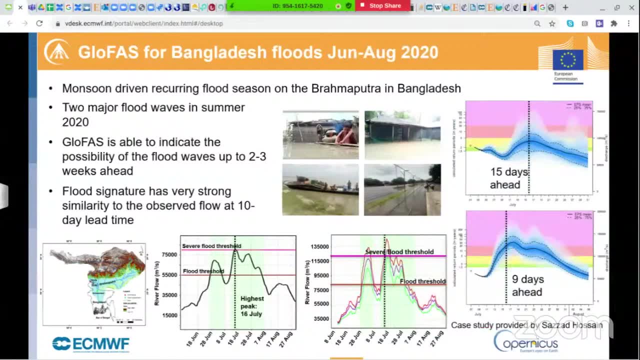 further uh verification products, uh later now an example on basically how glowfast can can work and and can showcase basically the capability of the systems. so glowfast is not yet the finished article. so there are areas where the model performance is lower. there are areas where obviously we are more. 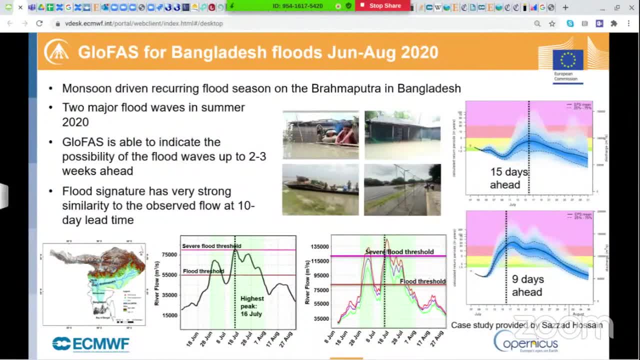 capable of picking up flood signals. this area in bangladesh on the brahmaputra river is definitely an area where where we can look very far ahead, so the predictability is really long in this case. uh, floods occur every year, kind of almost regularly. in this year they had like two big 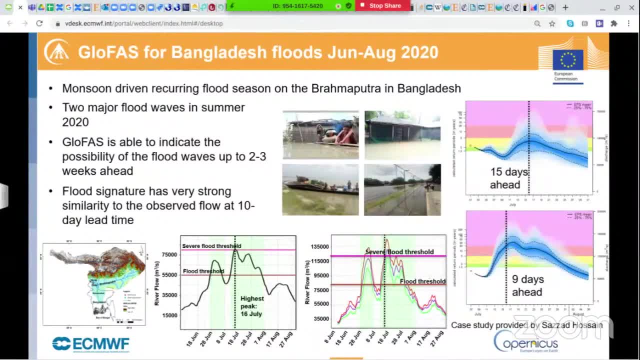 waves in june, end of june and also most of july, and from the forecast i picked the 20 year, sorry, 20 year to 20 day, 10 day forecast. and, by the way, thanks says that hussain from the bangladesh foreign. 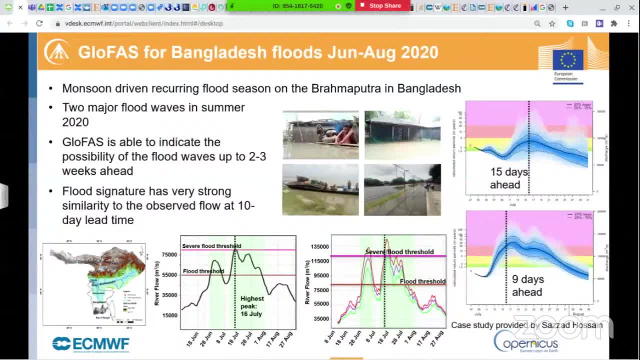 flood forecasting center and also phd students at reading university to provide this case study. so the 10-day forecast, as you can see, the pattern of the increase or decrease of the discharge, pretty much matches very, very nicely matches the observed discharge. uh, kind of like pattern. the. 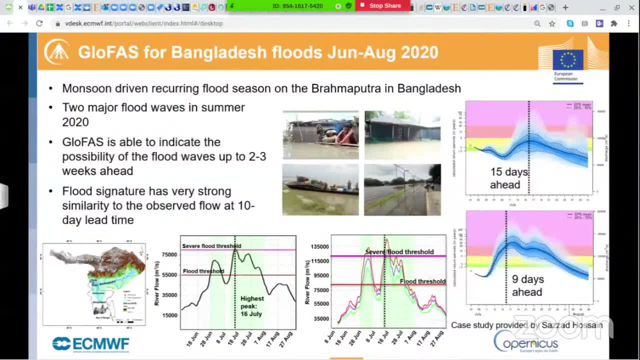 values are different. we have a positive bias, quite significant positive bias in this, in this location. but, as we intend or try to say to the users, the intended use of glowfast is basically looking at the forecast in the context of its own climatology. that kind of flood signal is is 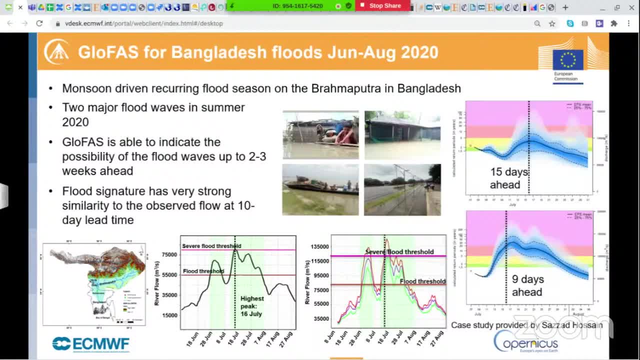 pretty realistic. in this case, we could look ahead. as you can see on the top right corner graph, 15 days ahead. there was a strong signal, albeit very strong and very high uncertainty, but still a good indication of a very early heads up on a potential- uh significant flood down the line. 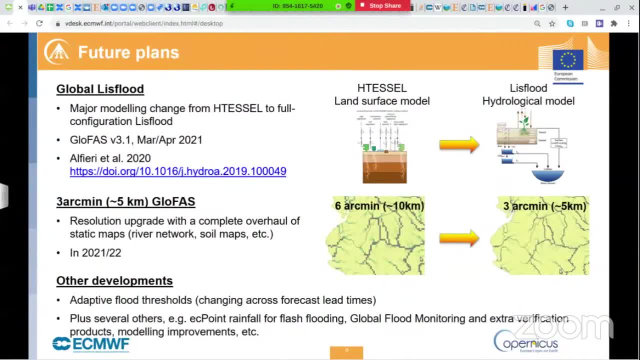 okay, but what was what going to happen with loafers? i mean, uh, glowfast has been operational for just over two and a half years and this is the period where we could really put uh resources and effort in in developing the system, and we will always look into uh developing and improving the system. 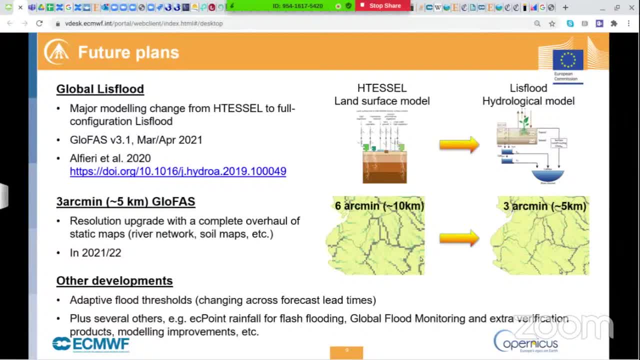 in in all sorts of different areas. two major upgrades are planned. one of them is looking into the core of the system, so basically how hydrology is modeled. so far it has been based on the hdsl land surface model of ecm wf. we are switching to the full. 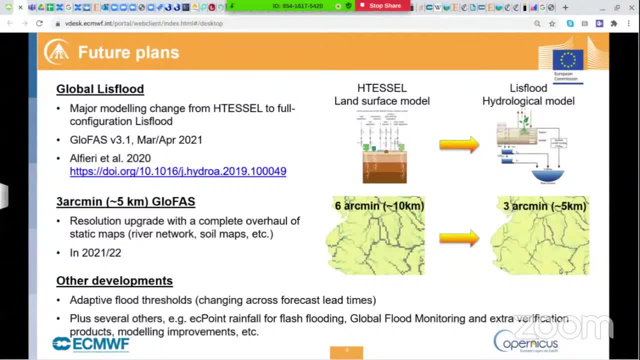 configuration using list flood in a runoff rainfall runoff model configuration, basically. so it's a major upgrade. we try to look at all sort of different aspects basically about it. another one will be a major resolution change going from 10 kilometer to five kilometer. uh, part of it. 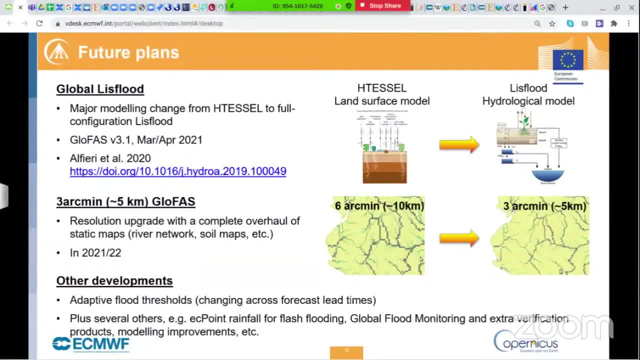 we also upgrade all the maps, the underlying maps, not just river network, but also soil maps, land use, all the likes. so it will really expect it to have a significant positive impact. other developments are planned. one of them is to look at how the thresholds are used in 30-day components. 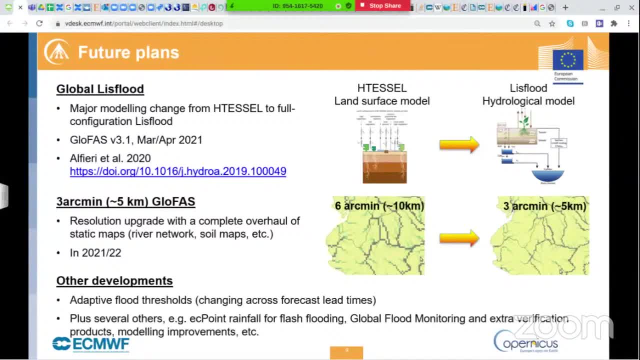 and and switching from the one rfi based threshold to a kind of like a range dependent one which represents the biases properly, and also other products like the global flood monitoring products- remember peter's talk last week. we are really looking forward to it- or having a flash. 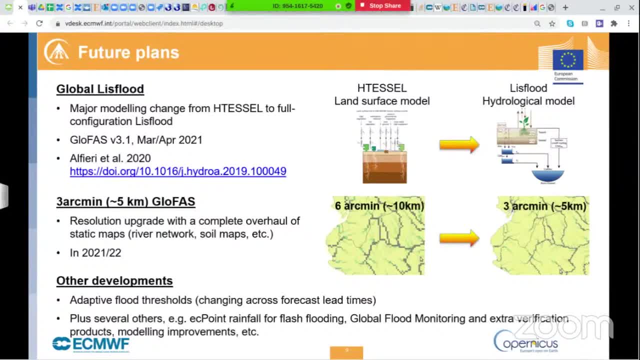 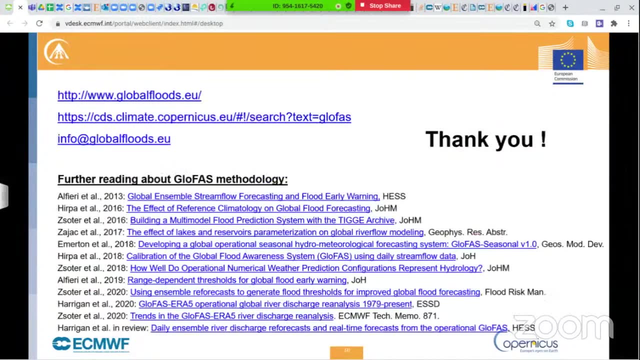 flood kind of prediction layer based on ec point, rainfall, post production, post processing, product of ecmwf or other verification maps or modeling improvements, of course. so basically the list is long and we are working hard. please go on the website, use the data, use the forecast, go on the cds. 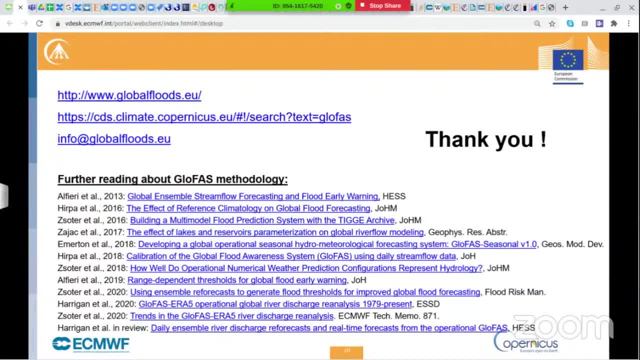 it's excellent use. the cds kind of like has also like a toolbox where you can just really go and dig into data, merge different data sets and plot them right there and then and also there's an api so the data can, problematic problem, programmatically be added into your systems. it's excellent if you are. 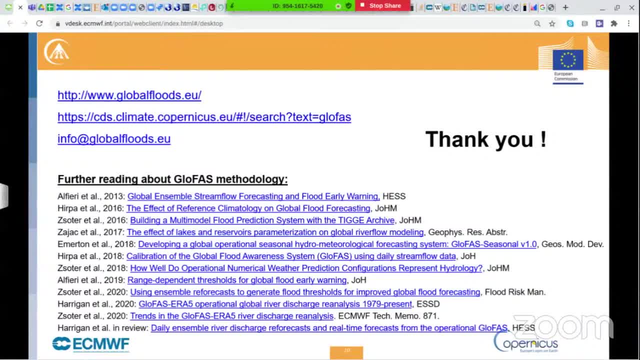 interested, go and check out these uh kind of like scientific papers. basically they will show all sorts of details about how glowfast the methodology has been evolving and and how the system was developed in the last few years. and with this, thank you, thank you so much, thanks so much i've been, i mean for the very rich presentation, and then we will take some 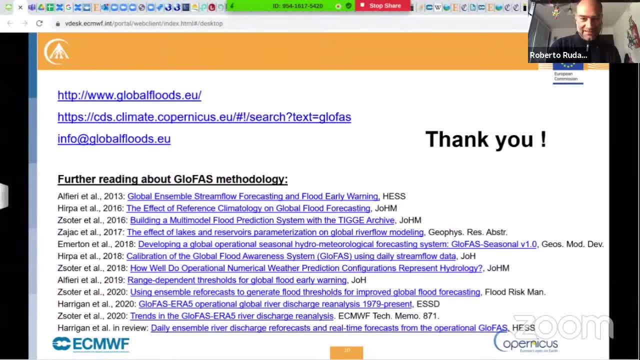 minutes. i mean also the audience, i mean today. just, i mean the great deal of information that you have presented and, um, i will pass it down. then i'm into the third speaker of today. uh, that is sella google that will talk about progresses and challenges in high accuracy flood forecasting. 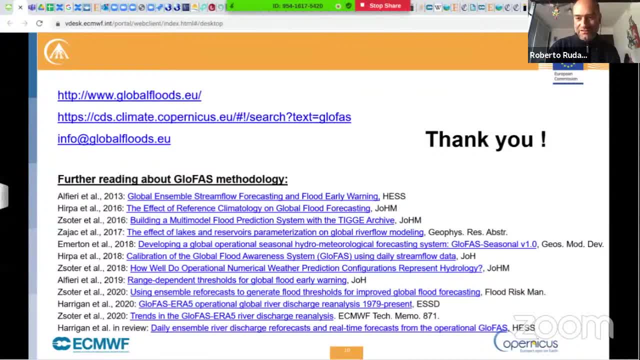 on global scales, which is quite an intriguing title. so we are really looking forward for your presentation. sella, if you would like to try to share your screen and steal the screen, i'm into irving. please proceed, sure, thank you, roberto and i let's see if this is working, can you? can you see me? 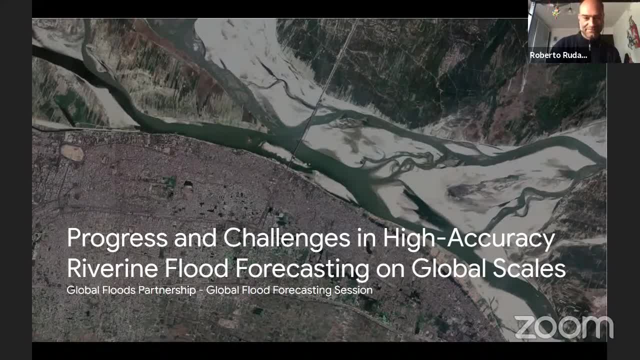 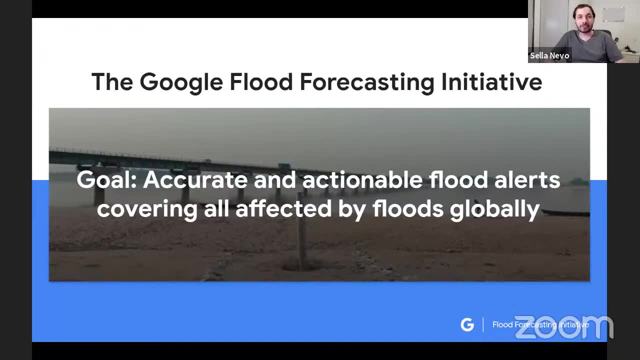 screen now, perfect, excellent, so, uh, hi everyone. uh, my name is sella and i lead the google flood forecasting initiative. the goal of this effort is to use google's data, computational resources and machine learning expertise to empower governments and other organizations to provide accurate and actionable flood alerts globally. our focus is currently on riverine floods, as opposed 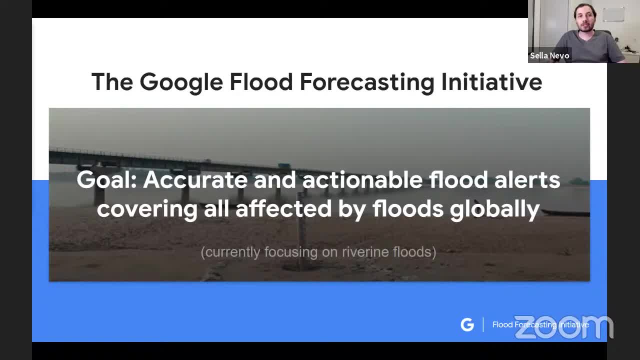 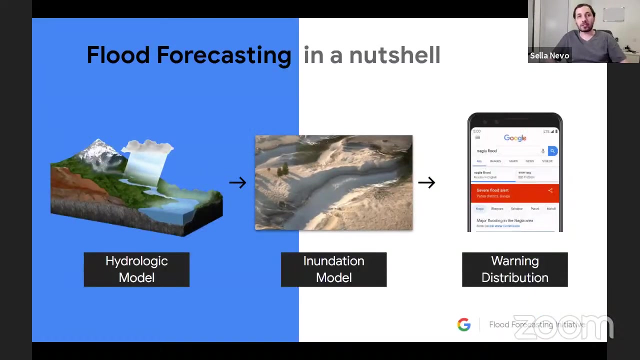 to flash floods or coastal floods, and today i want to talk about the challenges in scaling riverine flood forecasting systems to global scale, while retaining the accuracy and actionability of high end systems, and also discuss some of our recent progress towards that goal of high accuracy global flood forecasting systems. i want to focus on three important components. 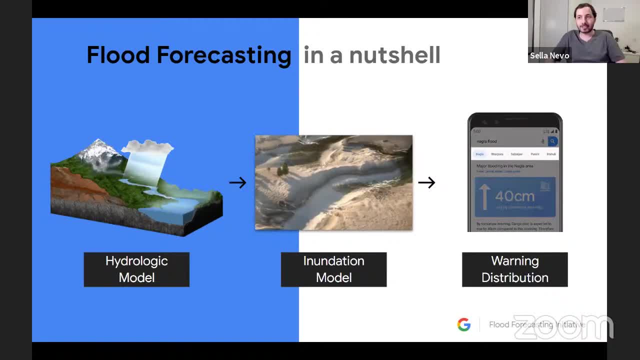 of such a system. the first will be the hydrologic model, the second will be the inundation model and then the third component will be the warning distribution at the end. let's dive straight into the first one, the hydrologic model, as i assume many of you knows. 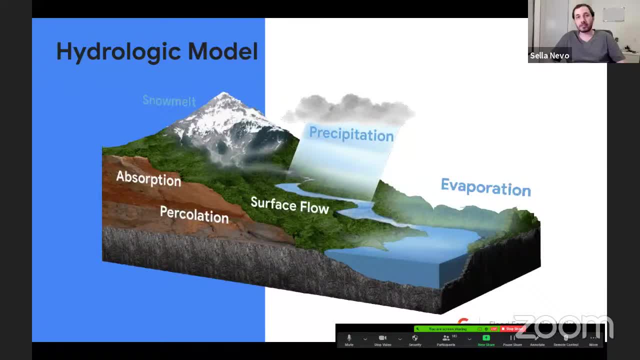 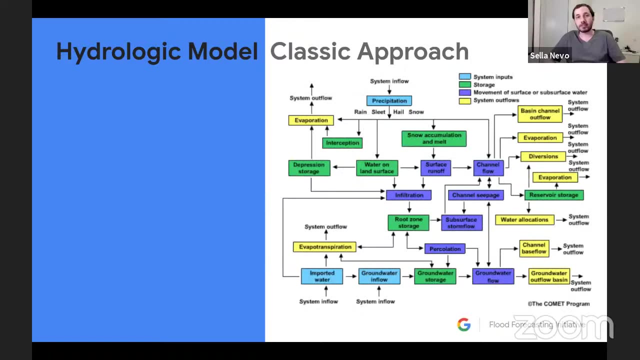 accepts various inputs, including precipitation, soil, moisture, though radiance and more, and produces as an output a forecast for either discharge or sometimes even water level throughout the river. and the classic approach for these kind of models is that each component represents a separate physical process, while in practice we don't have nearly enough information to 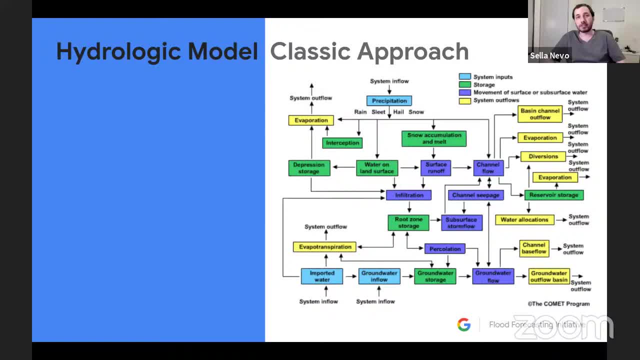 have actually defined the forcing data to implement full physics-based models, we use simplistic conceptual models that approximate them. now, this methodology, which today, ever since the- at least the models we're using today, many of them- existed since the 70s, has several disadvantages, several downsides. right one is that, despite being relatively 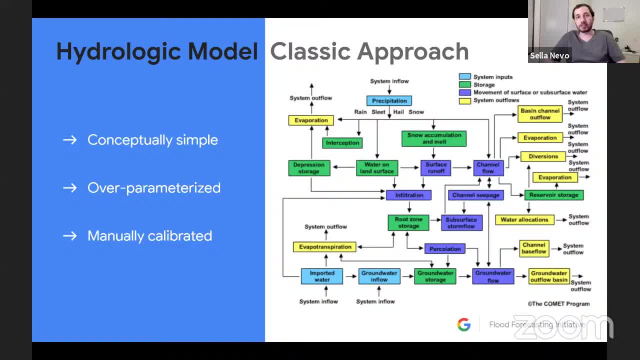 complex. from a human standpoint they're relatively simplistic relative to the actual typical processes. they are often open over parameterized right. we have a quality called equi finality, which means that many different parameters tend to lead to the same results and can match the historical data. but that doesn't mean they move towards in future predictions and they also 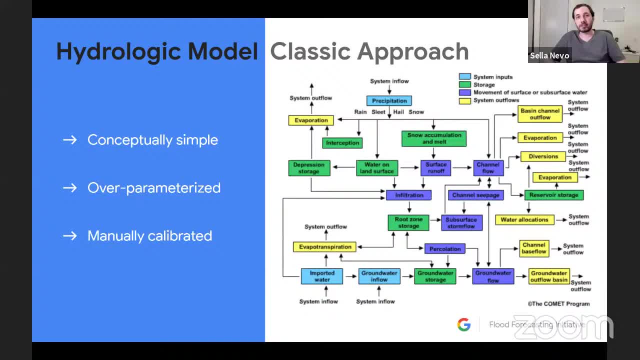 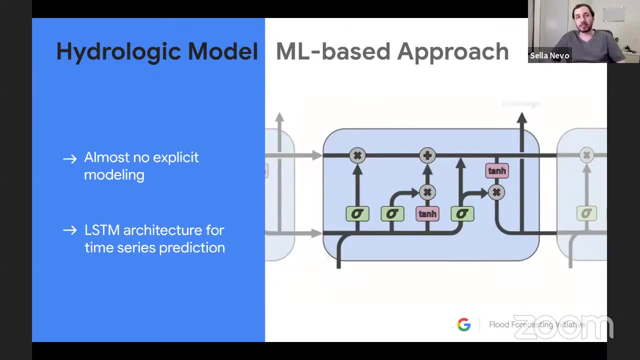 will often require continuous manual calibration, but at least the high-end systems that we tend to kind of trust the most will require manual calibration by experts, which can lead them to become incredibly expensive and not scalable, and so the approach that we and several other groups have been taken- 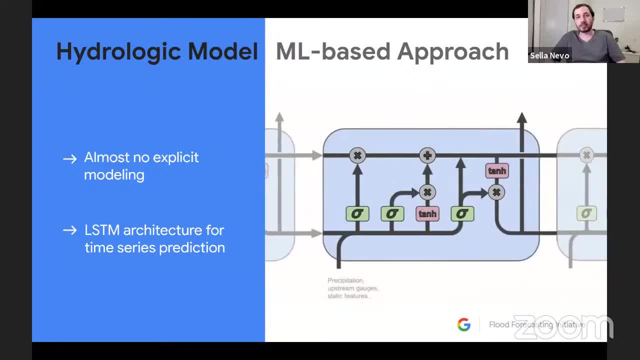 taking in recent years has been to kind of take a significant turn and instead go in the opposite direction of model of modern machine learning architectures. so, specifically, the type of model that we kind of we think the results have been most impressive so far- are lstms, which are a type of neural 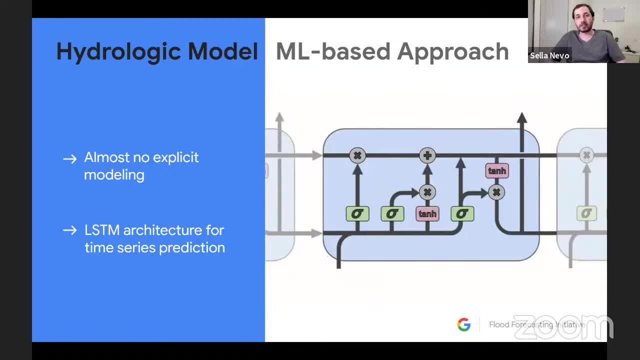 network that is optimized for modeling time series and specifically time series that require a long memory right. so, for example, in hydrologic uh models required to remember. let's say, if months ago uh there was more snow, that affects what happens right now, so lstms are very naturally. 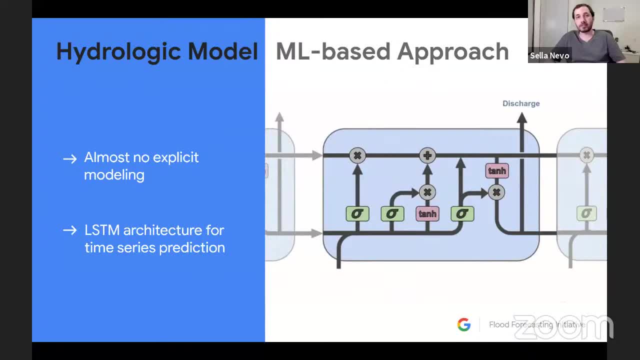 a very natural choice uh for doing this kind of modeling. but really the most important aspect of that i want to kind of share with these models is that there really is pretty much no explicit modeling of the different processes. instead, we allow the model to uh estimate the uh the different. 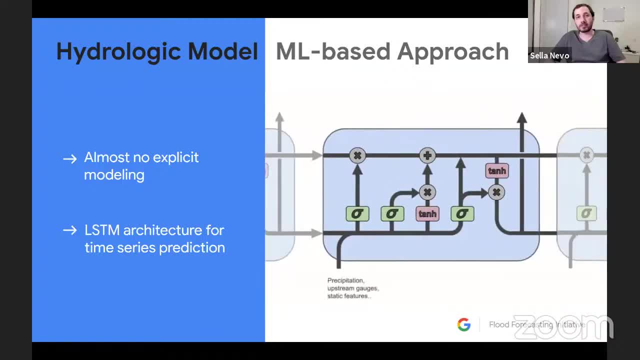 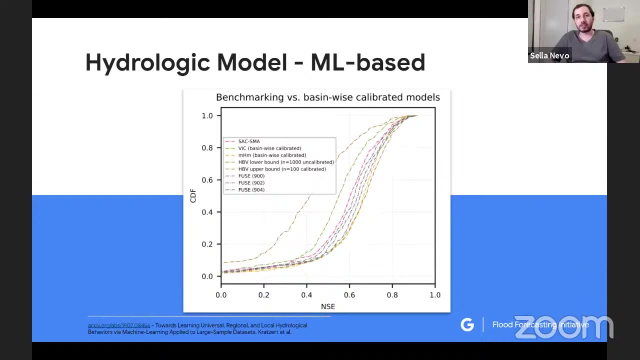 processes on its own, and while, of course, data-driven models uh have been kind of an option for many years and have often underperformed relative to more process-based models, we think that these modern architectures are showing us some different results that are really important and are worth uh taking note of. so uh one result that i want to share, and this is work done in- 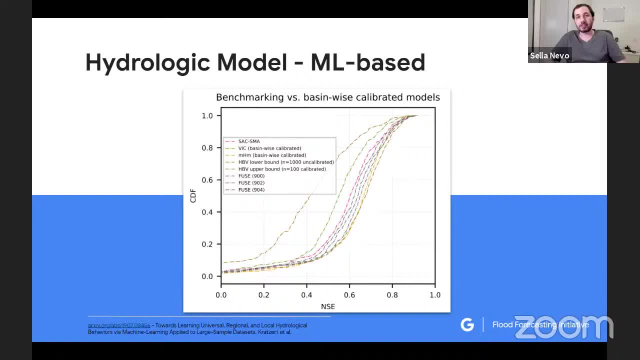 collaboration with uh frederick kratzer and gray nearing and seth hochreiter and several other contributors. um has shown that when benchmarked across a wide range of basins- this is specifically based on the camel's data set in the united states about over 600 uh different uh gauge sites across. 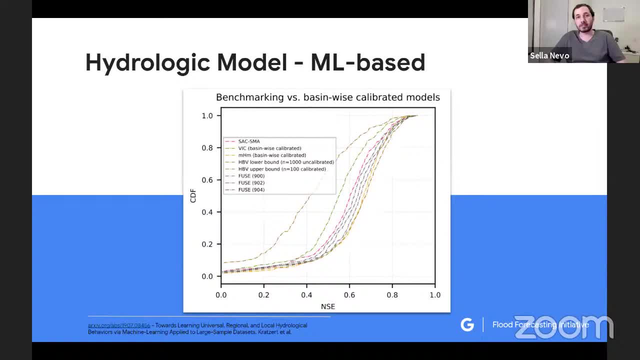 the united states. we achieved some very interesting results, so i'll take maybe a minute to go over and broadly say what we are seeing here. so this graph is a comparison of different models across the united states, so each line represents a different model and you can see. 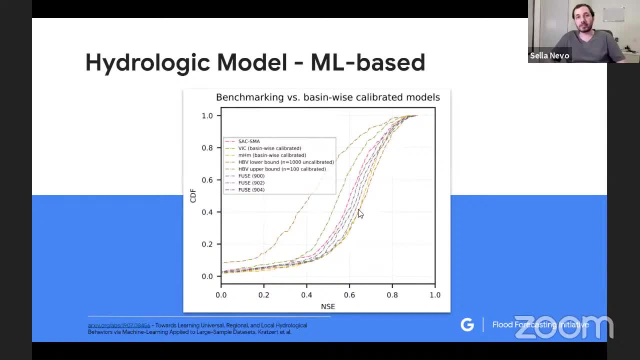 here the different uh ones, that that have been benchmarked, and um. what you're seeing is a cumulative distribution function over the nash sutcliffe efficiency coefficient, um. but for those of you who are not familiar with these terms, all you need to know is lower is better. 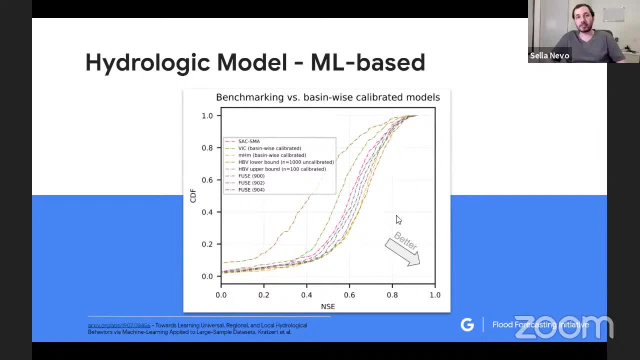 right. that means we're getting better scores on uh on more sites, and here you can see the performance of these new lstm based models across all these sites, and what we can see is a significant improvement across uh different sites, and it's also worth mentioning that these benchmarks are 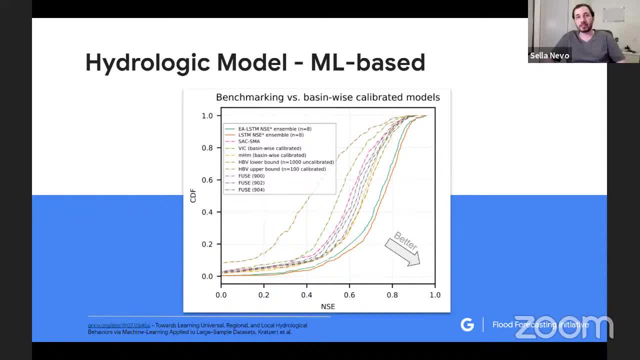 compared to when the creators of the original models have benchmarked it themselves. it's not us benchmarking, uh um, the other models that we are competing against. but in addition to quality improvements, there are two other advantages that are a bit harder to see from this graph alone. 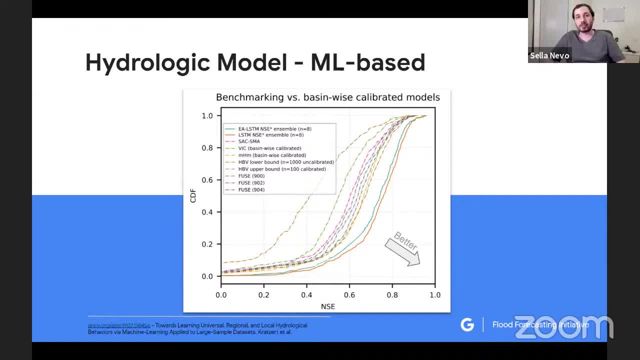 in these kinds of models. the first is just scalability. while classical models require kind of continuous calibration and often recalibration to achieve high accuracy. these models have been trained with a single lstm, trained across the full data set. so this is a single click button, a single training. there is no. 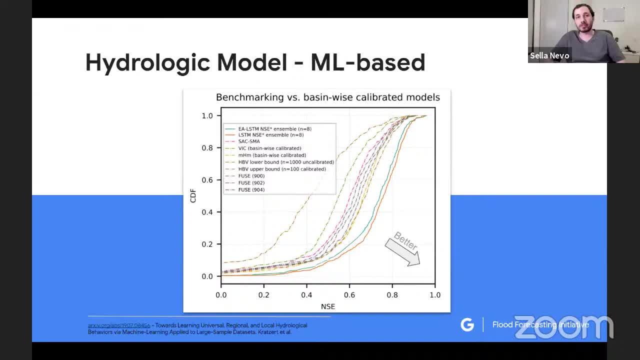 manual calibration in this process, which allows us to scale this to many more locations than was at least convenient in the past. and then the second is generalization. actually, the graph that you're seeing right here is not a fair comparison between these models, all classical models that 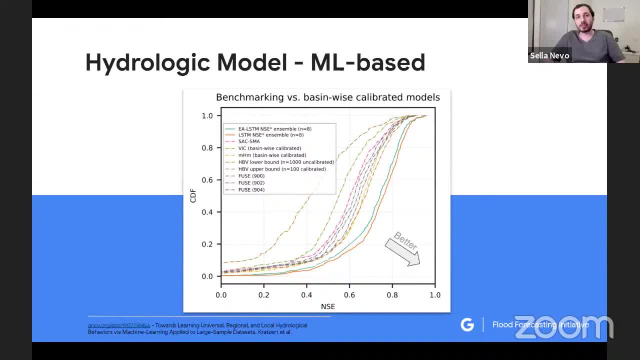 you've seen originally, have been given data for the specific basin that they are being tested on, while the two lstm models that you're seeing here- these two lines, have had the side that they are tested on hidden from them. all of the results that you're seeing here are for sites. 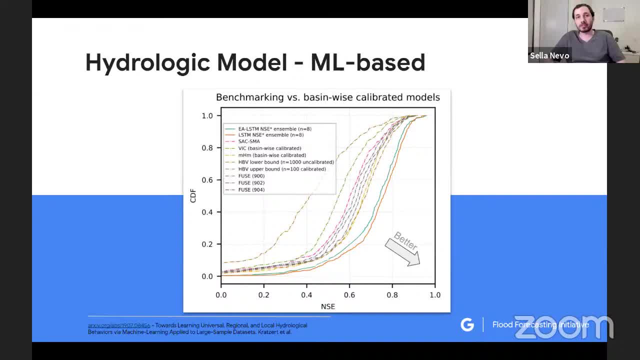 that they've never seen data from the site that they are being tested on, and what this means is that this really gives a lot of room for hope for kind of ungauged uh basin prediction. right, because this means that we can achieve, uh, some level of generalization. just a caveat: i'm not 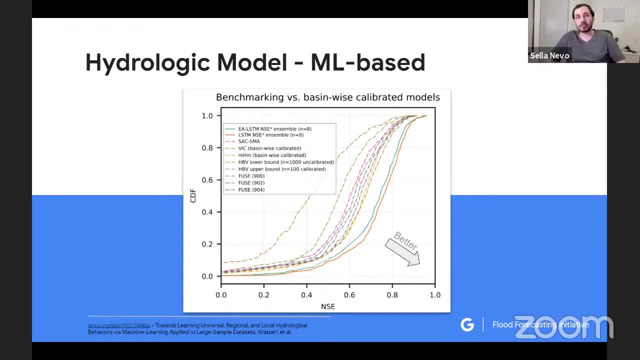 trying to claim generalization across completely different regions. these are all have been trained in states and have seen similar gauges, but there's at least some level of generalization here. now. this is still a work in progress. we're still working on, uh, a lot of improvements to this kind. 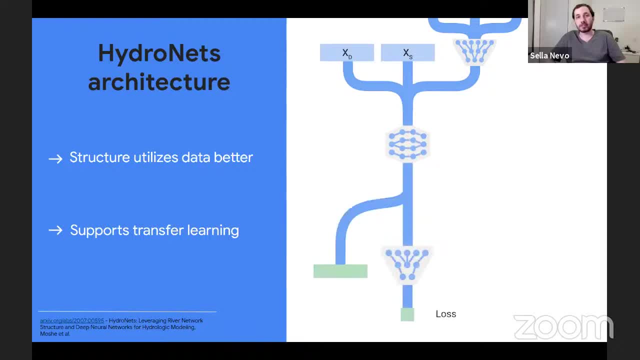 of modeling uh. two things that we are particularly focused on right now is, one, how to efficiently communicate information between locations across the uh uh, across the river network, and secondly, also combining this kind of shared model transfer learning approach that we've used in the previous slide uh, but combining that also with per site modeling that. 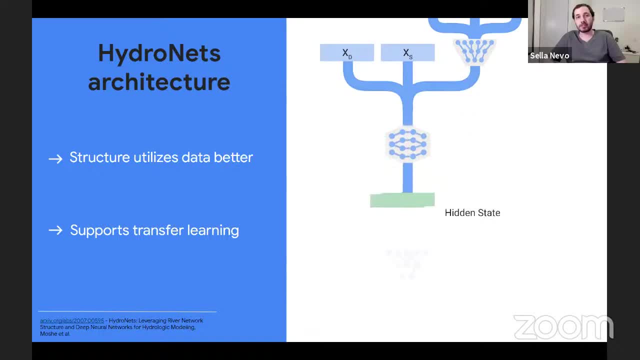 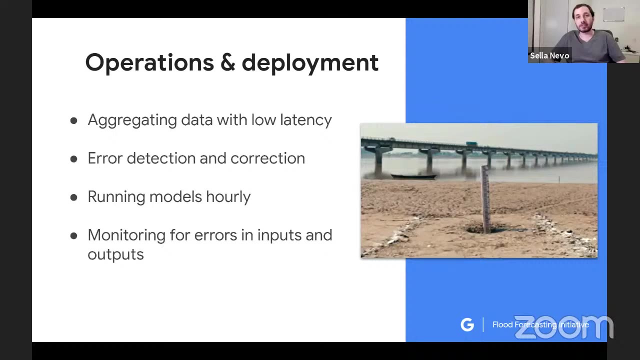 will allow the model to specialize more effectively to sites where we do have data. but we think there's a lot of exciting, exciting things going on here. of course, for these models to be useful in practice, we don't just need to improve kind of academic results. it's no less important to 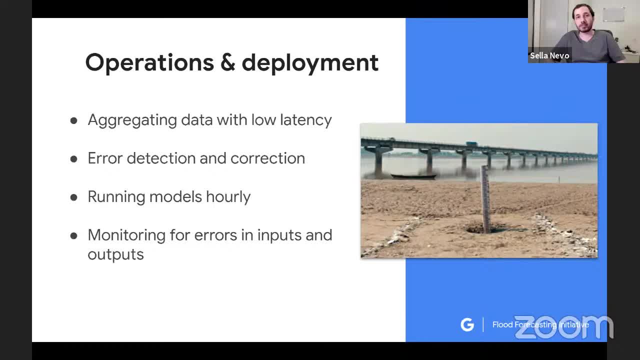 tackle the practical issues that are inherent to real world data and operational systems. we've done a lot of work in recent years on reducing data latency, detecting and correcting errors and data collection and increasing the speed and frequency at which these models are run, uh, which is kind of a bit less uh sexy in uh in conferences, but it's critically important. 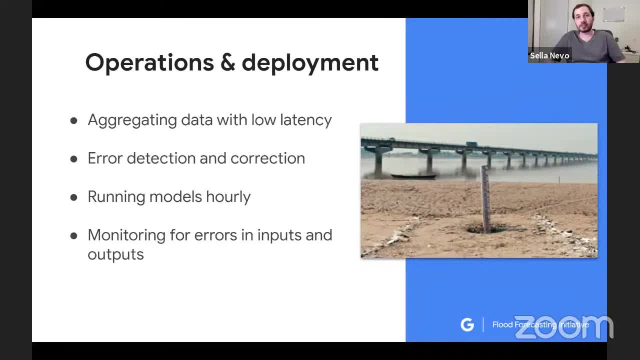 uh for uh, using these models not only in academia but actually creating change on the ground. and this hard work has allowed us to launch these systems operationally uh and currently covering about 75 million people in india and bangladesh, in collaboration, of course, with the indian central water commission and the bangladesh water development board. 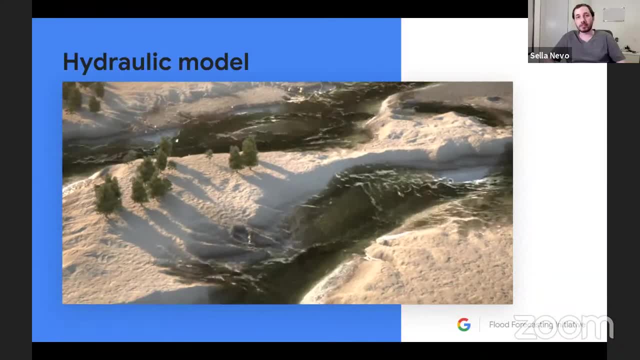 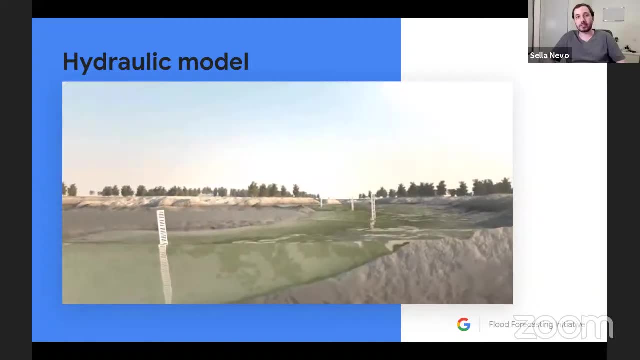 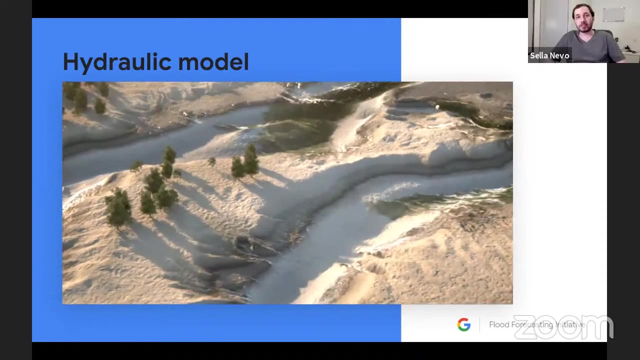 so we've deep dived into the hydrologic model. i want to move on now to the second component of an actionable flood forecasting system, the inundation model, or sometimes called the hydraulic model. now, these kinds of models simulate the water's behavior across the flood plane, like you're seeing on the screen right now, and this allows us to understand what areas. 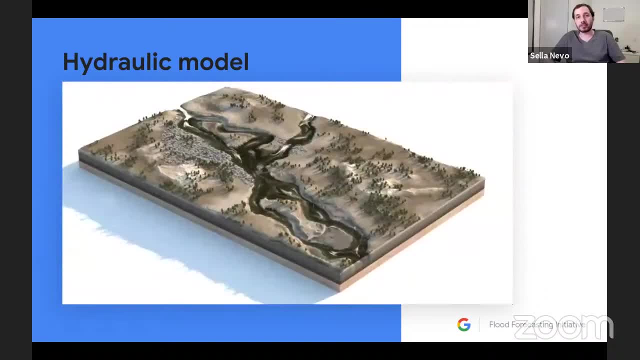 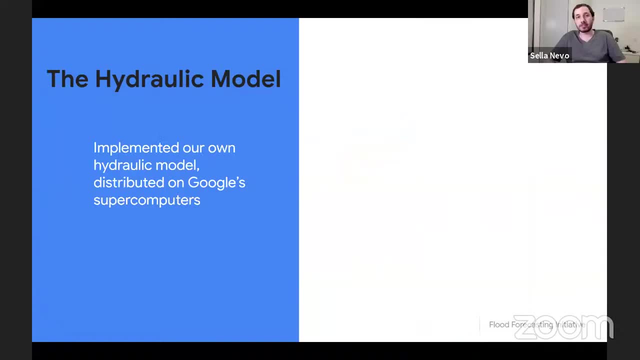 exactly, are going to be affected by an upcoming flood, and this means we can identify an example of this model. uh, that can be used in many ways and, of course, the first one is a. so it's these models that i'm showing you right now and in the video that you're seeing. 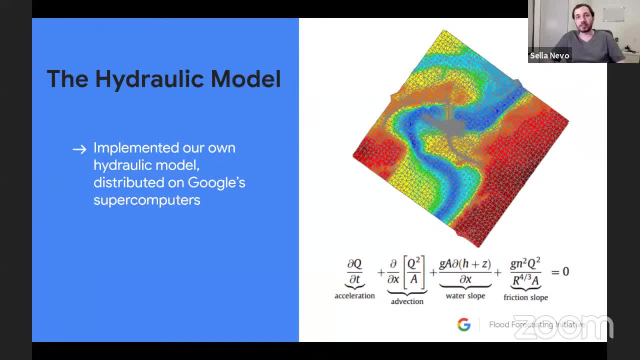 the sketches are those of the water levels that we have here, and this is an example of them as well. so this is the hydrologic model we're using, and this is one of the main models where we can build these systems from the very, very beginning. so you can see we can do what. 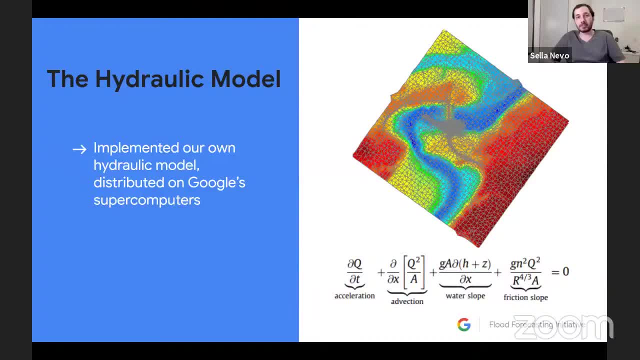 you're seeing right now, this is the water level and this is the water level increase and so on. but we've kind of re-implemented them so that we can distribute them efficiently on Google's supercomputers. But right from the start, if you want to scale this thing globally and specifically, 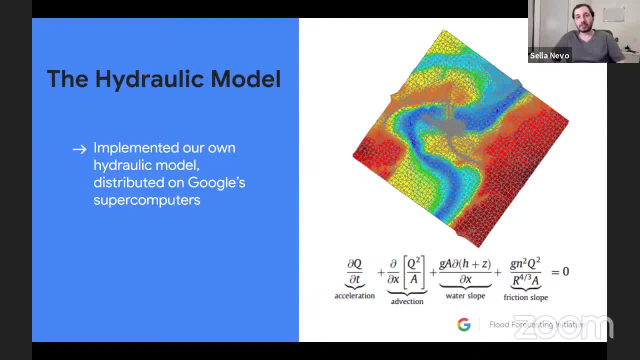 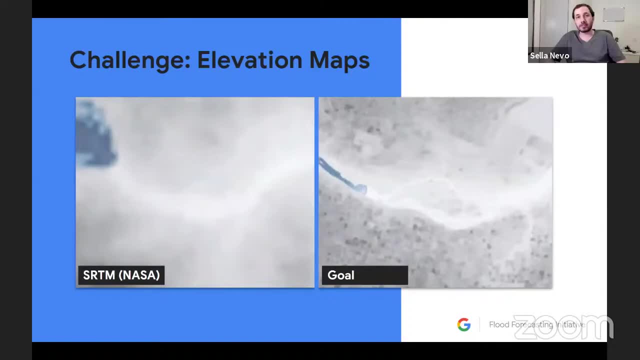 for the regions that currently have the largest amount of flood-related fatalities and harms. you run into a few challenges very quickly. The first challenge is elevation maps. These models rely critically on elevation maps, at least if we want highly spatially accurate results, And in the majority of the world it's very hard to attain maps that are. 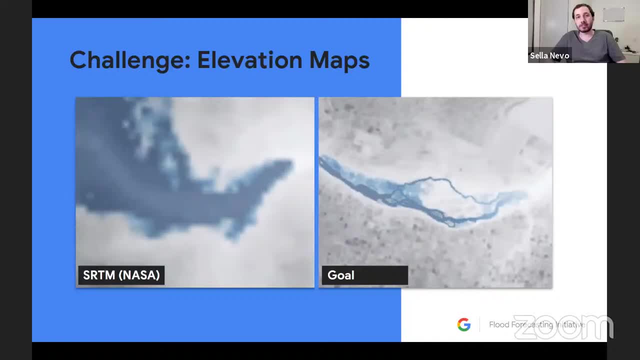 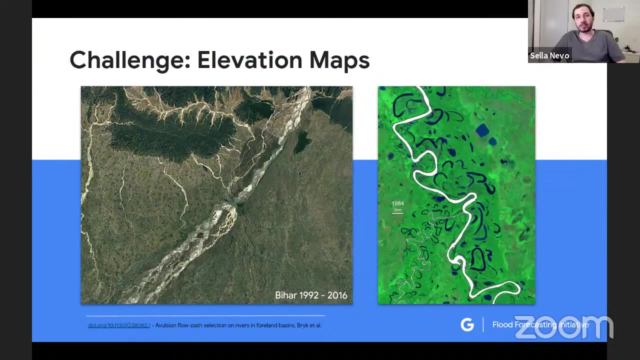 at high enough a resolution to be effective. You can see here an example of the simulation of the same river near Hyderabad, but one with one meter resolution and one with 90 meter resolution based on SRTM's elevation maps. And a second challenge is that, even if you go through all the work and 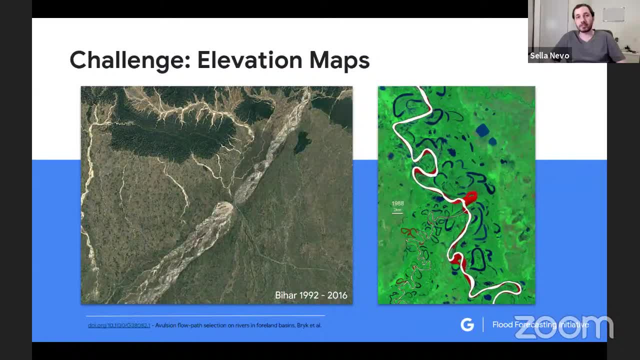 either purchase or collect data that's relevant to producing an elevation map. still, you're not going to be able to achieve the same results. So you're not going to be able to achieve the same results, especially on a global scale. Very quickly you'll find that it becomes. 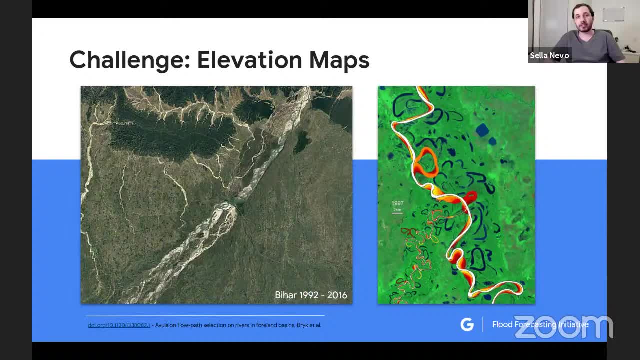 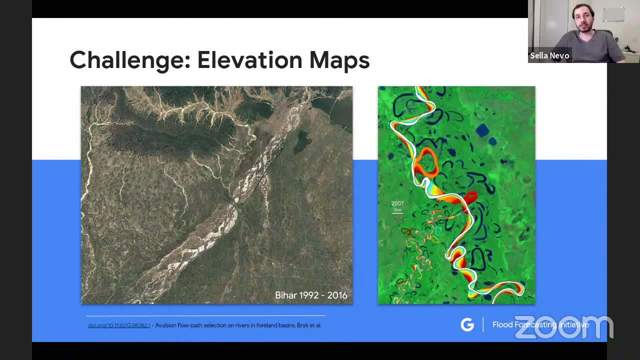 out of date, because some rivers change at a high rate and we care about the morphology now, not several years ago maybe, when we collected the data. And the challenge is that producing these can be expensive, right? One classic way of doing this is through stereographic imagery. 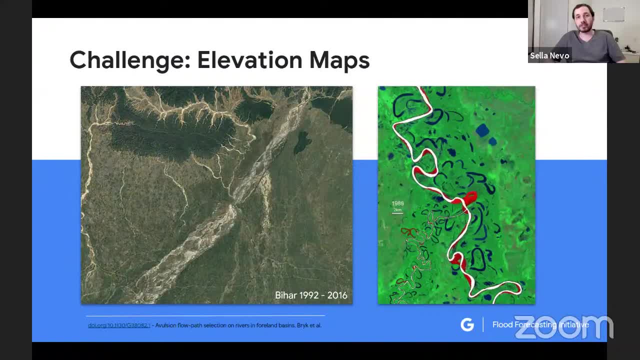 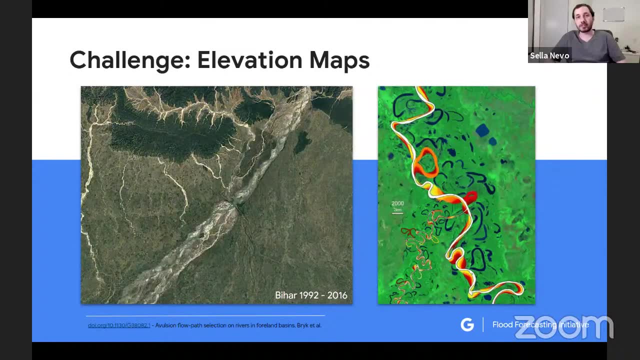 where we take multiple pictures of the same location with, let's say, a satellite or a plane. But again, because of these costs, if you want something that is global, it'll be at a low frequency and so your data will be stale. 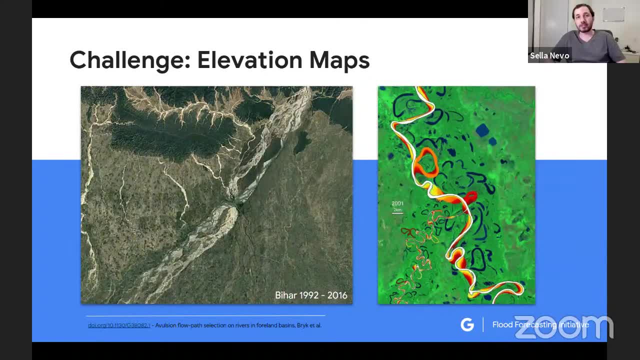 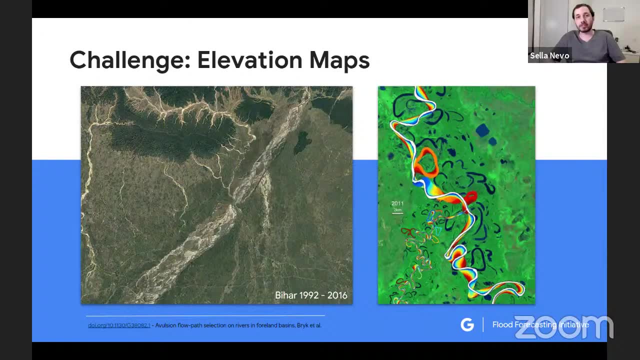 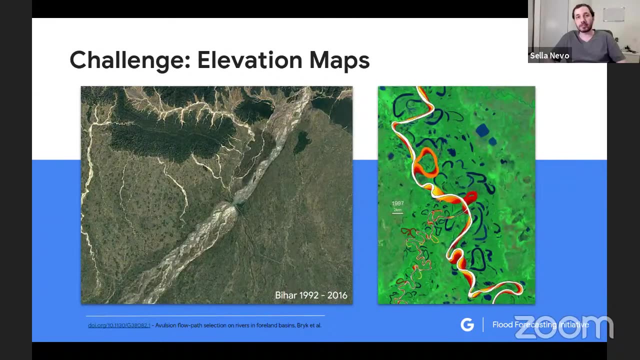 We've taken a slightly different approach to producing these elevation maps and, instead of using expensive specialized satellite missions, we purchased large amounts of high-resolution optical imagery that is captured anyway every day across the globe. These are completely standard optical images, no specialized devices or missions required, And what we do is we then do a process. 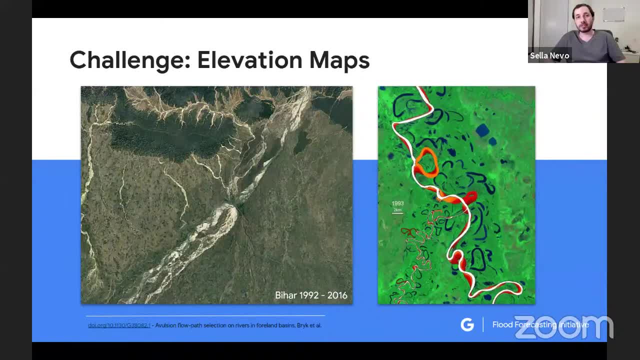 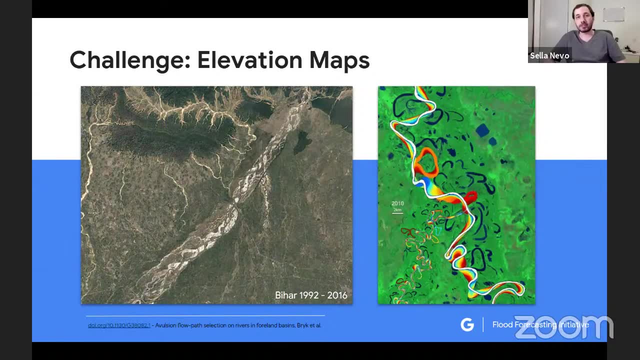 that is somewhat similar to stereographic imaging. We use the differences between the images to deduce the height on the ground, but using these arbitrary images, which is much harder work on the software side, but that allows us to produce these high-quality images on an annual basis anywhere. 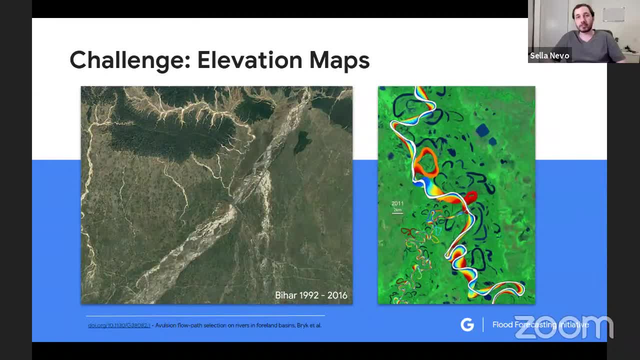 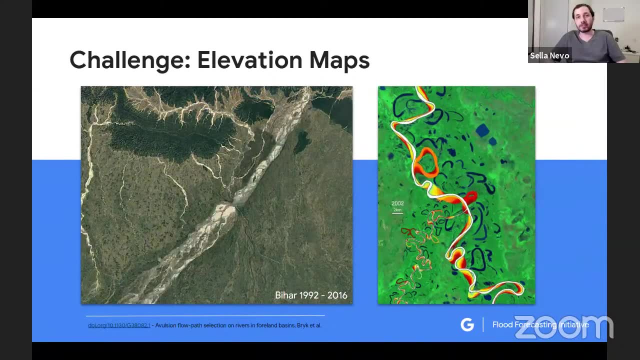 we'd like in the world, And here you can see an example of that. This is specifically in the Yamuna River, going through Delhi. But that's still not enough, and I want to share one example, maybe that we've run into What you're seeing here. 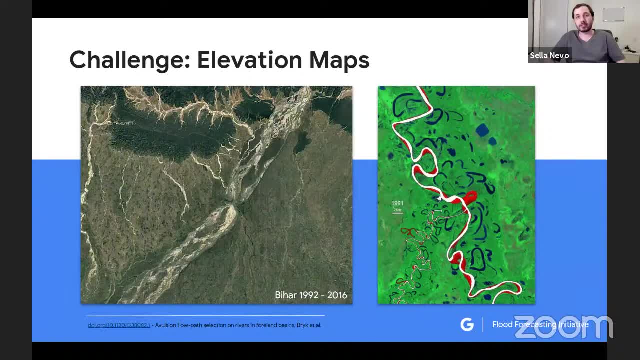 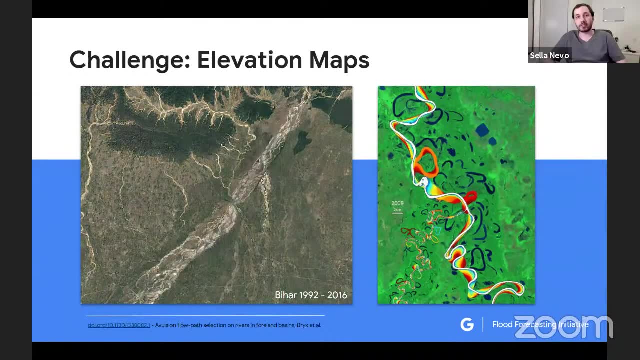 is an evaluation of one of the first alerts we ever sent out, And this one was in Patna about two years ago, in India, And what you're seeing here in blue is areas that were indeed inundated and we've alerted. In purple you can see areas that were not inundated but did receive. 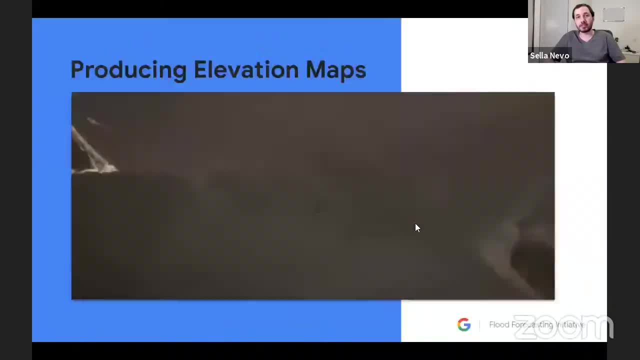 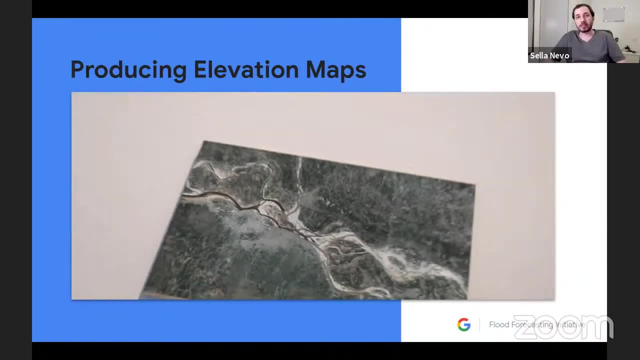 an alert. The idea was to also warn people who are very close to the inundation, so we felt very comfortable with the purple buffer. you can see here The red blobs are areas that were inundated but did not receive an alert, And that's of course a big problem and we have. most of them are pretty small and rare. 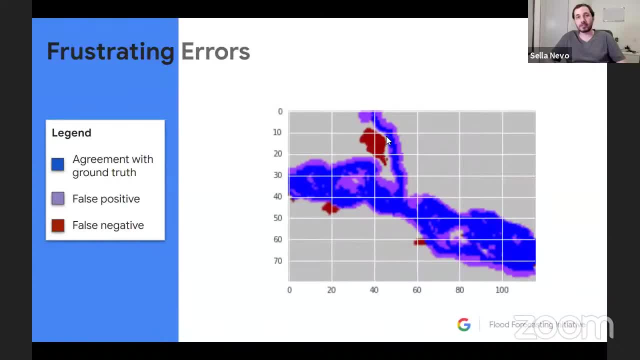 except this big annoying blob of red here which frustrated us for months because we just couldn't understand it. It didn't make sense physically. There's a huge embankment between the river here and the area that's flooded, and we couldn't understand how that happens. So we ended up. 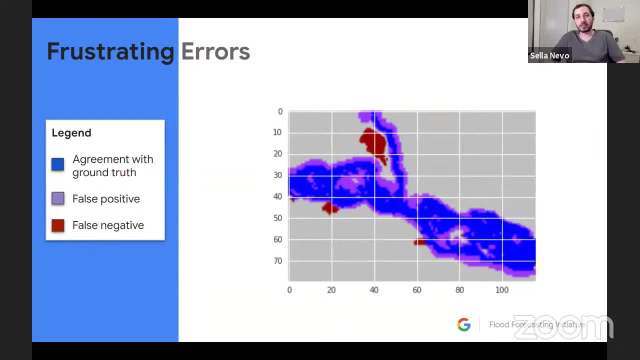 flying to Patna and talking to the farmers there, and immediately they told us: oh, of course, when farmers want to water their fields, then they'll kind of dig holes in the embankment so the water surpasses And this is very obvious. 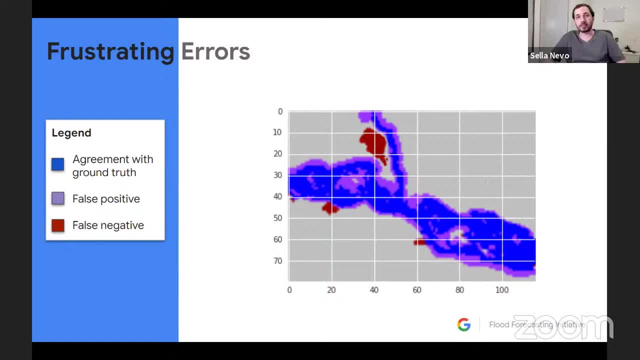 It's something that would be very hard for us to know, based on satellite data. So we started asking ourselves: well, how can we automatically learn this information? We want to be able to learn from experience, since we do have various types of data, let's say, optical imagery. 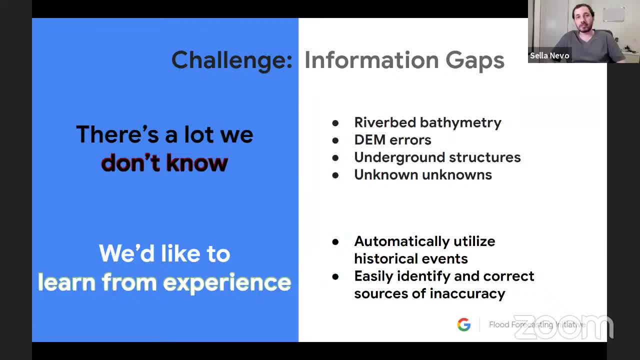 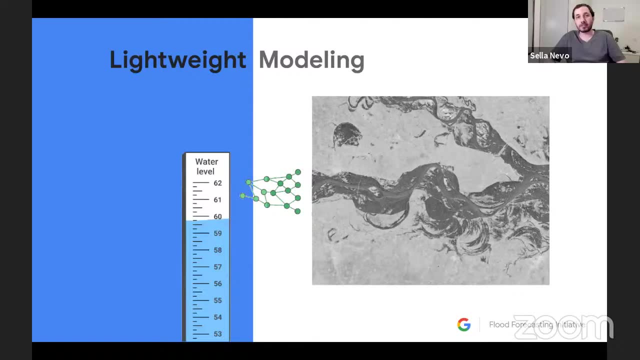 and SAR imagery. So we wanted to automatically learn those aspects of the flooding behavior that we don't know a priori from first principles or from the data that we have, And what we've developed is an end-to-end machine learning model that correlates the gauge measurements directly to 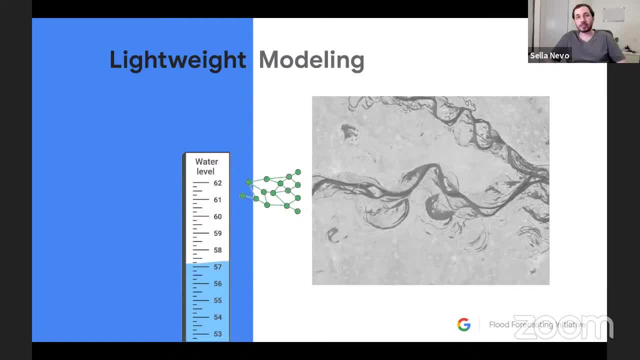 the flooding patterns. Now, this performs far better than physics-based components in areas with data scarcity, when the data we have to work with is pretty limited. But of course it might not perform well, let's say, in unprecedented events and other. 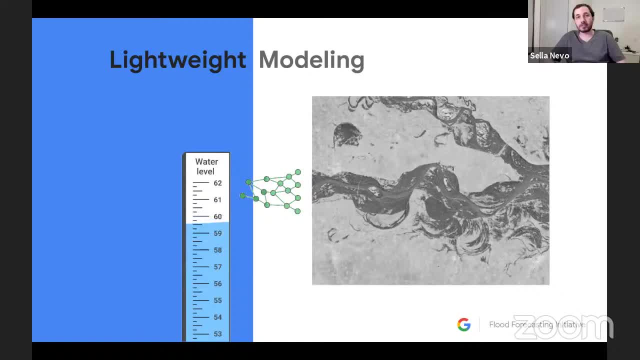 challenging circumstances. So we set out to combine these two approaches and to learn on the data that we have and to use them to work on the data that we have. and to learn on the data that we have and to learn on the data that we have. So the end-to-end machine learning model. 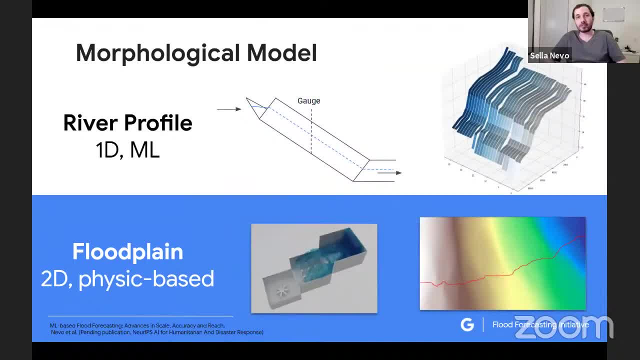 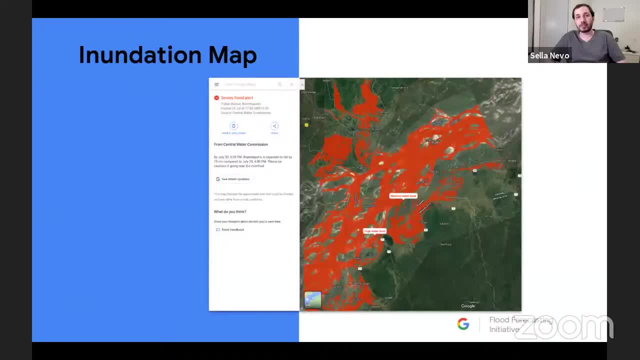 was a little bit more complicated than we had expected, But it's great for us because we can learn automatically what we don't know, For example, anything that has to do with the riverbed, which, at least in the elevation maps that we produce, doesn't include the bathymetry. 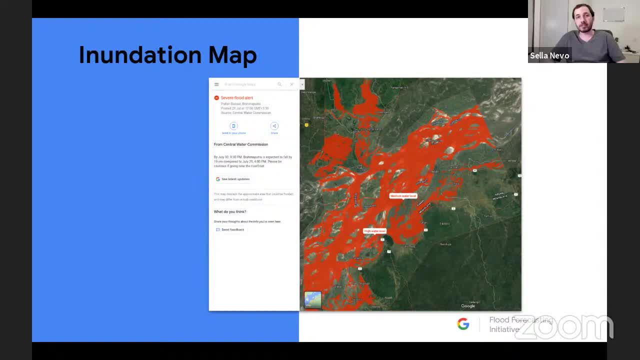 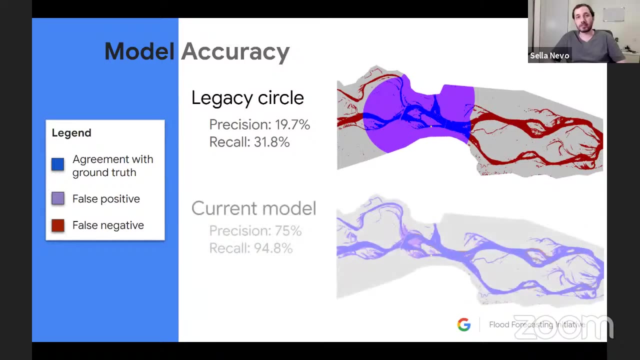 since it's optically based, while still extending much of that information to the full flood plane using physics-based processes, cover about 240 million people, and we're working hard to expand them further. now i said this is accurate. um, i want to so. here you can see an example, if you look at the bottom here, of another. 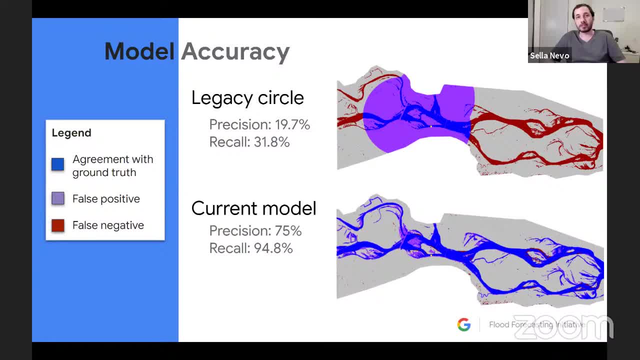 comparison between our forecasts and what ended up uh happening. based on optical and star imagery and uh, as you can see, at a 64 meter resolution, we achieve pretty high precision recall, which means that we're usually right about what every 64 meter uh area on the ground. 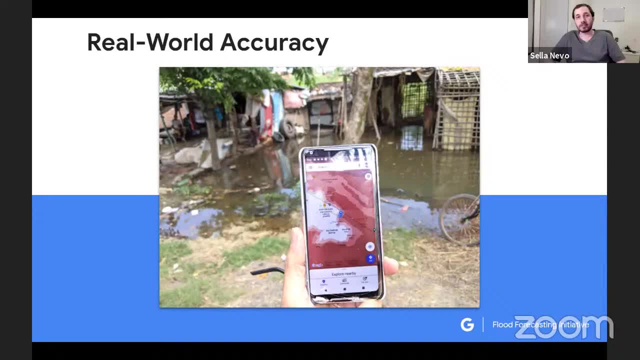 of course, this is even more kind of uh inspiring to see when you look at it in real life. this is when we were uh in, uh, bihar, india, uh, while flooding occurred, and here you can see kind of our forecast. we're standing right at the edge of where we expect flooding to begin and, as you 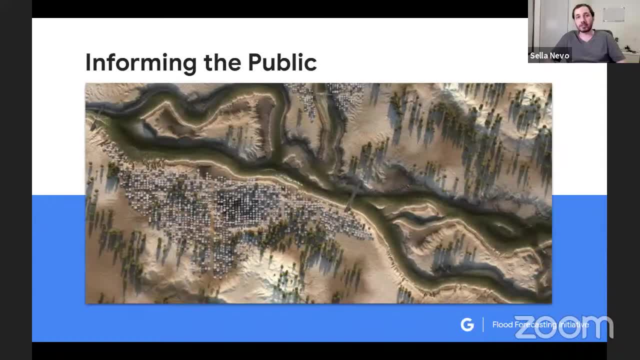 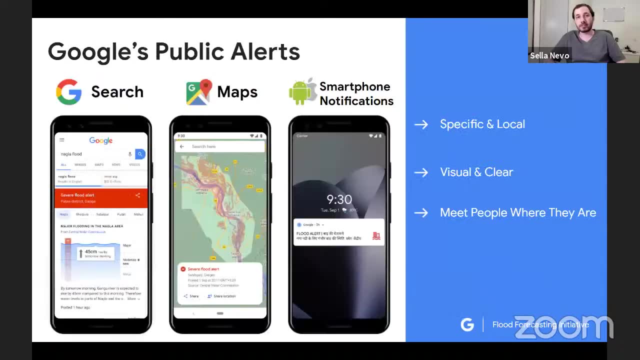 can see. that is indeed where it happens. finally, i don't have much time, i just want to quickly mention: uh, of course, none of this is useful if it doesn't reach the right people in the right time, and we use google's public alert in alerts infrastructure to notify millions of people. 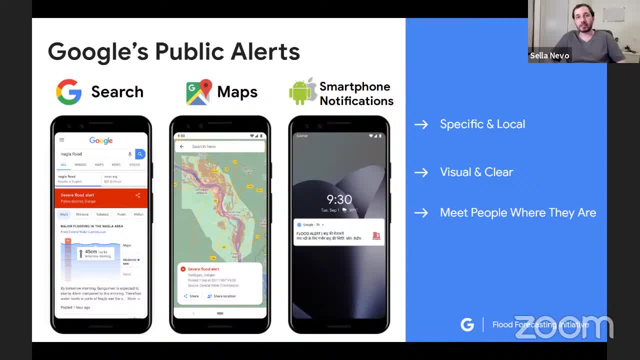 within minutes of an alert, we can notify them, based on existing alerts that we get from governments and disaster management agencies, or based on the models that we just talked about, which we developed and approved in partnership with the relevant governments. we put a strong emphasis on making things visual, providing local information, making 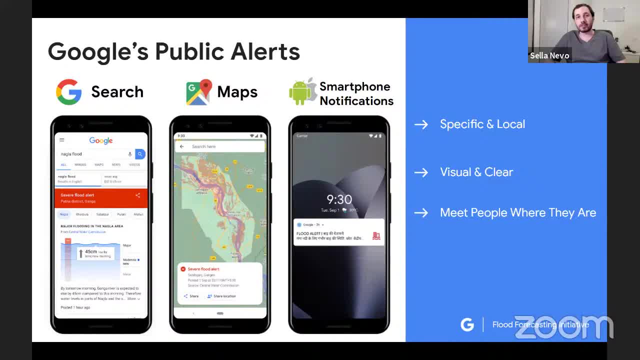 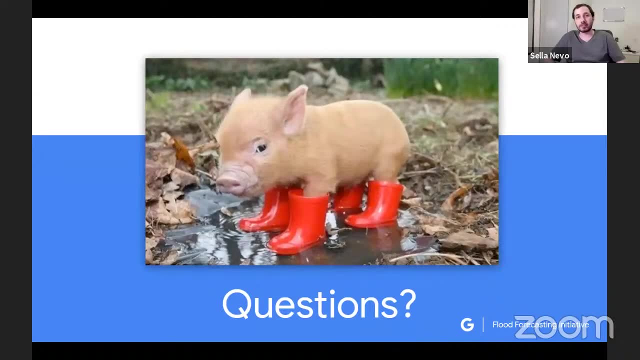 them interactive, supporting local languages, and just over the past few months we've sent uh active alerts of warning to more than 10 million people. so that was kind of a quick overview of what we think are the most uh interesting challenges and what we've done so far to try and address them, and thank you all for listening. 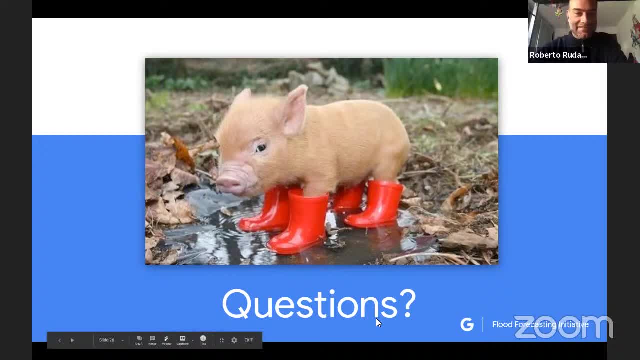 well, thank you, salah, definitely. i mean it is uh really like again a dense presentation, i mean full of inspiring. i mean uh full of inspiring, i mean hints for everyone and uh congratulations, for i mean all the challenges that you've been uh taken upon. thank you for that. i i i'm for forecasting a lot of i mean questions actually. i mean coming up in 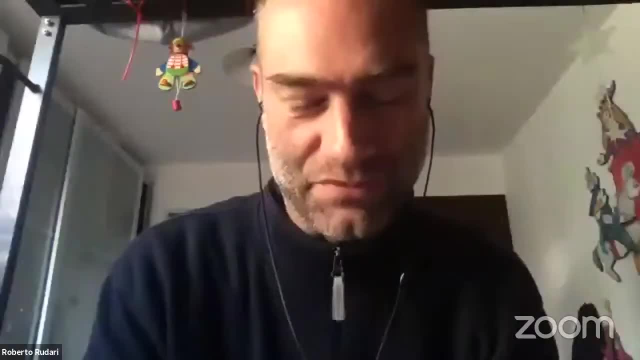 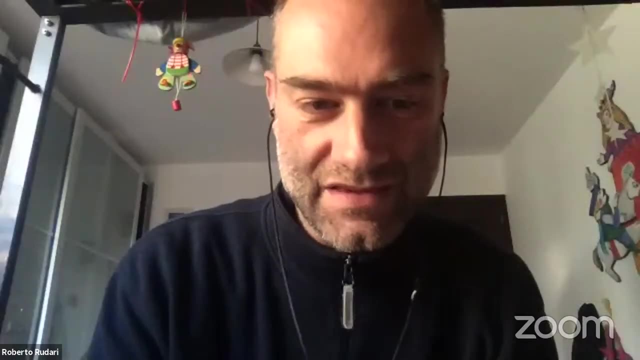 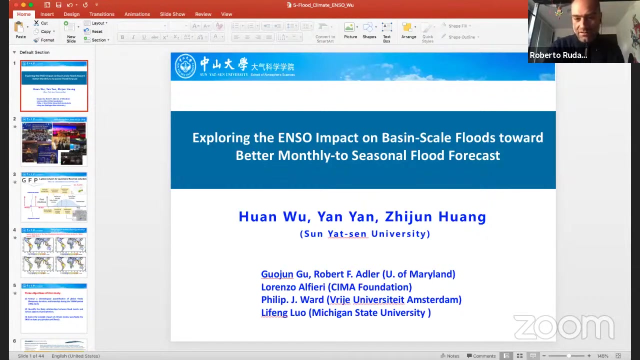 the chat, i mean in the next few minutes, i'm pretty sure. with this, i would like uh actually to give the word to our fourth speaker, one uh that uh will speak about. uh exploring the answer. impact on uh capital catchment scale- floods. there was a better monthly to seasonal forecast, so something more. 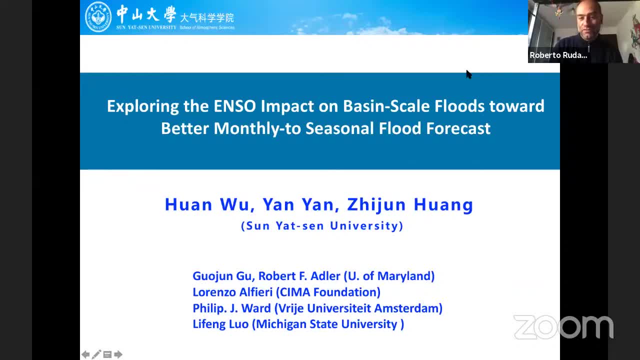 let's say classical. uh, please one. i mean, the flow is yours. hello everyone, can you uh hear me? yeah, perfectly, one, go on. yeah, thank you. thank you very much for having me. um, yes, uh, my topic will be a little uh different, but still, i think it is a very right one. 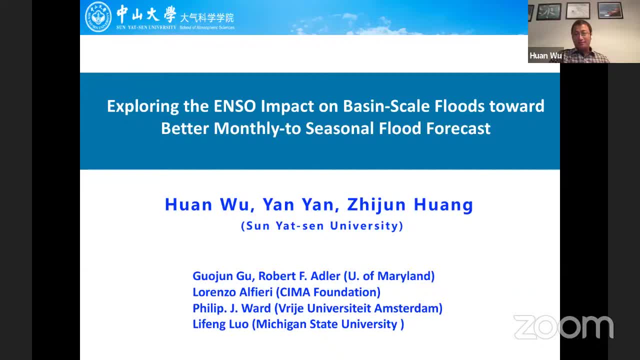 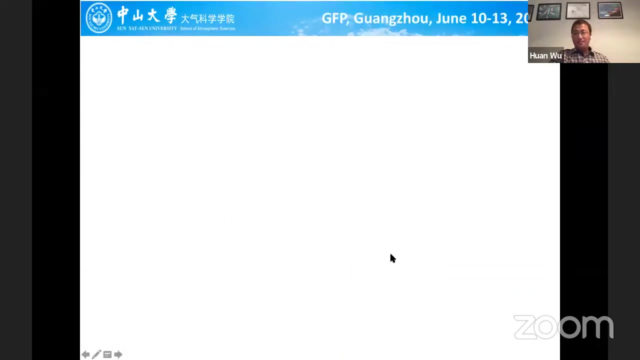 to this topic and I'm gonna talk in something a little behind of the system updates by previous speakers And this work has been done recently by my few students and some colleagues listed here. And first I'd like to share a few photos we took from last year's GFP meetings. as many of GFPers 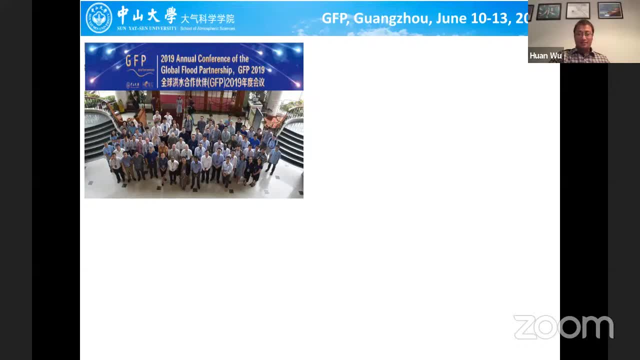 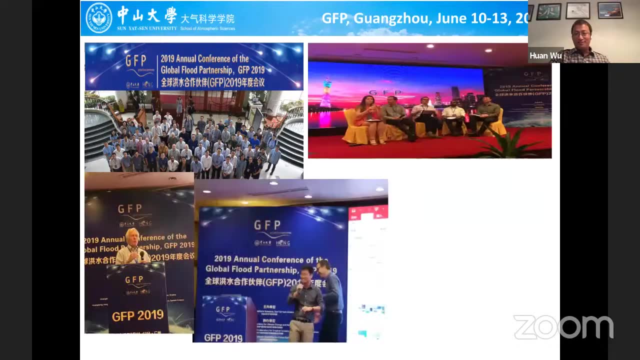 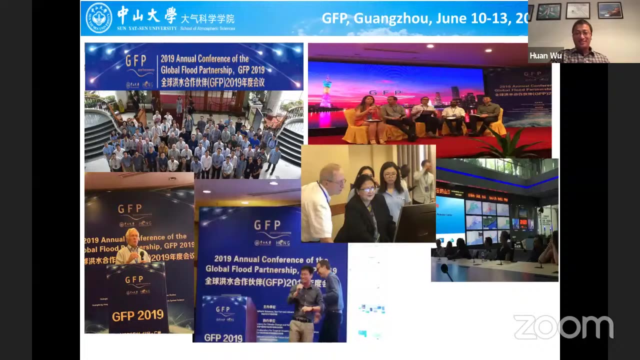 and participants may not attend last year, but of course not this year. we cannot do it, But this moment hopefully can give you guys some good memories And it's always been very nice to see GFP meetings. We see GFPers every year face-to-face. 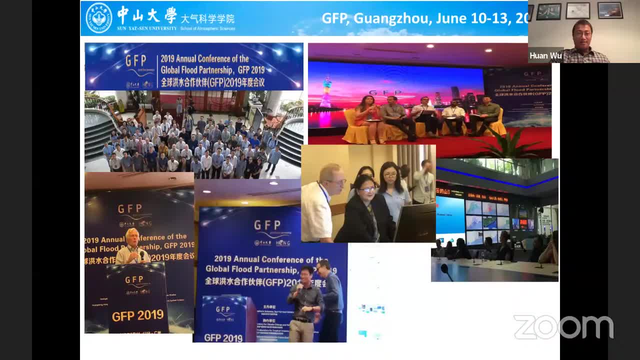 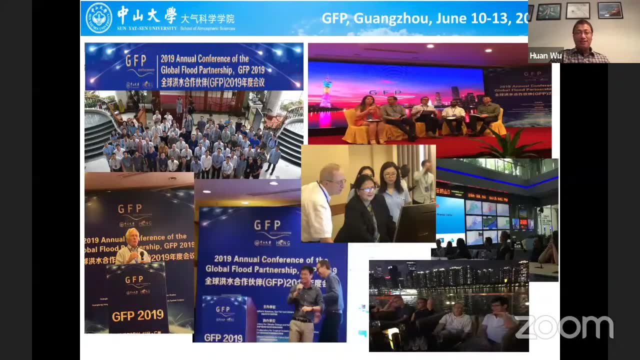 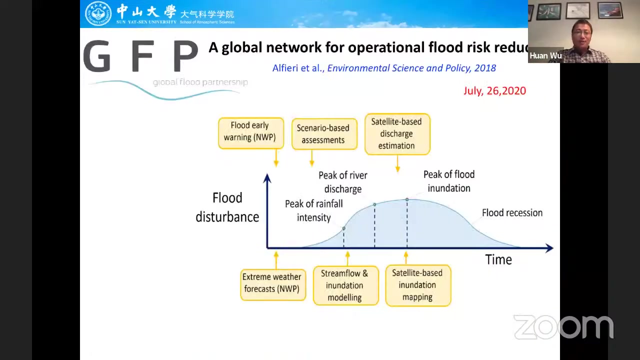 with a lot of updates and science, chatting and meetings and hand-on experience and also, of course, some beers. These are really good memories and hope everything come back to the normal sewing And so now I come back to my normal life. Usually I talk about the flow of the floods. 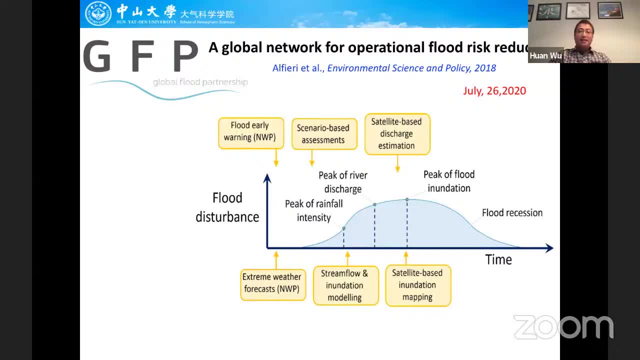 So recently Lorenzo Infuri and many others. We have a paper defines GFP as a global network of science and uses for operational flood risk reductions for a lot of flood events, from the early warning and to the flood recession, and monitoring all of these flood dynamics. 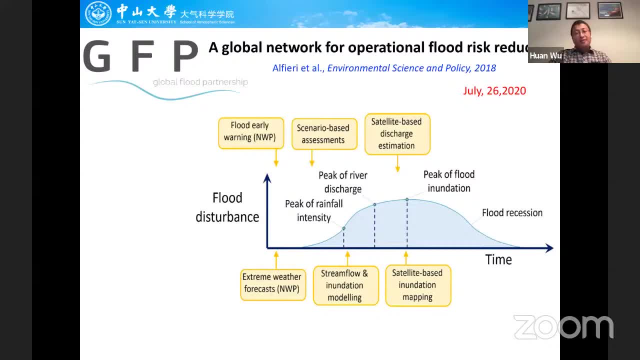 evolutions and the potential impacts, And recently, for this year, some of you may notice that in China we had a really serious flood problems and we do this similar thing And according to something like that this diagram defined, and we provide flooding information on daily basis. 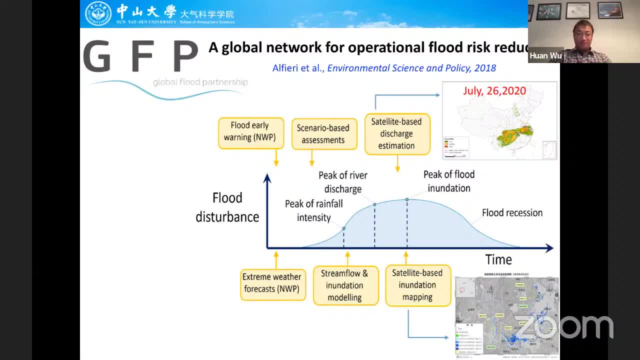 for the Ministry of Emergency Management of China, that's FEMA of China, And we got a lot of challenges of course for this response of the ongoing flooding events, as already mentioned by the speaker in the last week. So one of the questions and challenges we've got, 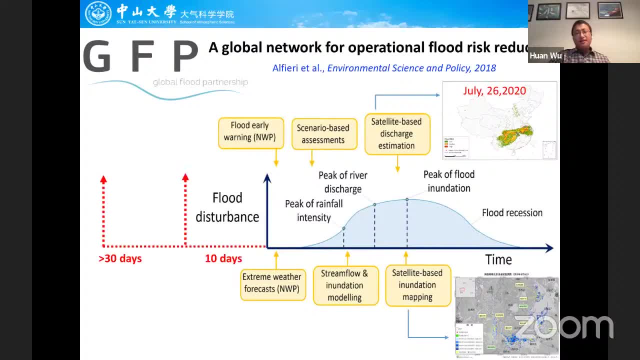 from this year's. responding from the MEM, they particularly ask us: how can we provide this flood information even earlier? They ask for like 10 days and even longer, but we know that it's very challenging And even when we provide the monitoring-wise. 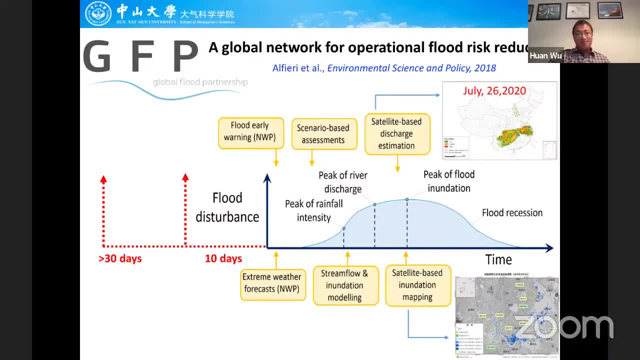 the data information, like from the real-time forecasting, and even for the one-day forecasting, there's a lot of uncertainties, as we know, And but with something we have to do and the next flood season, just I think it's just coming the way. 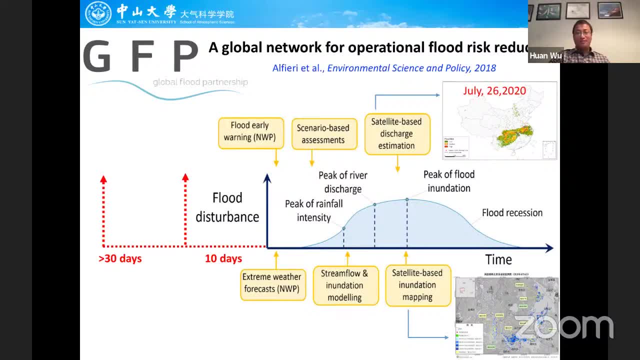 just a few, a couple of months away, we're going to have another flood season in China for the South Park. So look, so we, you know, we, you know, we, you know we have to do something. 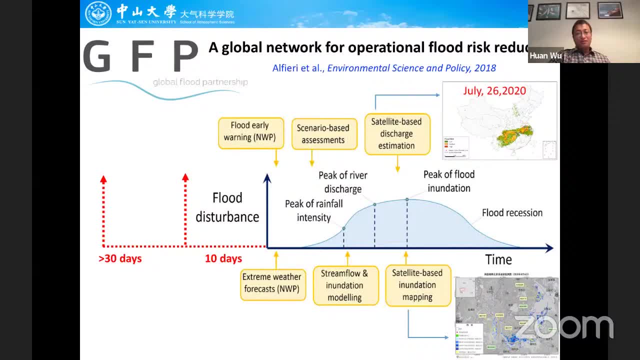 We have to do something. So what do we? what do we can do for this monthly? the seasonal forecast is is still always in our task list. So in this talk I'm going to talk about the what, some prerequisites to work toward. 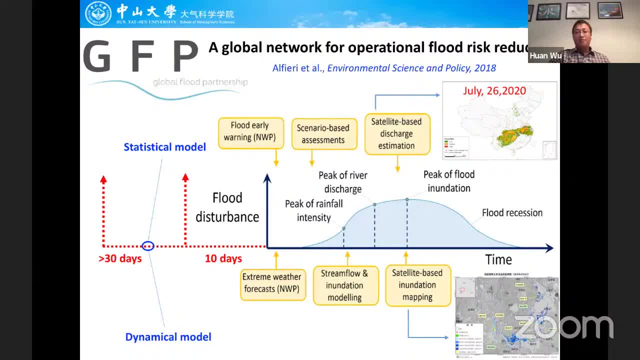 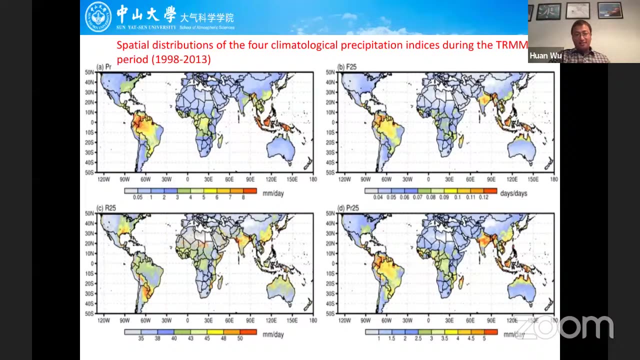 for better statistical modeling or machine learning, or provide more information for the dynamic modeling, for a better long-term or seasonal forecast. So so every flood has their own story and mostly are driven by different precipitation, So precipitation is a major one causing the difference. 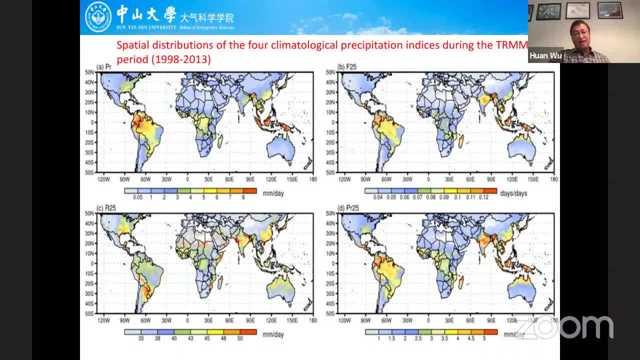 in the floods. but what are the characteristics of this precipitation actually are more important for flood occurrences than others, So it's not quite yet known. So what do you look at Here? is that we mapping the precipitation climb college, based around like 16 years? 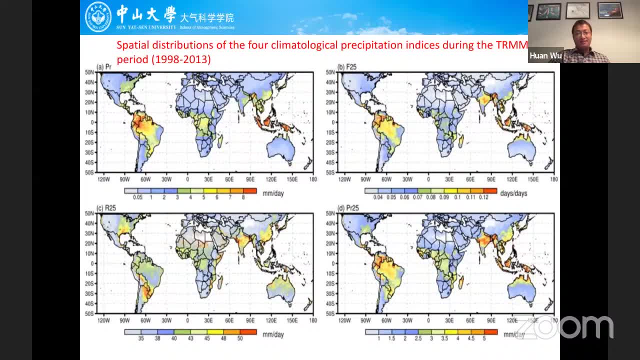 a trim data You can clearly say that the tablet panel PR, shows the total amount of precipitation And the way. the second one at 25, that's the frequency of the daily precipitation over there in 25 millimeter. And here's: 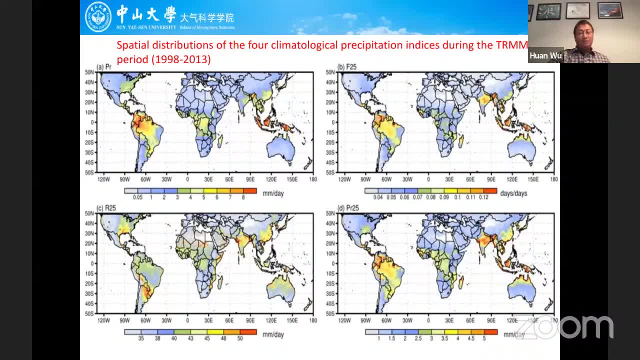 the intensity of the precipitation above the threshold of 25 millimeter, And the last one is the amount of the precipitation above the 25 millimeter daily. So you can clearly see that the white three panels shows a similar pattern, but the intensity shows a quite different. 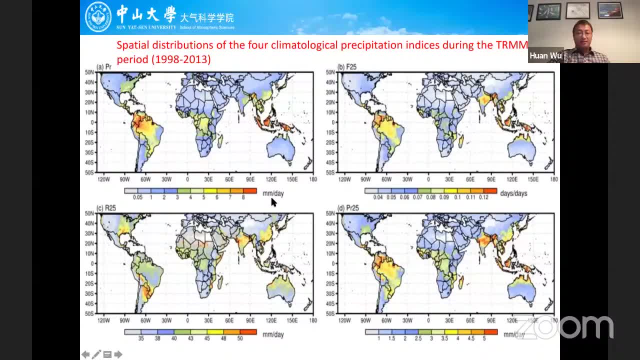 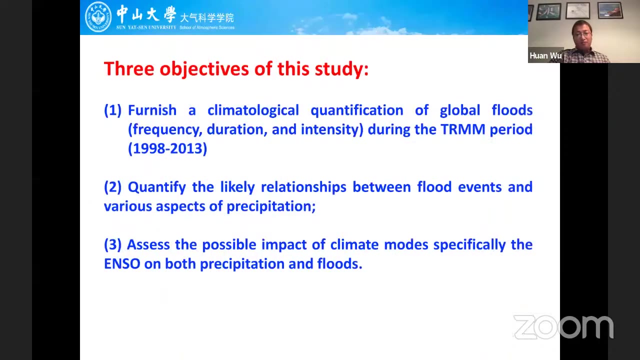 a huge difference than others. So the basic question we can ask right away which one- F25 or R25,, which one is more important to trigger flooding? And this kind of information is very useful for us to better understand the flood mechanisms and for the prediction. 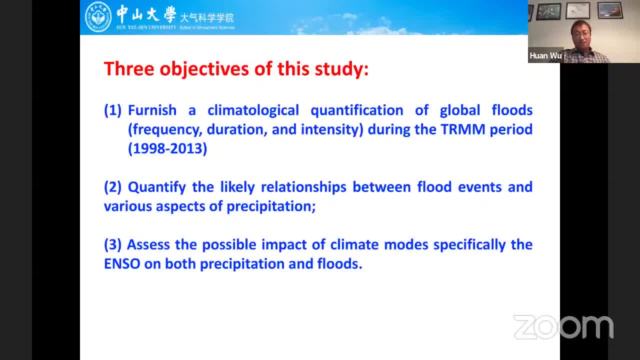 So the object of this study is, to the first, that we furnished a climate college qualification of global floods and from the model simulations, and then we couldn't find the likely relationships between floods and precipitation. And then the further state: we further look into the possible impact of the climate. 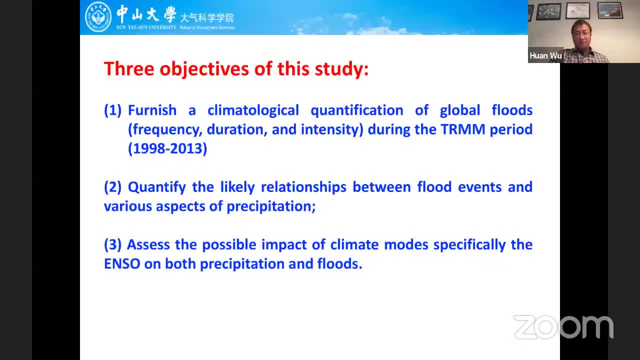 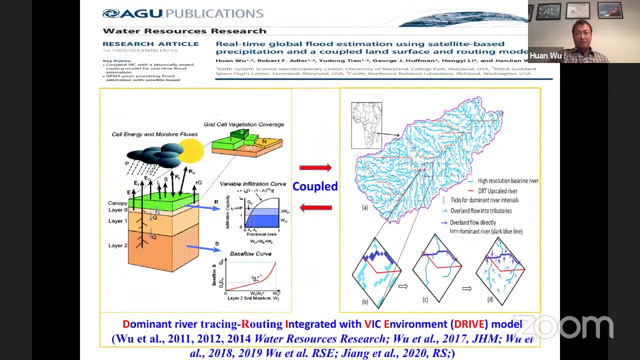 Specifically here, the end zone for the both precipitation and the flood. So then the next step: once we have the better understanding this, we can use this kind of information for, for the data, for the prediction at the various time scales, The model for this study. we use a model called the dry model, and I don't go to the more. 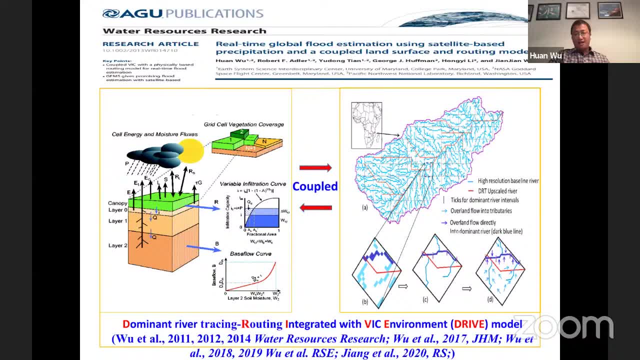 details here and this is a pretty similar as the growth us. we use the land surface model coupled with a rod model and this model has been applied globally and for years and validated, use a lot of ground observations and remote sensing and in the comparison with the other models, etc. 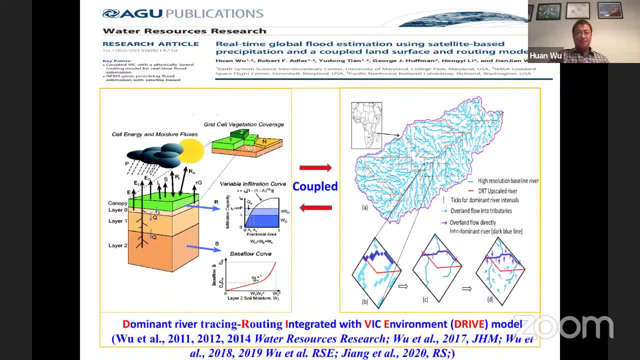 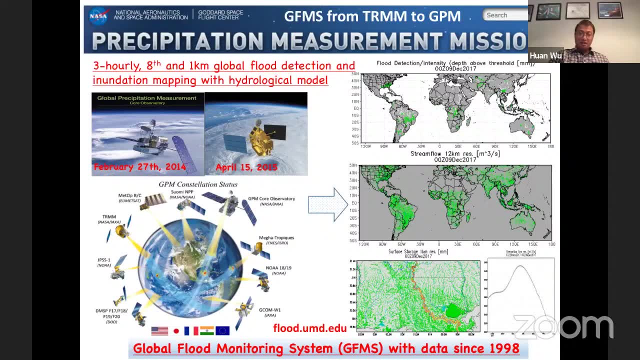 So one interest can look into this paper, and now I'm not going to that detail, I use a dry model. we developed the global flood monitoring system, the GFMS, running a nearly real-timely three-hour one s degree resolution globally and meanwhile, and there are also a one kilometer resolution, global stream flow simulation. 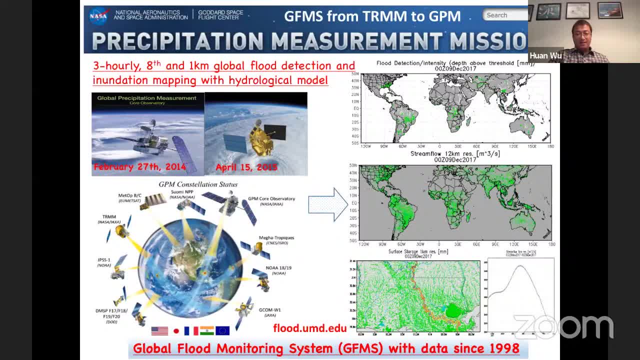 at the same time step. So the system has archived more than 20 years data since 2019 to the 98 and with this, basically for this study. we use the data from such system by using a better quality quality precipitation, with the ground data adjusted to the tmpa, which could drive the 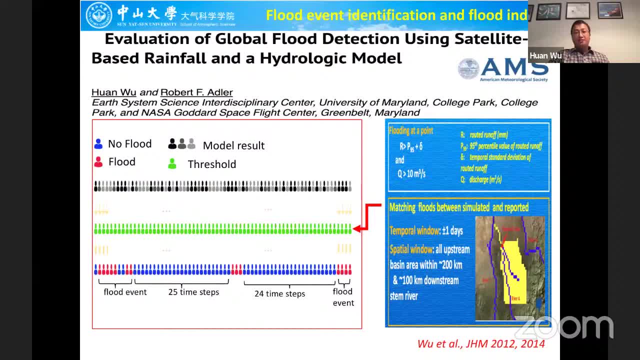 model for the 20 years and then we use every time steps data. we define the flood events. we developed the methods like the right side here. basically, we use a threshold map using the equations like the threshold defined as the 95 percentile plus stem deviation, and with the stream flow. 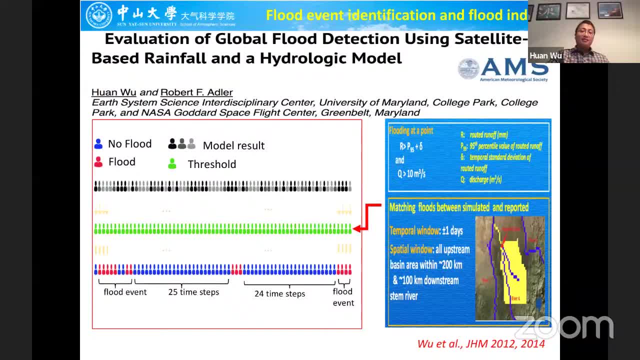 For a concentration, etc. and then apply this threshold map to each grid, cells, time series, basically putting the model simulations and compared to the threshold map which is screen, and come out to the flood events and and basically they will give you the flood indices which are for here, flood frequency and the flood duration and the further intensities. 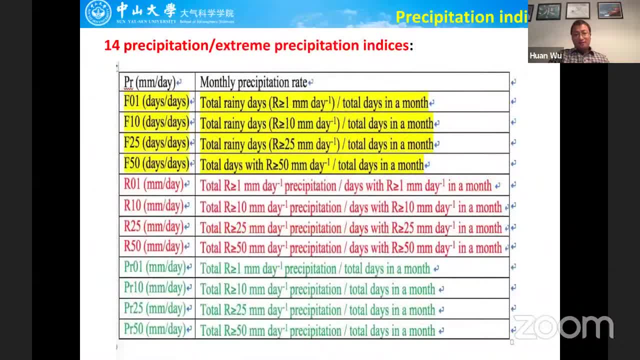 We look at this for flood indices, the their relation to the precipitation indices. four of them are the same by you are in the previous slide slides here. there are more others, but they are basically falling into three categories of frequency and the intensity and the amount, but defined at a different threshold. So I'm going to share some results here. 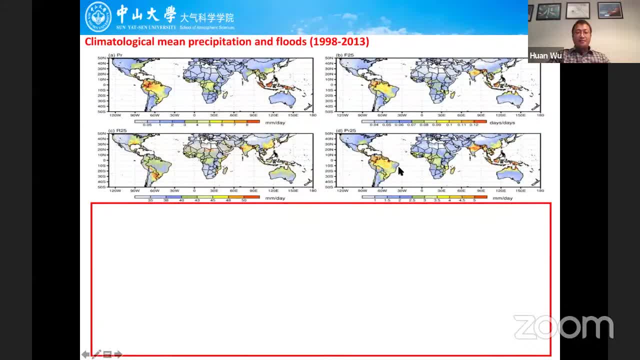 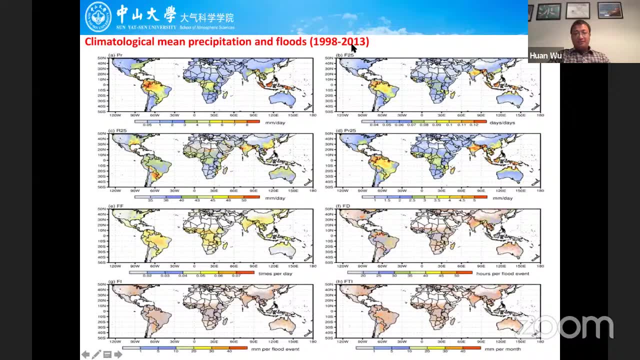 so the top panels you are seeing before and now, we connecting them to the flood. So from this, which is actually 16 years- simulation results and we aggregate it by the by average at the monthly climatology and then we can see here the flood frequency. almost all of these flood indices basically follows the precipitation's. 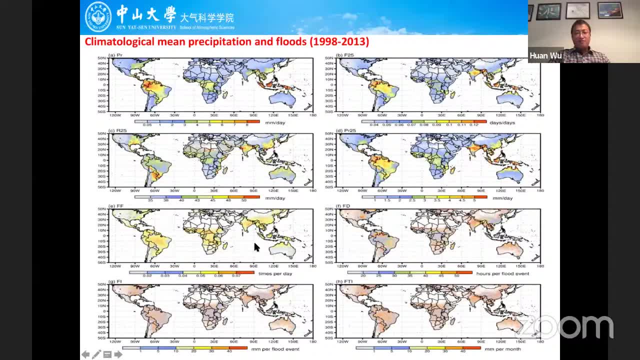 distributions. but flood frequency follows a beta to the precipitation amount and the frequency and the PRR25 here with those high values, basically approximately the same at the same locations in many places. but the other three indices shows a more fragmented spatial patterns, which is not surprisingly because they seem to also not only response. 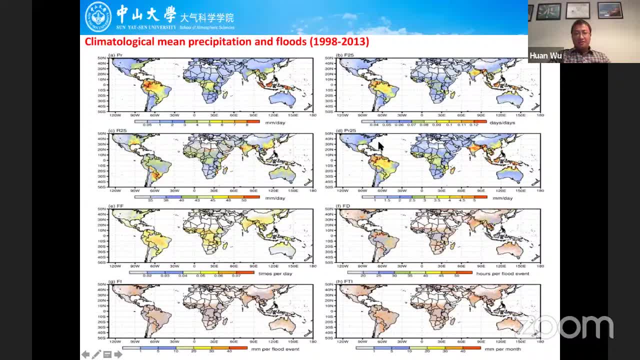 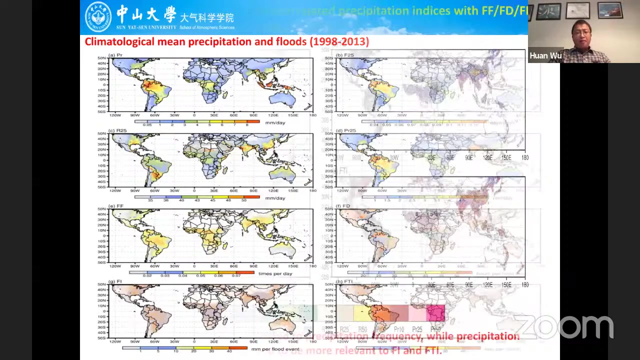 to the precipitation frequency and the amount, but also the response to the intensity of the precipitation, for example, the South American. here I cannot get my mouse, but it did not show the peak on the frequency, but the flood intensity shows a more clear picture. and when we look, 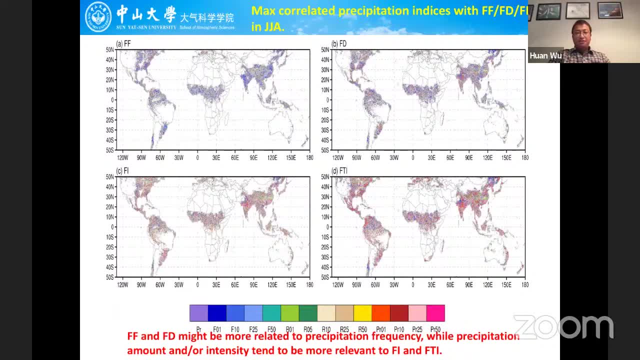 at the max correct precipitation indices with the flood indices for all of these four precipitation indices. here, and this map shows, there are more, even more fragmented distribution distribution indices here. and this map shows there are more, even more fragmented distribution indices here. and this map shows there are more, even more fragmented distribution indices here. 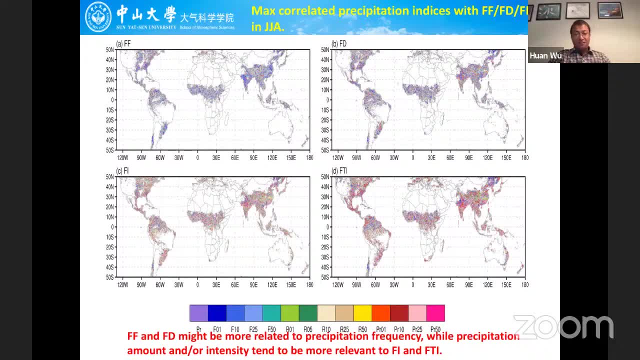 which indicates that the nature of the incongruity of the our work and that, however, we can see clearly collectively, there are some patterns here and we see more of the blue colors, which is the precipitation frequency, are more relevant to the flood frequency and the further duration. 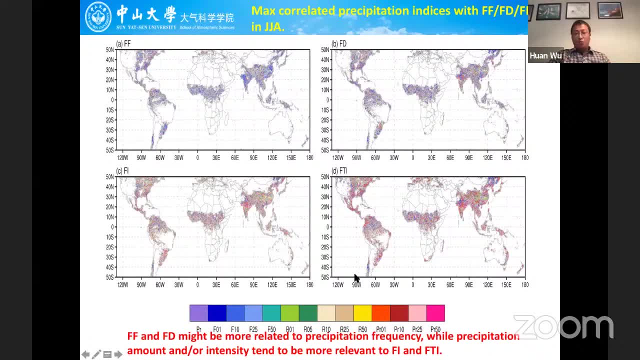 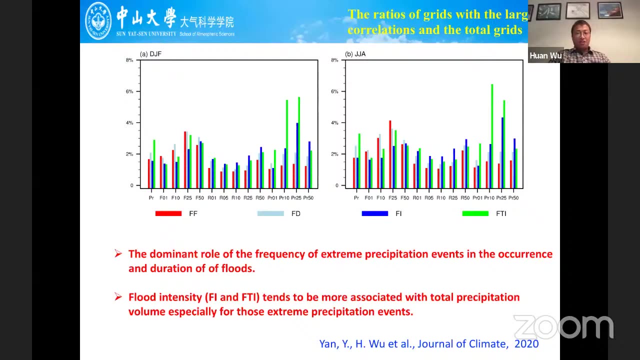 but for the flood intensity you can see a more the more the warmer colors, which is red, and it indicates the flood intensity. comes into play a more important rule here: if you look at this statistically, you can even see more clearly that the dominant rule of the frequency of this extreme precipitation events is is 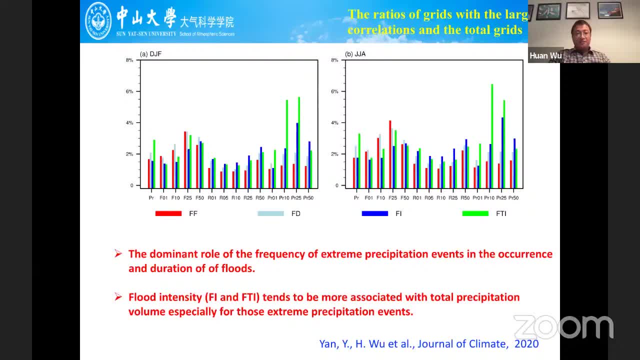 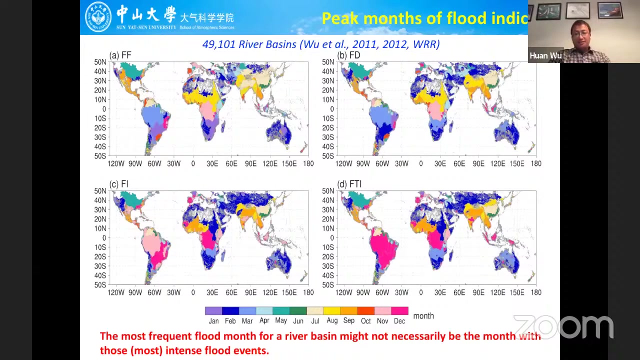 more important for the flood frequency and duration, but the flood intensity is more important, but the intensity tends to be more associated to, associated with the total precipitation which you can see here, this green characteristics of the green and and duckbill biosphere. and then, uh, we, we took a further step to look at this indices length at the beta scale actually. 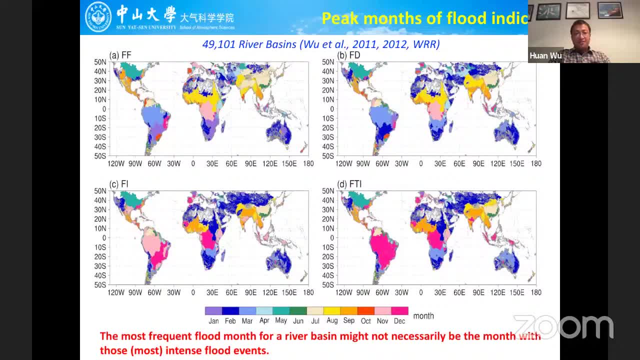 usually we do the flood forecasting at the base scale. so what do you see here? the peak of the flood indices shows clearly that annual preferred flood occurrence time for each individual basins And one can look into those areas that you are interested And we can see this flood frequency and flood duration. 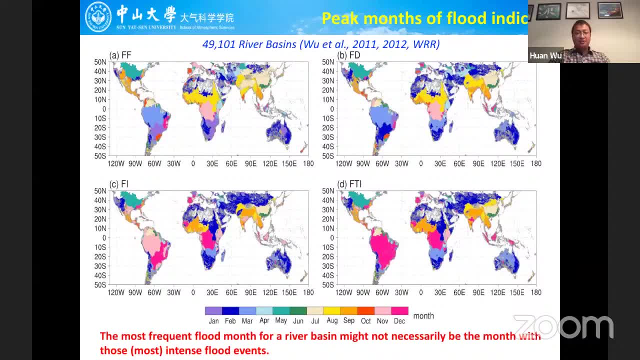 Again, this is a similar patterns with a similar peak time, but they are different from the flood intensity peak months, which is very important for the flood risk and the water resources management, because there's a different strategy would need to be adjusted for this kind of information. 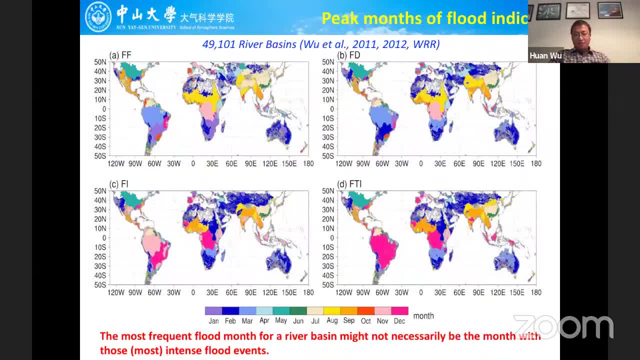 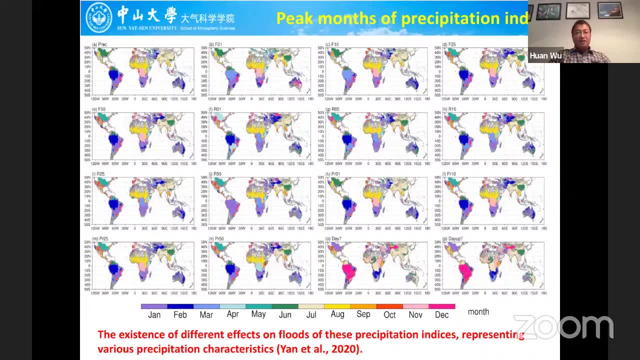 And when you compare this flood peaks to the precipitation over this flood precipitation indexes that you can see floods are usually consistent with precipitation special structures but we can still see some of the river basins have like a one month ahead of the peak. They are different. 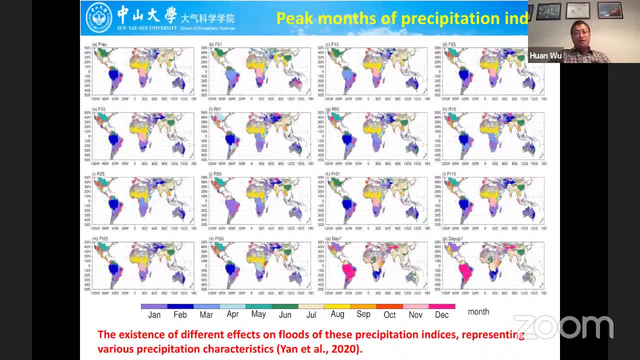 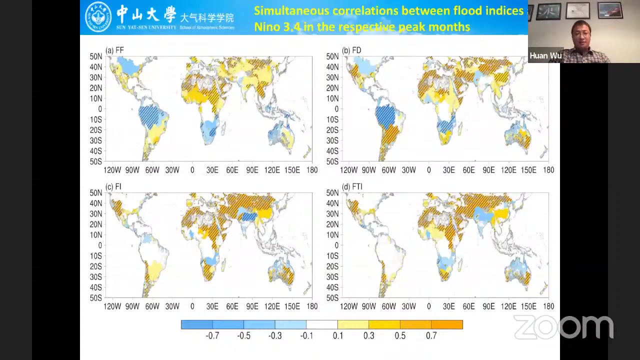 but this is the difference between the flood indices and the precipitation indices and the differences between this precipitation indices- We have the same kind of and then, importantly, we trying to look at this indices led to the answer: the simultaneous curation between flood indices. 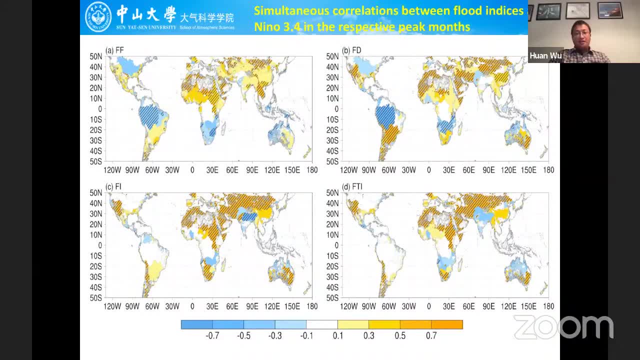 and the answers over this, respective indexes. So we can see that, for example, in the third index we find a. currently the rate of precipitation, the ratio is 60,000.. And then if you just look at the anche instead of the tide index, it is so much faster. 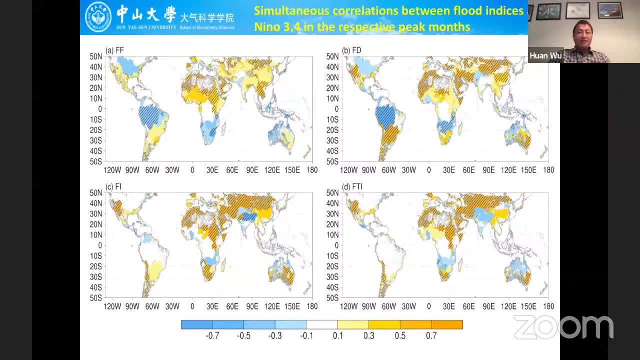 peak months of the flood indices and we can clearly say that flood frequency and flood duration has a significant positive and negative correlations with the answers and we can even say the flood duration has even a stronger link to the answer in many areas and because of time I want to point out all of them, but you can clearly see those stronger colors and which is 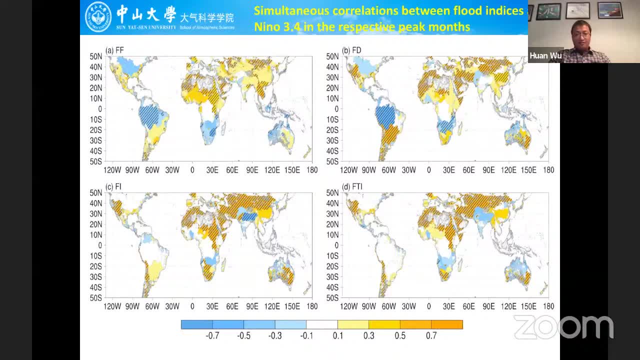 consistent with previous studies by Philip Ward using a different model and data. and when you look at the flood intensity, they also show different patterns with flood frequency. but a clear pattern here is that in a north area in the north, to the 20 degree north, they are. 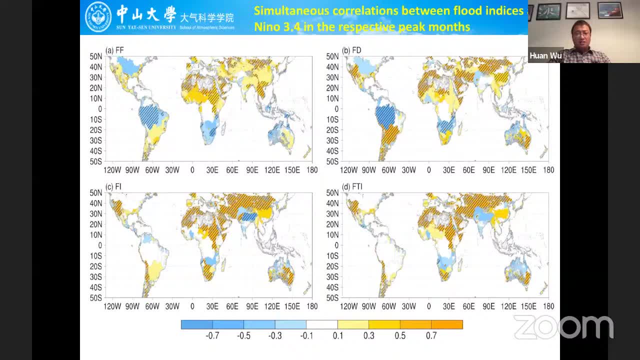 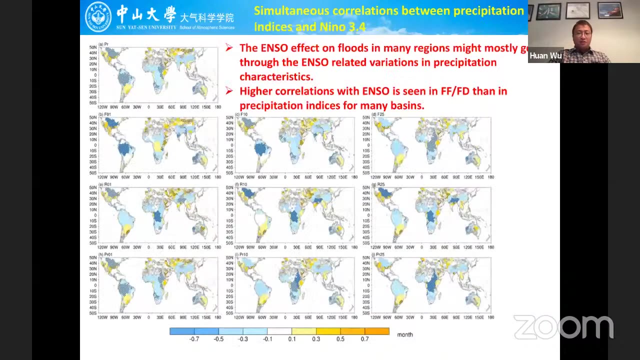 you know, even stronger intensity linked to the answer, which is: I think this information is very important for the flood forecast and again we compare to the precipitation here. the answer links to this precipitation indices and also clearly shows that the answer in fact actually is higher. So 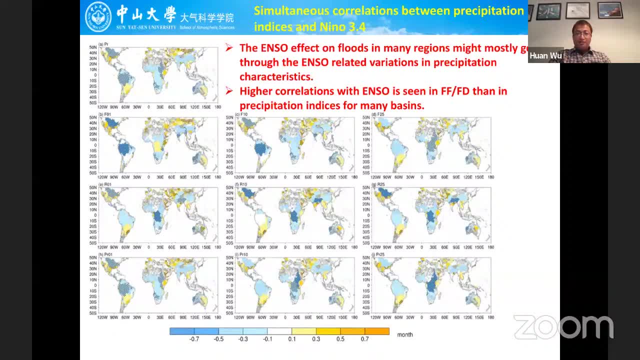 we can see that the rain, the rainfall and the soil are relatively lower and this is to compare the🎁, the rainfall between the summer and the fall to find that actual answers for the print is stronger at the flood. that can be explained. 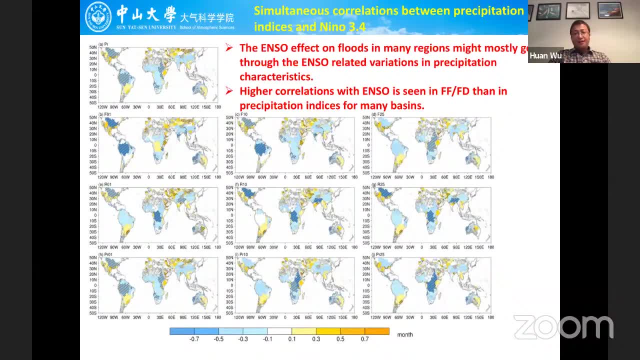 that the streamflow can be a better indicator of the water cycle of a real bedding scale, And it might also the answer can moderate to other important variables, which affects the floods too. which one for the studies? but these are very good news to say. 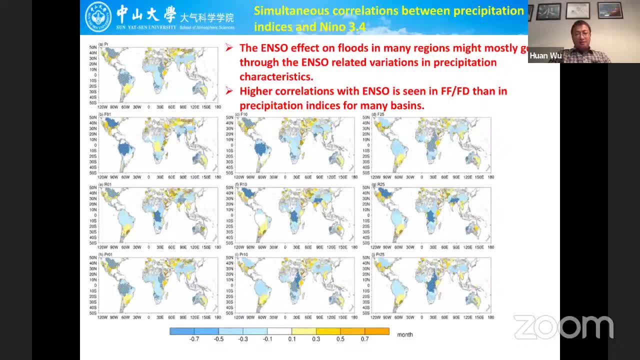 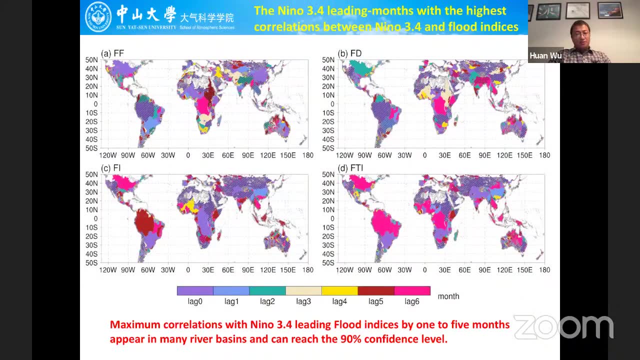 that the ENSO affects the floods through precipitation And, even more important to that we are looking at when we map out the ENSO's leading months with highest correlation between the ENSO and the flood indexes. so we can clearly say: 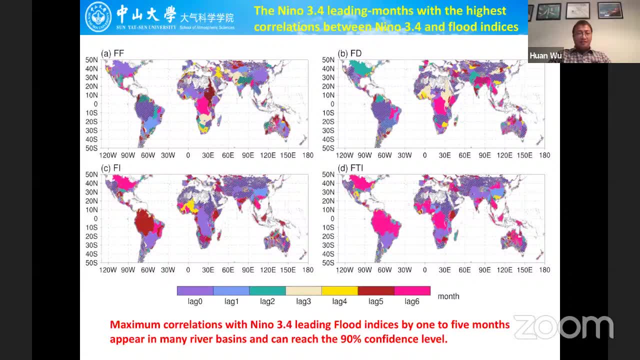 there are a lot of differences and we can say this ENSO: lead months can be one to five months ahead of the floods and the significant relations there And even some simultaneous correlation peaks at peaks shows in some of the real basin, but they mean one to five months ahead of the floods. 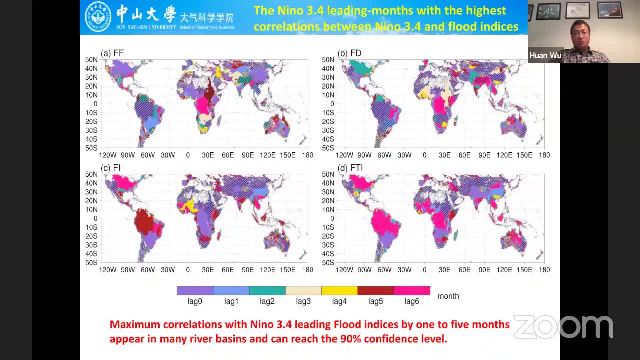 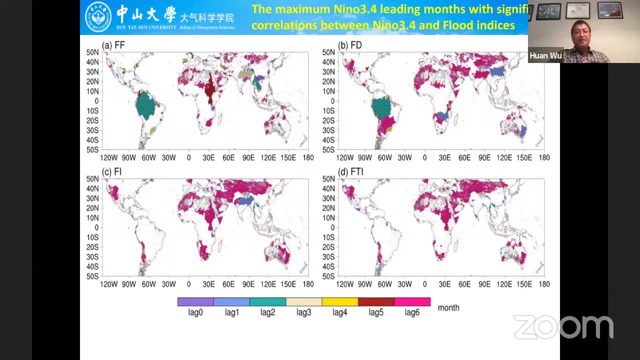 So that's why the significant correlation can still hold for a few ENSO lead months, which is as shown in this slide here, And this is another very good news. That means we can use more of this kind of information continuously for a few months into the future. 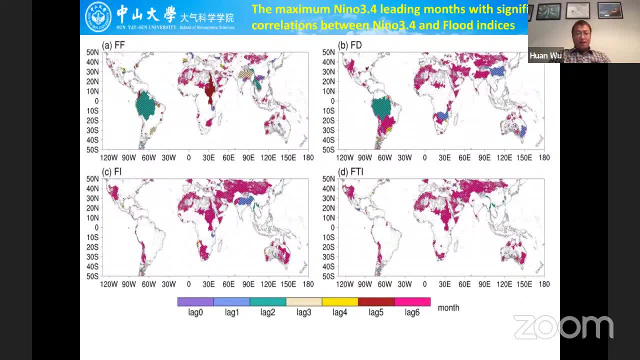 for the flood assessment forecasts. We don't have the time to look into one-to-one comparison, but I will encourage you, if you have one interest, that can look into these figures. you just play the one-to-one comparison and the flip over. 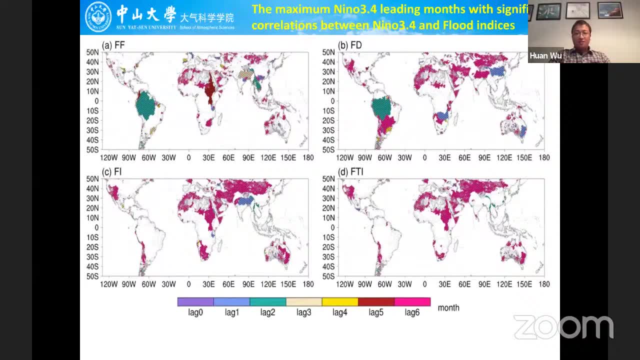 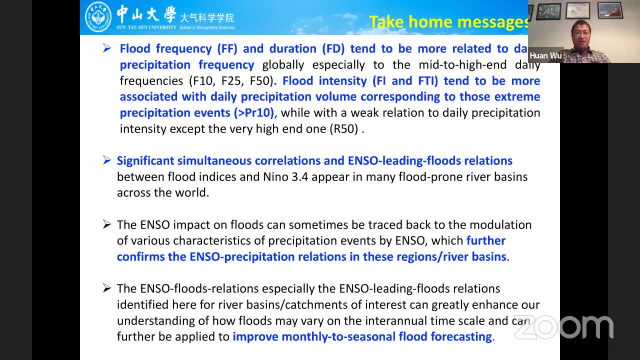 and you can see more interested information in this area too. And here's my taking home messages. I will go really quick. Flood frequency and flood duration tend to be more relaxed to the precipitation frequency. Intensity tends to be associated with daily precipitation volume. 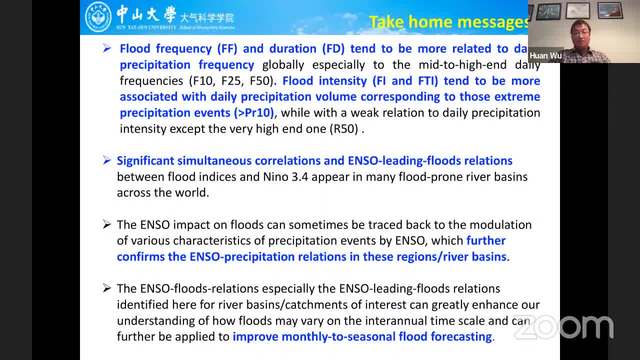 corresponding to this extreme precipitation events, particularly the precipitation larger than 10 millimeter And the significant simultaneous and ENSO leading floods, relations are found in many of the real basins, which is very useful, And I think that's all what I'm going to share. 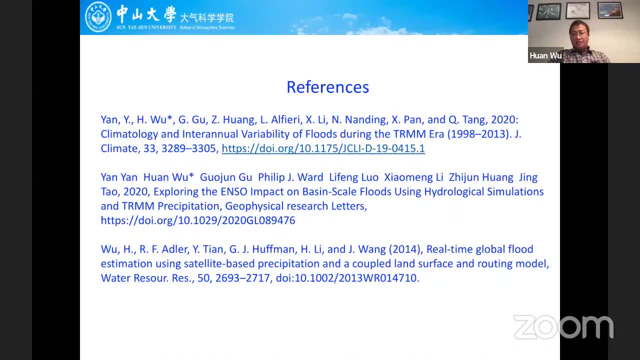 And for more details, I would point basically to these three papers and for more details. Thank you very much. That's all that I have And I would be glad to have any questions. Thank you so much, Juan. Thank you for the presentation. 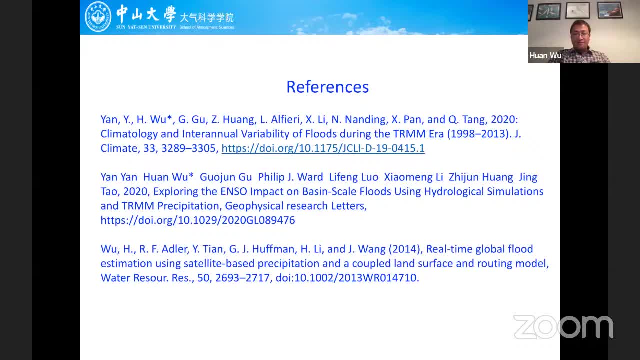 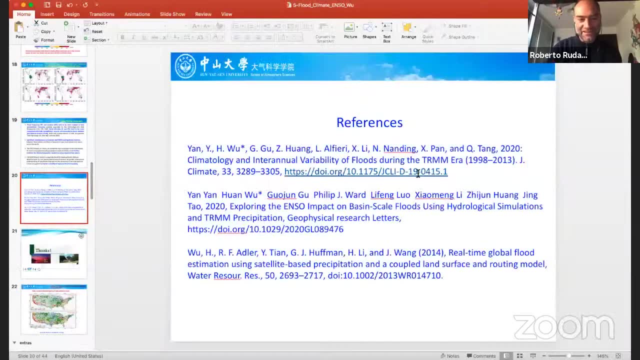 I think I mean we can fast moving forward. I mean to the last presenter today, that is, Kei Yoshimura, from the University of Tokyo, talking about the predictability of the floods caused by typhoon like this in 2019, using today's Earth. 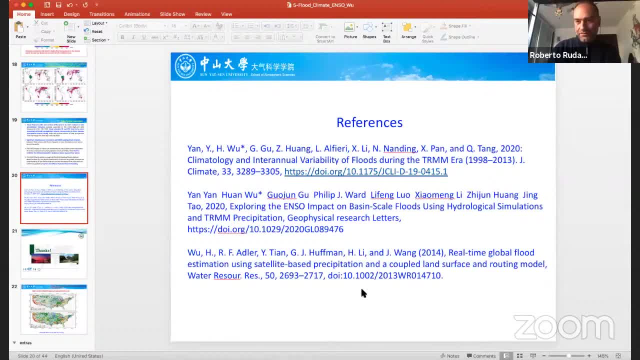 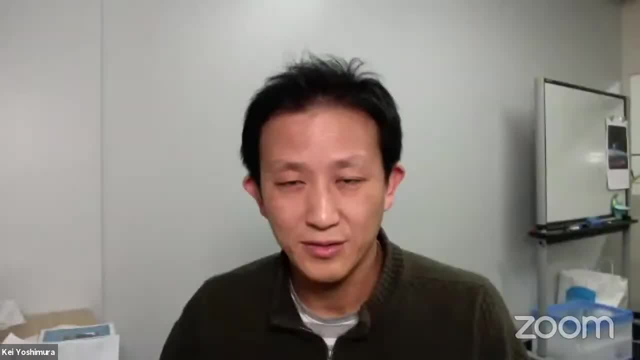 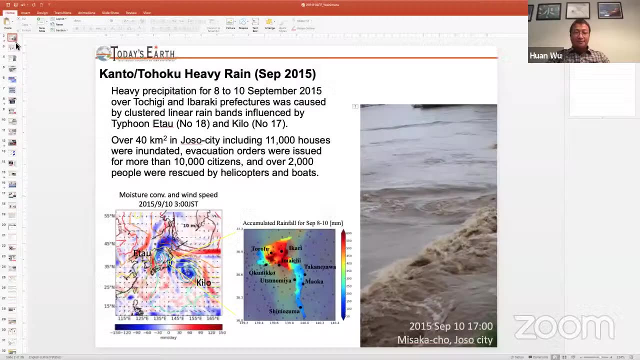 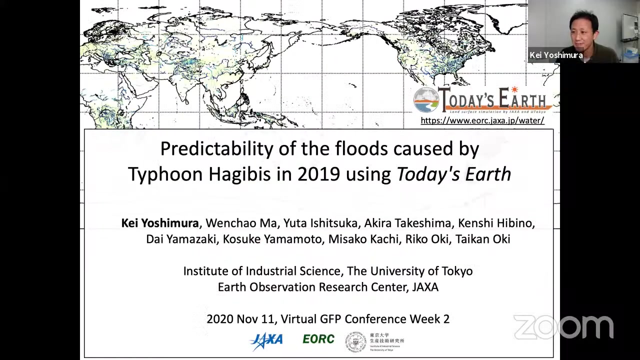 Kei, we are looking forward to your presentation. I mean, if you would like to try and steal the screen to Juan Juan, can you? Yes, I did Okay, Perfect, Okay, Hi everyone, Good evening. Actually, it is now 1230 in the midnight in Japan. 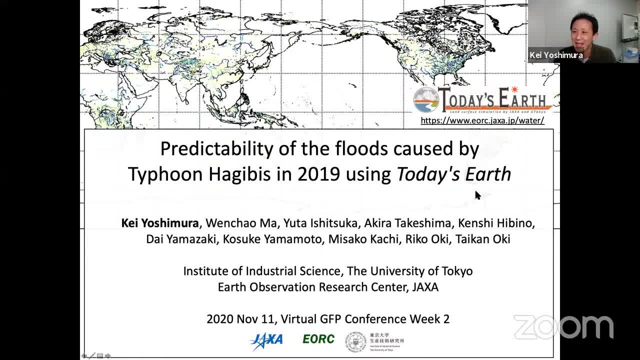 So it's kind of harsh timing, But my name is Kei Yoshimura from Japan University of Tokyo, And I'd like to present on the predictability of the floods caused by typhoon Hagibis 2019 using today's Earth. 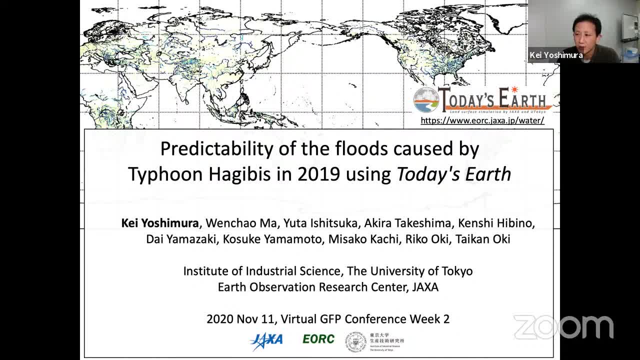 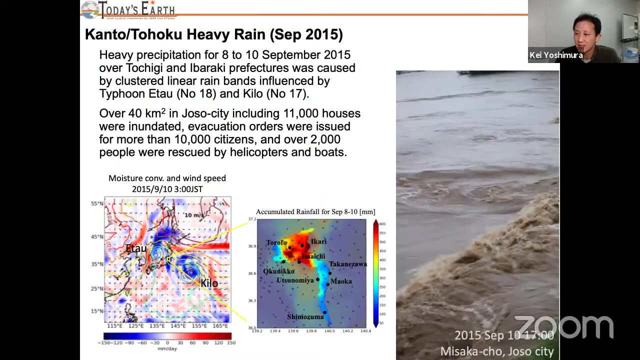 which is our global flood forecasting system, And then there are a number of names here, So these are our collaborators, And also this work is collaboratively done by University of Tokyo and JAXA. So, starting from, I would like to start with some flood events. 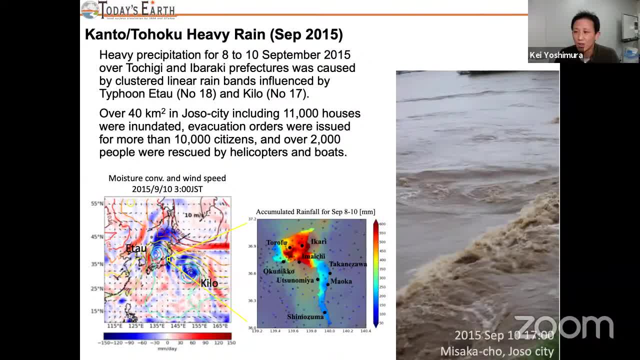 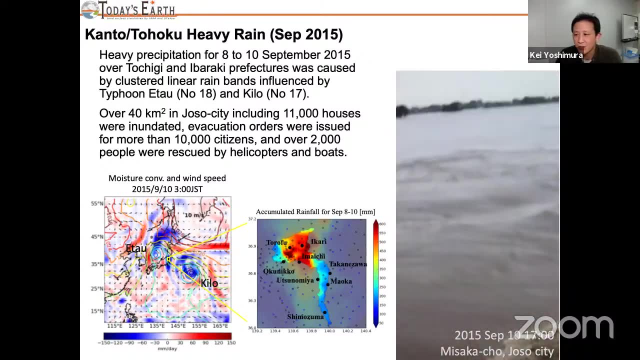 seriously occurred over Japan, So it's starting from 2015 events. So I'm going to start the video, but it has some sounds, So please be minded. So heavy precipitation caused by two typhoons, but actually it's not the direct. 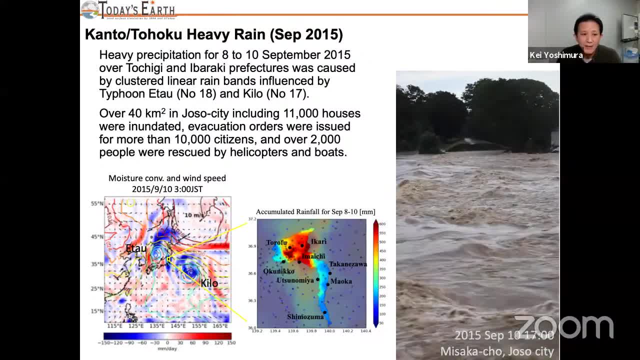 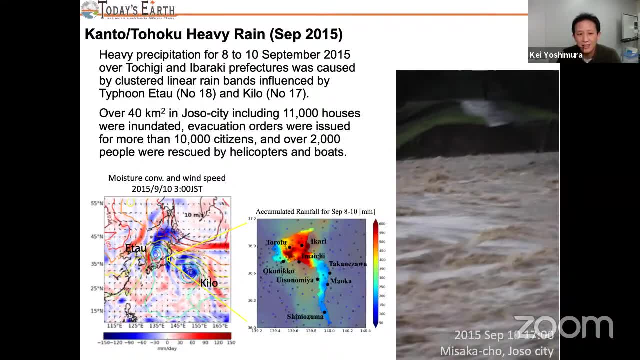 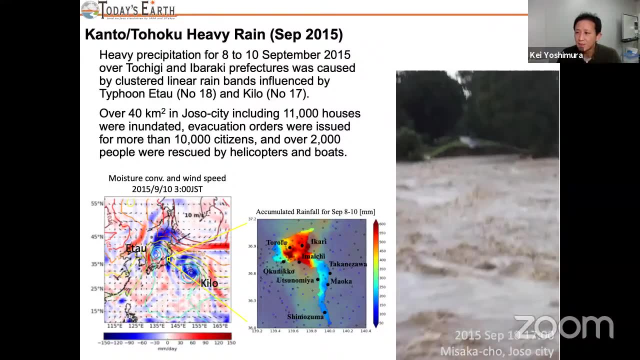 directly caused by the typhoon, but indirect. But as a result, whole city, Joseon city, was inundated And then 10,000 citizens or 11,000 houses were inundated. So actually, it struck me, it was a very shocked moment of my. 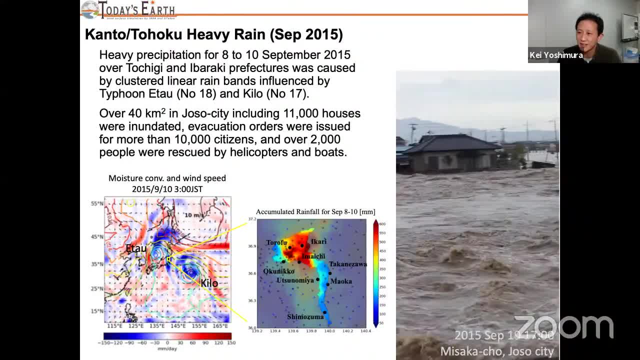 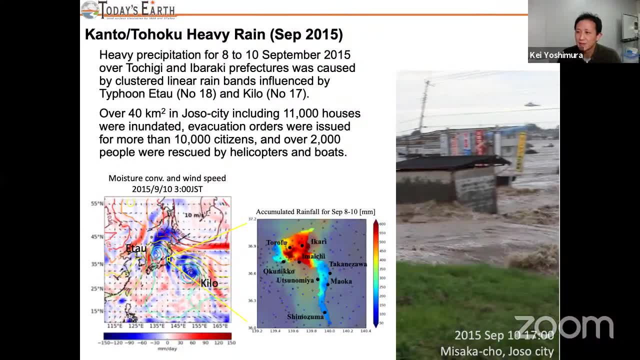 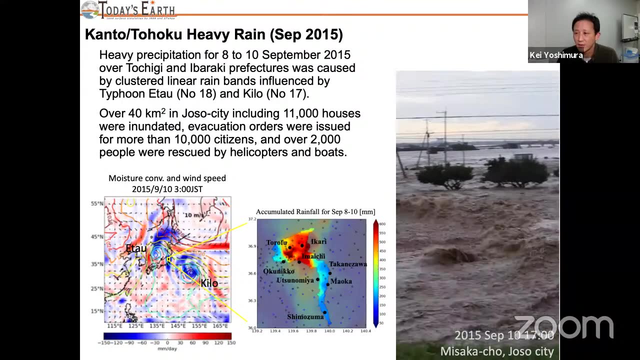 for myself because it's actually quite close to my region And so I was. I didn't realize that it also happens to like urban area area like near Tokyo, So actually it triggered our motivation towards the flood forecasting. So three, three years later, 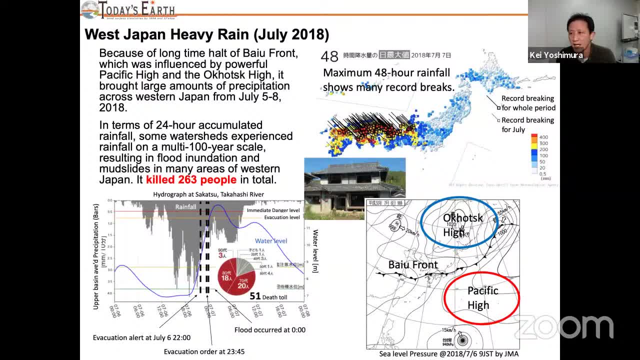 this was on 18.. There was an even more, even worse floods hits occurred in West part of Japan- It is called West Japan heavy rain And then the. it was caused by bio front, So rain land, but it was a 24 accumulated rainfall was all. 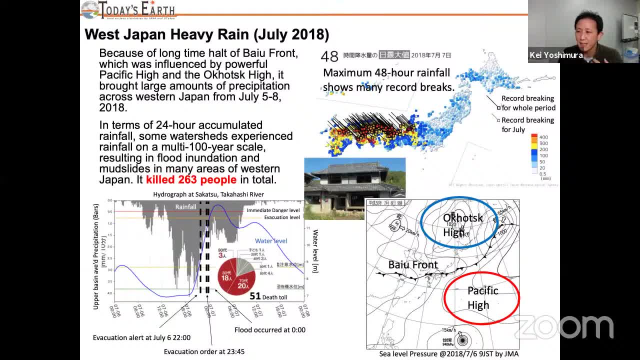 all, very many, many, uh, record breaking rainfall was recorded And then actually it killed more than 200 people. And then the left bottom part: uh, it's a hydrograph at uh uh, one river called Takashi river, at. 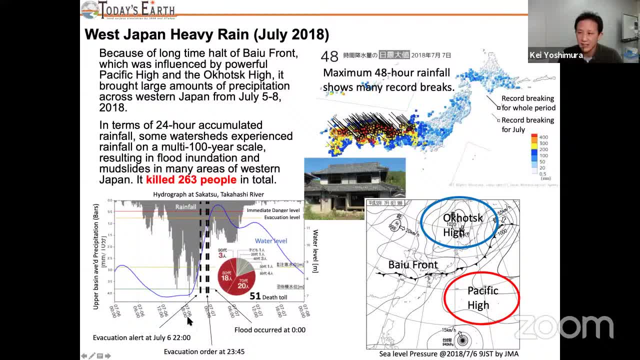 uh, it is only 20, uh, 48 hours, two days in the horizontal access, And so, uh, the hydrograph here with blue line is a very rapid. It's so typically uh that, uh, uh. 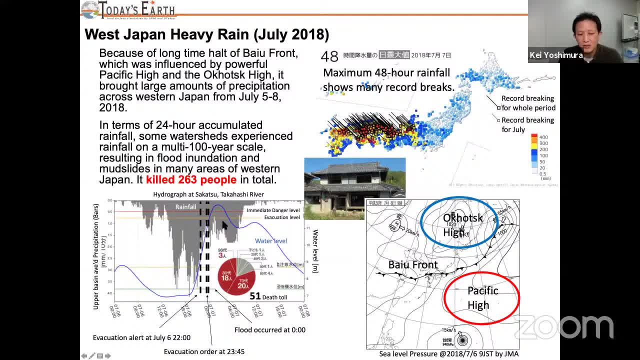 even because of this uh very rapid change of the uh water level, so that uh uh 50 people could not escape from this uh business, Then uh actually uh more striking is uh. 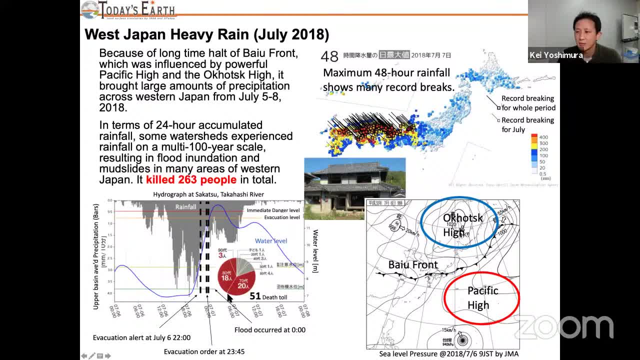 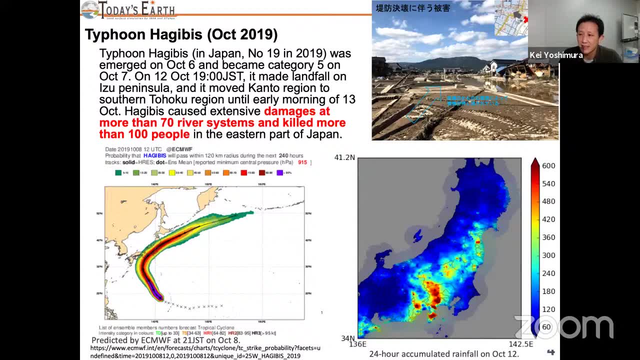 80% of this uh casuality was elderly people who couldn't uh escape even to the uh rooftop of the resident. So, uh, we, we really uh, we do not have enough. we do not have enough water. 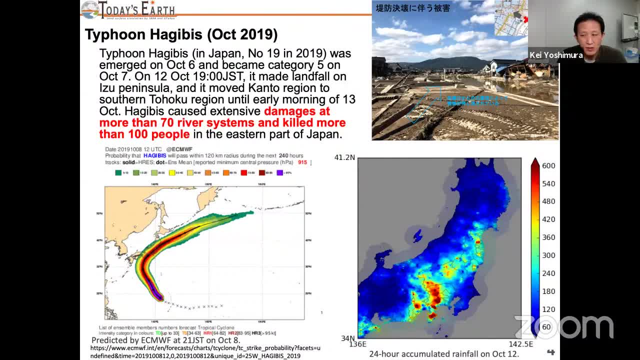 uh water supply. We, we have to do everything in order to uh uh, to uh, uh, uh uh, to to uh, to uh, to to um, to to uh. 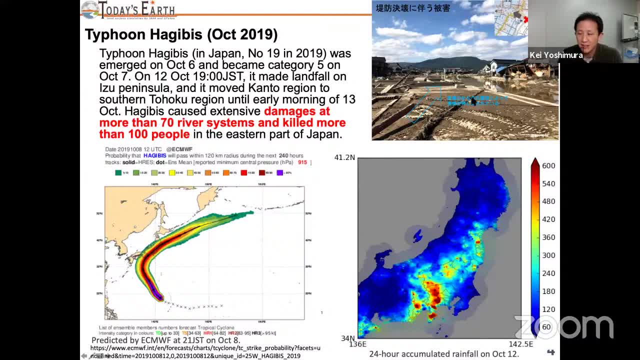 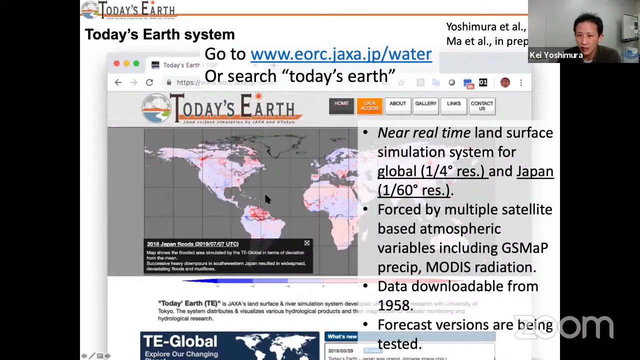 to uh uh damage in the nagano prefecture. but and then, uh, actually what it was unique here was actually this was a ecmwf typhoon prediction, but the ensemble spread was very small, so the predictability of this event meteorologically was quite high. and then actually we created something called today's. 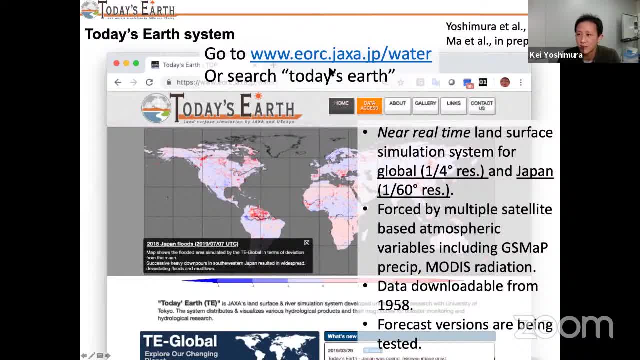 earth. please google today's earth or please click this link if possible, but it's a near real-time land surface simulation system and then globally one fourth degree- and then actually it has a regional version- over japan is 160 degree, which is corresponding to one kilometer. 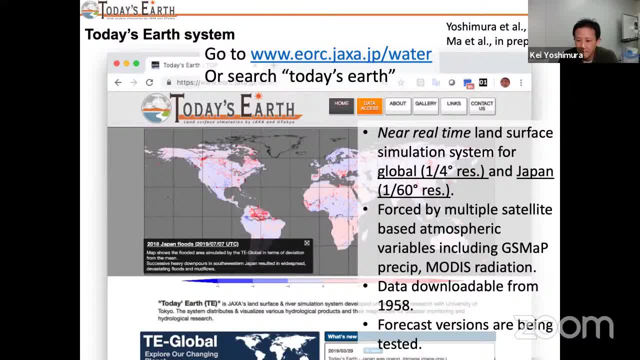 so with exactly the same modeling system, and then uniqueness is forced by a multiple satellite-based atmospheric variables, including gsmap, precipitation or modest radiation, and then it is downloadable. uh up to 1958 standard forecast version is going to be tested, which i'm going to introduce from now. 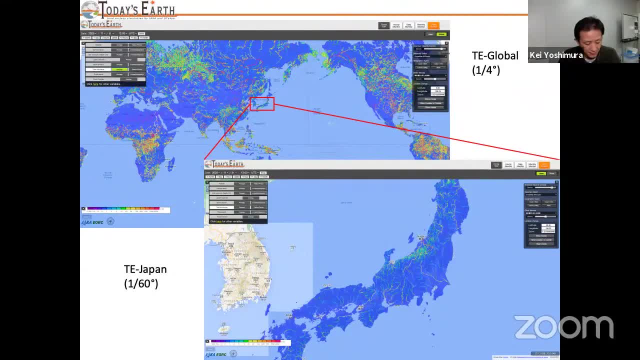 so this is a graphical user interface of the system and then, similarly, it's a uh, similar to the go first or running system. it has a globally- i mean zooming in, zoom out- system and then many variables, not only discharge quantity, geophysical quantities, but also return period of major variables as well, so that uh and then 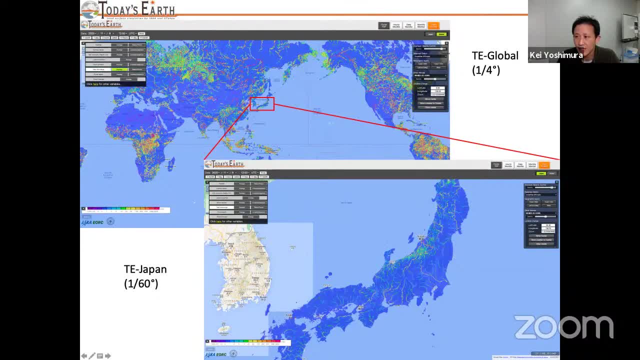 uh, as i said, it does a regional version of the system, which is, uh, the geosynthetic field. uh, so, And so the system is can be ported to any other of the region. So actually, we are planning to extend it to the other, for example, in Indonesia, I mean the South, Southeast Asia or Africa, and so on. 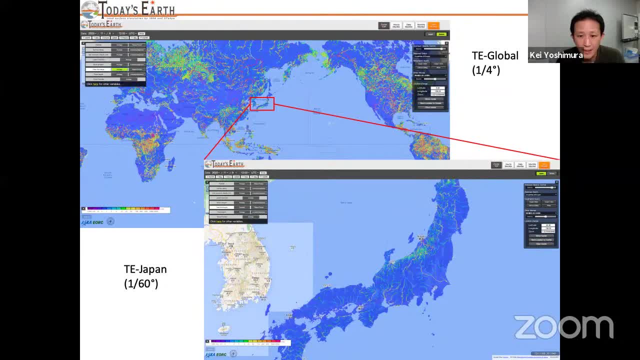 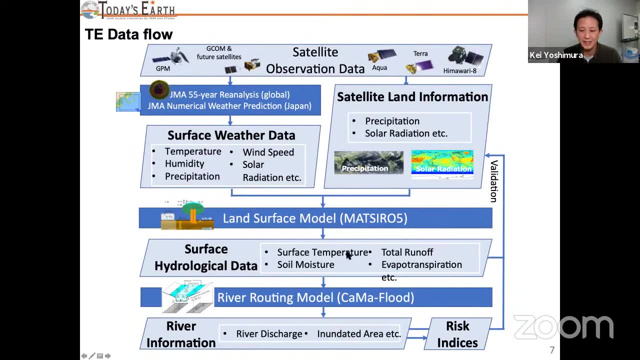 This is the data flow, But because of the time limitation I will skip it. But it has not only physical quantities, but also it has a return period- how rare the values are as well. And then this is a structure of prediction system using today's Earth. 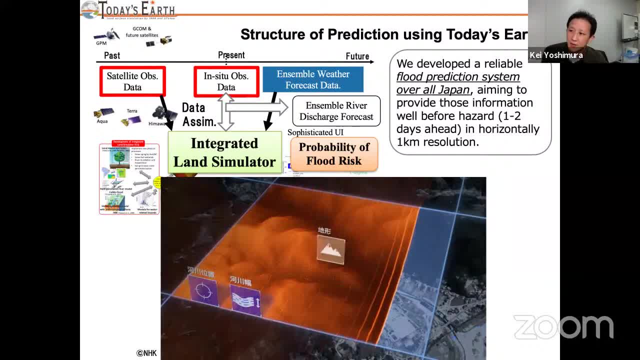 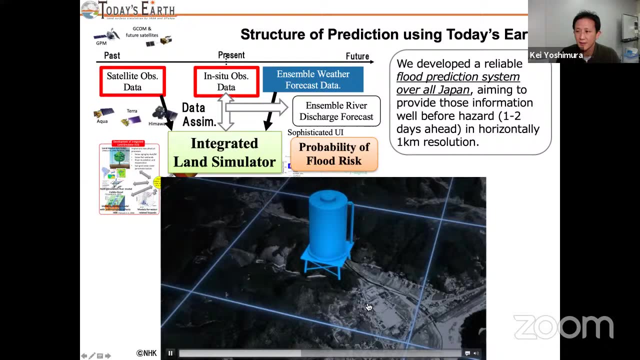 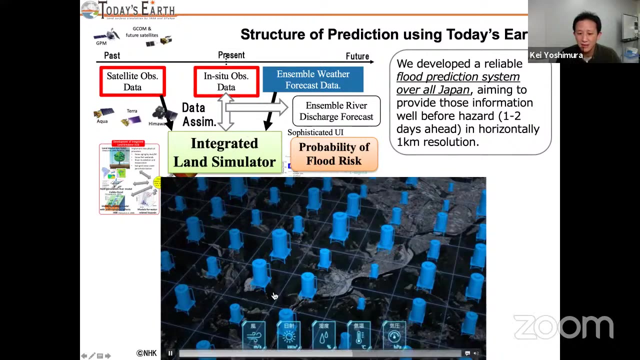 So, as I said, today's Earth is very rare. Today's Earth system is that until near real time, But as you can use it by using using a forecasting, forecasted atmospheric variables we can apply to towards the future. So this is a schematic diagram And then some video is also showing. 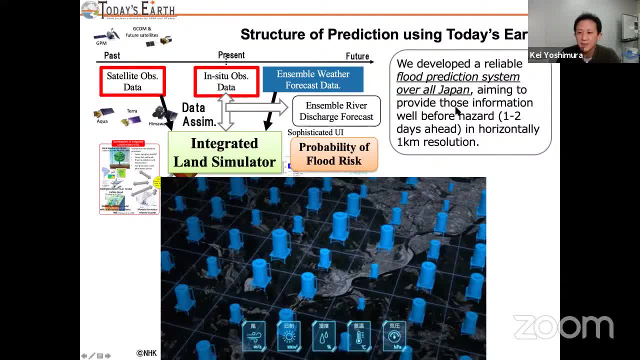 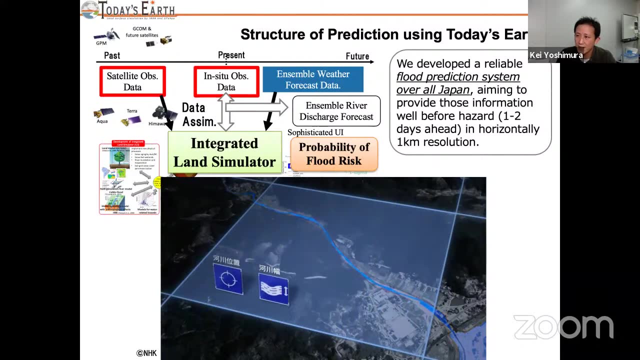 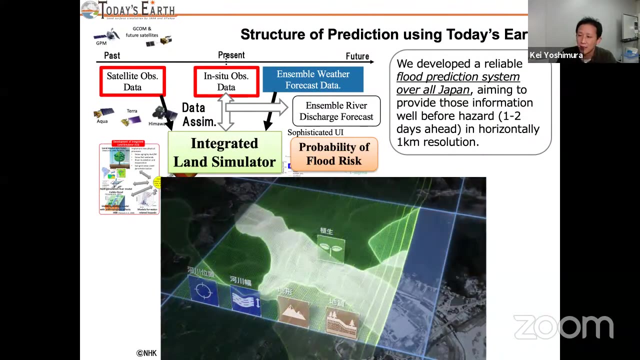 So in Japanese we developed a reliable flood prediction system over all Japan, aiming to provide those information Well before hazard. So I mean it is relatively shorter, I mean one to two days, But actually for Japan I mean it fits because because of short and smaller business size over in total. 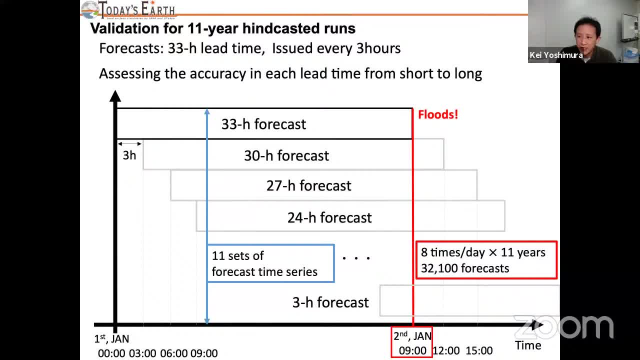 And then we were moving on to the case studies. But I would like to introduce general performance of the system. So We kind of cast it for 11 years by using that system And then every three hours we forecasted. it forecasted 33 hours. 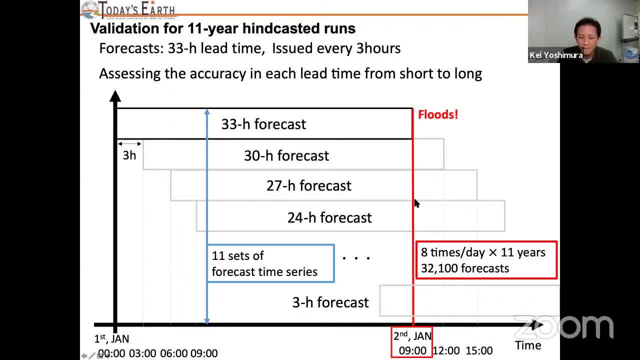 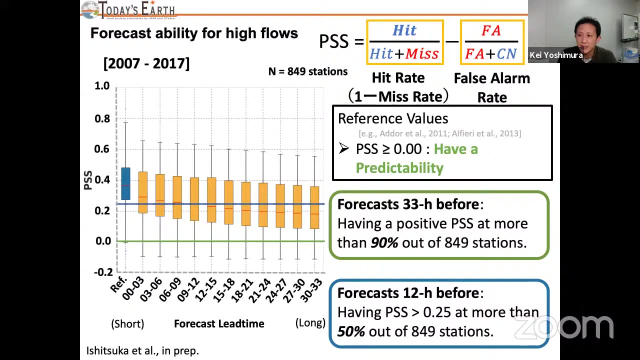 So that every- I mean every three hours, we have 11 sets of forecasting time series. So, and then we assess the accuracy in each lead time, So how the performance is degrading as the lead time longer, As a longer lead time. And then we use PSS. 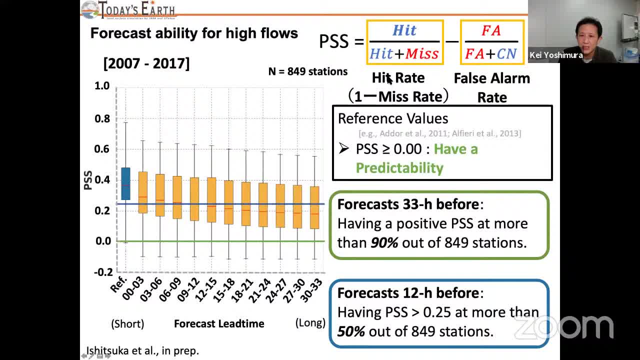 pure skill score to express the performance, which is consists of the heat rate minus false alarm rate, And using 850 water level measuring stations over Japan. As I said, it is 11 year hindcasted experiments And then. So horizontal axis is forecasting lead time. 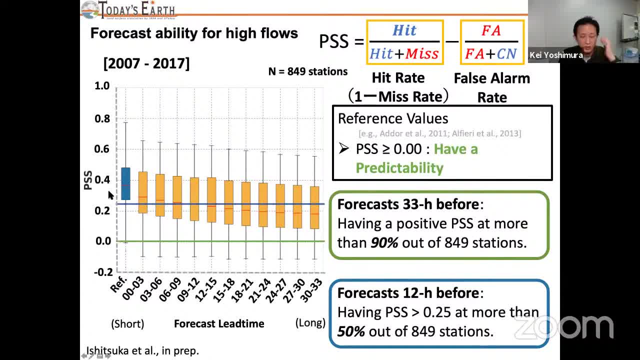 And then the vertical axis is a scope skill score, And then zero reference is when we use- I mean, it's a zero analysis- So using observed, observed atmospheric forcing, And then try to simulate the discharge. So it's a kind of a maximum scale of our system. 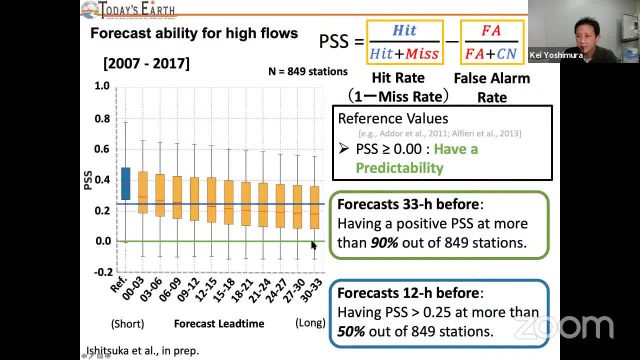 And 80 degrees over time. And then reference value is how our interprets The PSS is a positive value. How about predictability? And then 0.25. It means a good predictability. So for us to focus 33 hours before. 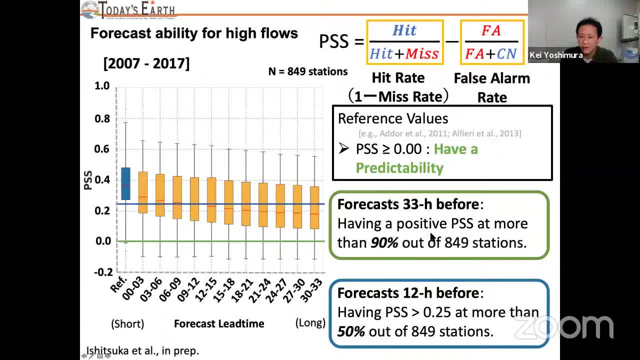 It shows having positive PSS at more than 90,- 90% out of 850 stations, And then 12 hours before, So 0.25.. So it means a good predictability. So of course I we are not satisfied with this performance. 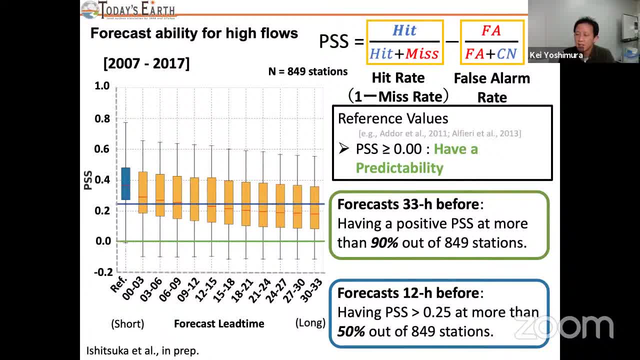 And then there is lots of room to be improved. However, by showing such kind of Performance or the evaluation, Then user can choose. Depends on the purpose How Those kinds of information can be utilized for that purpose. So let's move on to. 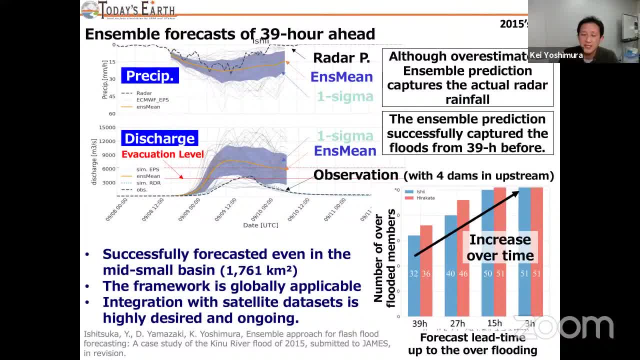 The 2015 case And the 2018, 2019 case, So 2009,- 15.. It was actually Simulated After the event, So ensemble forecast was tested And then the Top one is a precipitation. 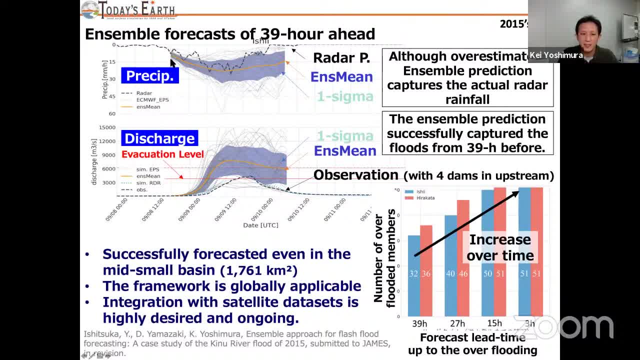 So there is an ensemble spread from the Particular initial condition And then, depending on this presentation, the discharge is simulated And then there is a large Variance of the ensemble member. However, what it is showing here is we can quantify how 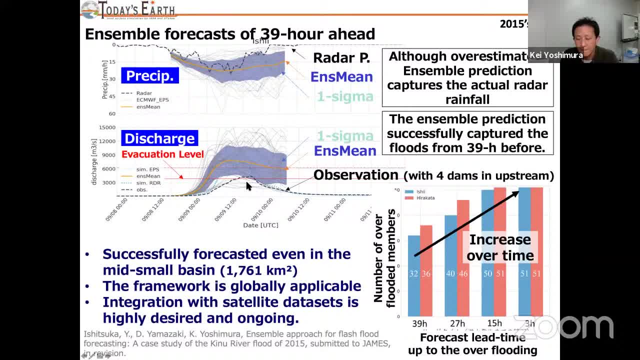 How dangerous the situations are. So we set the specials And I mean this is You got it as evacuation level, But By showing the bottom Right figure, 39 hours before 36, ensemble member Out of 50.. 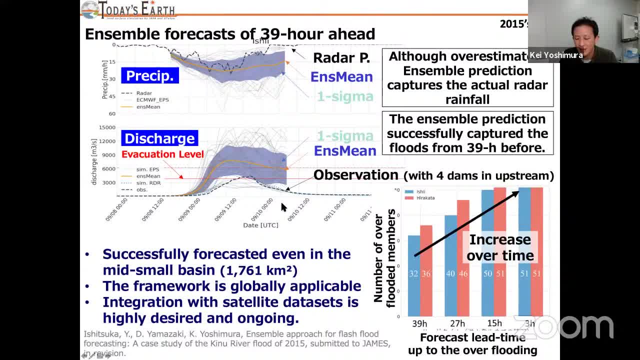 Shows More than the Flooded, Flooded Or alert. But That rate increases over time. So 15 hours before the Actual Disaster, Almost a hundred percent Of the members Showing the sign of Flats. 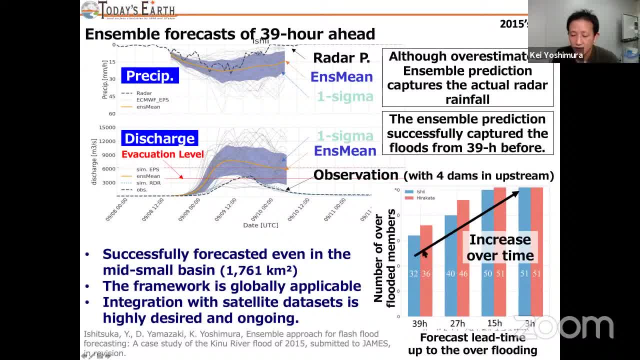 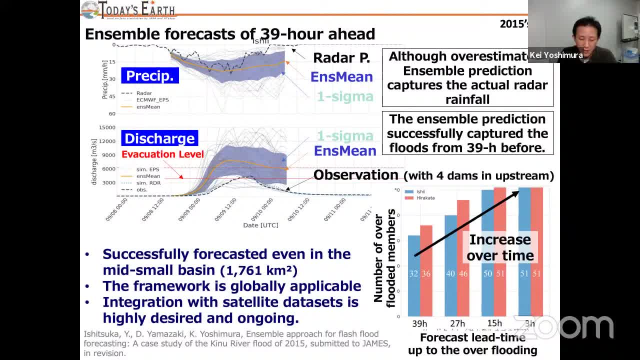 here We see a A sharp boost from obscene. There's a lot going on here We can see like on the dominant Lead Basically. so sil billing So they Are On the Middle Size of isn't Only exceeding. 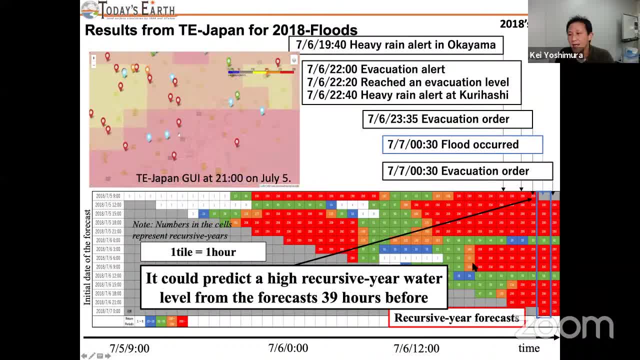 1000 square kilometers. So it is, and then showing a red is an alert, but compared to the real situation, occurred only three hours before. actually there was alerts from the government, but it can be extended towards more than 24 hours possibly. 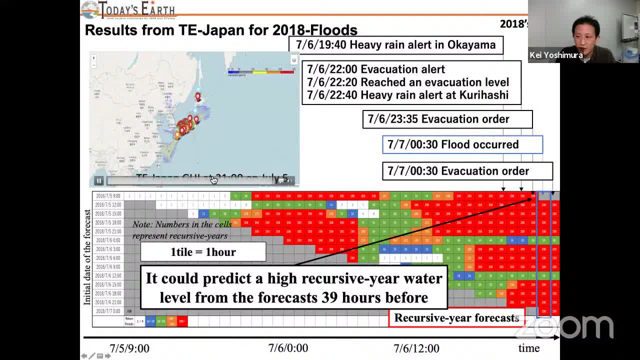 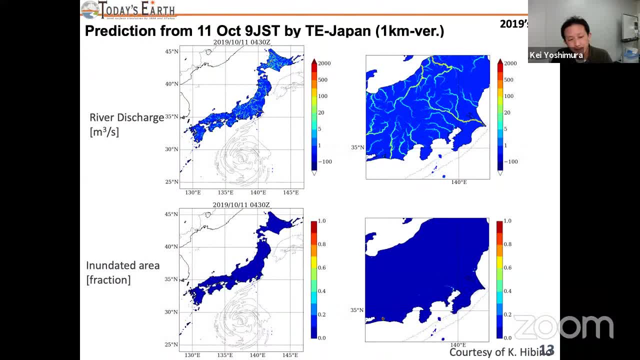 So this is an example in 2018.. And then, moving on to just last year, actually this figure, this illustration was used when the actual disaster was happening, So exactly the same figure is shown here. So as typhoon approaches, the river discharge amount is increased. 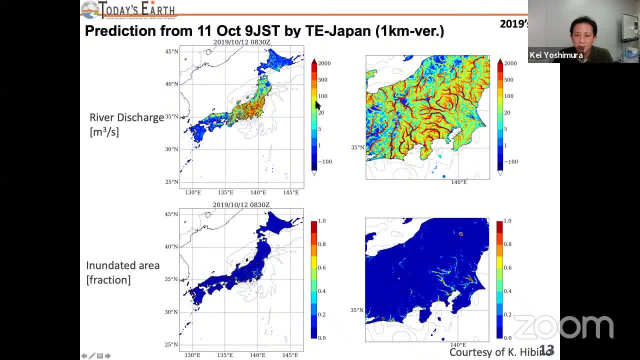 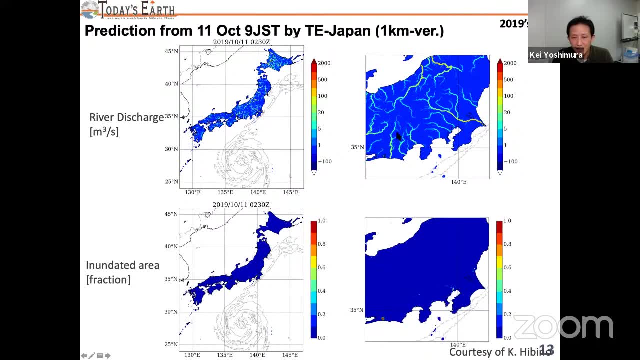 going tons into green, yellow or orange and then it goes up And then it goes down to orange like a blood vessels. But that level of water discharge- I mean river discharge- is we cannot convert it to the danger level directly. 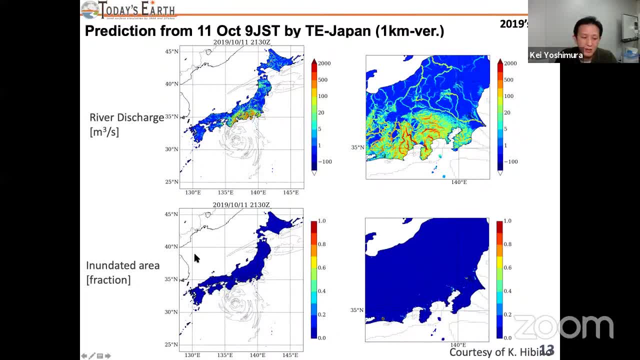 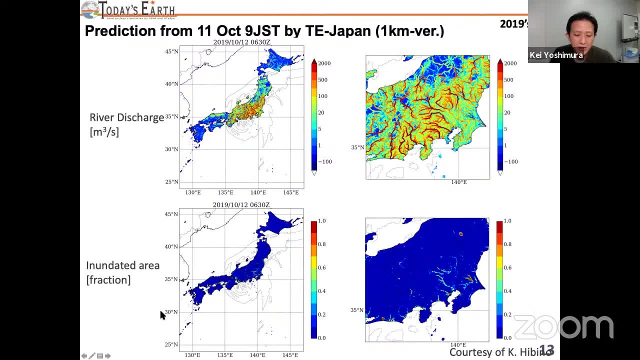 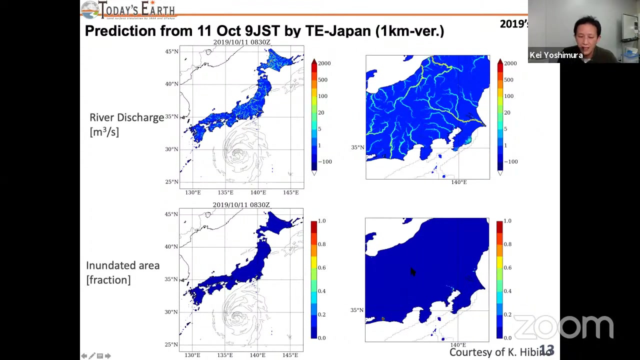 because there are big rivers or small rivers. So we also simulate inundated area by using the K-Math Lab model. So K-Math Lab is able to simulate inundation, inundated fraction. So inundated fraction is actually more fair indicator of the flood. 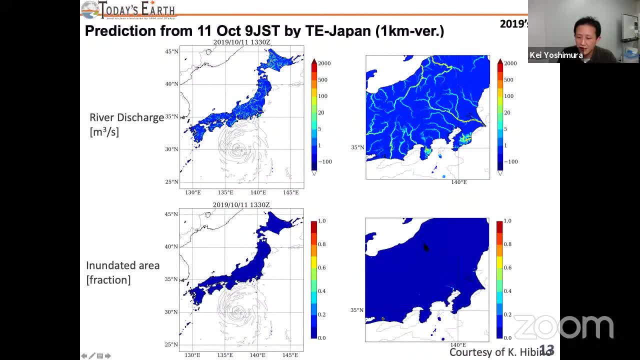 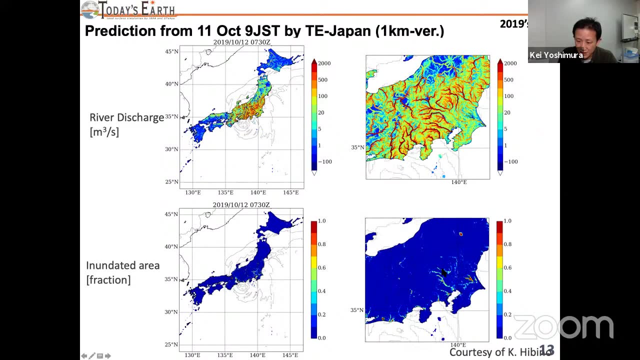 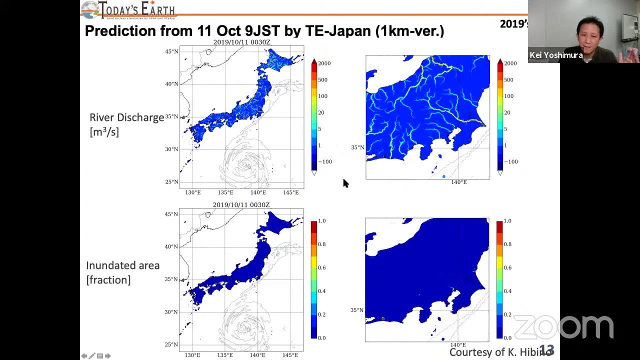 So from totally violet blue color in the beginning but it suddenly turns into, you know, red in the many places. So it indicates, indicated danger of the danger for those area which was predicted day before what is happening. And then it turned out. 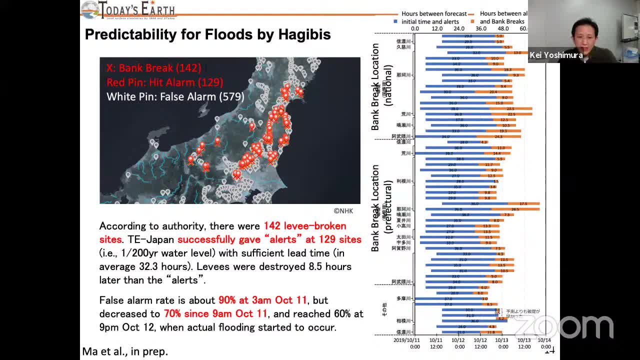 and actually I was so worried at that time. but actually it happened as somehow simulated or predicted. So according to the authority, there were 142 levee broken sites And out of that TE Japan successfully gave alerts, which is defined as once in 200 year water level. 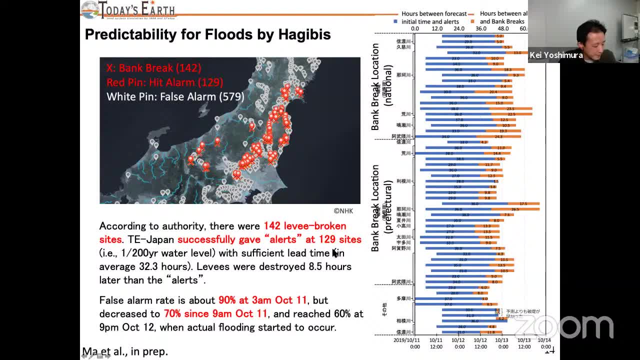 at 129 sites. So the recall is more than 90%. And then the good point is: there is plenty of lead time, more than 30 hours. However, there is. what it shows in the figure is white pins are showing a full solar. 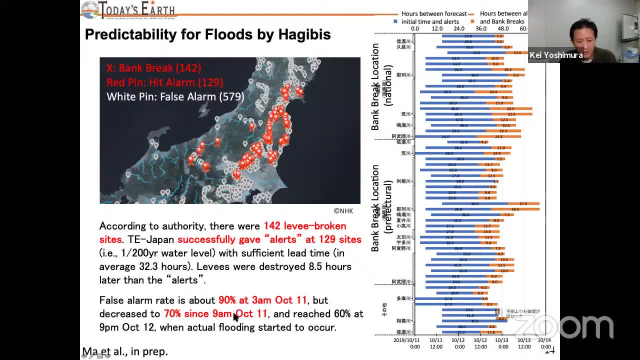 So full solar alarm rate was, I mean, somehow 90%, and it varies in time, but about 70 to 80%. So yeah, that's actually a shortcoming. However, we are not so worried about such a large number of full solar, because this is a levee break. 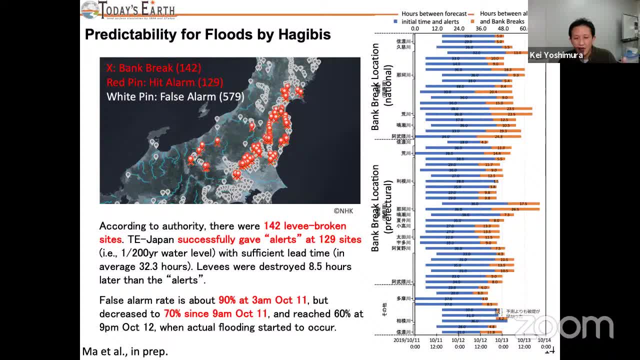 And then levee break is when levee break occurred. actually, the safety level of the different place is getting safer, So it means that. and then our system is showing alerts along the river. So actually it isn't. so how can I say? 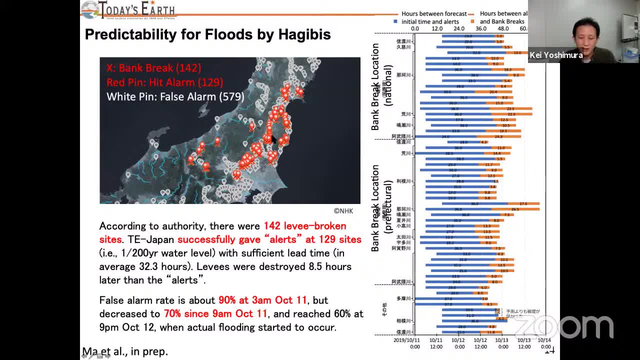 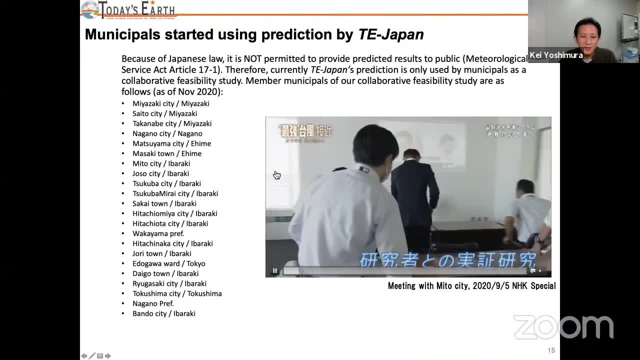 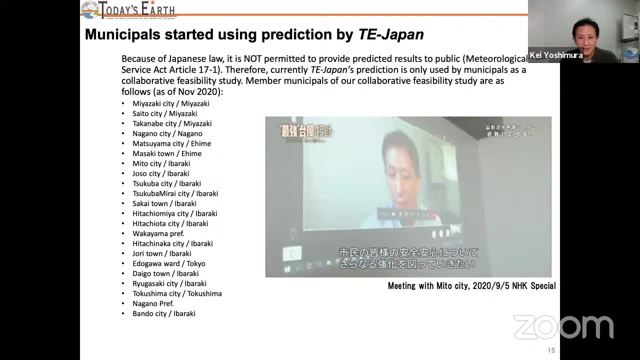 wrong to show pins along the rivers here. Well, actually, those information is cannot be, cannot be provided to the citizens directly in Japan actually. So there because of our law, So only those information is provided to the municipalities right now. 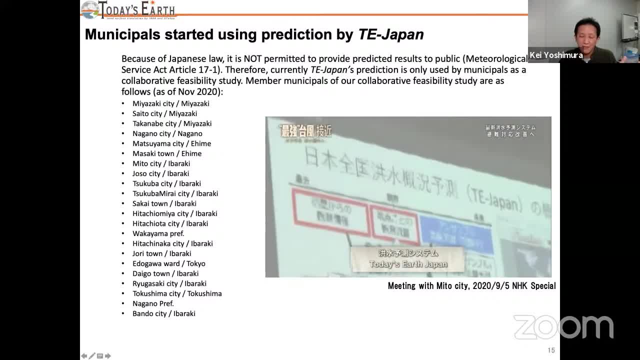 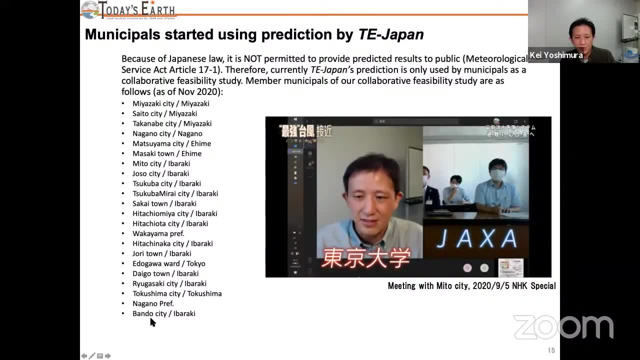 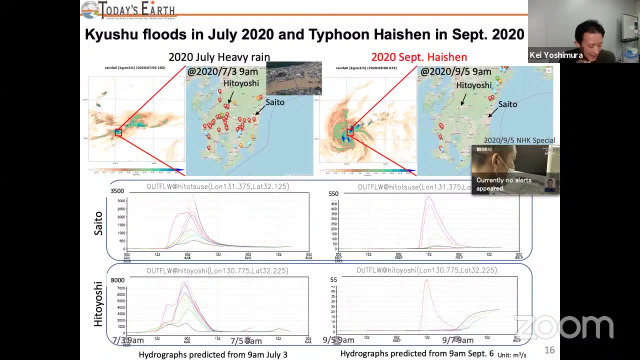 And then there are as many municipalities as we collaborate to research right now, So we are trying to find a way to utilize those predicted information with municipal officers. And then actually there was a floods occurred this year as well, And then there were two very different floods. 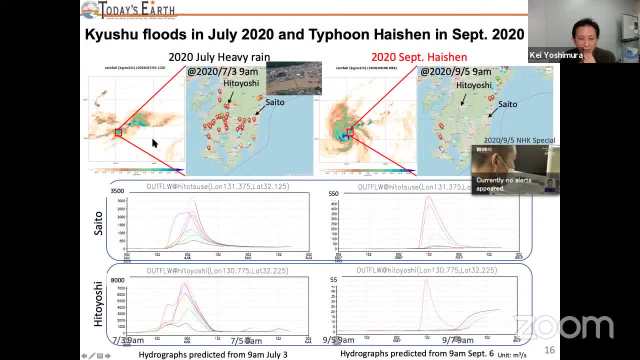 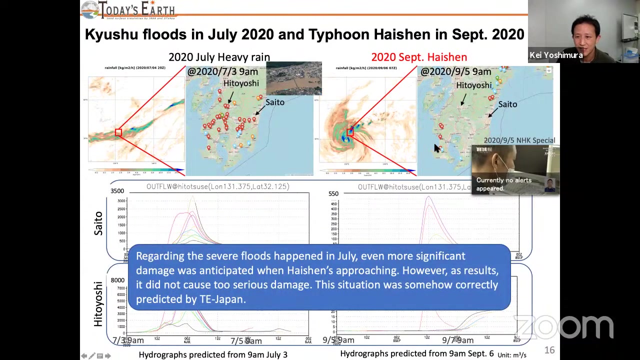 One is caused in July because of the bi-front over Chushu Island And then other is typhoon Haitian in September And actually typhoon Haitian was anticipated, I mean July. there was a flood in July, so that typhoon Haitian was very much worried about. 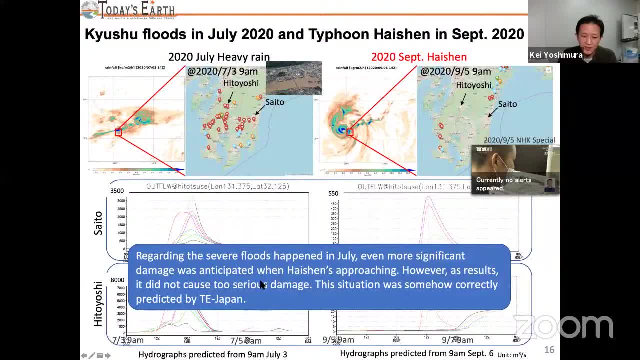 I mean flood. bigger damage was anticipated, but as Haitian approach it, However, as a result it did not cause too serious damage. And then our system also didn't show as much as July events, So it shows. it proved that somehow. 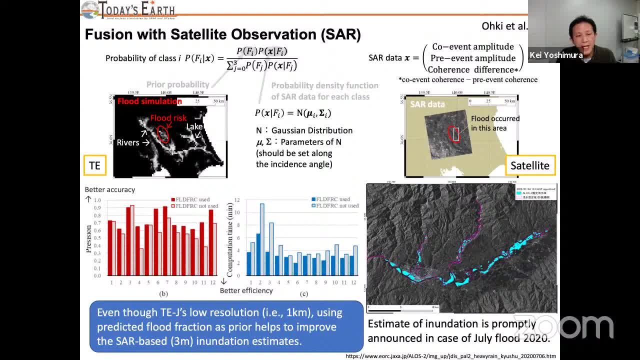 our collection systems is quite right. And then future direction. as a future direction, I would like to introduce newest work done by Mr Oki. It's a fusion with a satellite observation, especially synthetic aperture radar, SAR, And then today's Earth is shown in this. 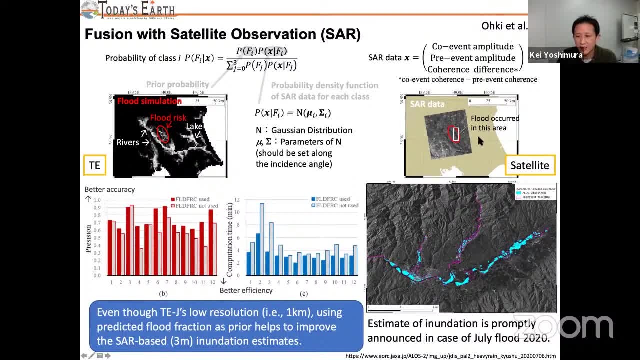 And then today's Earth is shown in this, And then today's Earth is shown in the left-hand side, And then SAR is shown here, right-hand side, And then, using the TE prediction as a prior of the Bayesian estimates of the inundation area, 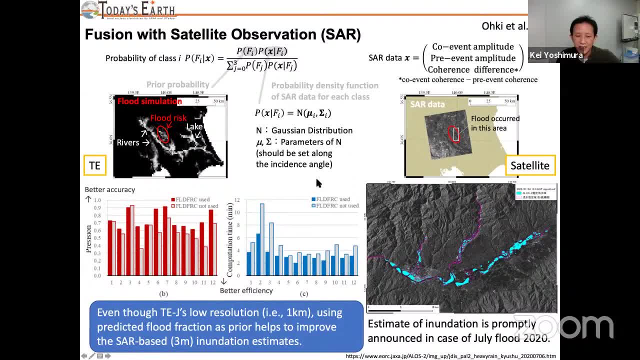 So that actually it helped to improve the inundated area detection, So in terms of the precision and also computational efficiency. So we quickly implemented this scheme into the operation system so that nowadays we actually in July event we could use this system to estimate the inundation. 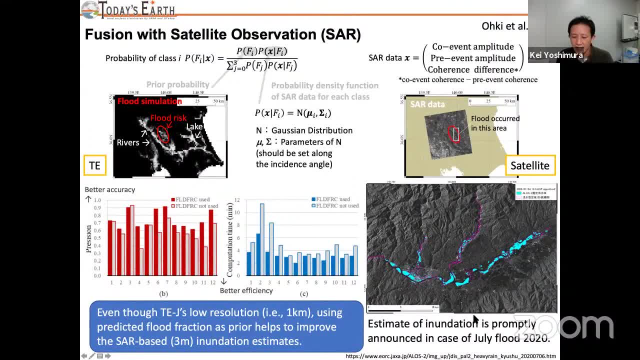 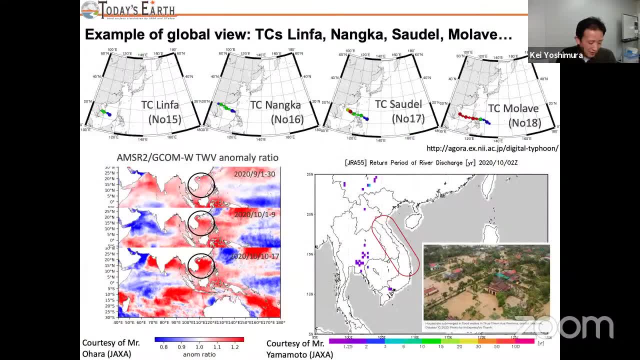 for the Kyushu Islands floods, promptly announced in case right after the image was taken, And then I actually I concentrated on the Japanese system. So this is an example for the global, one of the global example, And then actually, unfortunately, 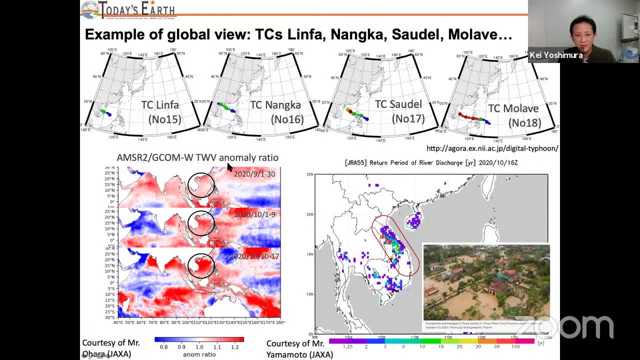 in Vietnam. there was a series of typhoons, tropical cyclones, hits in the lower And then our goal, TE global. even though it is a lower resolution, one fourth degree, the return period of the discharge is showing the animation here in the daily scales. 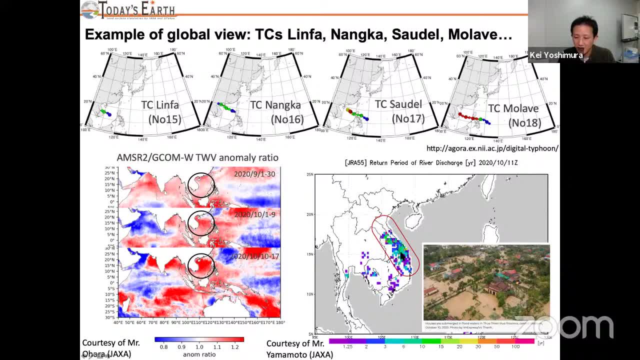 And then it shows a pretty high value depending on the day And then so it actually helps to show the alerts, I mean show the danger level for those area. So this is a summary And then, because of the time limitation, 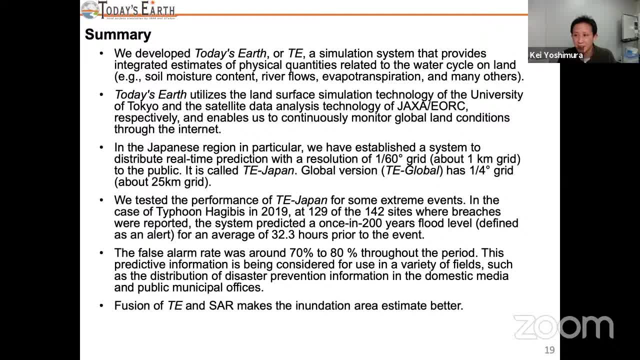 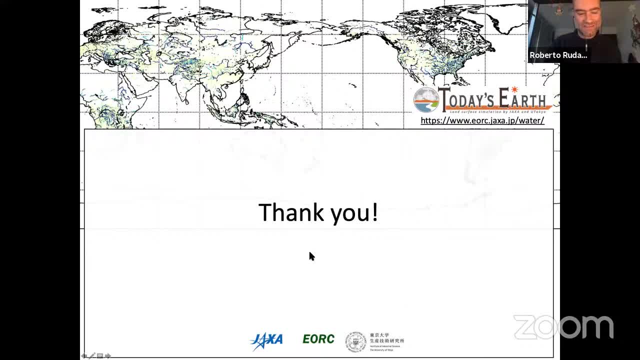 I will do that. I wouldn't read it, So thank you very much. Thank you so much, Kei, I mean, for your presentation. I mean very interesting. Thank you for that And I'm thanking also. I mean: 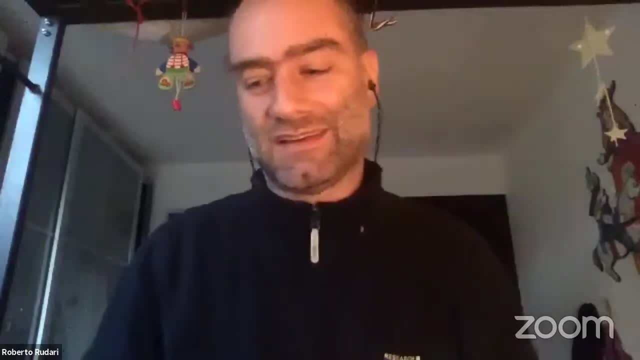 all the other presenters that really gave us and deliver I mean very, very nice in presentation. I mean you could see, I mean from the reaction of the audience, that we have a lot of interest there. Now I mean I would be clear. 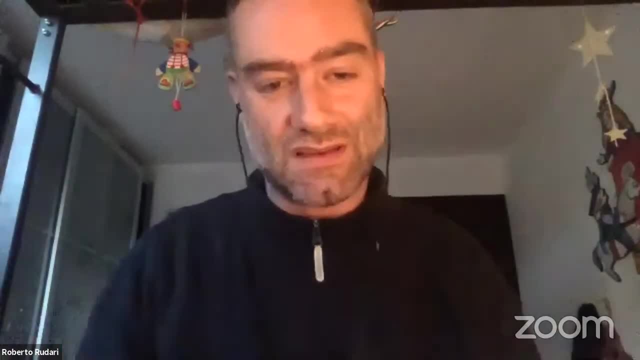 I mean, together with Peter, the discussion, let's say session, open, maybe I mean. one thing I would like to start with doing is to resume few of the key questions that were posed, I mean and also answered already, like in the chat. 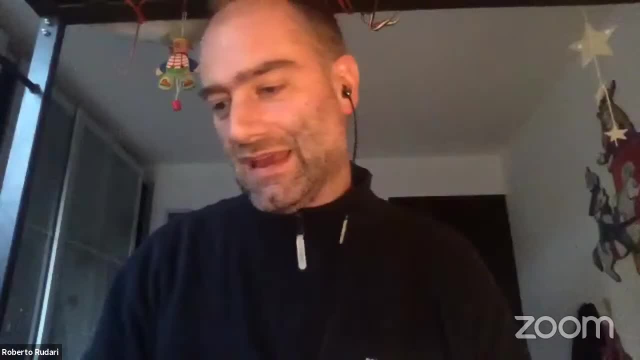 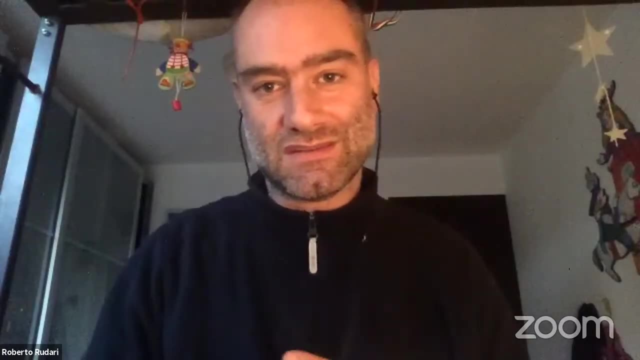 that might help. I mean a little bit. you know the discussion flow And so, Margaret Maggie, I mean, if you agree, I will start with you. I mean you've been the first speaker and having had, like I mean to deal with, many questions, 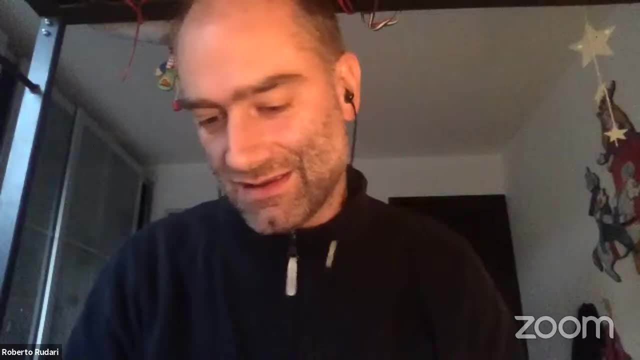 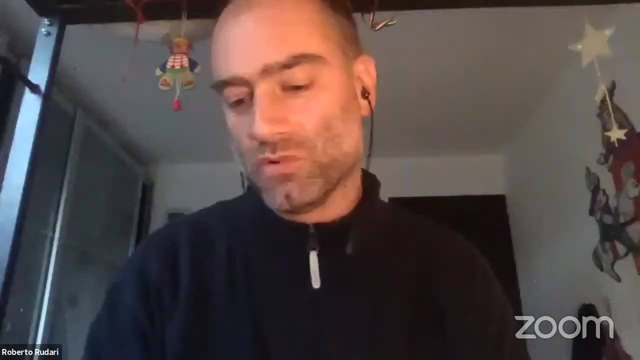 actually I mean in your chat and you've been replying to them. I mean very nicely, I've actually picked. I mean two teams, and that I mean came along. I mean more frequently, I mean in the questions. 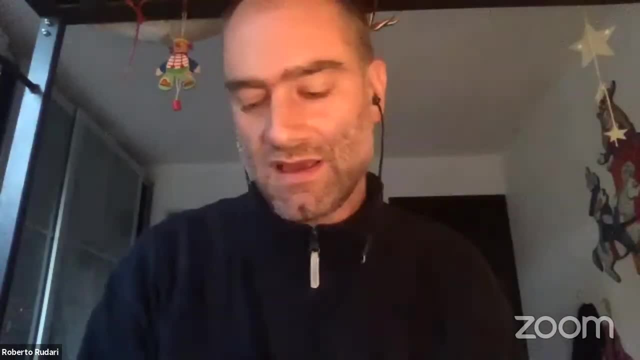 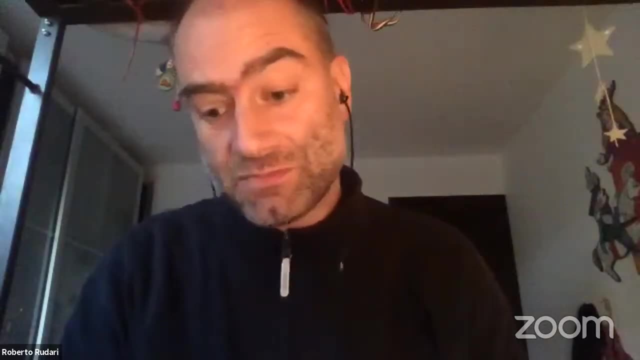 And maybe I mean it would be nice, I mean if you could say a few words in live, I mean lively, I mean here. So the first one is in respect to the validation of the system. There were many- I mean- questions. 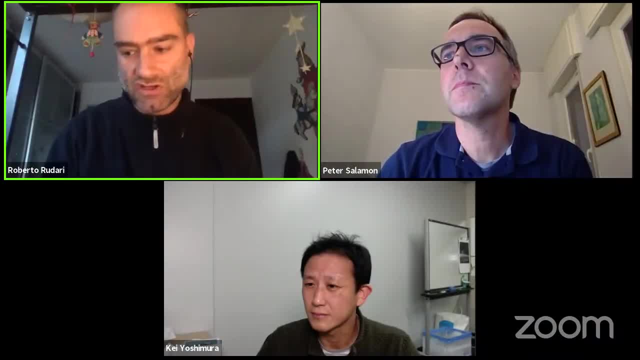 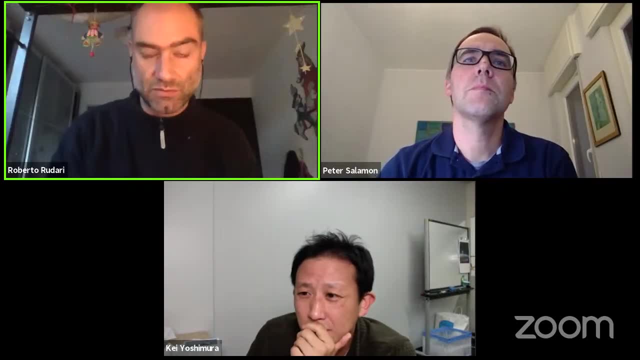 about how you validate the system if you use the Earth observation data, if you are using other information also. I mean to validate the system both in the hazard component and the impact component and how you deal with, for example, 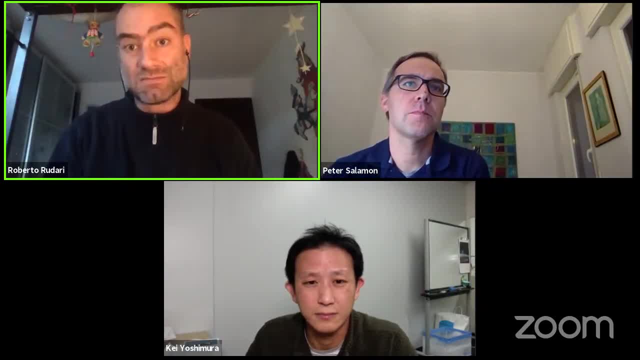 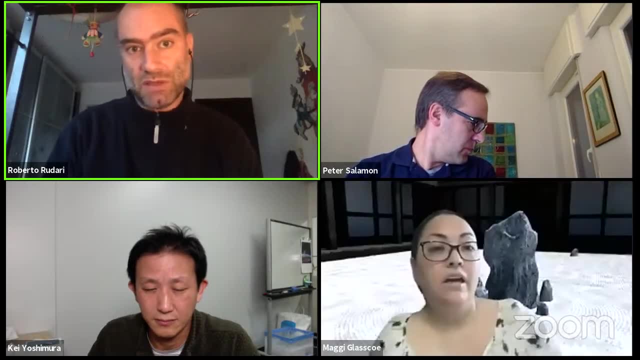 if you're using the remote sensing part. I mean how you deal with the mismatch in scale between- you know this- and the source of data for the validation. So maybe I mean, if you want to start from that And then the second one, I'm just I mean. 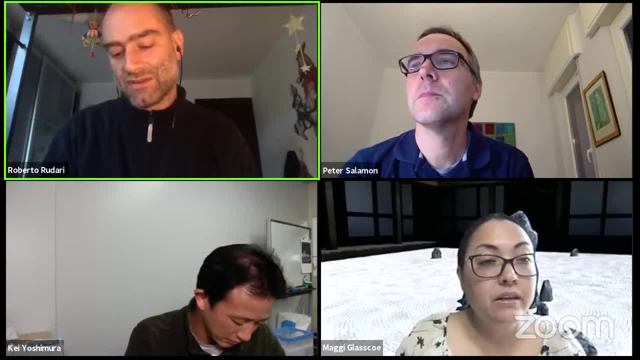 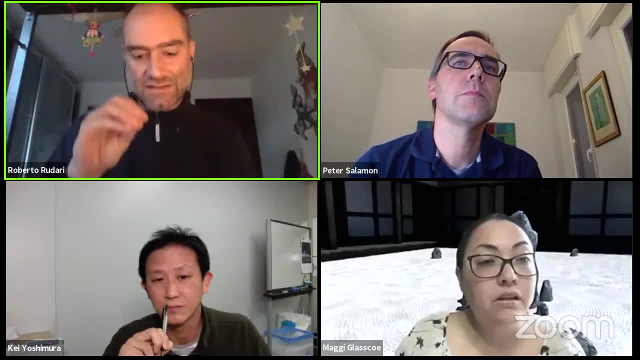 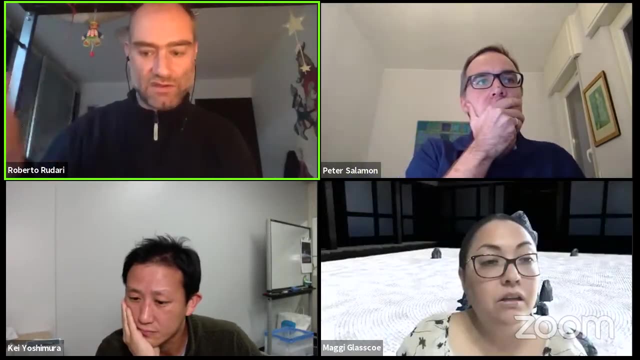 that is also the second thing for you, which I think is very important, and there were, I mean, few questions about how do you, let's say, insert, or if you use, if you would deliver also additional information in addition to the level of alert. 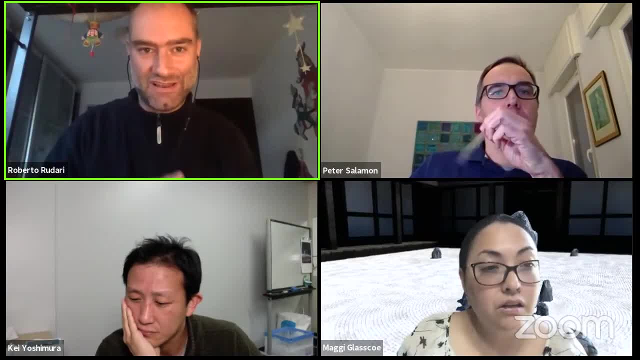 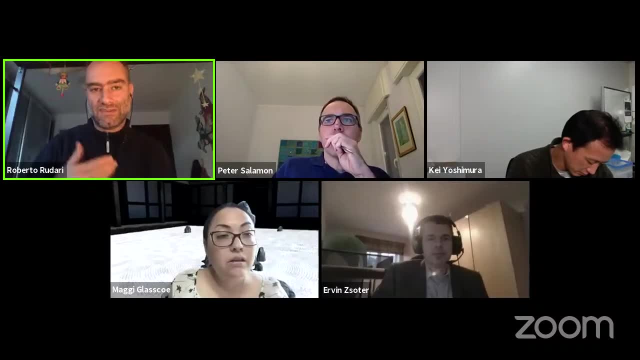 like you know the extent that you certainly do, because you have, like, both the models and your part there, but also the flood depths and the flood duration part component, If that is considered, I mean you use some proxy or you deliver. I mean this type of information. 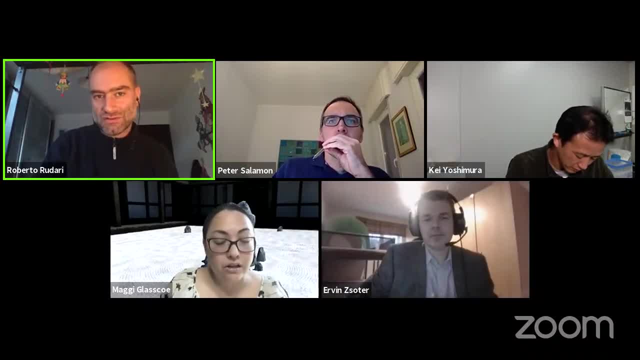 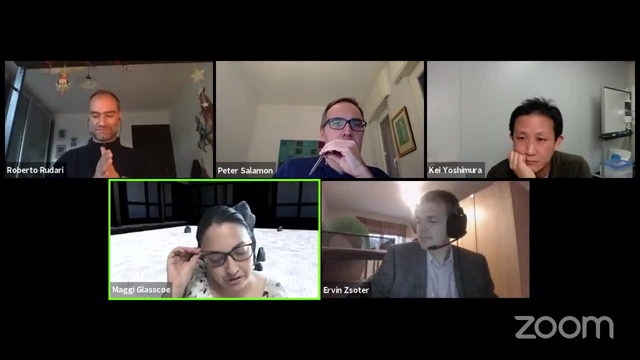 do you plan to deliver it? Thank you, Madhya. I mean, if you want to Sure. So on the first question about the resolution and the for the flood models and the Earth observation data, I believe that the way that they handle that. 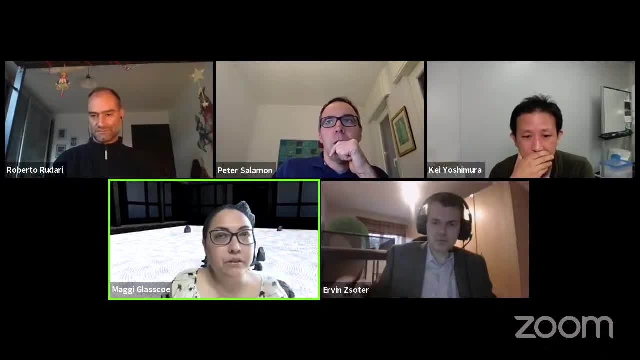 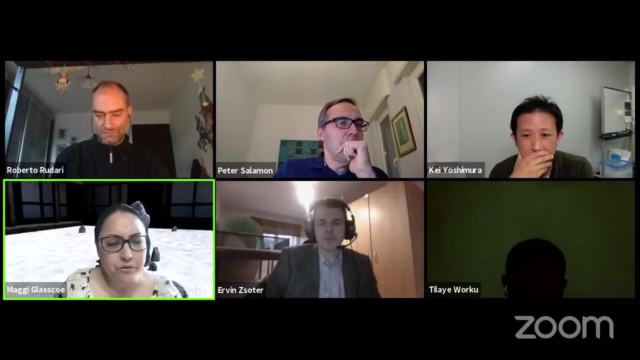 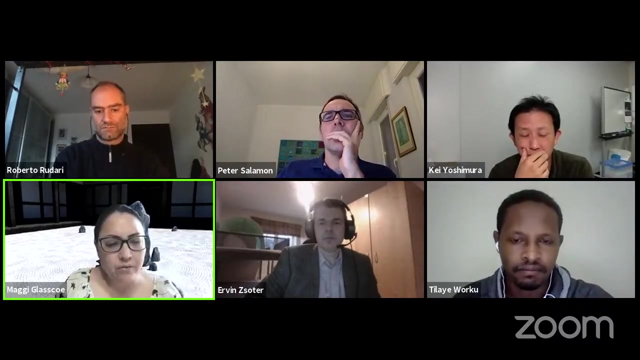 is that they interpolate the data. So what they do is they either downsample or upsample the Earth observation data so that it matches the flood models, and that way they're able to validate that way. And so, and then, as for the other question about 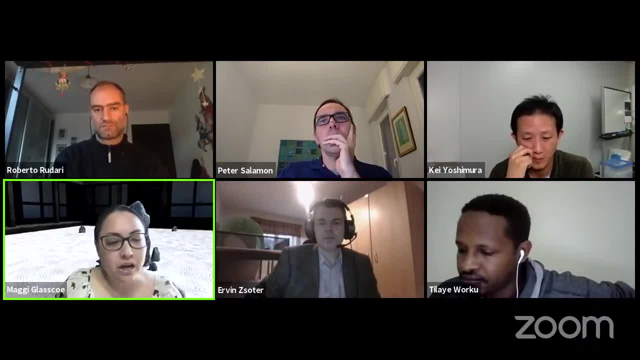 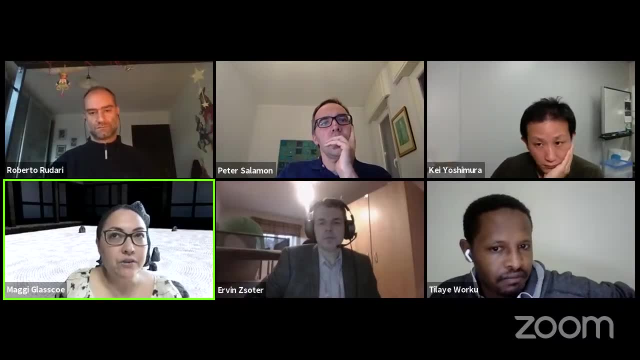 I believe that there was a question about whether we use other data, other than Earth observation data, to validate the flood models, And right now we're not using other than Earth observation data. I know that there's in-situ data that is available. 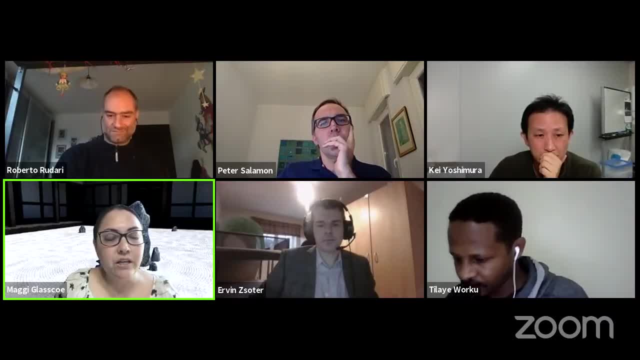 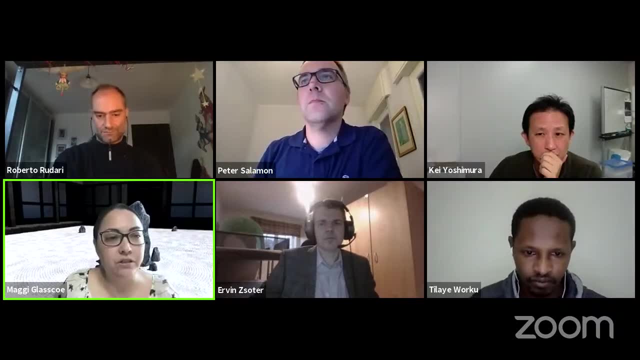 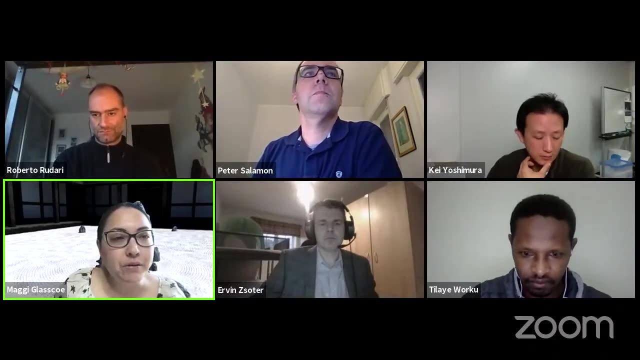 but we haven't integrated that into the system as of yet. But there's some consideration of perhaps using in-situ data to help validate, other than using the Earth observation data. As to the second question, I'm sorry. could you remind me what the second question was, Roberto? 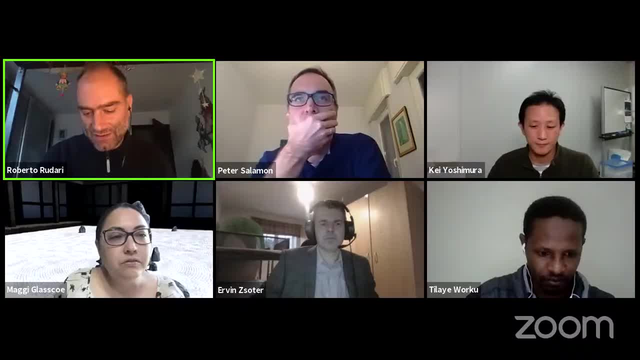 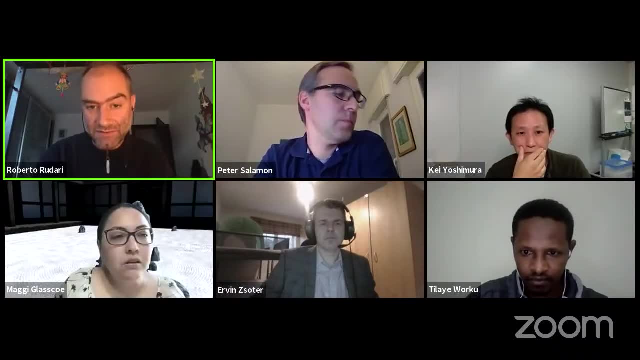 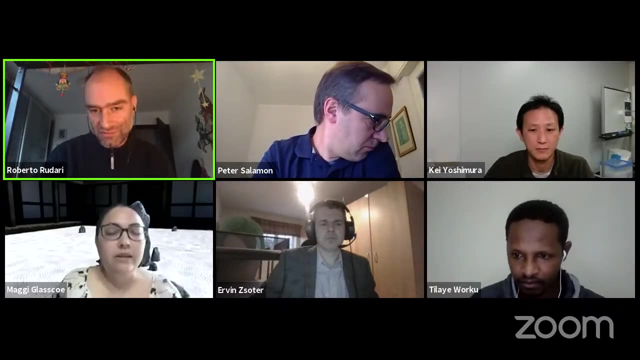 Yeah, sure, If you are, let's say, delivering also information about not only on the, let's say, on the extent of the flood, but also on the water depth- I mean related to the floods- and also on the flood duration. I mean, what type of variables are connected to the flood. 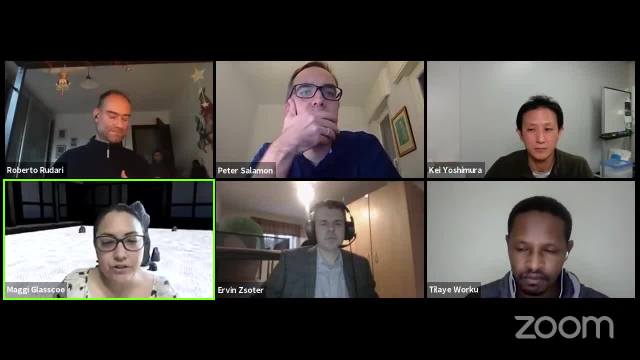 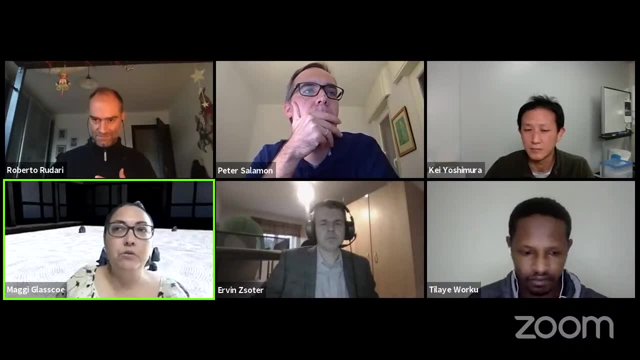 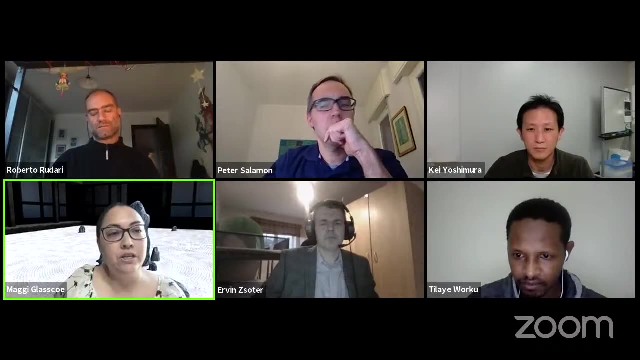 Yes, so we are using the Earth observations to deliver the flood inundation extent or, sorry, the flood extent, but we're also creating high-resolution DEMs to help to determine the flood depth. So the inundation and depth information will be secondary alerts that will be delivered to the PDC. 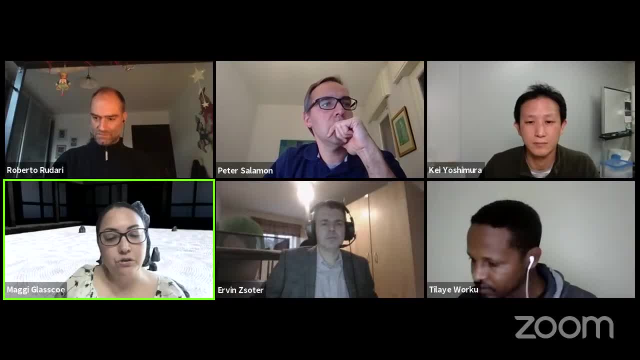 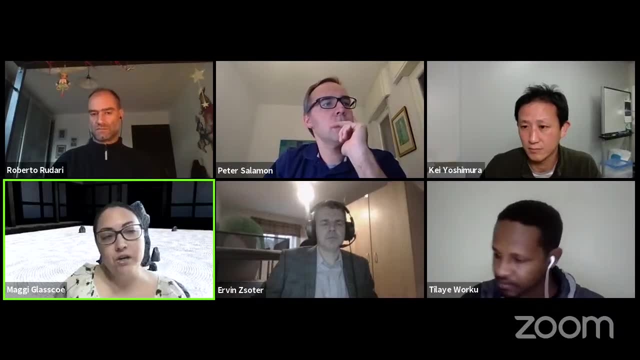 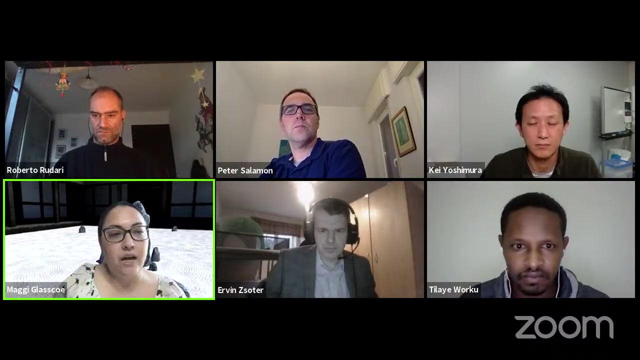 So Disaster Aware allows us to provide the flood severity alert as a primary alert and then create secondary alerts within that alert, And so the flood depth and extent will be created as a secondary alert or additional information within that flood severity alert that comes out from our model of models. 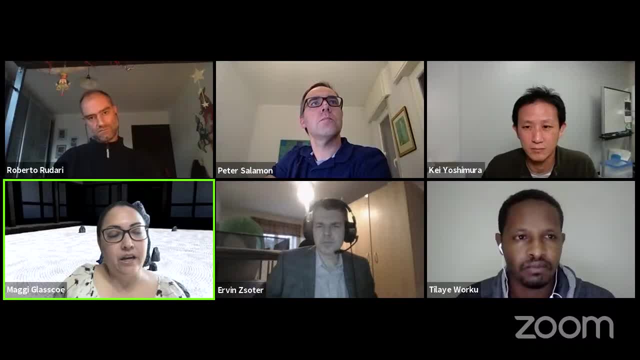 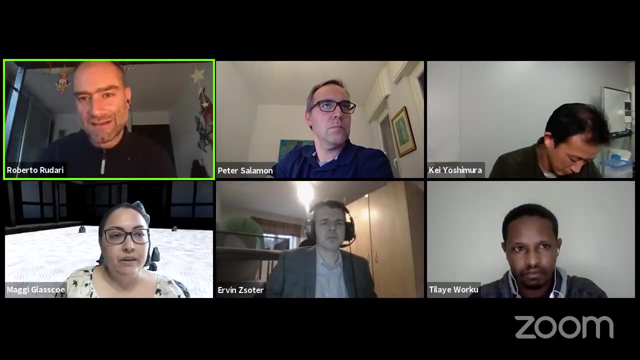 We're also, as I mentioned, there's a third track that is going to include some flood damage assessment and that will come in as additional information to the flood severity alert. Thank you, Margie. Thanks a lot, I mean, Peter, if you want to follow up with questions to Erwin. 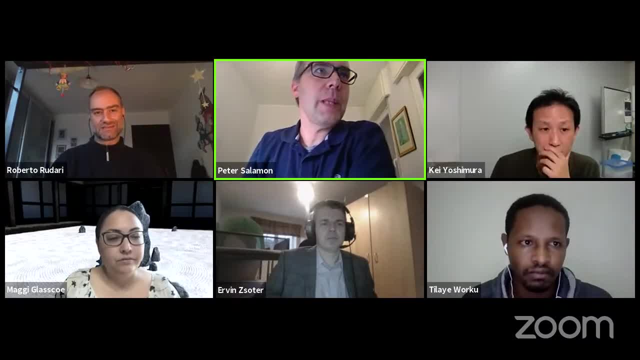 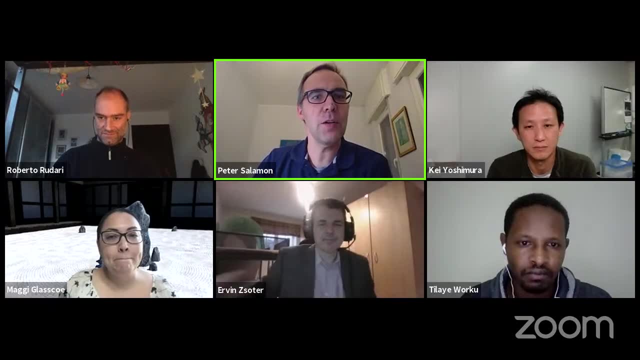 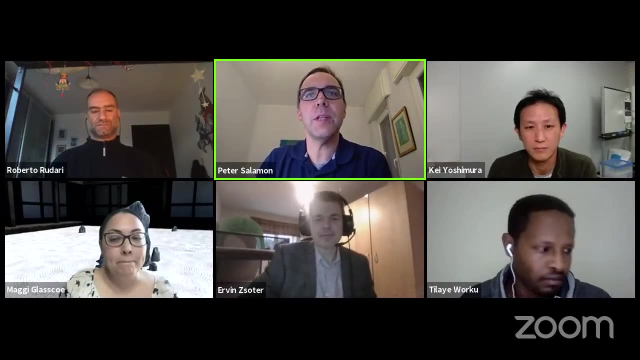 and then I will ask Selah, if you want. Yes, thanks, Otto. from my side, Erwin, I've seen that you've answered already a lot of questions in relation to your presentation, So I kind of grabbed three of them and they're all kind of connected. 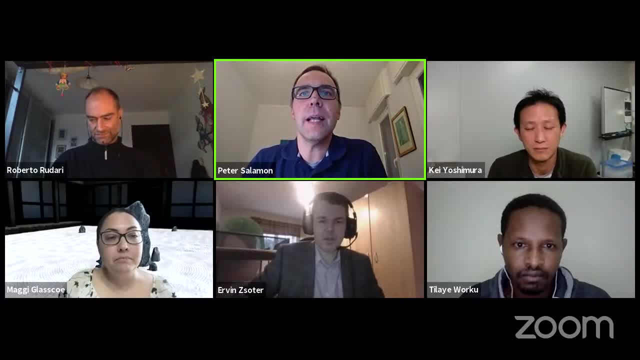 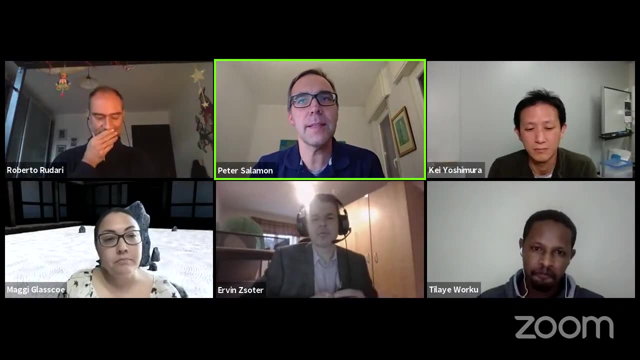 So there was one question In relation to this- an underestimation of streamflow in Glowfast during the rainy season in West Africa- And I saw your reply that this is probably one problem. We know that numerical weather predictions in the tropical areas tend to have lower skills. 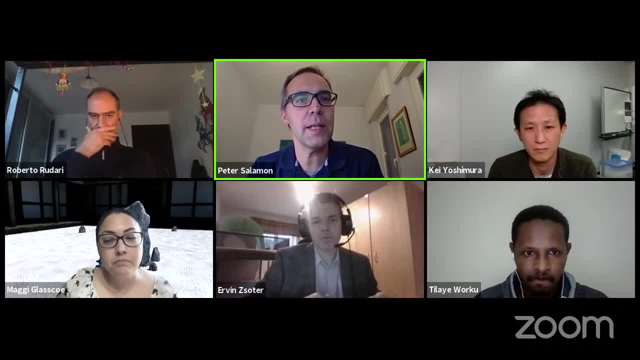 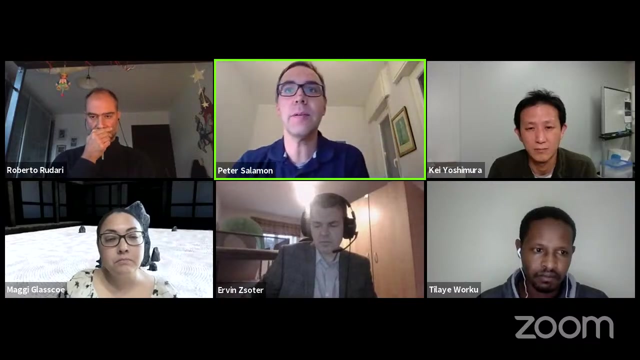 But I wanted to generalize that question a little bit more and maybe you can comment in the first. So the first question is: how can users basically can users know what are the problematic areas where skill is low or high in certain areas, And how can they find that out? 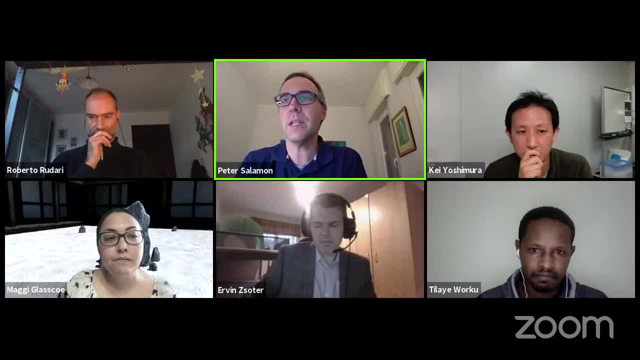 I mean, you saw that or I saw in your presentation. you had something about forecast skill. And then the second question is actually related to that, because when we look at forecast skill, there was a question: why don't we use observed runoff from existing data sources? 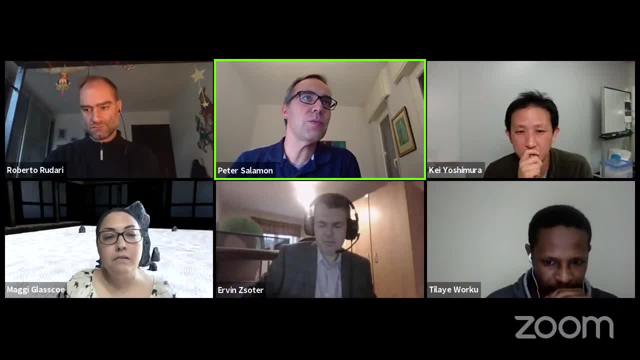 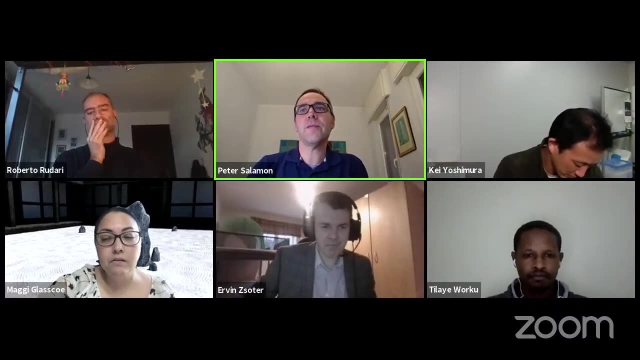 And I think that's a generic problem with regards to in situ data that many of the colleagues here have. But maybe you can elaborate on that problem with in situ data and why are we not using this in situ data for skill, for Erwin? 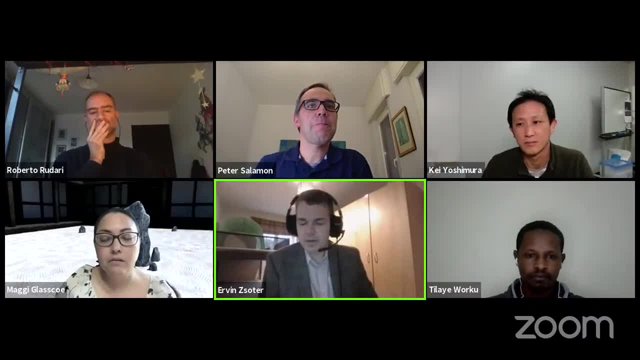 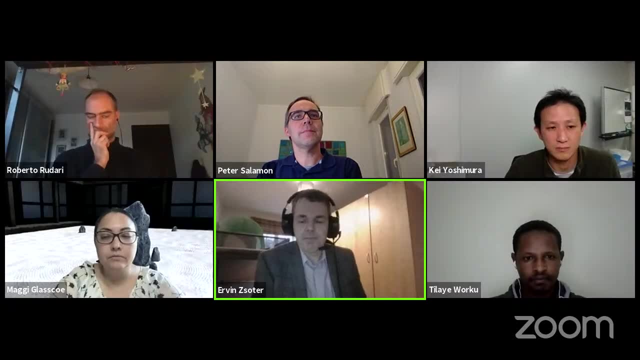 Yeah, thanks, Peter, for the questions. As you said, they are kind of like born out of the same issue or problem. I mean just to make sure we are using observations. so this challenge observations And although for the forecast skill this is the first step is to look at the predictability. 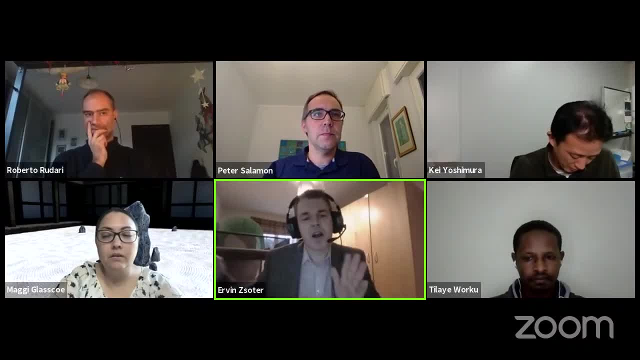 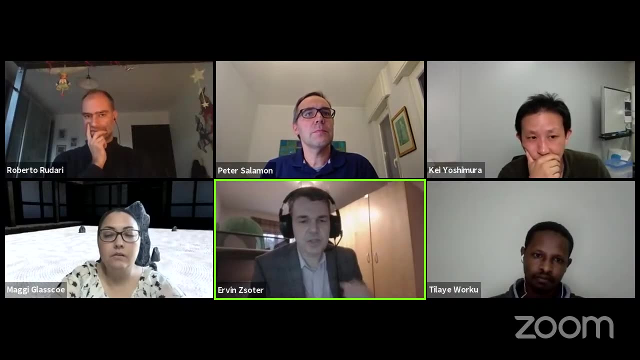 So basically the forecast, how far it can go, And in this first step we didn't want to mix the model error with kind of like the predictive error and therefore only concentrated on using this, on using reanalysis. Generally, discharge observations are kind of sparse, so that obviously 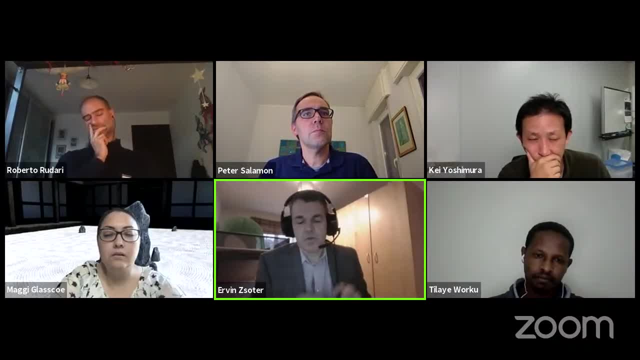 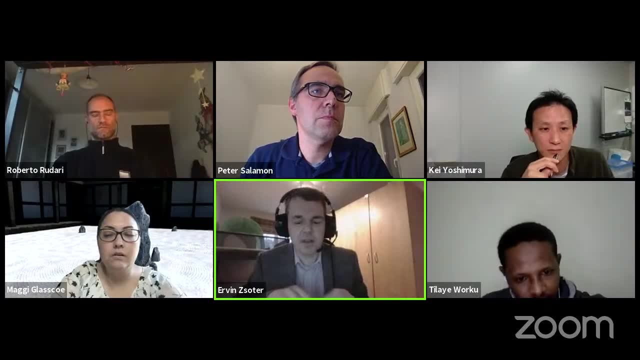 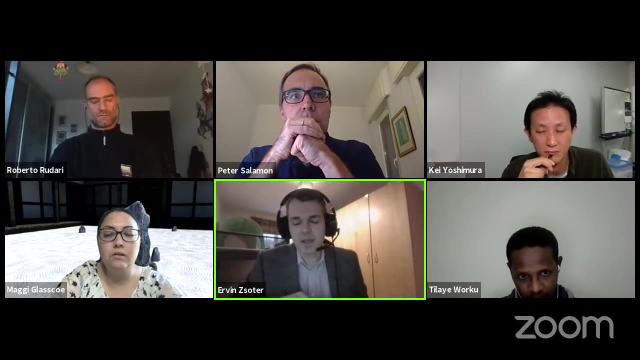 all of us. we are suffering from that, So it will only give a sparse look, at least in maybe interesting areas like especially in Africa. we're always working on acquiring more and more observations, but there will be always kind of gaps in space and, importantly, in time. 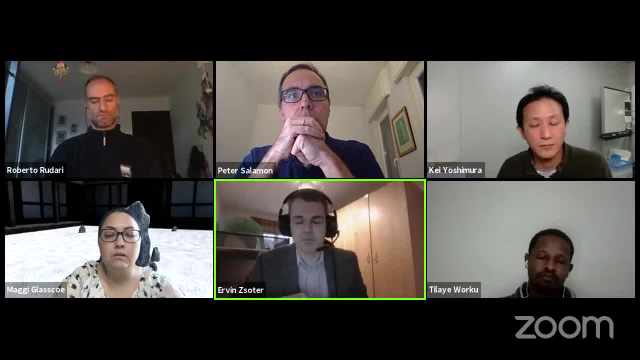 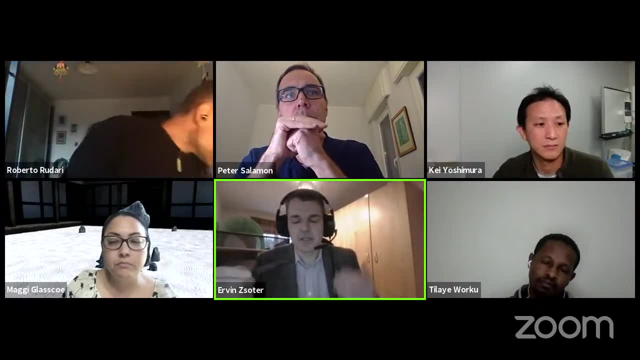 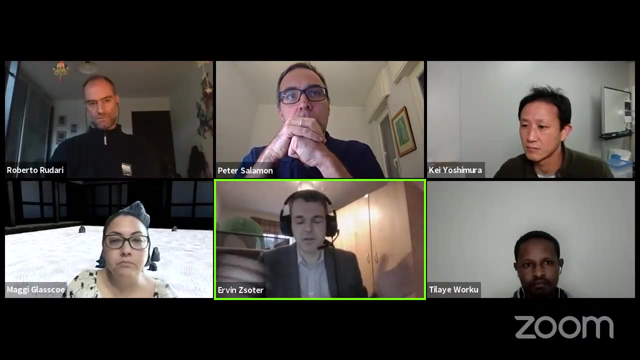 More recent periods are even less covered by observations. However, the model performance or the hydrological scale basically, is documented against observations. So I would- and it is put in the chat basically the reference to the paper, the Gloufos R5 paper. That's basically a good. 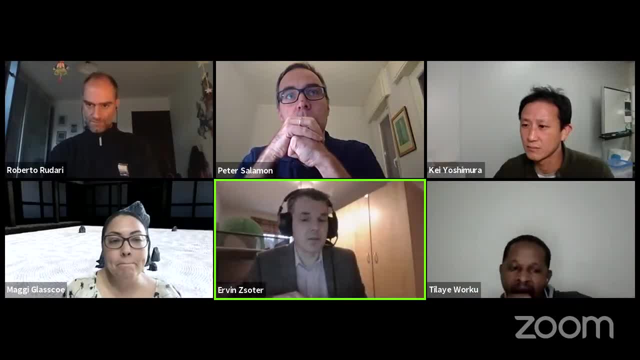 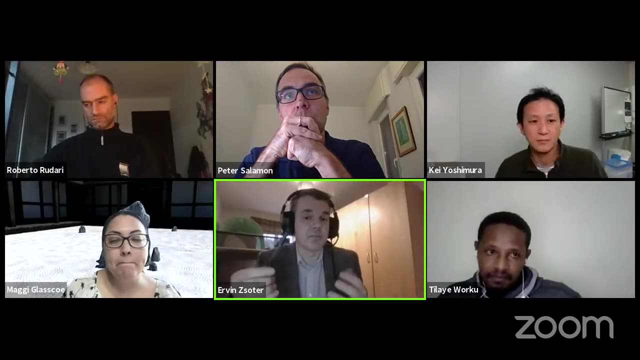 source, where you can, at those points where we had observations, where we could actually add in that study, compare the model performance where your area is and, basically, is it acceptable, Is it not acceptable? And in many areas it is pretty good And in many areas, unfortunately, 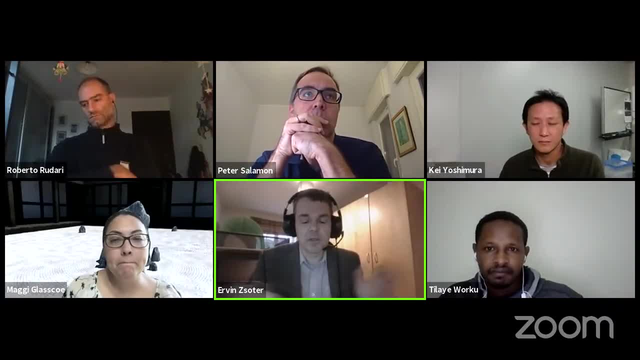 it is not very good at the moment And often in the tropics, also, as you've mentioned, related to the lower scale, methodological forcing and maybe other problems as well. the scale, the hydrological scale, is still lower. In the future there will be new. 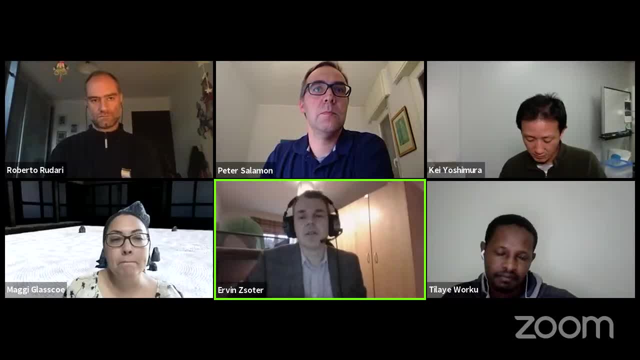 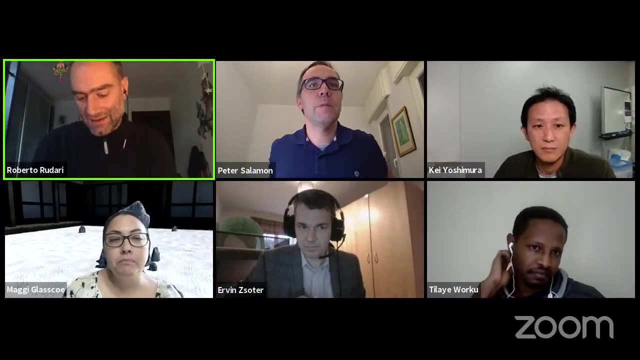 information provided also in the web, different layers which will show performance, like focused performance against observations as well. Okay, Thanks. Thanks, Erwin, Roberto, I pass to you. So yes, I mean Sela, I think I mean. your presentation was very much. 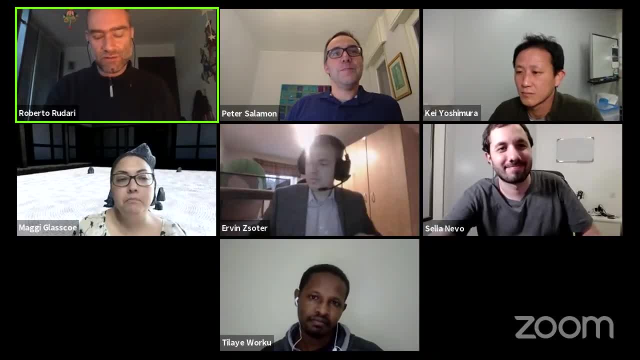 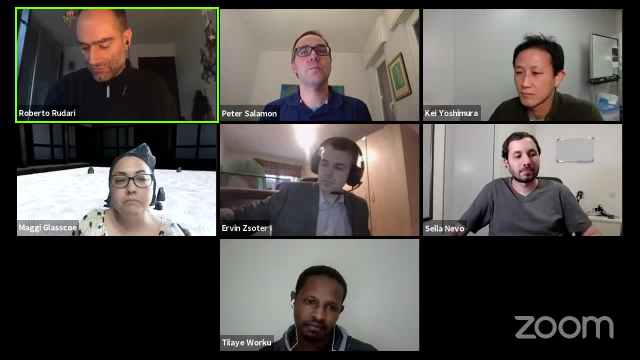 kind of interesting. I mean a lot of. I mean new items and new food for thought. I mean also for us like working in the field, And you've received, I mean, so many questions. I mean again, I picked just, I mean one or two, three actually that I think I mean are 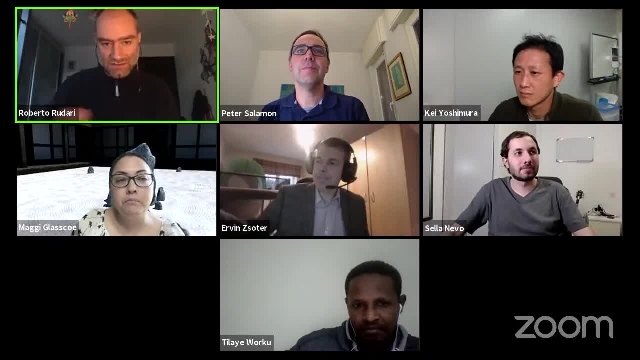 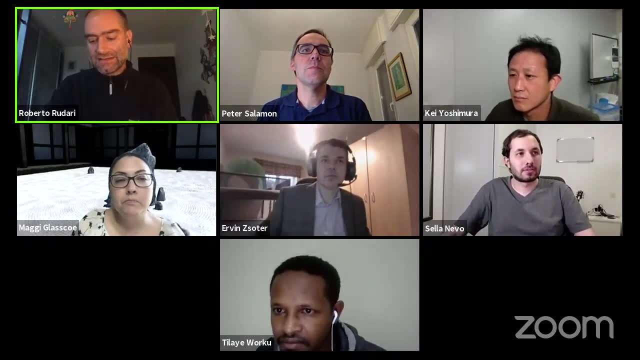 representative. The first one actually is many questions, but they have all the same, let's say, I mean scope in a sense. I mean so about you know the data needs. I mean for you know training, basically the machine learning, I mean model that, I mean you. 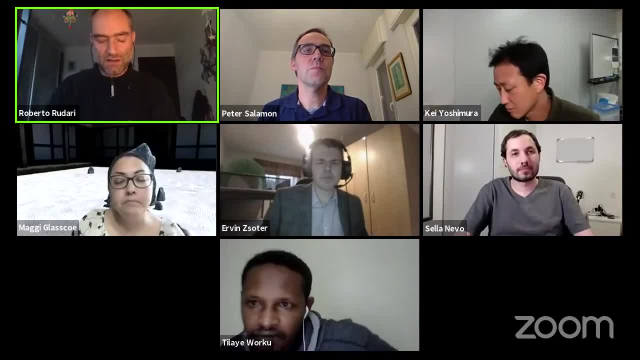 presented. I mean there are evidently I mean- concerns about you know the level of how deep in time I mean the training data set should go. I mean what is the you know the type of input data. 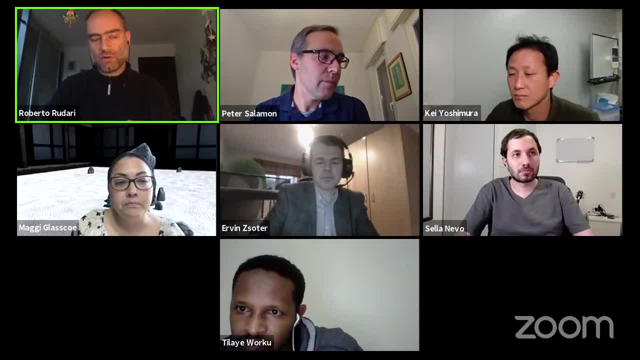 and target data that you're you would like to use. I mean so I read in all these questions like I mean some concerns about you know portability. I mean to you know, at a global. 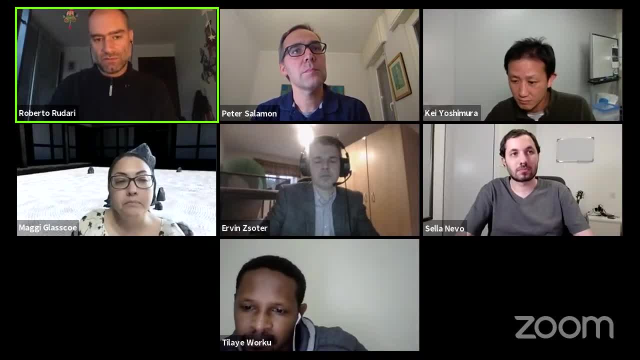 scale where you know data scarcity is certainly an issue. I mean, it's not not, let's say not everywhere we are. We have the luxury of having a global scale of data, of you know datavine and 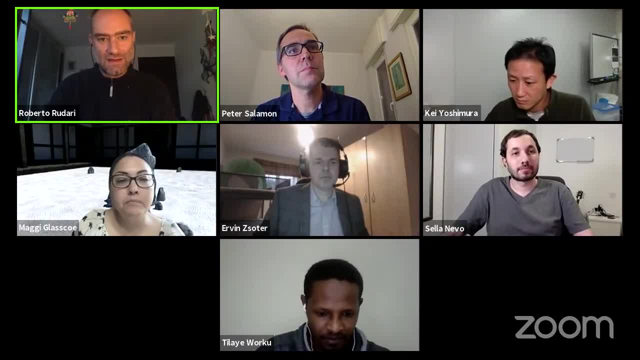 you know having a global scale of data, For example, we have these, you know these, you know having the same, you know data sets that you've been using the us and so i mean maybe, i mean if you could reply, i mean on to the portability of this type of models, i mean on a larger 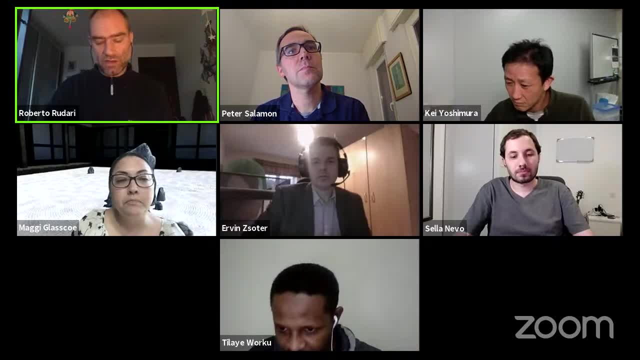 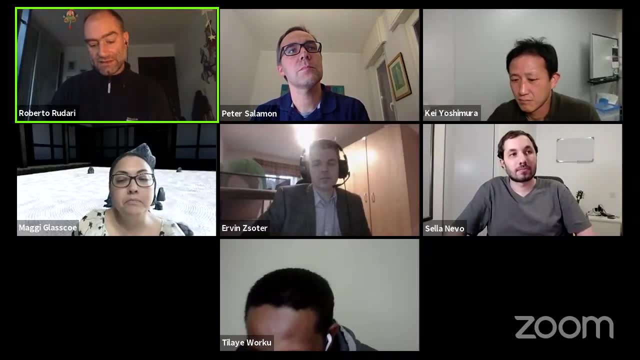 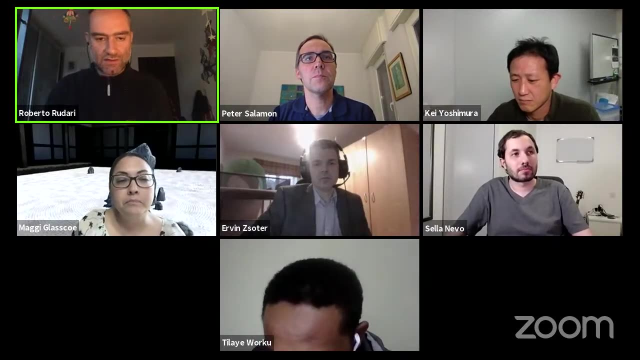 on larger domain also, like in places where you know the data, the data availability, i mean in times and space, i mean it's very scarce. and that is the first i mean point, um, the second one was about the availability of the google alert. i mean that i mean was was raised. i mean is that? 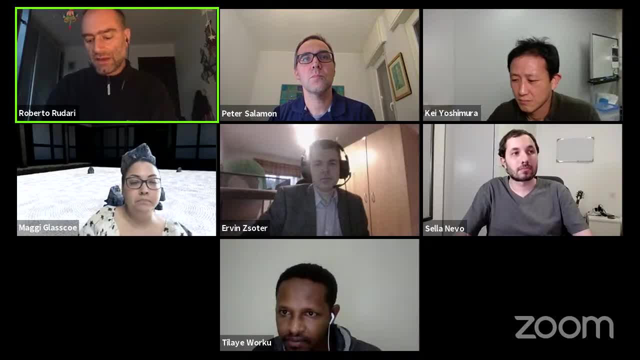 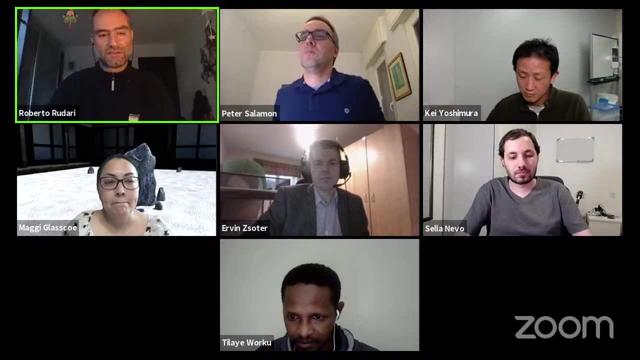 available and you say, yes, i mean it is. i would be actually, i mean uh, interested in learning a little bit more about the institutional setup that you have, i mean in delivering these alerts. i know you have, i mean, a good setup, for example in india, but i mean going again to a global scale. i mean, how do 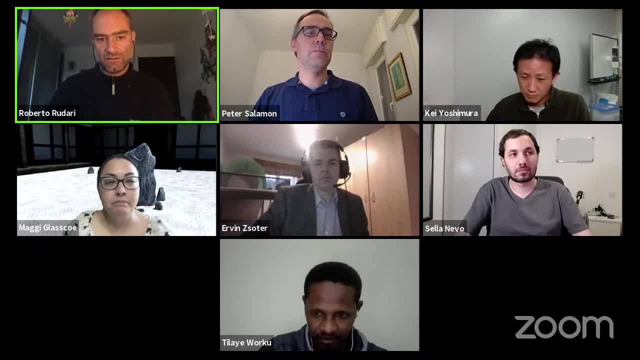 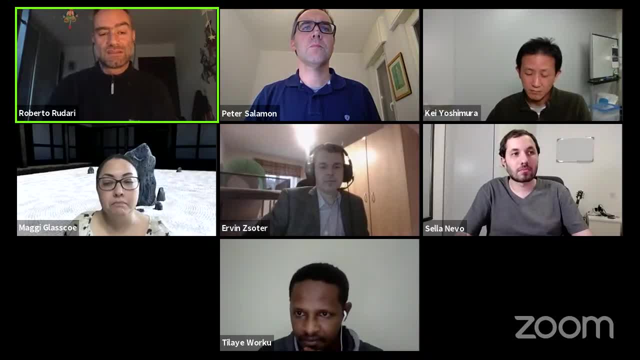 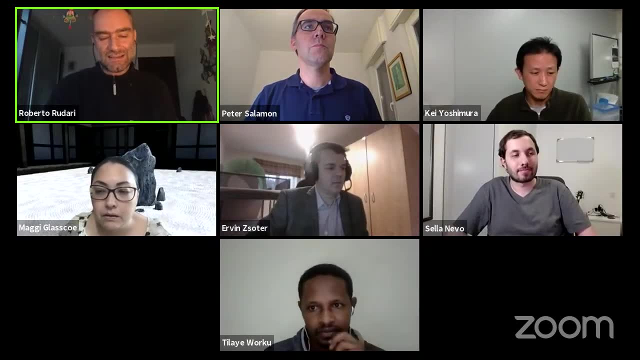 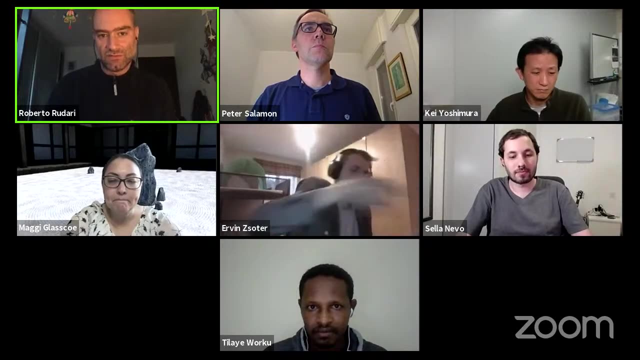 images, which is a very interesting topic, and the question there maybe i mean nobody asked, i would ask i mean: is that, uh, the accessibility, uh, of that data set? that looks very interesting, i mean for you know different types of of studies and then including also, you know, morphological studies and so forth, so also that 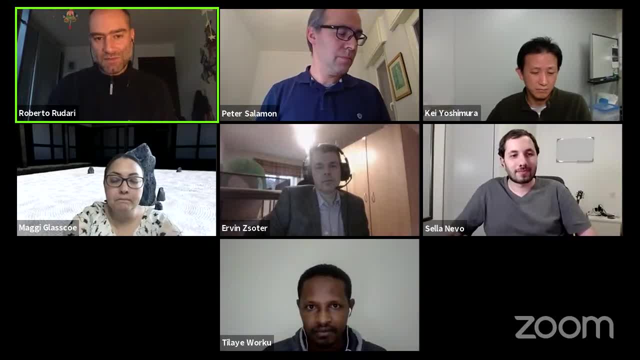 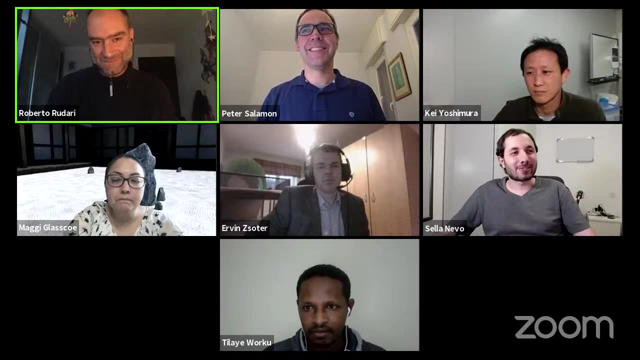 part and then if you could uh tell us, i mean if that is available and where and and how, basically, i mean, this could be accessible. you can start, i mean, from anywhere, and i can repeat. you know the questions if you don't remember them, and instead of yeah, i'll try to answer all of them. i'm also 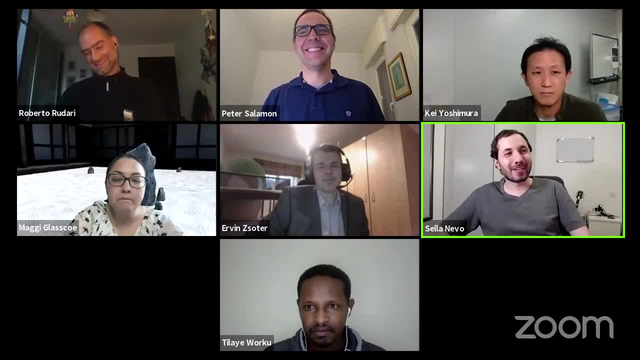 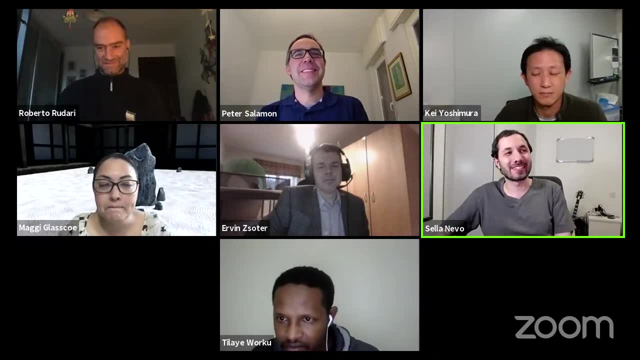 aware we're limited in time, so i'll try to rush through them. this also applies to the chat. i've tried to answer everything. if there's something i didn't get to answer, i'm going to try to answer it again. i missed it, but uh, yeah, thank you all for the questions. so first, in terms of uh machine, 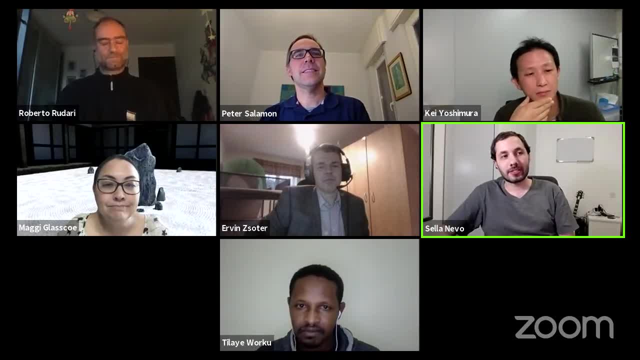 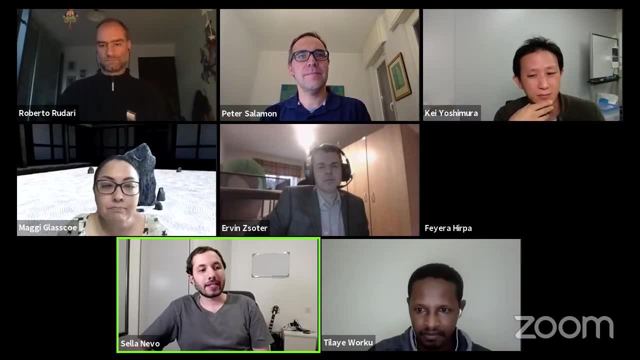 learning and data needs. so i think, um, in general, it is definitely true that machine learning methods are kind of data hungry and data driven. in general, methods are uh need more data. i think. when used intelligently, though, they can actually be useful in data scarce regions. that's actually. 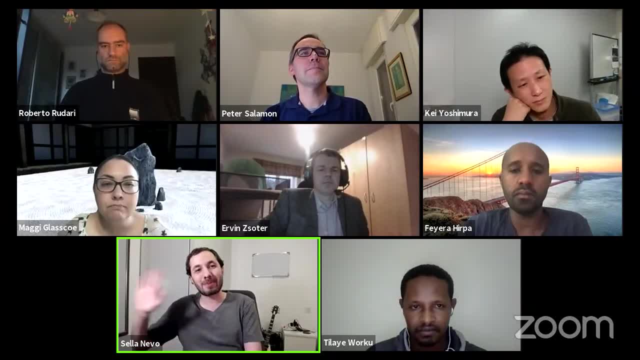 where we've done most of our work, so it's easier to publish, right? so our academic publications are usually in places like the us, but actually most of our work is in data scarce regions and that's where we're doing a lot of data: in bahrain, india and bangladesh, which have very serious data. 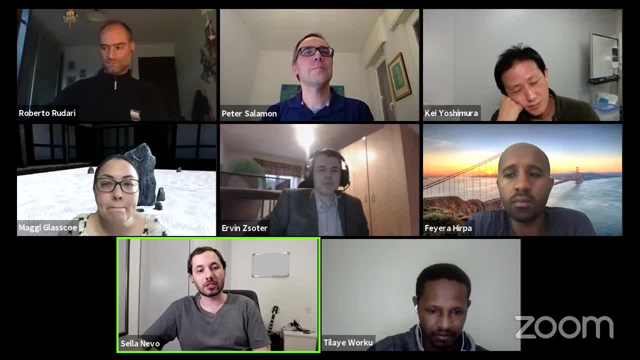 scarcity problems and just the two things that i kind of slightly mentioned in the talk um are one: if you break the assumption that you can't learn across basins, then you can require more data overall but less data per basin, and that's kind of in the hydrologic modeling, i think, one of the 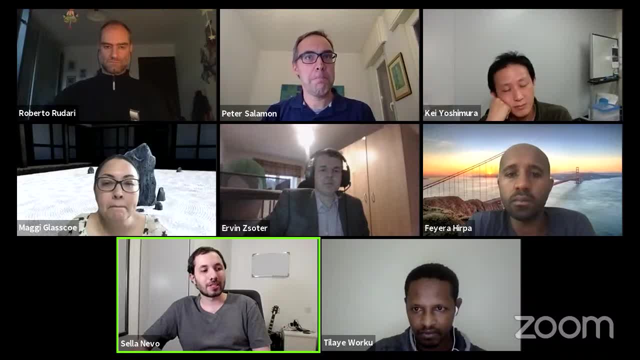 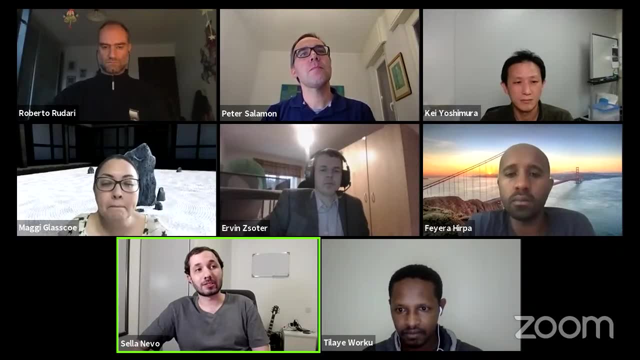 uh, one of the best advantages of these lstm based methods- and we actually have a separate paper that i haven't linked to yet, but i can, if people are interested- where we show that we actually achieve better results with extremely little historical data. So even after one year of data, we can. 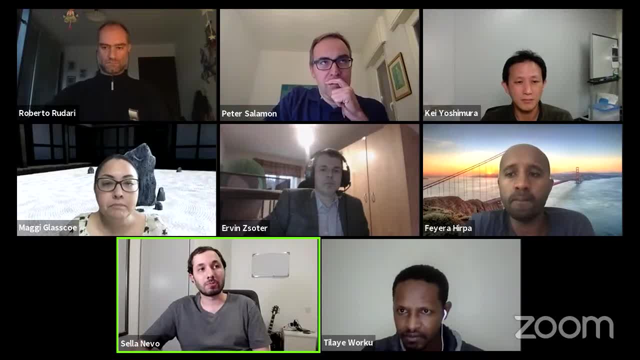 achieve better results when we use this kind of distributed, shared model across different basins. And then secondly, is how we use optical and SAR imagery to correct our inundation models. So here as well, again, we're kind of overcoming one type of data scarcity, for example. 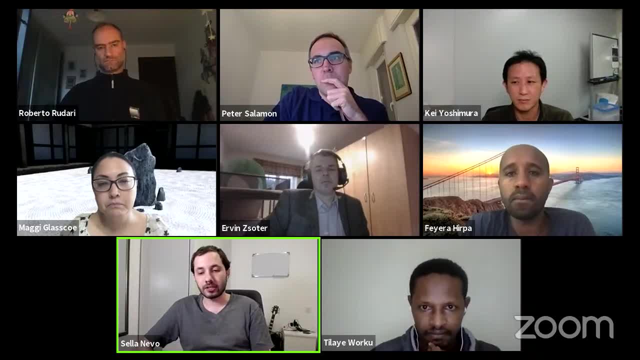 high quality elevation maps and on the ground structures, with utilizing the data that is available globally, like optical and SAR imagery. So that's kind of my short answer for machine learning and data needs, but an important question, just to say I'm not trying to say. 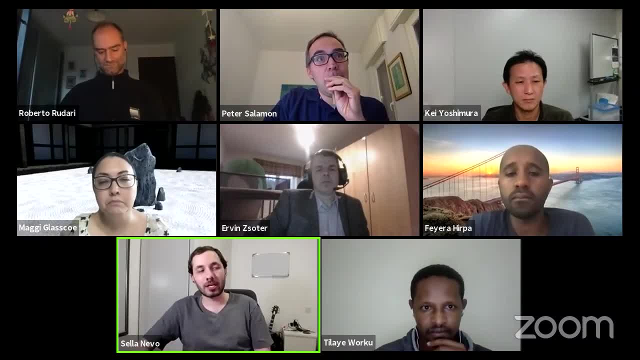 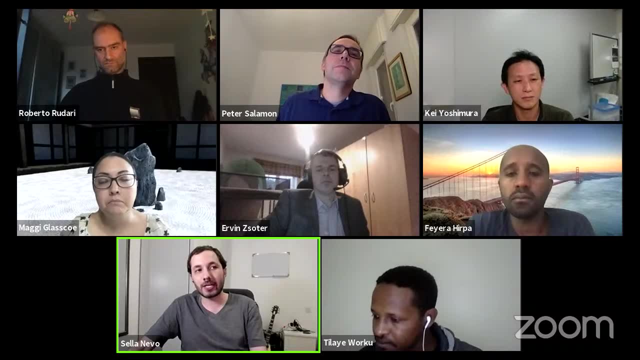 and therefore it'll work everywhere. I'm just saying it really depends how we apply these models. The second question was about the availability of Google Alerts. So I think there are two main ways to access our alerts. The first: we have two types of interfaces: One: 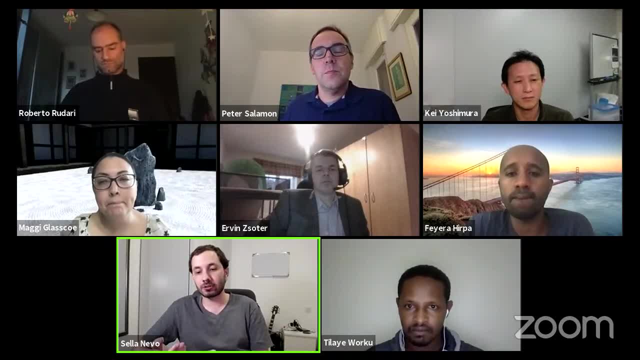 is kind of the same as the other. The first is kind of the same as the other. The second is kind of the same as the other. The third is kind of the same as the other. The fourth is kind of public-facing interfaces. So if you search for floods in your area in Google Search Maps and so on, you can. 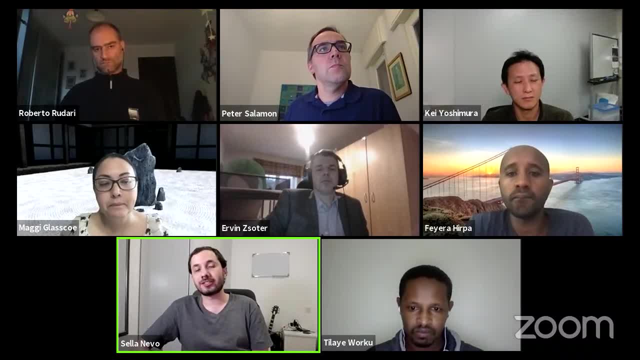 see it. You can also see an aggregate of all of our current alerts in gco- slash floods. So that's kind of public-facing. We also have close collaborations with organizational partners, So with the Indian government, the Bangladeshi government, with the Red Cross and so on. We. 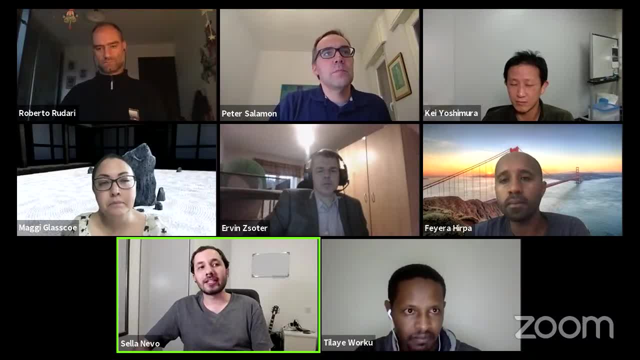 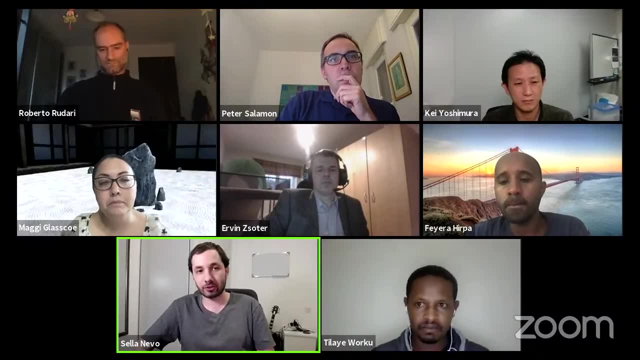 currently don't provide a kind of broad institutional public service in the same way that GloBefest, for example, and NASA do. NASA do, Which I think are doing an amazing, amazing job at that. We don't have currently anything in parallel to that. Maybe we will someday in the future. At the moment, if you 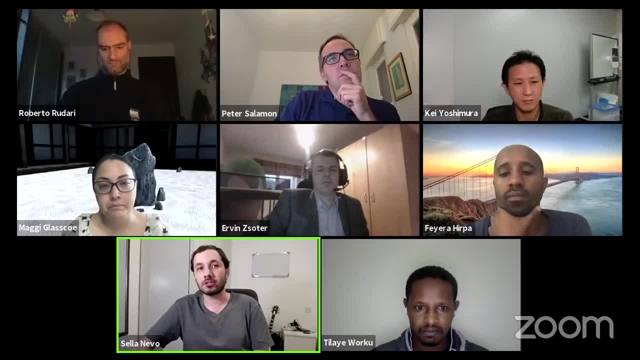 want to institutionally utilize our alerts, then you do need to talk to us. And then, finally, about the DEM generation. So I'll just very quickly say that. so currently, the DEMs themselves the raw data we don't share publicly. We're trying to work on making it accessible for 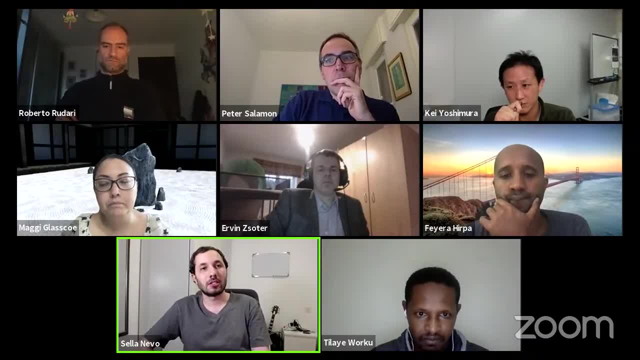 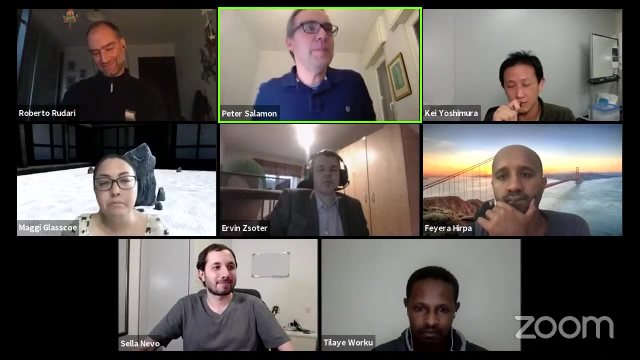 academic uses. There are some legal constraints there, But again, if this is something that people are interested in, they can reach out to me and just I can at least keep them updated on what the status is. Thanks so much, Peter, again to you, Yes, thanks. Thanks, Roberto. Now, Juan, we saw your great presentation on 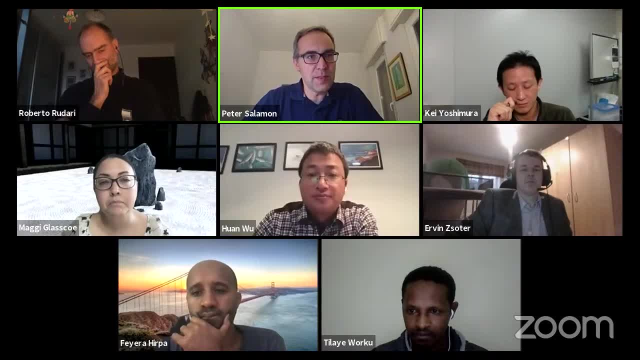 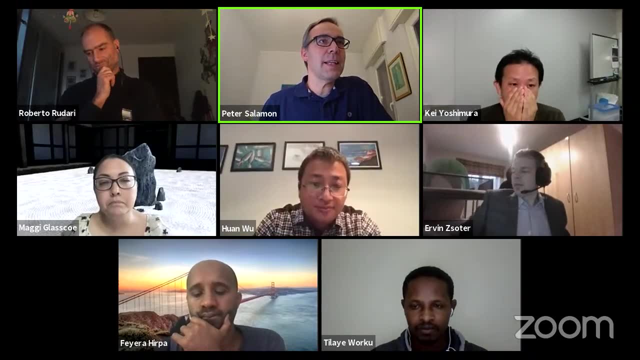 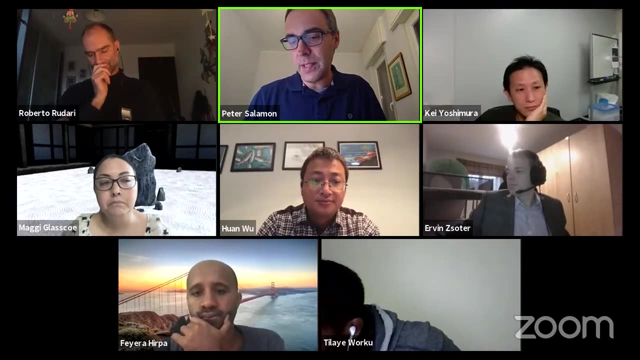 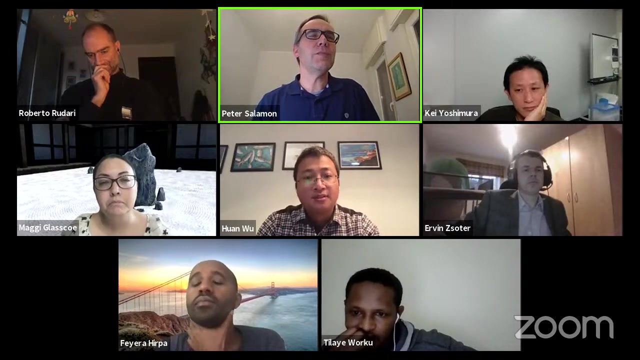 linking basically seasonal forecasts or looking at the seasonal predictability of floods, And rather than asking specifically about an element on your presentation, what comes up always- and I see this in many other presentations- when it comes related to to seasonal predictability and the question is: do you have an example how you then can put? 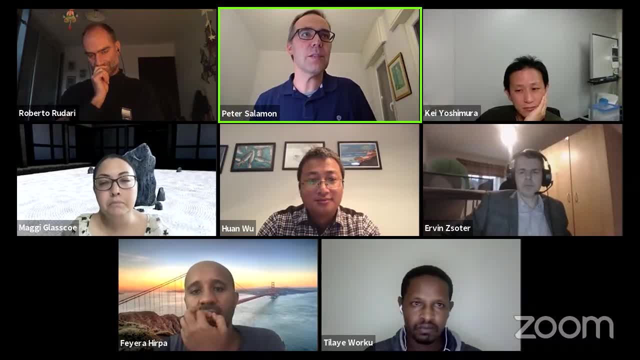 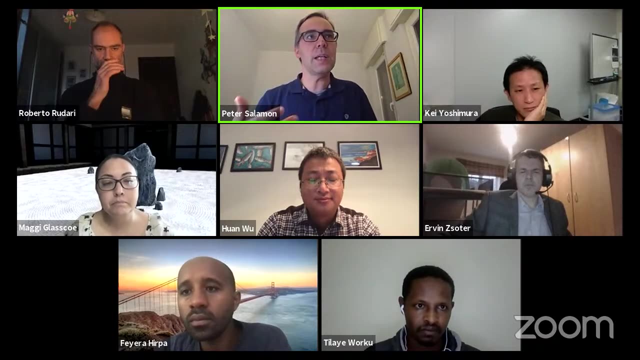 did you put them, your indicators or your seasonal predictions, in practice, Like how you know, because they're so fundamental, fundamentally different from a five-day forecast? let's say, you know where you predict a certain river discharge When you look at seasonal or these predictors for ENSOs, you know. 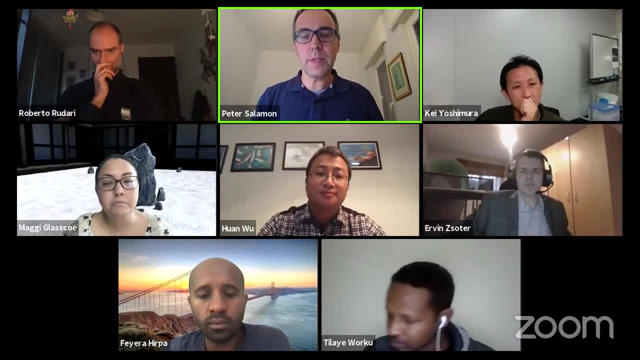 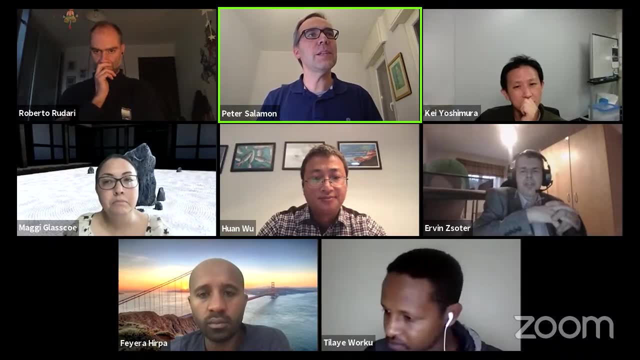 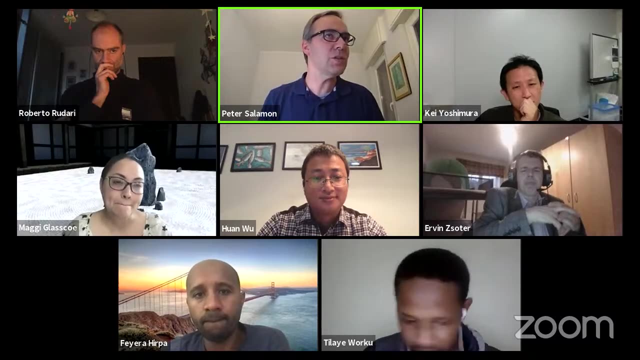 they're usually done at large scale. They're really, yeah, they show a different type of information, And hence what I'm really interested in. do you have an example of how, then, a user put them, use the information to make decisions? And, yeah, this is something which I feel is still an. 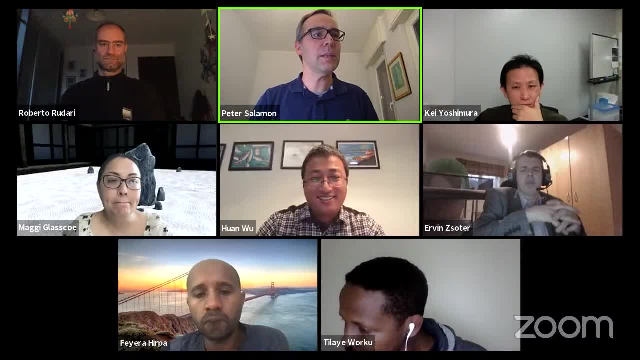 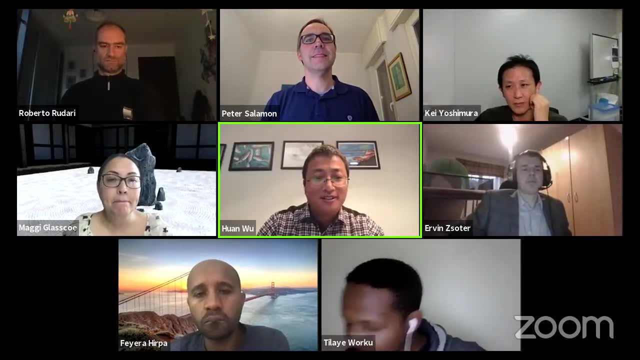 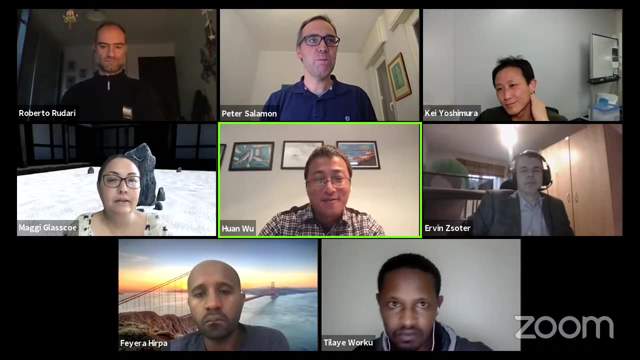 area of work. So, Juan, do you have an example on that? Okay, thank you very much, Peter. That's a very good question, which you actually put me on the grill. I don't have really any example yet, But we do have some thinking about that. 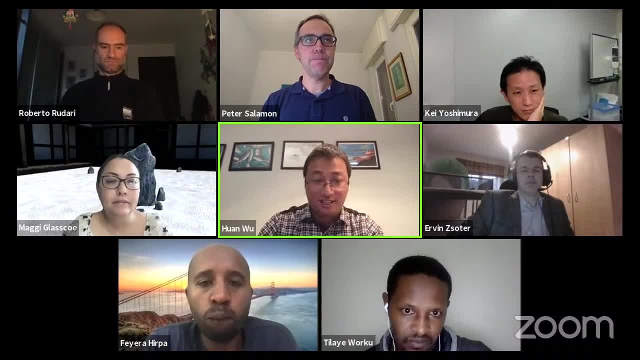 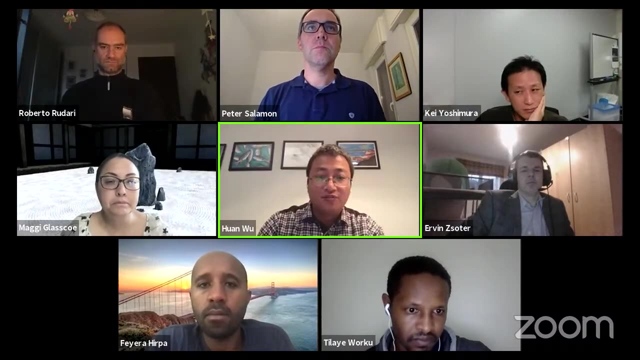 And this, apparently, this is our first step. The first step is try to quantify these kind of relations, which could be very solid at real basin scales and even further at a subcatchment scales, So we can use that information for those individual basin by basin. So, but the question: 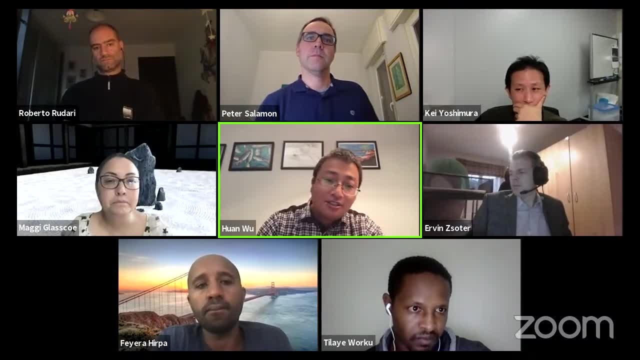 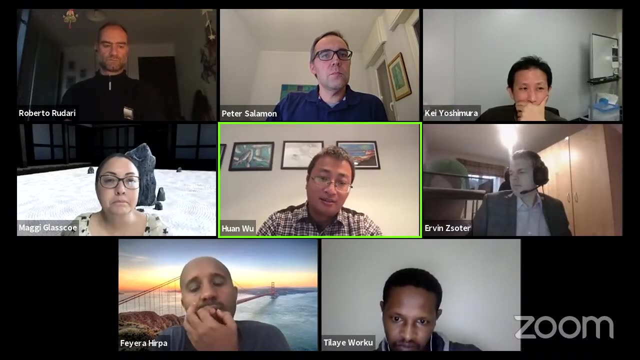 is how, and there are some literature work that has been nicely done there And we have some studies that show that we could do that statistically or using that to constrain our dynamic models. at least there are multiple ways to do that. I think that that's in our next to-do list. 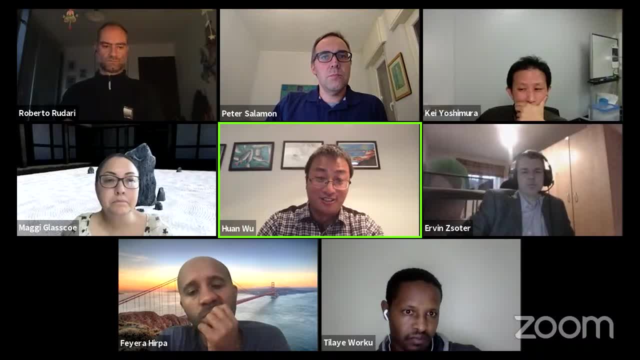 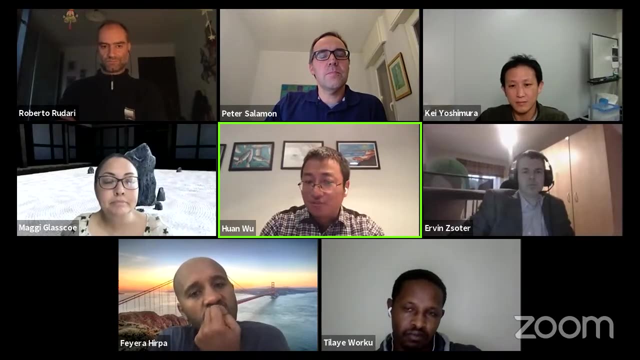 Hopefully, like one or two years, we can have some examples for you. I would not overpromise that, But we at this stage I would really encourage more colleagues to actually do the similar work, replicate it. We can use different results using different models, even observing data, So we can really 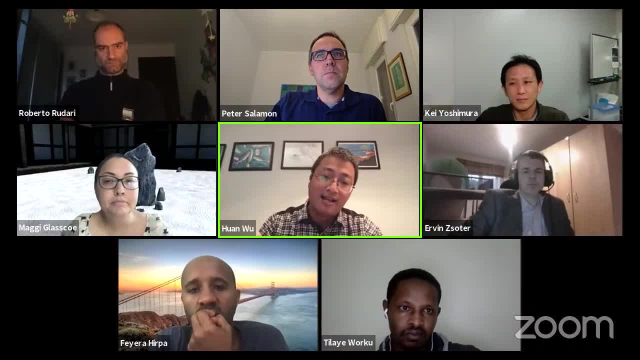 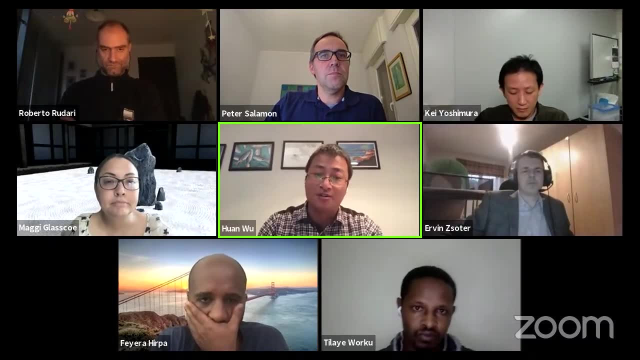 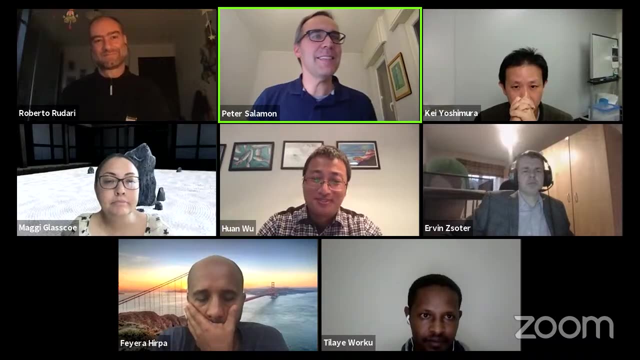 have a confidence of this kind of information at a basin scale That can come into play, like even machine learning methodologies, Those kinds of knowledge that we can put into our models. So again, we don't have any example yet. No thanks, Yes, indeed, I mean, I'm looking, we're looking forward to your next steps on 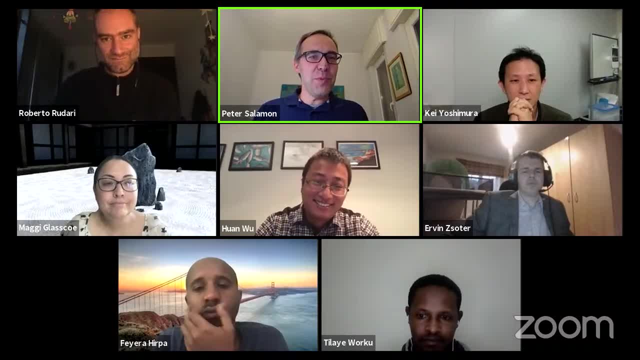 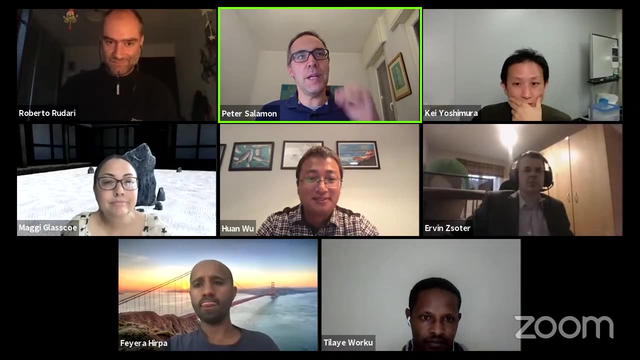 this, And I have a suspicion that we will get more and more examples also from other researchers on how to use the seasonal in terms of within flood risk management. So thanks, Juan Roberto, back to you. Yeah, I mean, we are fast approaching, I mean, I would say, the end of the session. 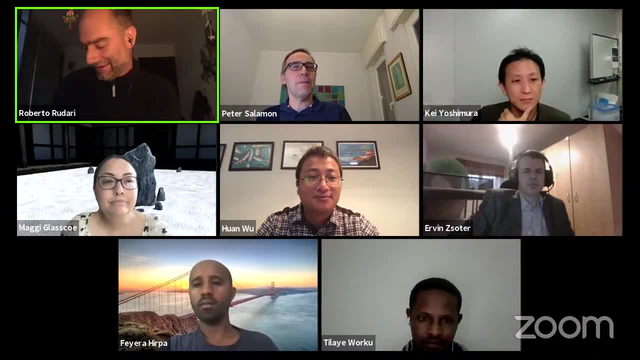 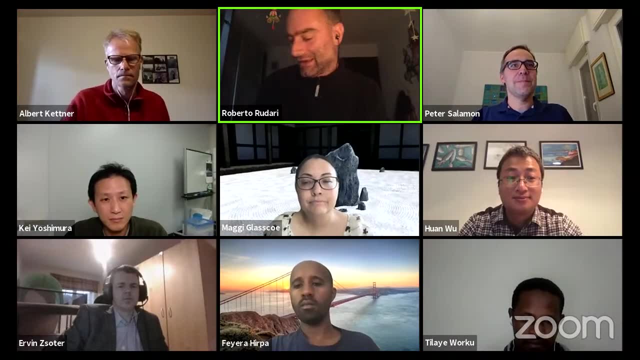 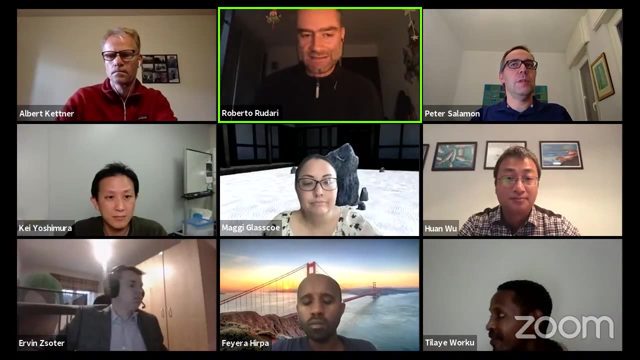 So I will actually, I mean, ask Kay one topic or question. let's say that is, and then I will pass it over to you, Peter, maybe I mean for the closure, Kay. actually, I mean, I think I mean here we had like yet another great example of you know is, let's say, availability of global flood models. 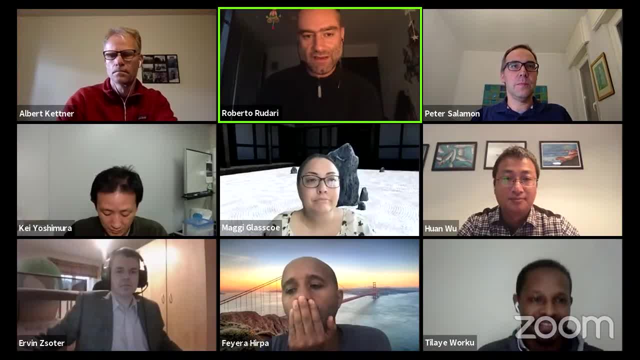 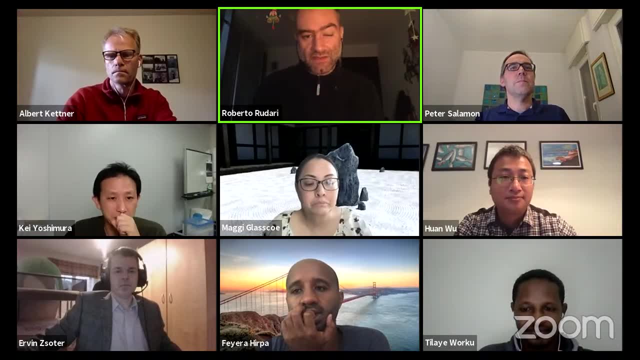 I mean, we've seen GLOFAs and we know, you know, the global flood monitoring system as well. I mean from From US, and your ones is the third one. So my question is, what is the policy of accessibility of, I mean of today's earth, and being in love with the idea of the model of models that I mean Margaret, I mean showed, I mean in the first place? 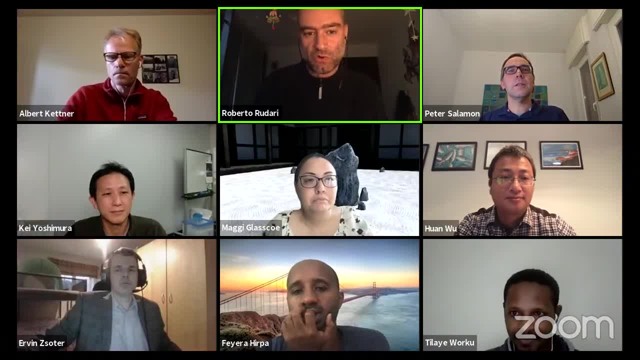 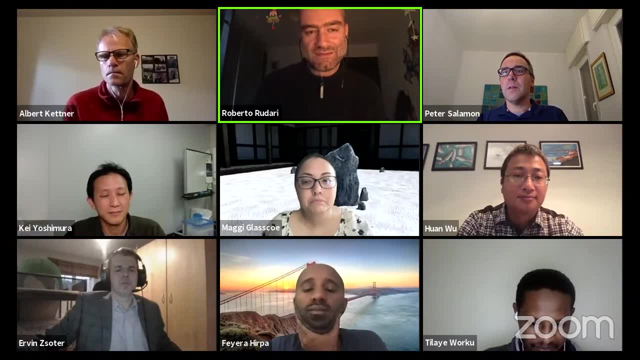 I mean if you have plans or there could be plans. also, I mean to augment, for example, the model of borders. I mean assemble, using, you know, today's earth And you think that is feasible. I mean 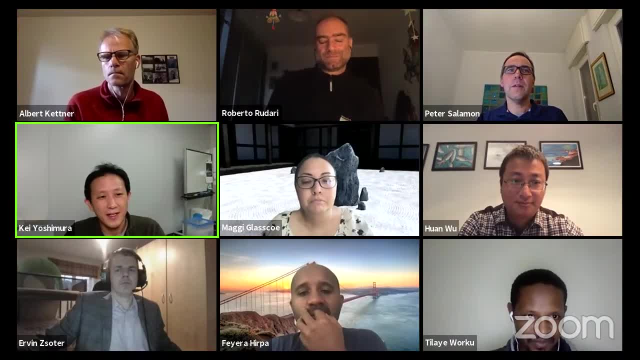 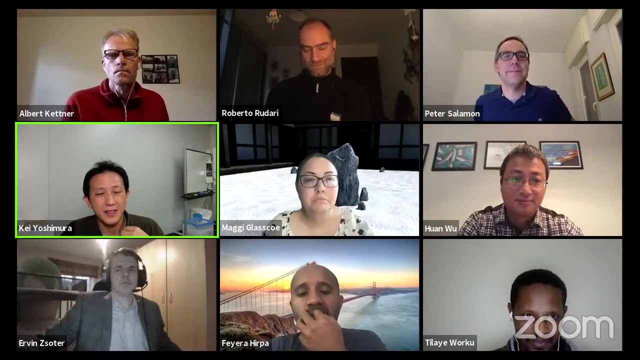 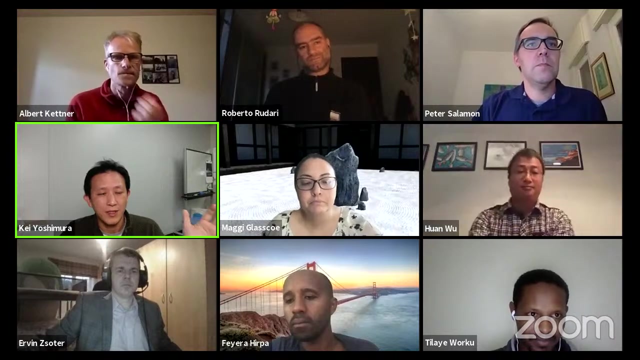 Is that a possibility or not? Okay, thank you. Yeah, that's a good question. And then we are thinking, I mean, basically the approach is very similar, I guess. And then so well, I mean so basically, the data policy is we are trying to provide those data available from and downloadable. 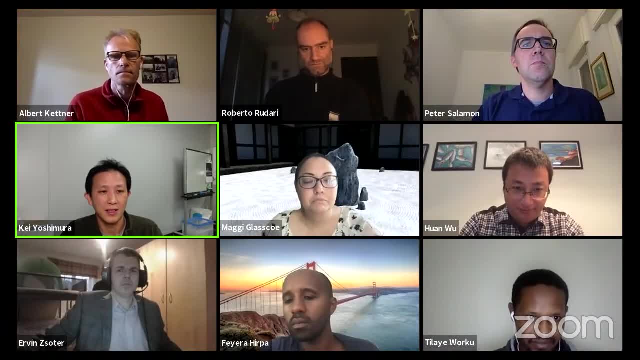 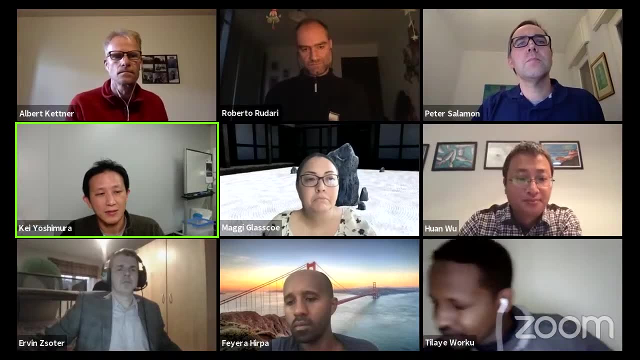 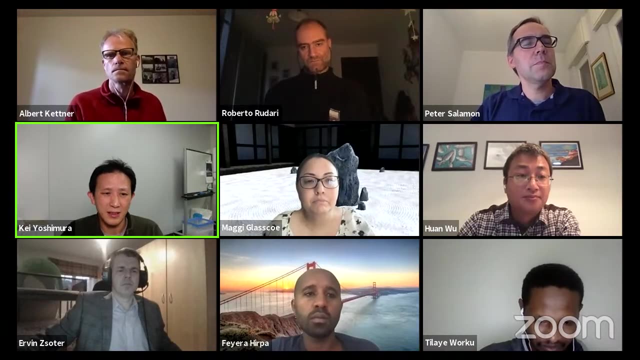 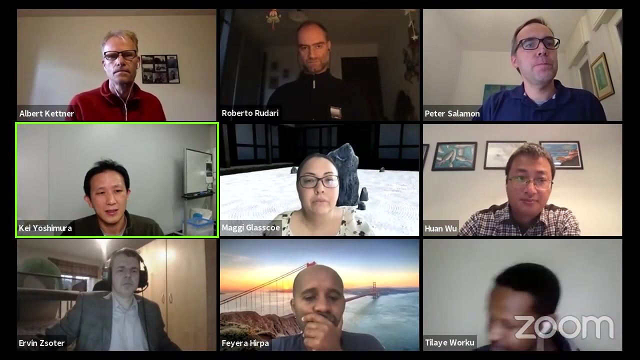 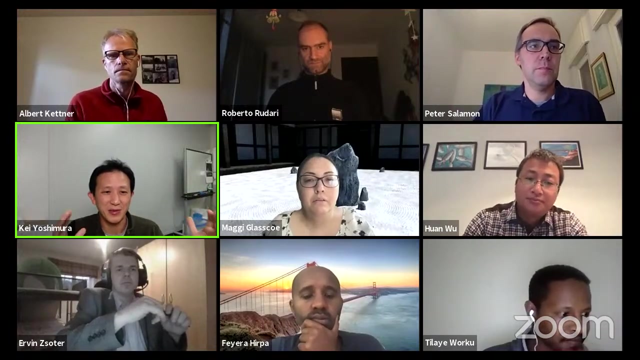 And also can be shown in the website as well, and free user registration. And then also for the special collaboration, I mean because it's kind of restricted to provide the forecasted data currently. So we are still working on that, but we cannot provide the information actually for Japan. 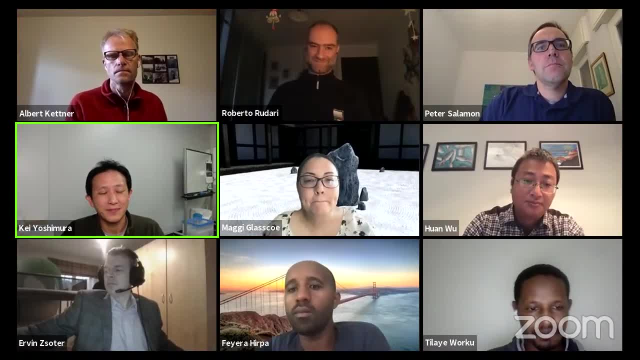 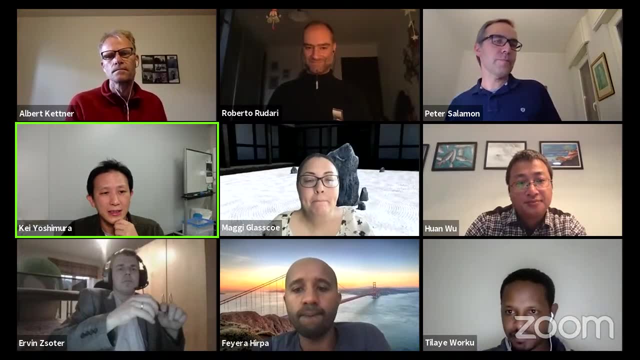 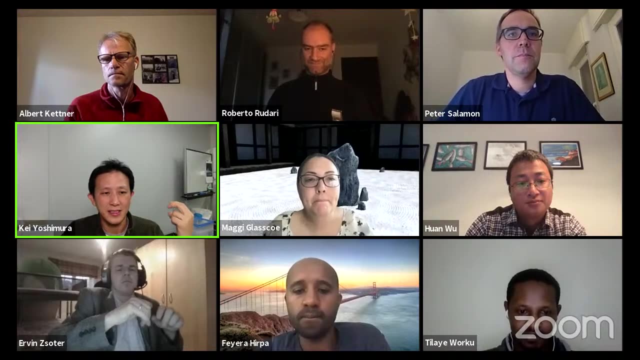 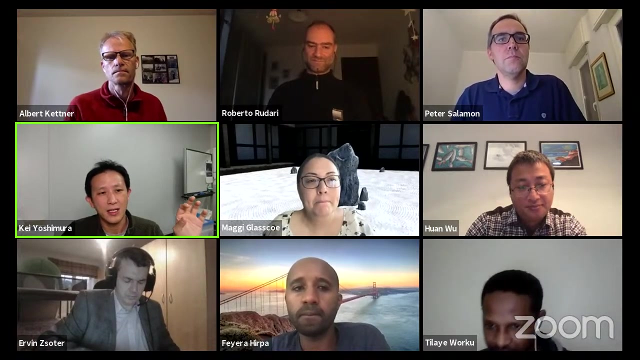 Outside of Japan, it's possible. So we are trying to work on that. But well, and then also we are trying to improve the system, And then the one thing I would like to emphasize is the seamless of the model framework. So 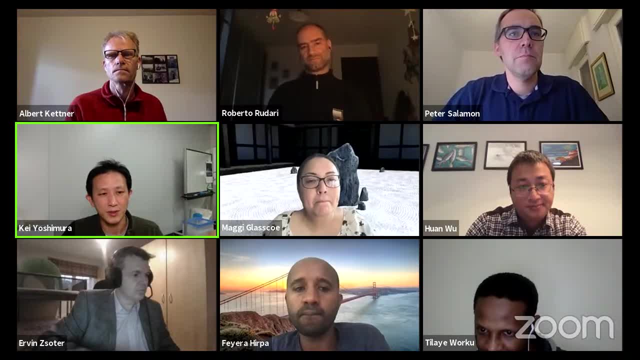 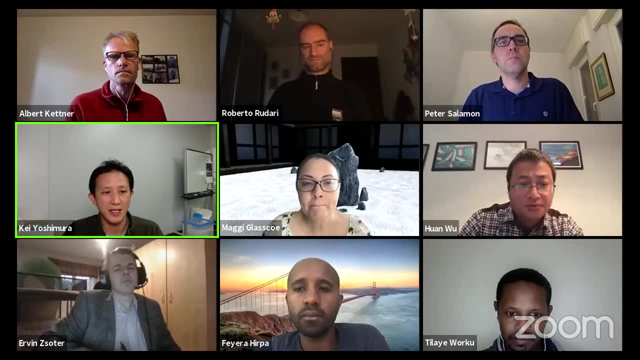 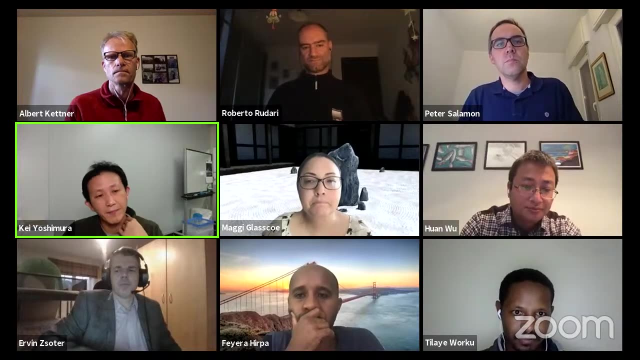 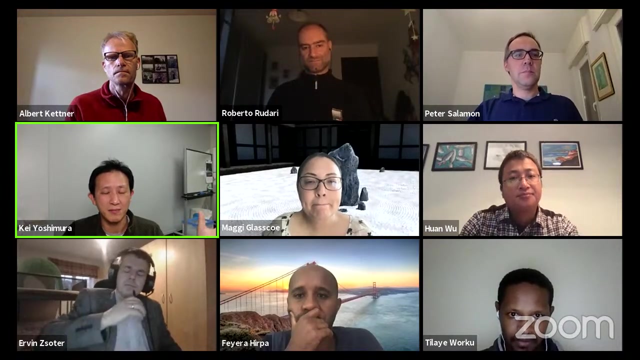 we are trying to use the same models, same set of models, for global system and the regional system. Regional system can be downscaled into one kilometer or an even higher resolution is quite easy. So academic side, actually it is really interesting because there was a kind of academic 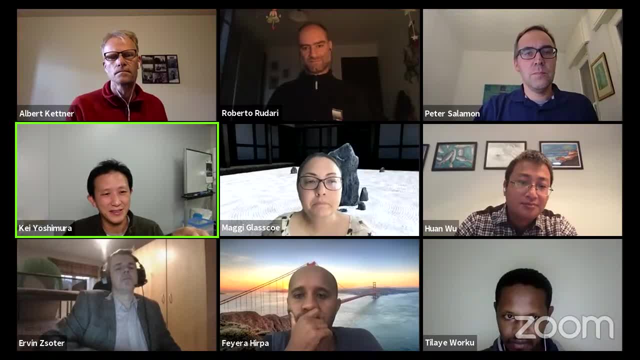 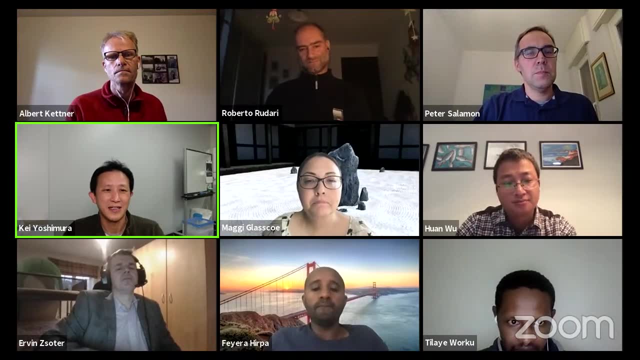 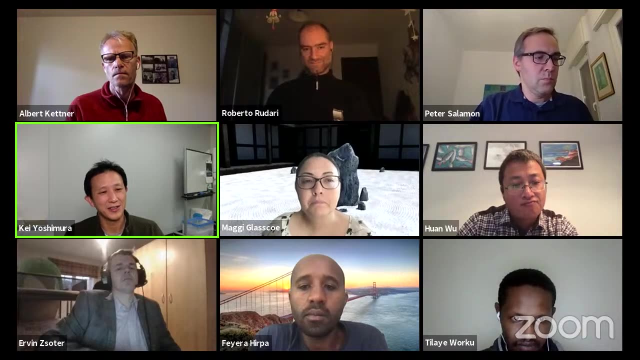 yeah, between the scale, scale, scale scale, I mean Rick Bezant's scale hydrology and the global scale hydrology. and then there was a kind of debate, but that still, I mean we are, I mean actually both directions are. 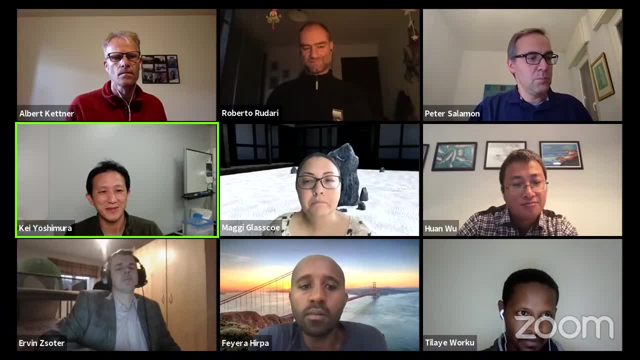 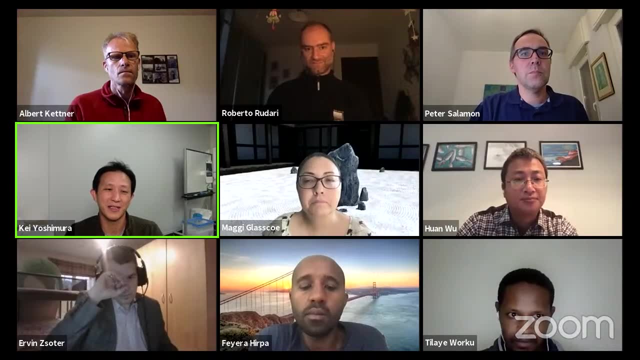 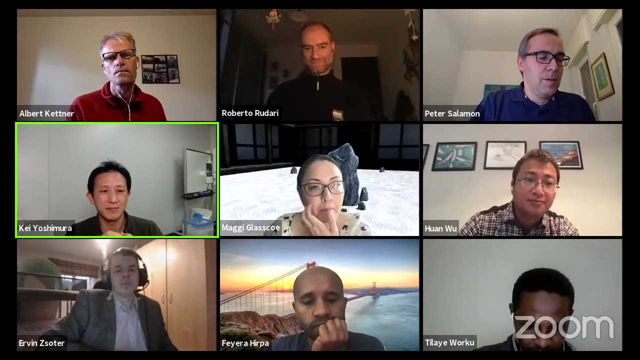 you know, proceeding towards the same, and then our regional models also extends to the larger area. I mean global skill is can be, is now getting a higher level up here, a higher resolution. And then I mean we are trying to make our model system capable to. 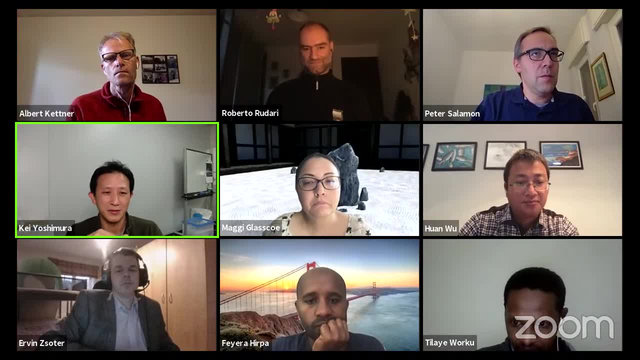 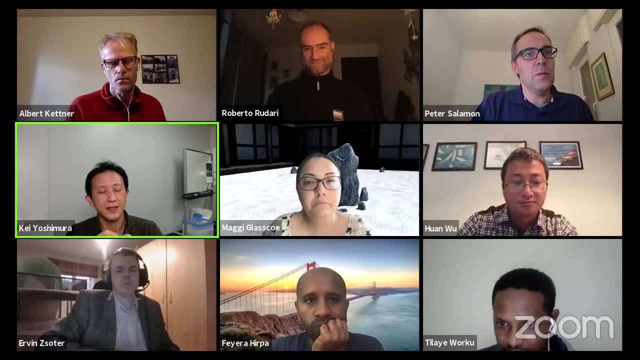 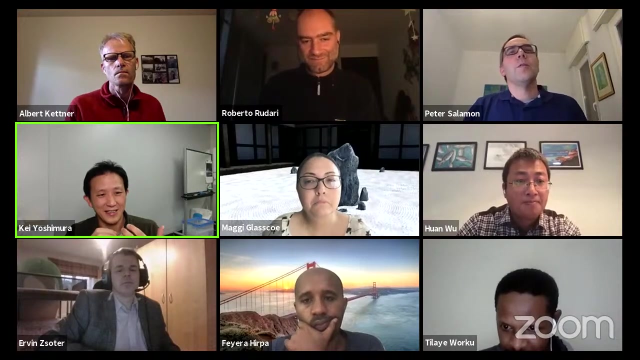 or feasible for the very high resolution as well. So we are trying to extend that kind of system or specific region, if there is some means, over those regions like Japan, which is. but that's our kind of, maybe some of the answers- I mean answers to your- some of 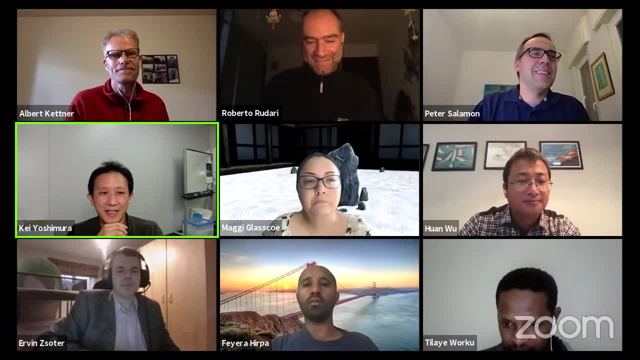 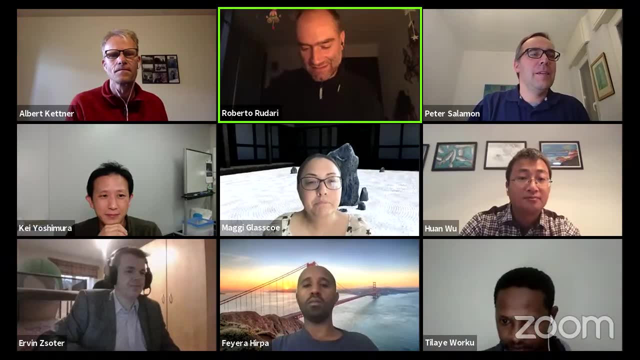 your questions not fully, I would end up with it, Thank you. thank you, Kai. I hope I mean we will. I mean see in future, I mean we see. I mean that the you know the difference between. 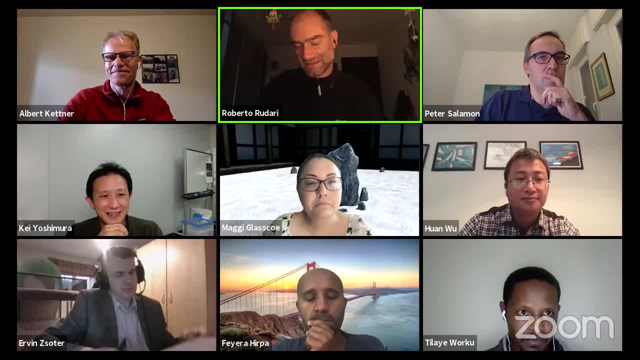 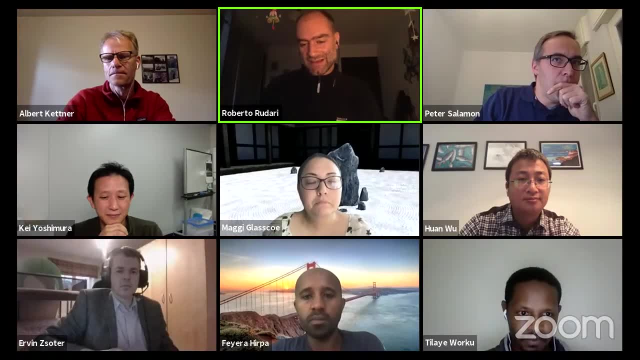 you know the global modeling side and you know the catchment based in sky side. I mean it's definitely. I mean closing up, I mean very fast, So I mean I would say that we are on the right, I mean. 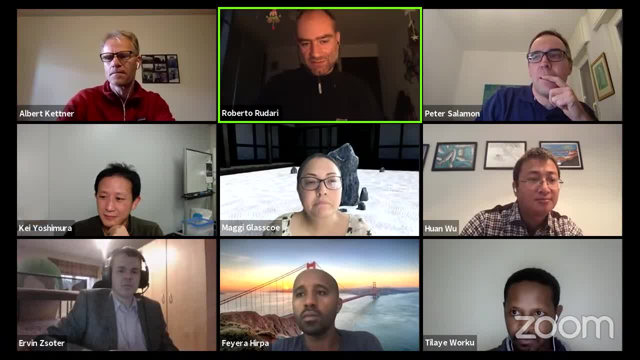 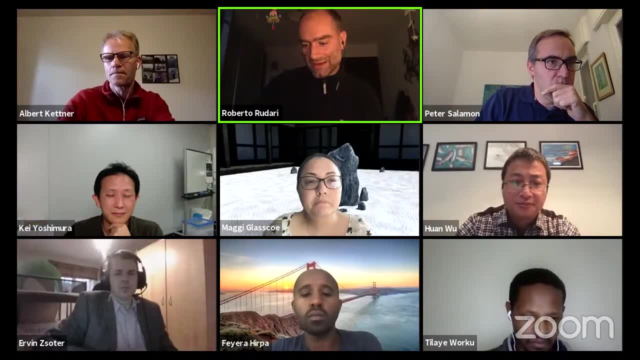 developing in the right direction, also for this community that is mainly involved in the global part. I hope I mean we'll be able also to work on this, you know, data openness, I mean, and that availability and accessibility part, because I think it's important I mean really to leverage. 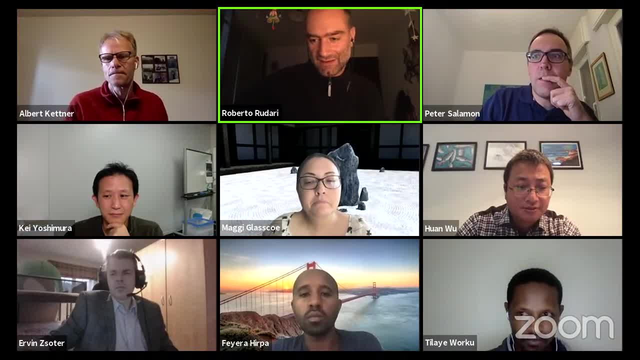 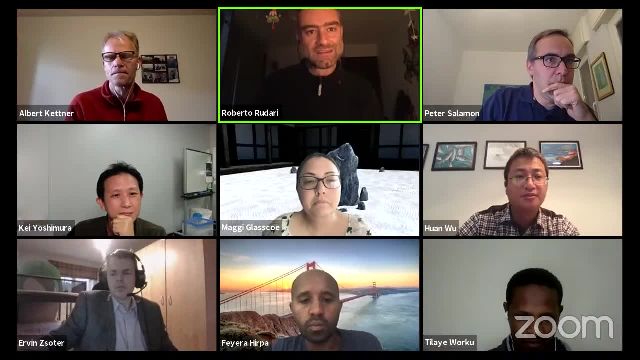 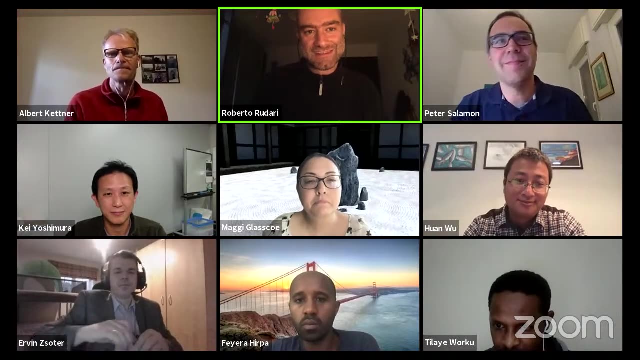 on. you know the level of effort that you've done. Let's say the global community would very much benefit from that, All the good work that you've done. in today's definitely, Peter, over to you for the closure. We are like I mean eight minutes later than expected, but I think I mean we're thankful, yeah. 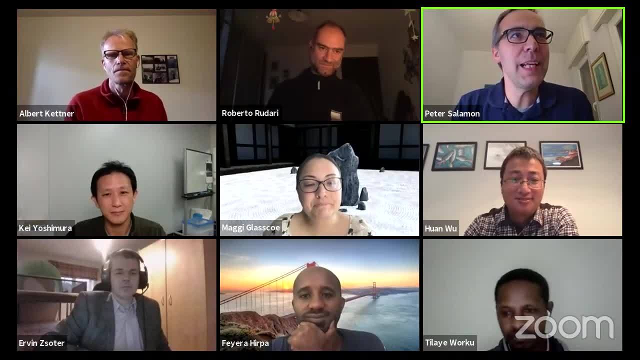 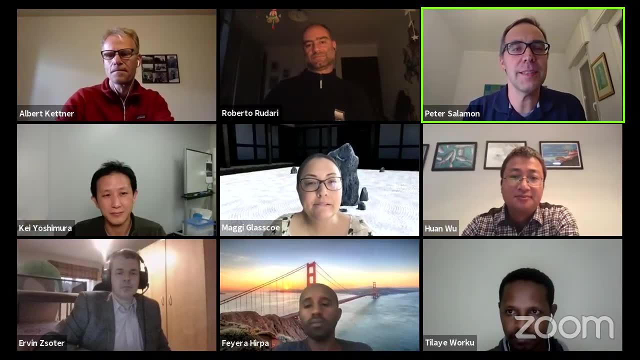 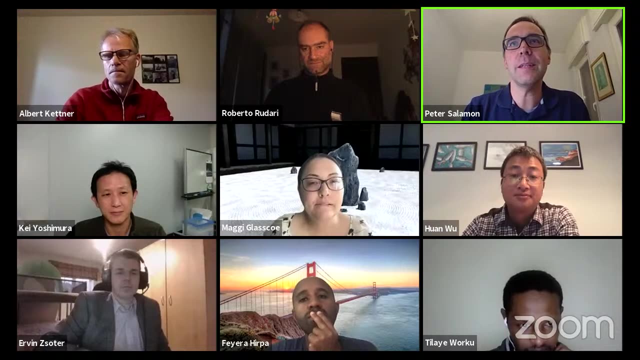 Yes, thanks, thanks, Roberto, and really thanks a lot, especially to the five speakers. It was really great having you in our second session and hearing from you. Thanks to all, thanks also to all the participants. I mean it's really great to see. 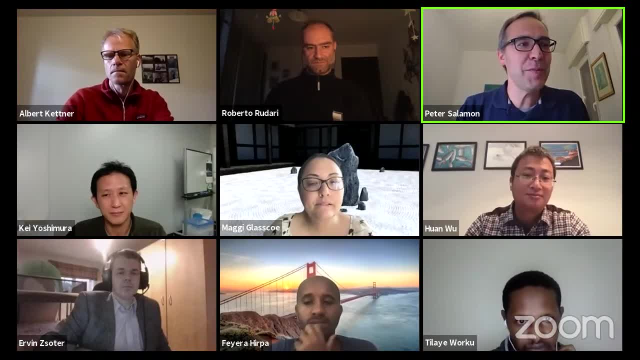 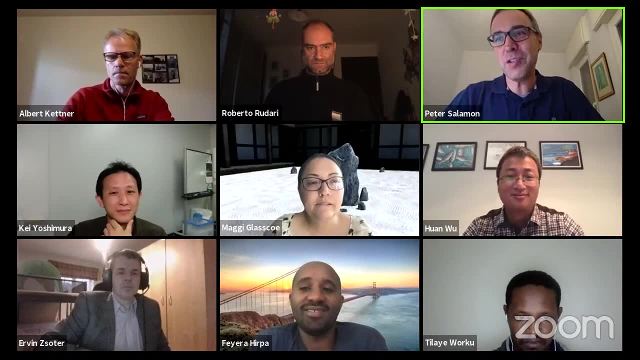 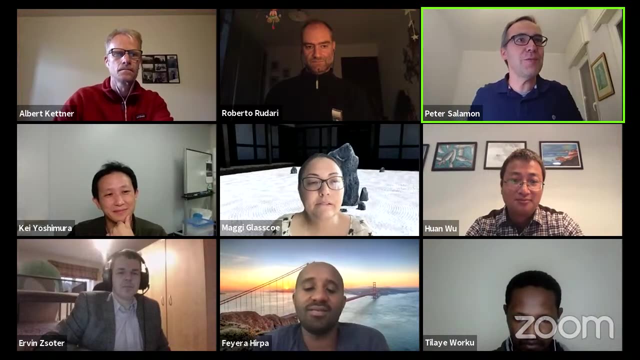 so many of you here. I know for those in the Americas it's an early start in the day. For those sitting in Asia, in Australia, it's probably already bedtime, so it's really great, nevertheless, to bring so many people together and share the experiences and knowledges. 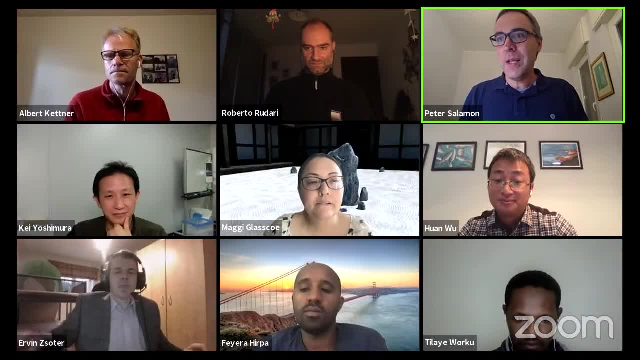 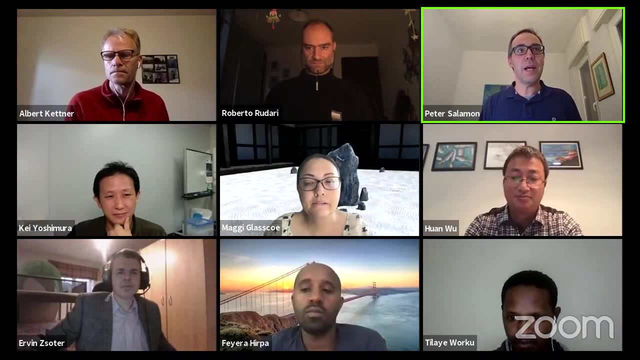 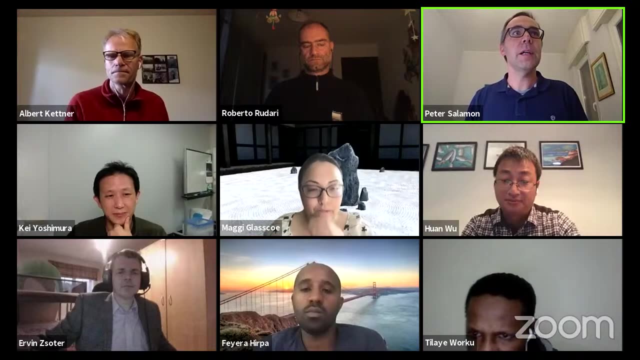 you know about global flood forecasting with you, So I hope you really liked the session. the second session of the GFP. Next week, again Wednesday, same time, we have the third session on flood hazard, global flood hazard and risk modeling, also with a range of interesting 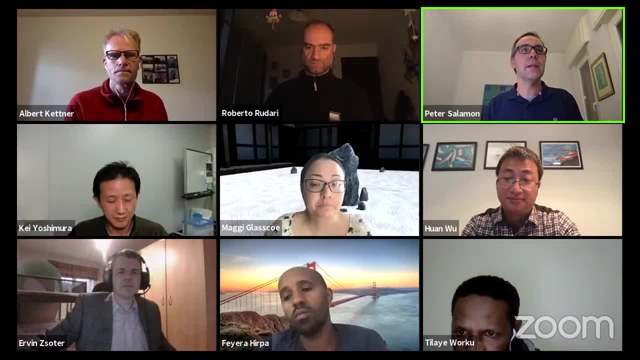 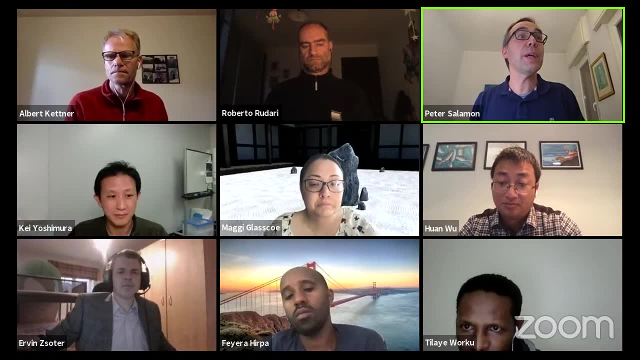 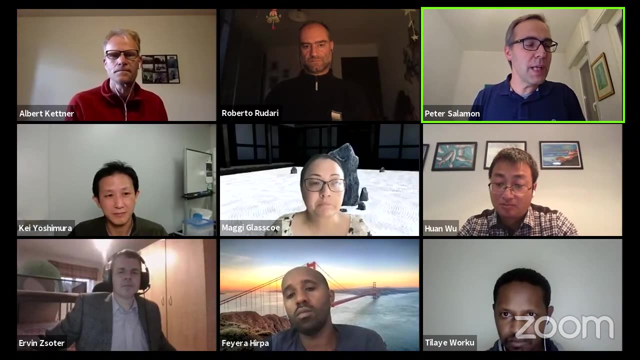 speakers, So hope to see many of you there. The recordings will, as usual, be made soon available. The presentations that I've seen that have been asked as well. please be patient. We will put everything if presenters allow, including the presentations on the GFP website.